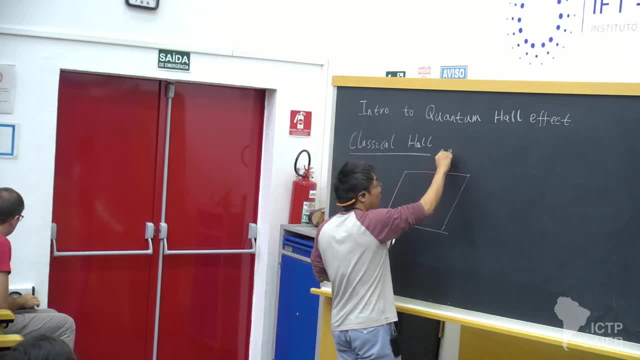 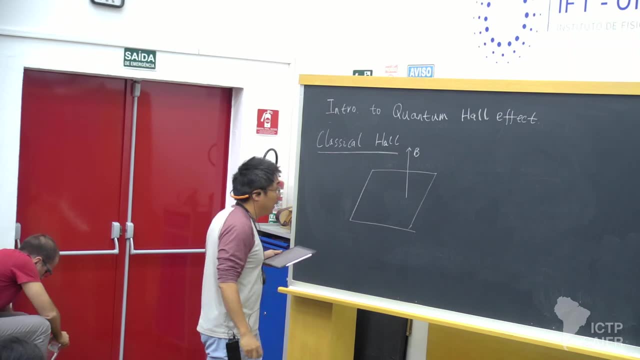 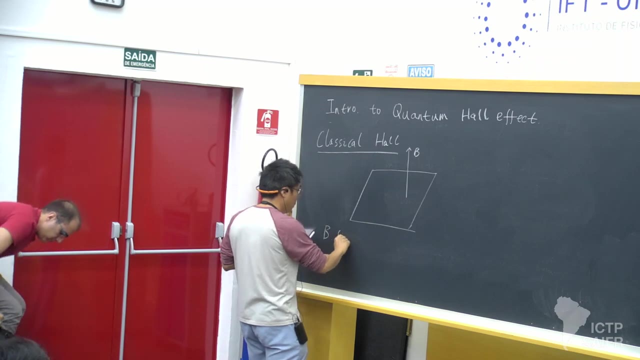 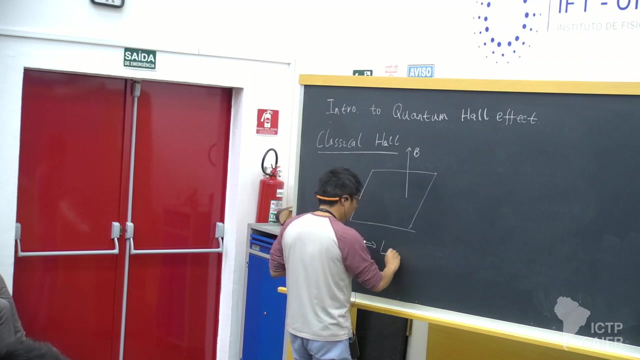 and you apply a magnetic field that is perpendicular to the plane And then the upshot for the quantum Hall effect is that the quantum Hall effect is that the magnetic field, the B field, will introduce a Lorentz force that we learned in high school. 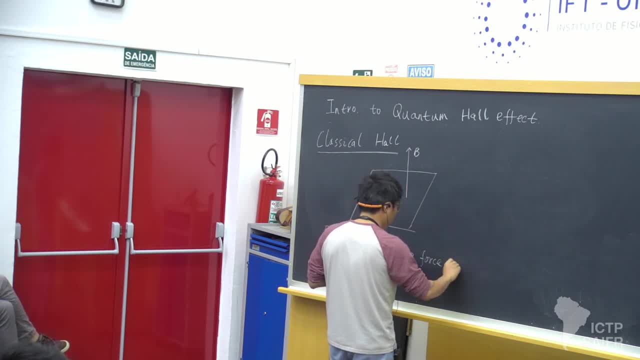 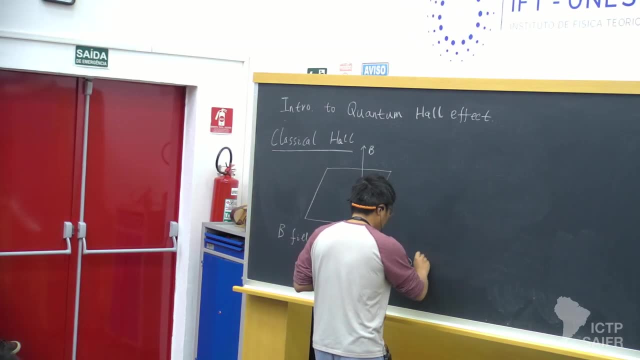 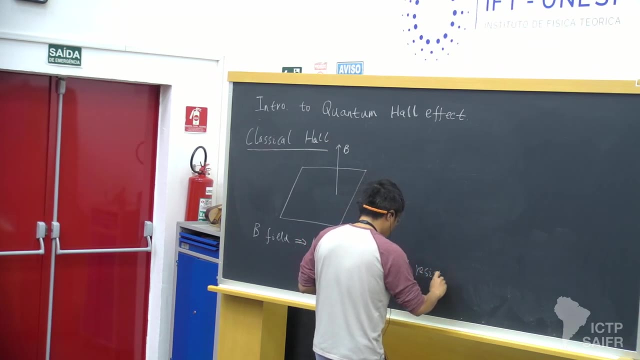 And the Lorentz force, and the consequence of Lorentz force is that the system will have some resistance. that is a transverse. We call it Hall resistance or transverse resistance, And this is a resistance that I will explain in a minute. 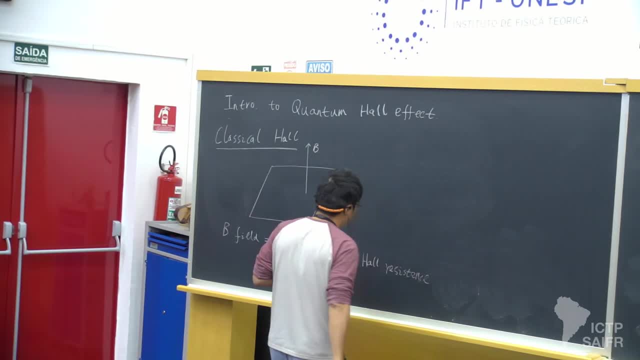 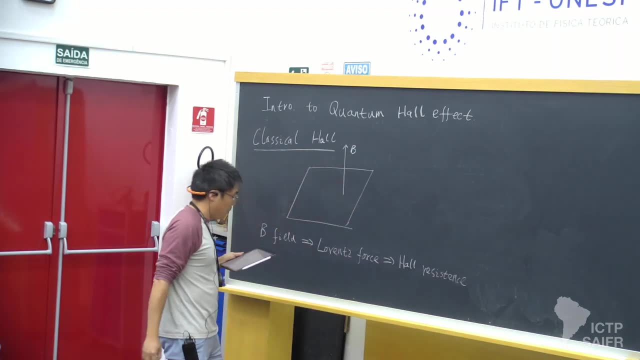 So, and that is what Hall effect is. So let's say the concrete setup is that. let's say we want the system to have a current that, let's say, along the x-directions. This Gx is my current density. 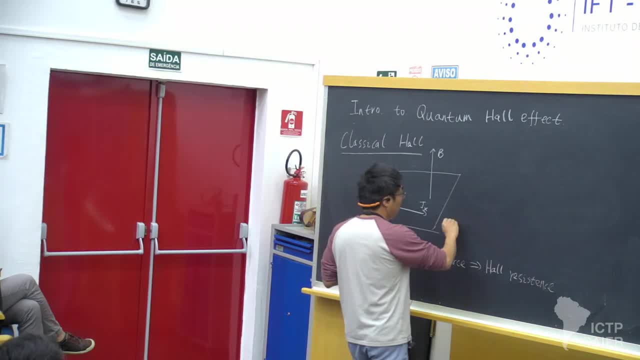 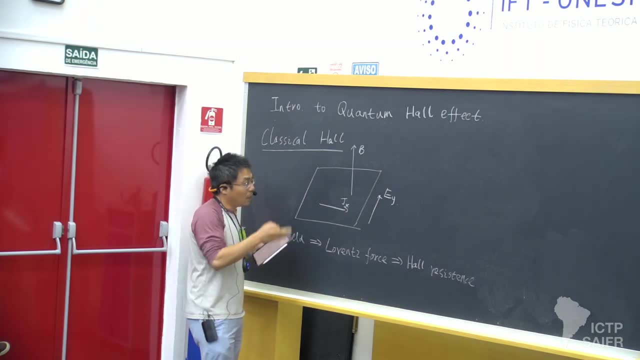 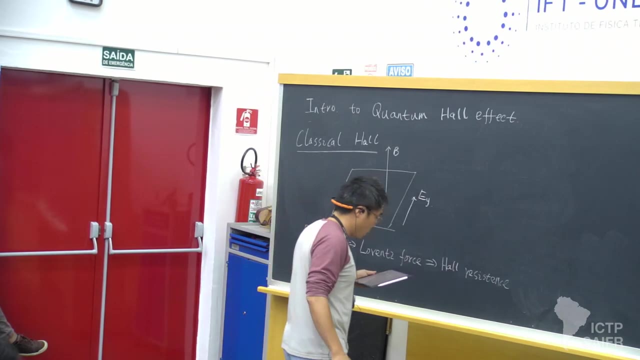 And to achieve that goal, what I need need to do in the end is that I need to apply an electric field perpendicular in the y direction in order to compensate the Lorentz force right. That is something we learned in high school, So we can try to be more concrete. 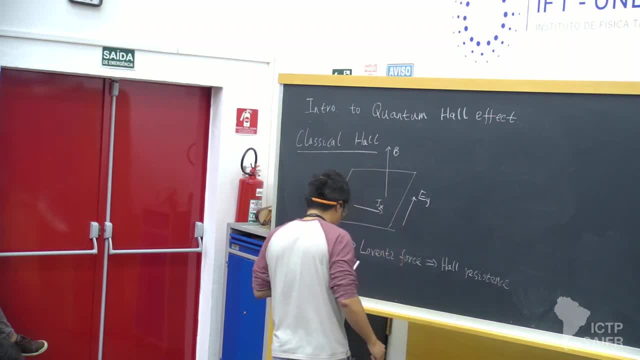 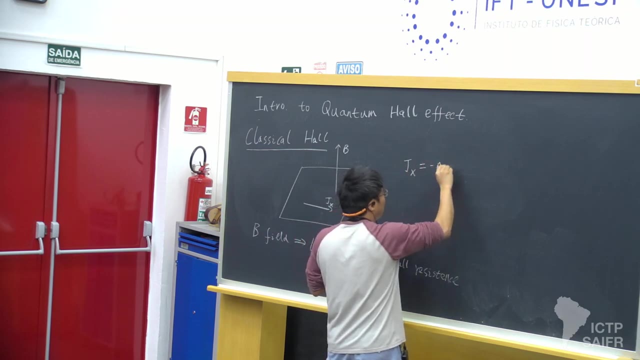 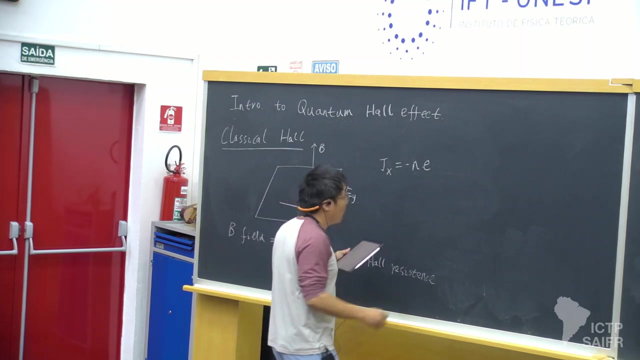 about this physics. Let's say we have this current density and then the current density can be written as the number, the density of the carriers, that is, electrons that can carry the current in the system that I will call n, and then times the electric charge and then times the. 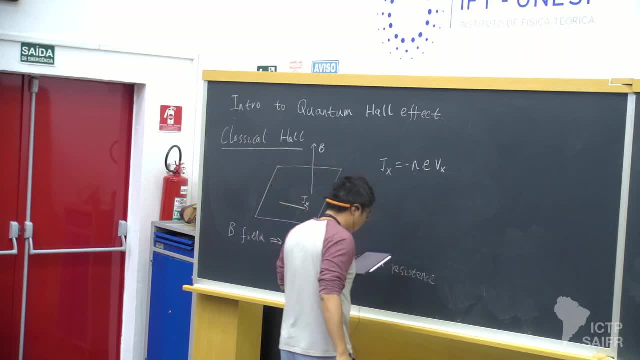 velocity of the electrons that I called Vx right. And then what we know is that on each electron there will be a Lorentz force right as well as a force come from the electric field right, And the force will be minus E times EY. 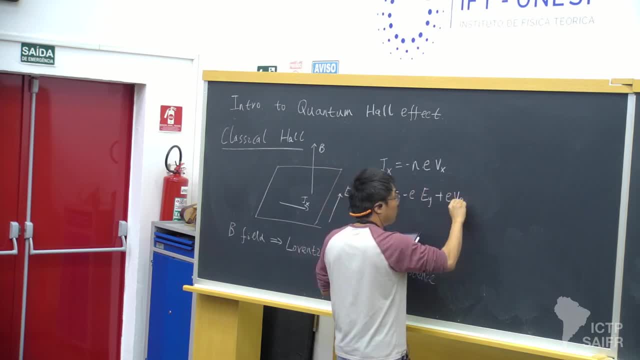 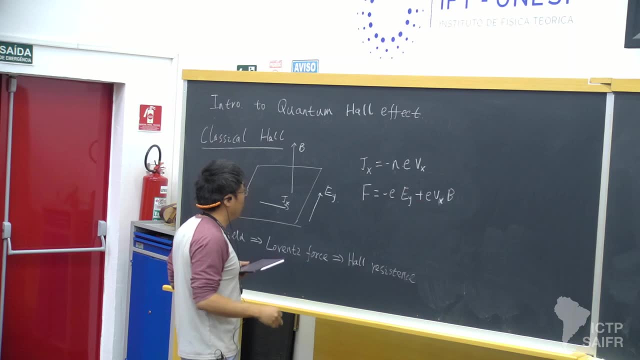 and plus my Lorentz force right, So sorry VX times B. And then, in order to have this current, then what we need is that this Lorentz force go to zero right. This gives me a relation that is my electric field. 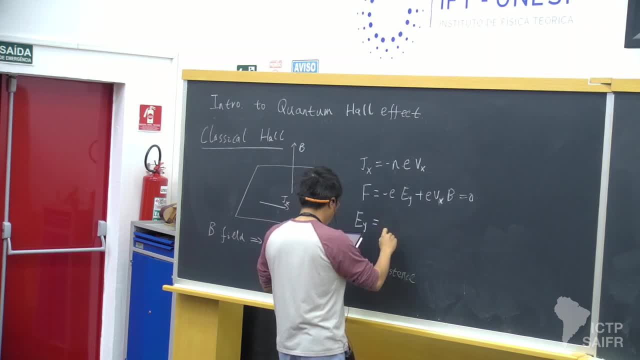 should equal to VX times B, that is, minus JX over N times E, and then multiply by Magnetic field stress. right, That is what we know from high school, And then what we can do is to compute to the so-called Hall resistance. 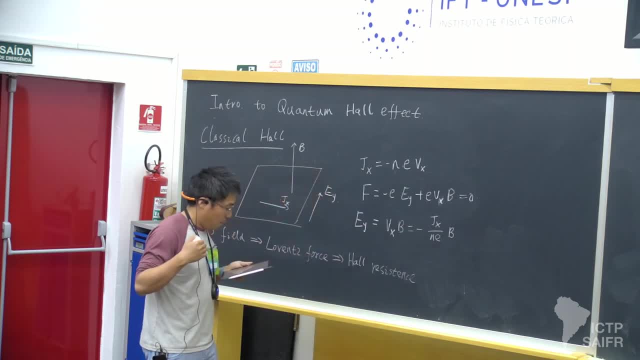 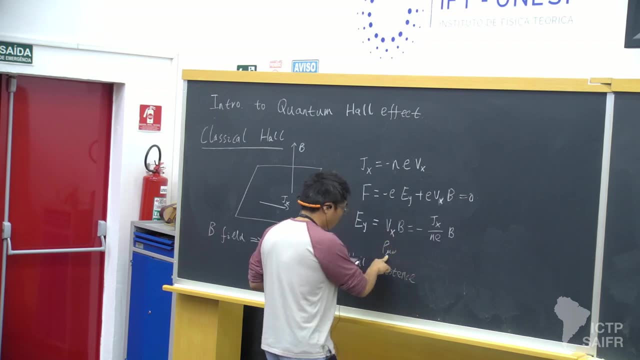 which, in general, we can define the resistivity as a tensor or a matrix that takes a value that I will call rho of mu nu and with the mu and nu take value as X or Y. that's really just my Directions on the plane, right. 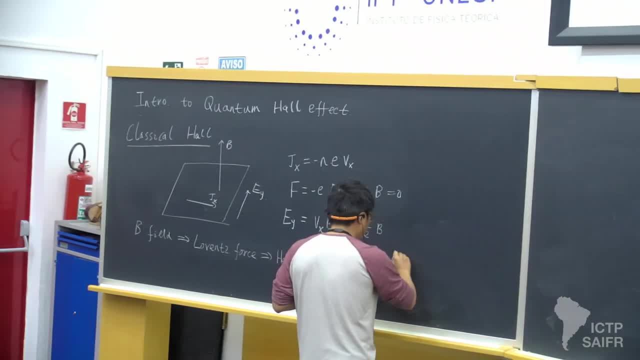 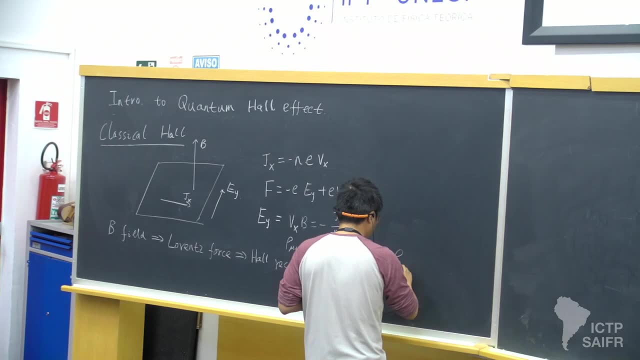 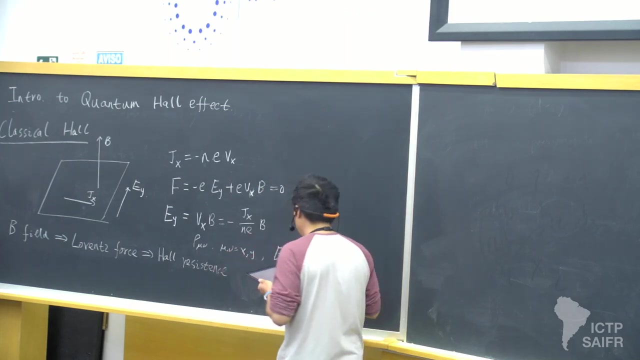 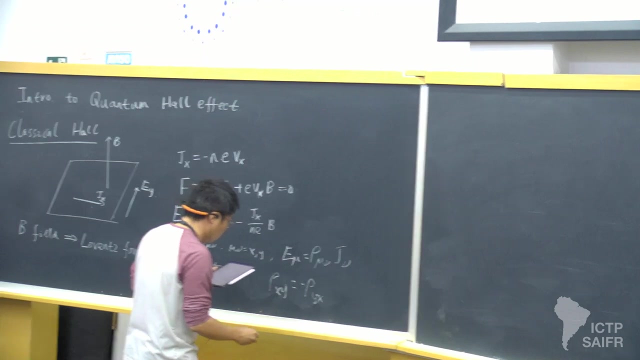 So then we will have this Ohm's law, that is, my electric field will be equal to my resistivity, tensor times the current density. right With this relation, what we will end up with is this Hall resistance, which is an anti-symmetric. if you exchange the X, Y, 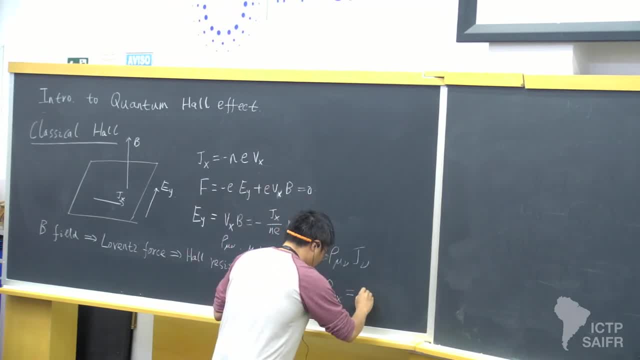 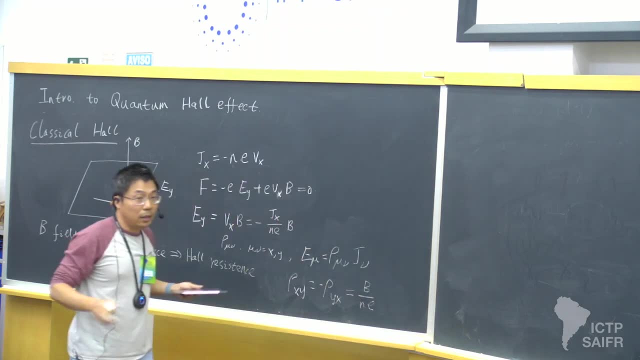 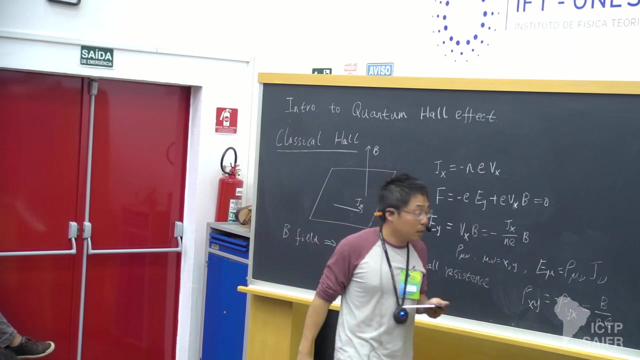 and it will be B over N times E right, That is what we learned from high school, By the way, so feel free to interrupt me at any point. ask any questions you would like. Okay, So that is the Hall resistance. 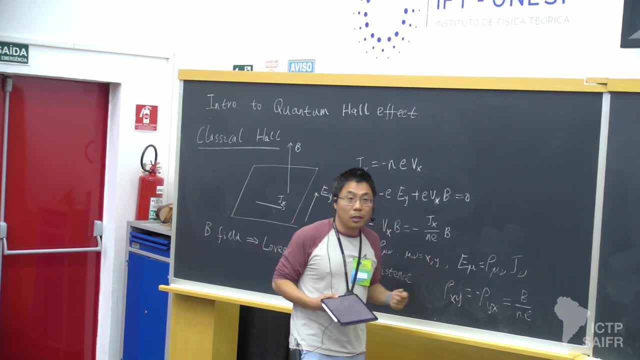 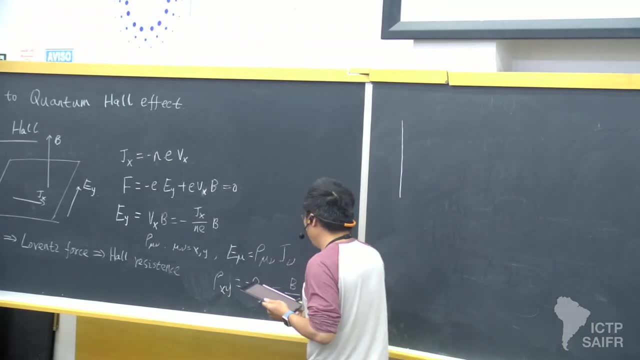 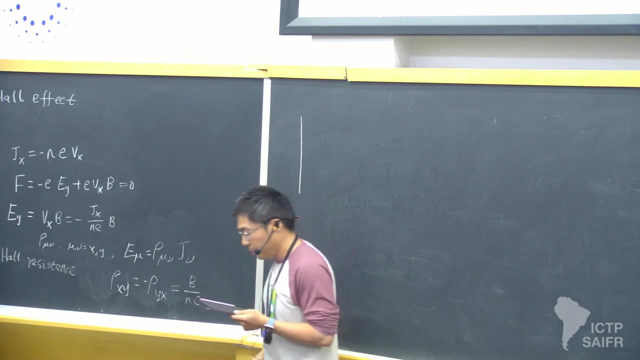 So this is the Hall resistivity in a classical world, right? So we can draw a plot. So the thing you would notice is that the resistivity is really proportional to the strands of my magnetic field, And we can draw a plot that is on my X axis. 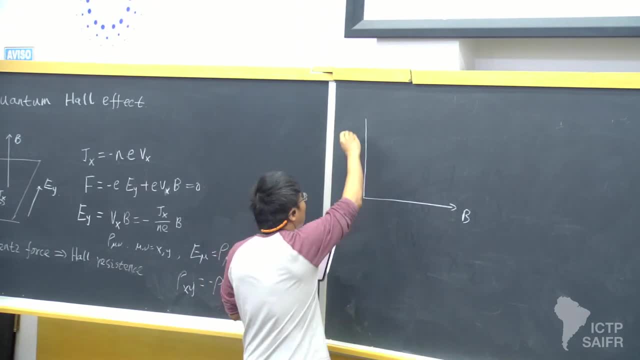 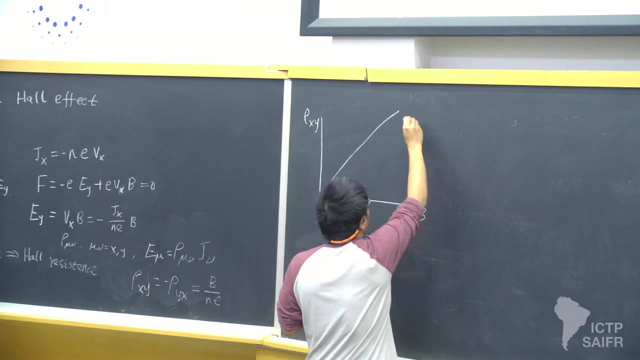 I have my field strands and on the X axis, Y axis, is the Hall resistivity right. And then from this we know that, classically, what you should expect is really just a straight line that has it equals to the resistivity, equals to: 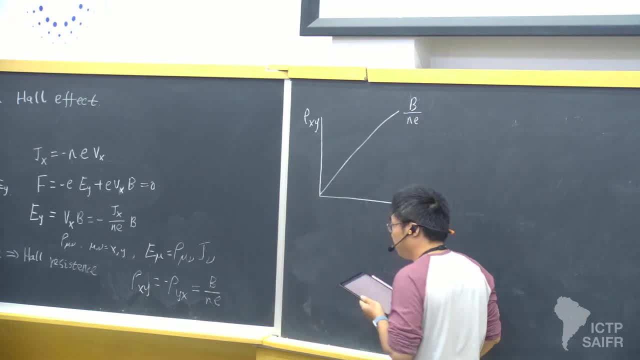 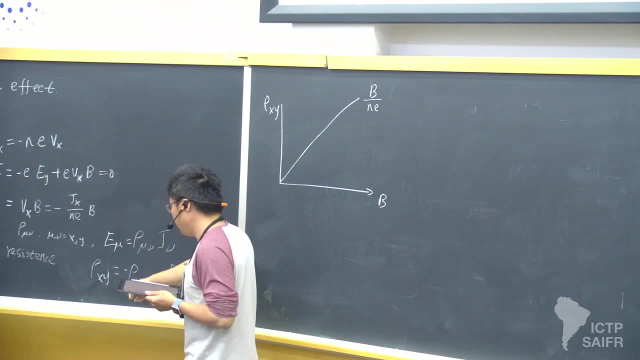 yeah, the slope is B over N times E. That is the classical story. We can also work a little bit harder to get the transverse Okay. So this is the longitudinal resistivity, like rho, X, X and what you will have. 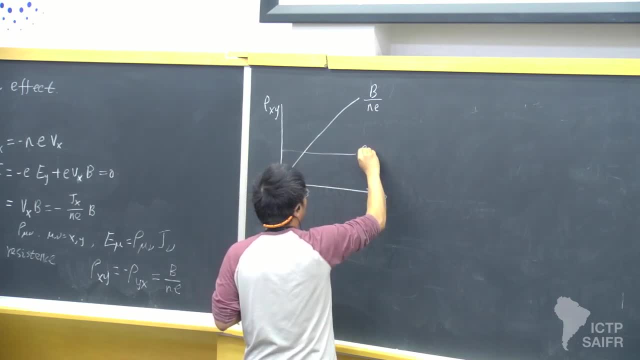 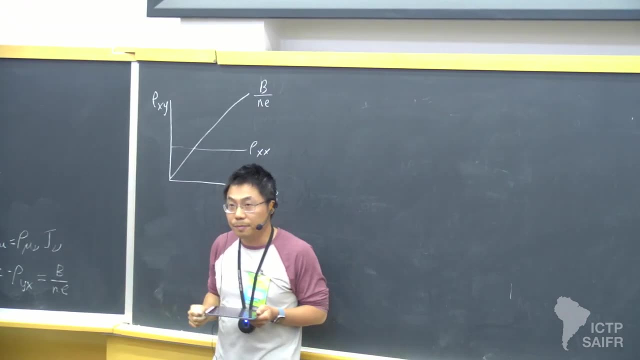 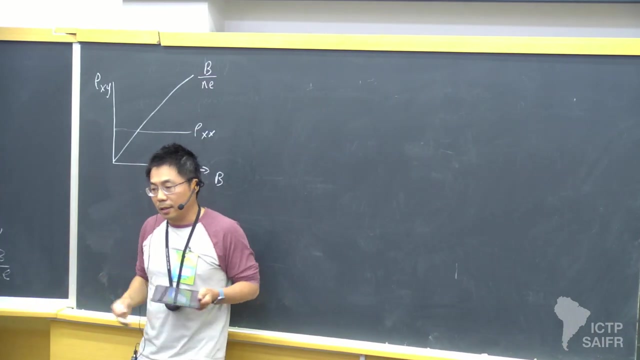 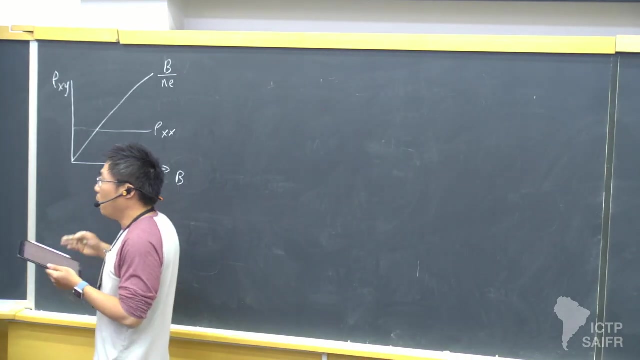 find is actually just stays as a constant that is independent of the magnetic field, right, That is the classical story And as we learned in quantum mechanics, we know that many like classical phenomenon will break down in the quantum world. That's also the case for this Hall effect. 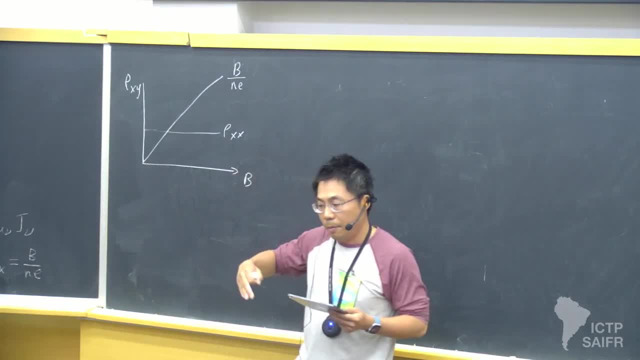 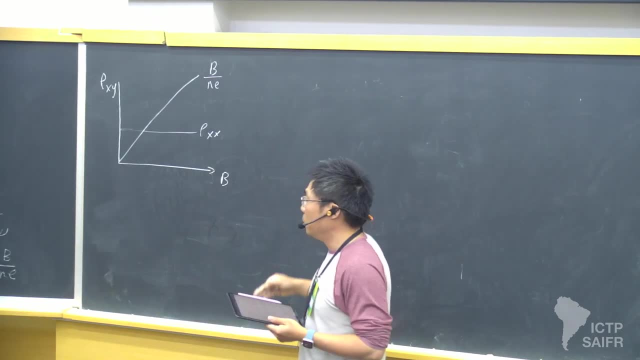 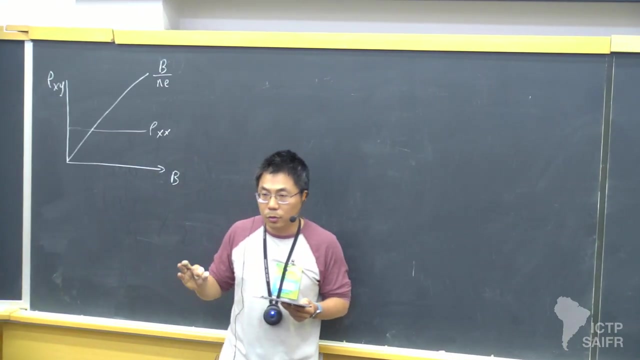 So the thing is, if you lower the temperature of the system to, if you make the temperature low enough, and you look at a region that is has very strong magnetic field, typically around five to 10 Tesla- and then what you will find is that 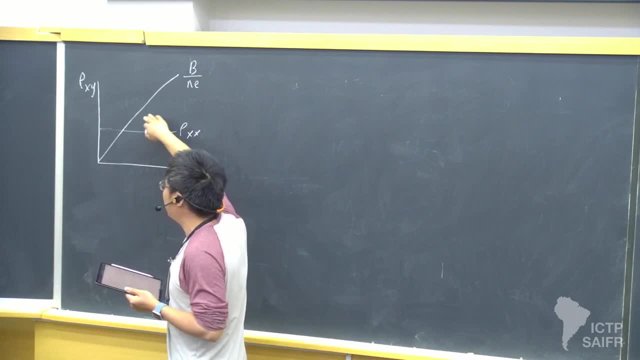 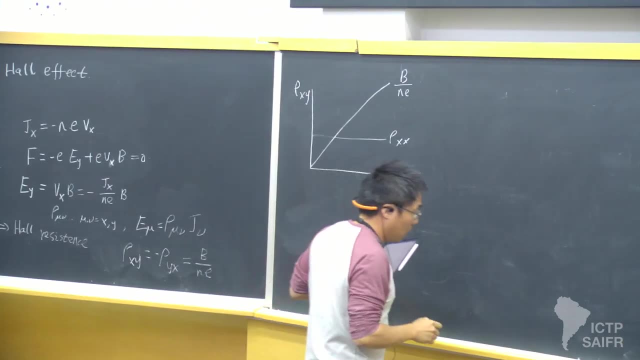 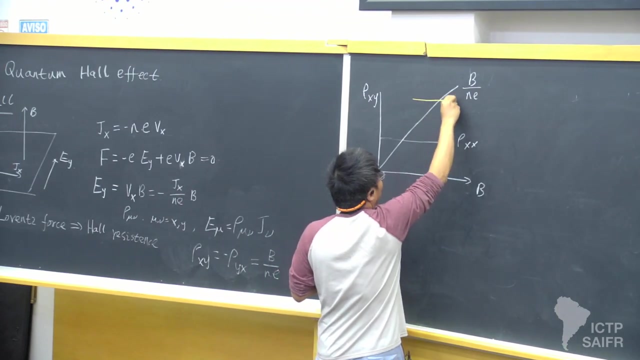 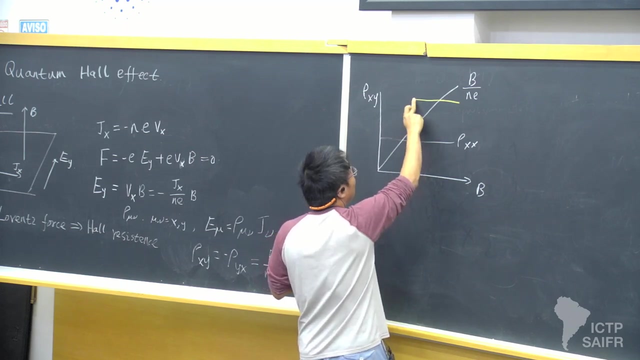 this Hall resistivity starts to develop the so-called plateaus, That is, do I have some other colors? So it will start to say that my Hall resistivity starts to form a pattern like this, So I will say the quantized plateaus. 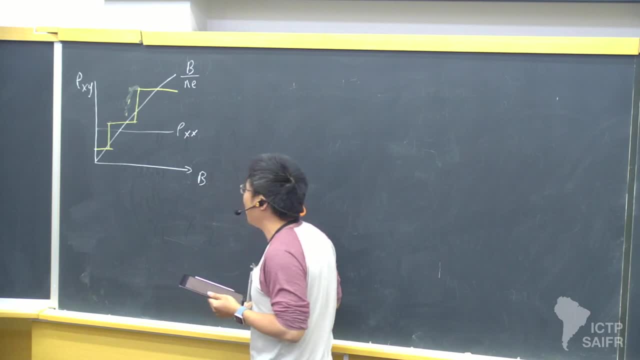 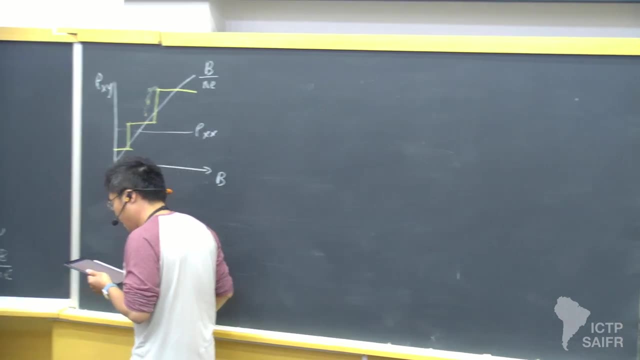 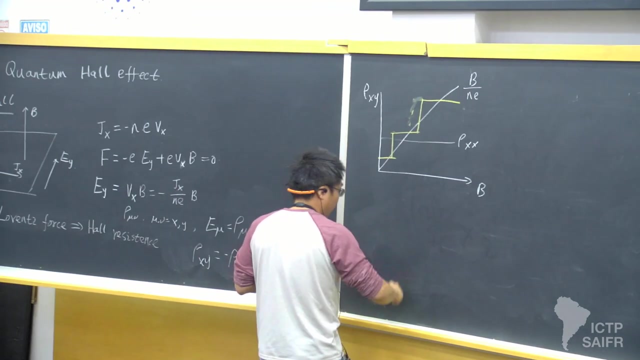 of the Hall resistivity rho X- Y, and then there are multiple plateaus of this Hall resistivity And, more remarkably, the Hall resistivity at each plateaus actually takes a quantized value. that is, rho X- Y equals to two pi X- Y. 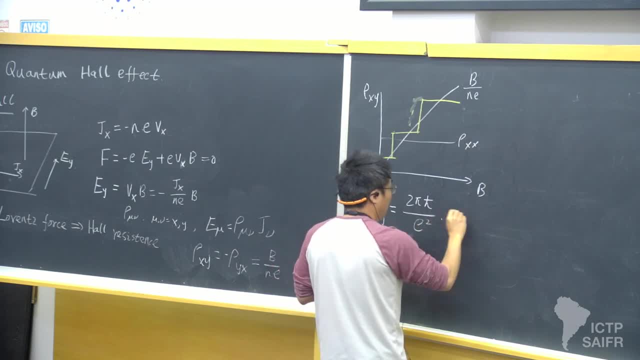 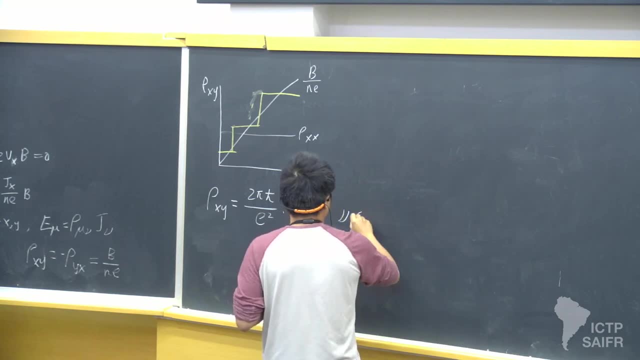 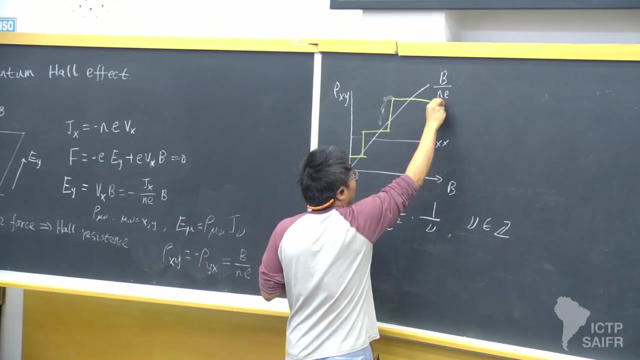 H bar over E square and times one of nu, And this nu is what we usually call a filling factor, and nu equals to integer. So that means, for those plateaus that I draw here you will have the first plateau: equals to mu, equals one. 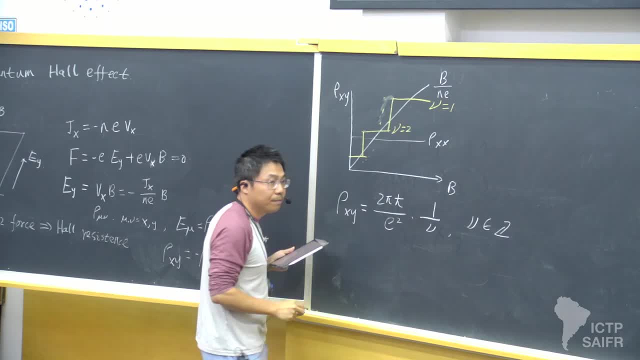 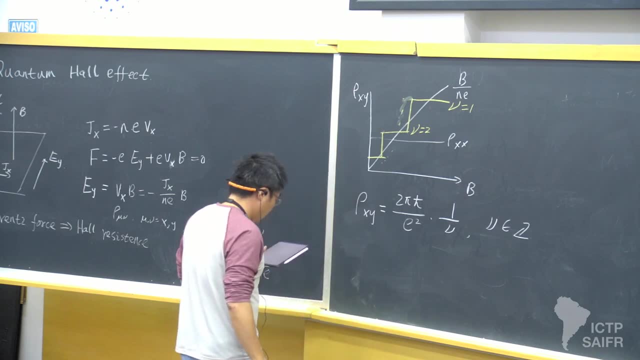 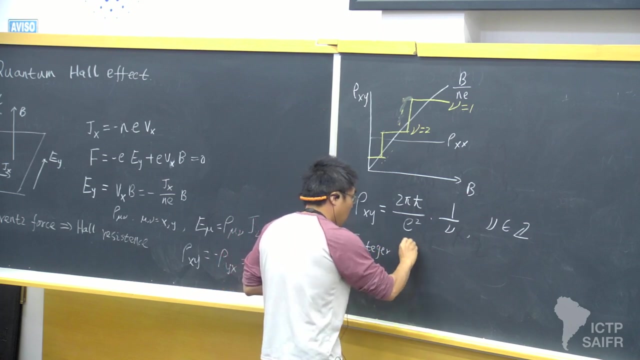 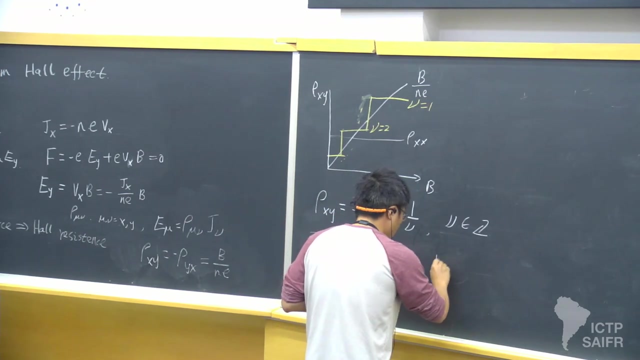 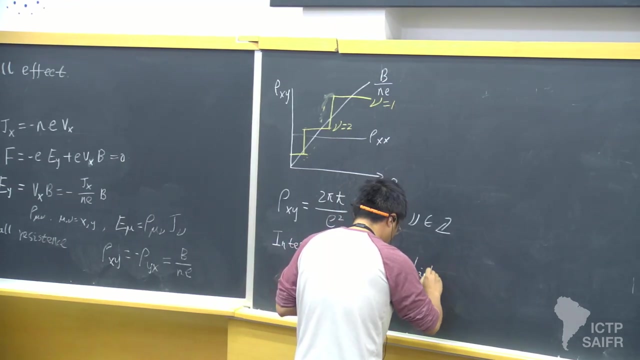 and the second equals to mu, equals two, and it keeps on going. So that is the what we called quantum Hall effect, and it was. that is what we called integer quantum Hall effect, which was originally discovered by von Gleisen in 1980.. 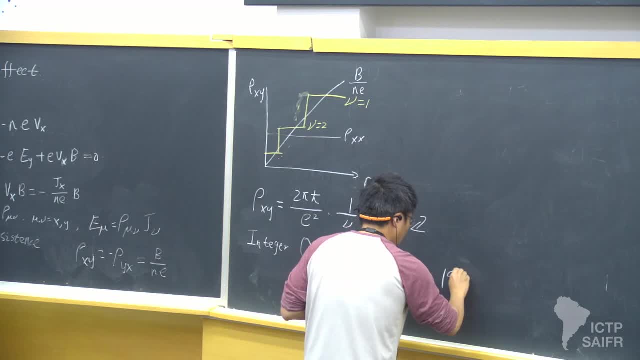 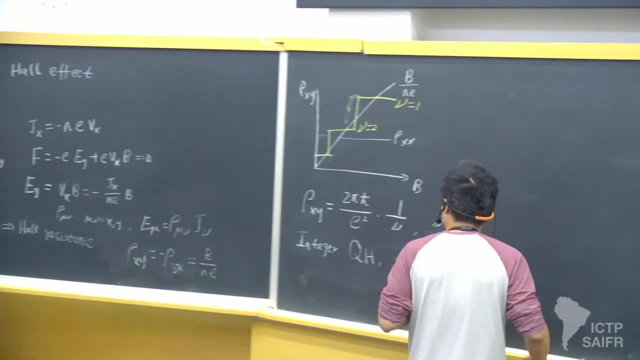 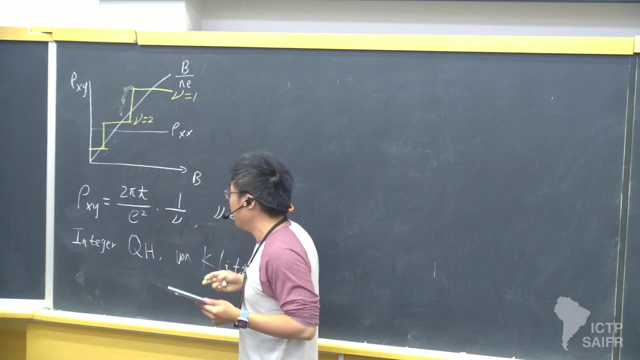 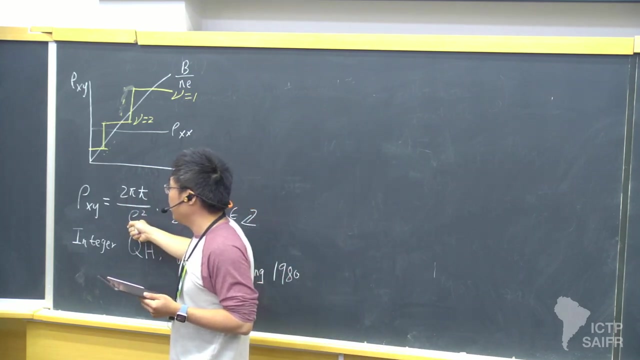 And of course he got a Nobel Prize for this remarkable discovery And this quantity. so you can say that the Hall resistivity at those quantum Hall effect is really, first of all it's independent of the magnetic field and it's a combination. 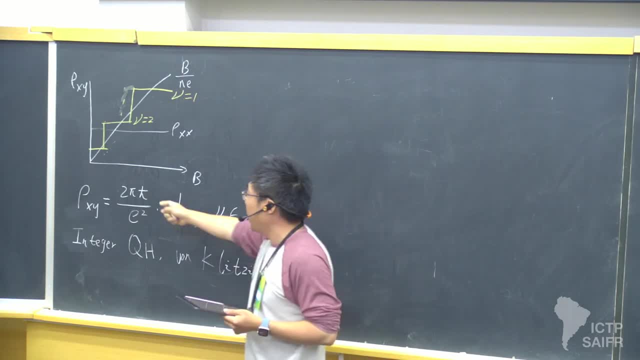 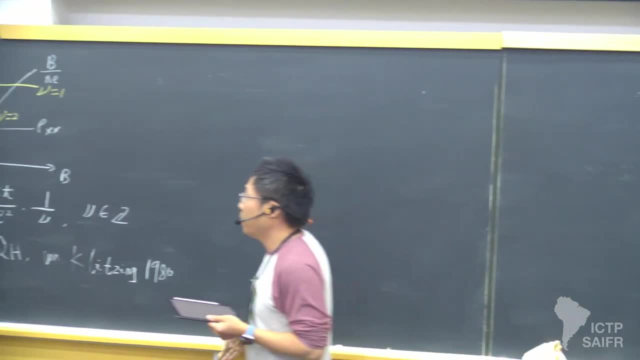 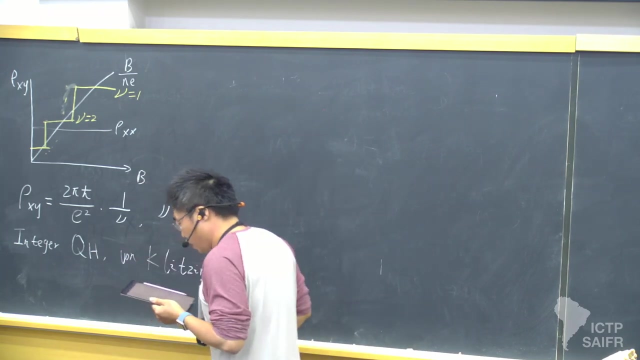 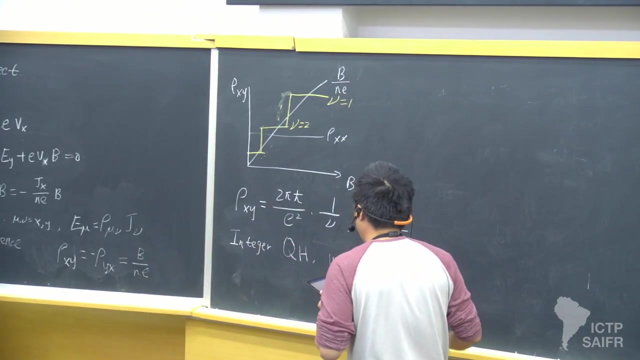 of two physical constants. One is the Planck constant, the other is the electric charge, And indeed experimentally people can achieve really accurate measurement for this Hall resistivity. So I can. for example, this constant is also called the Gleisen constant. 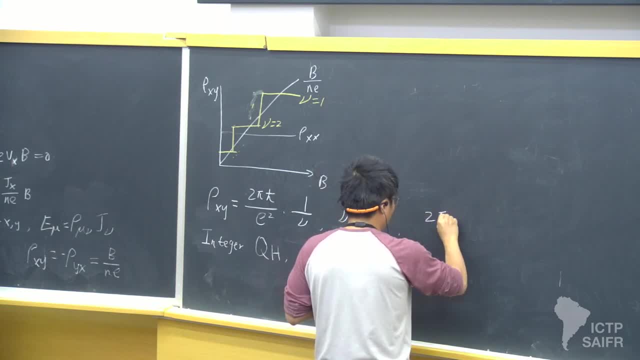 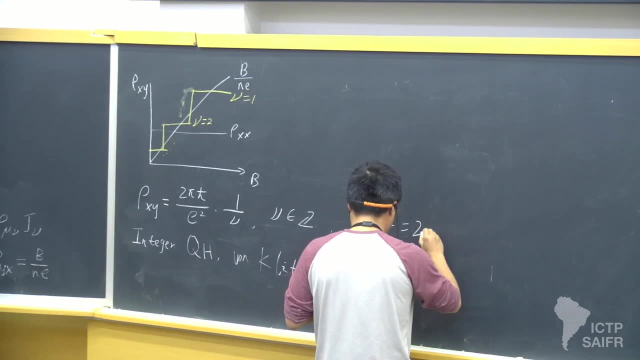 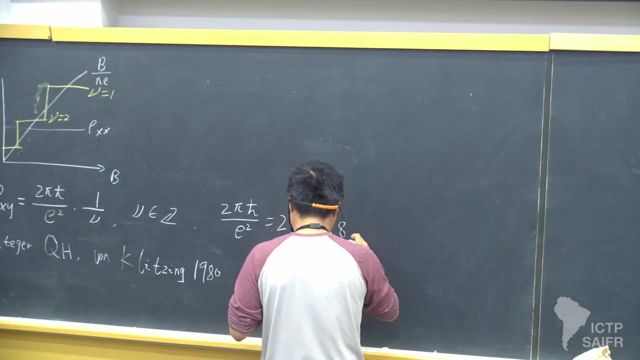 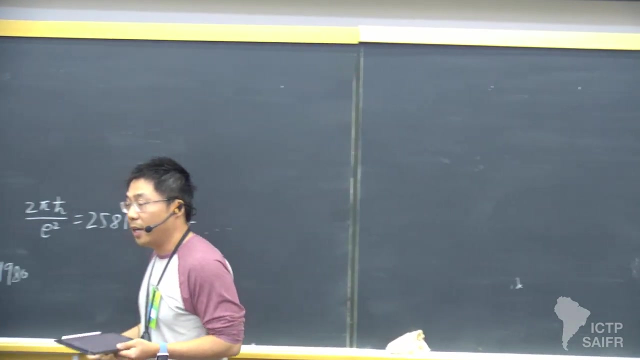 and experimentally people can really measure it to extraordinary accuracy, which I will write it down to showcase that, how accurate people experimentally this number can go to. So you see there are many digits that people can experimentally can measure, just for this phenomenon. 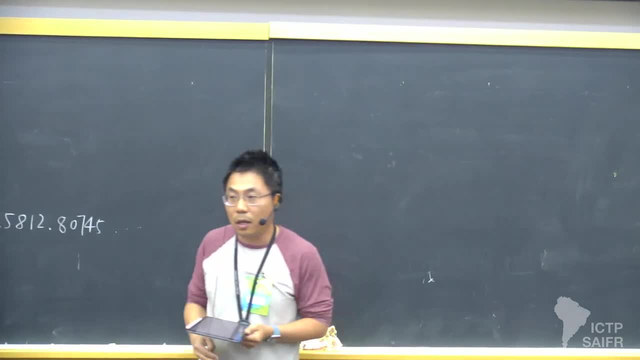 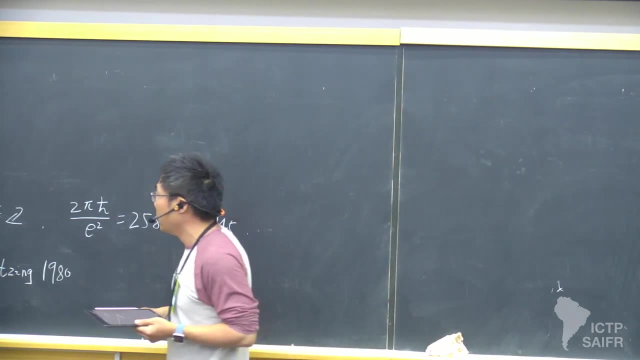 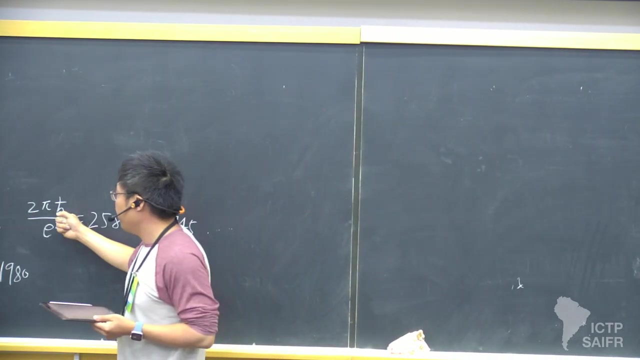 And indeed that's one of the most precise physical quantities that we human beings can measure, And for a while, I think this method was used to determine the values of Planck constant, But I think, if I remember correctly, nowadays there's another way. 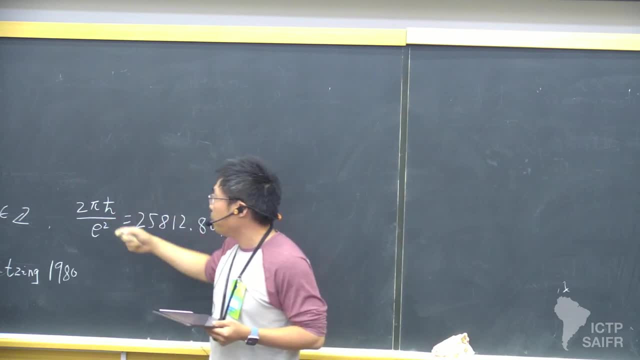 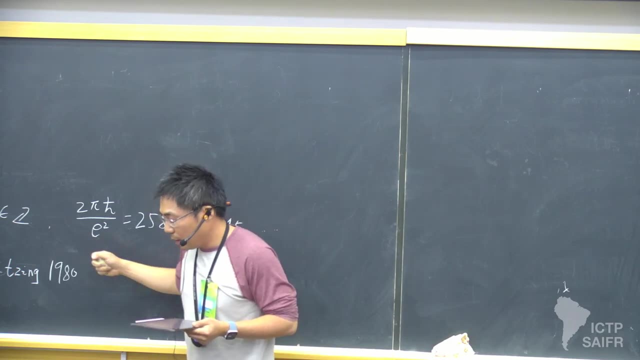 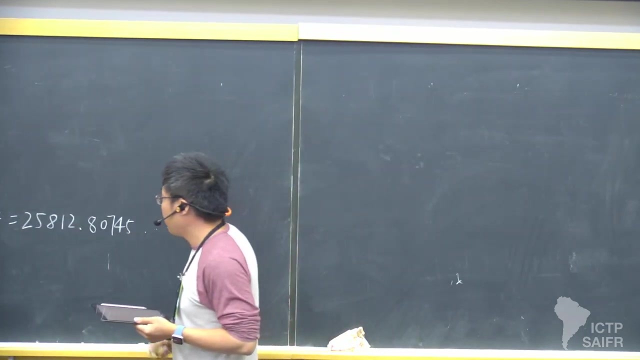 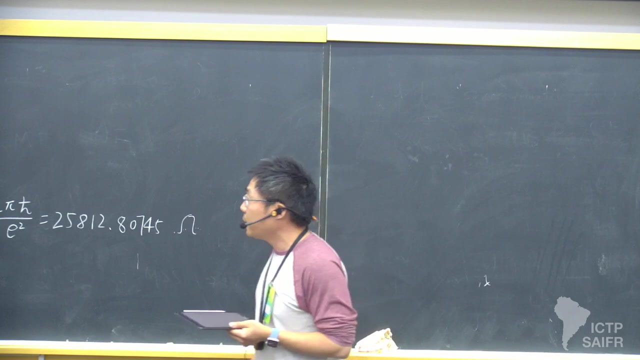 to give you a more precise evaluation of Planck constant. and this Hall resistance becomes the canonical way for people to measure the physical constant, this electric charge. So this is really a remarkable method and this is really a remarkable phenomenon in quantum matter physics. 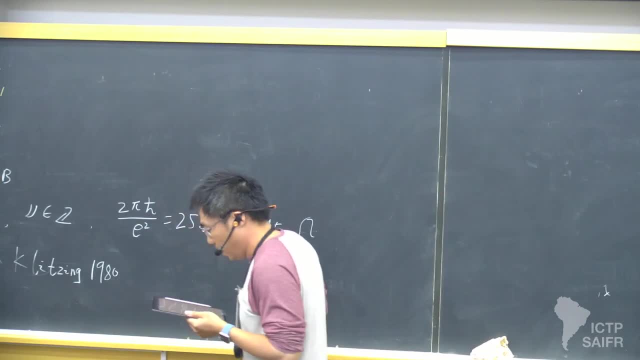 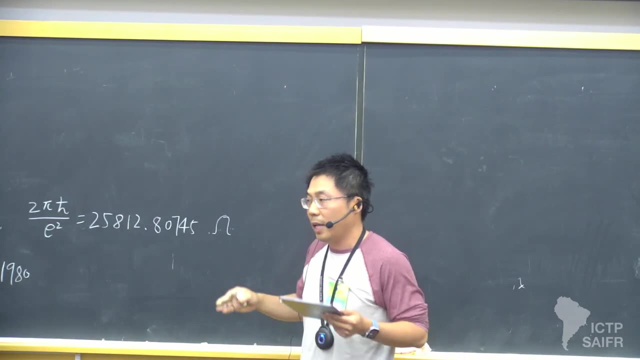 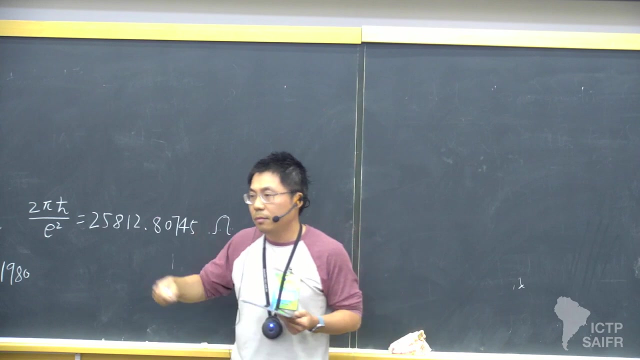 And one important thing is here: this quantum phenomenon happens in the macroscopic level, not in the microscopic level like what we learned in quantum mechanics, that if you consider a single atom you may say the levels of the energies get quantized. But here it's a phenomenon 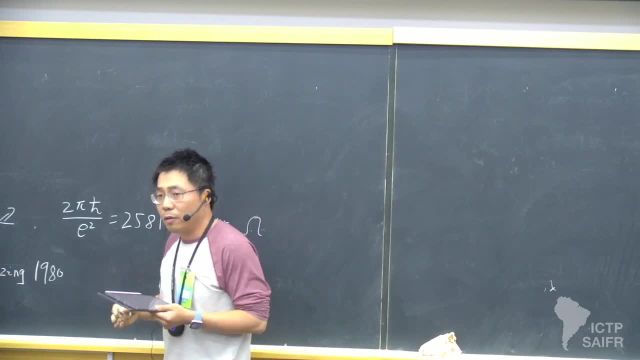 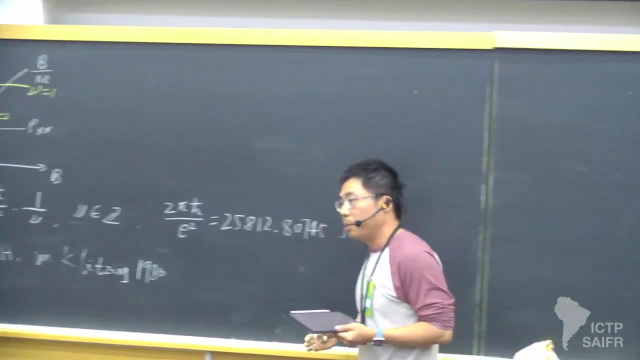 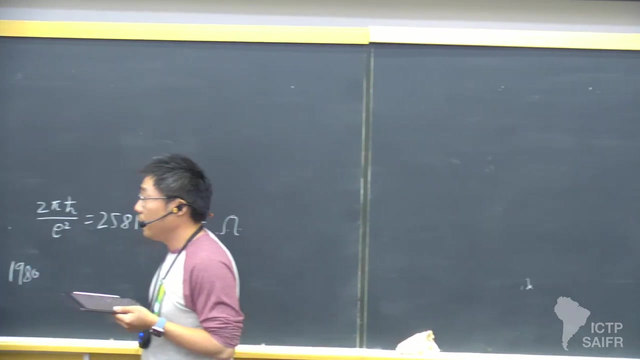 that comes out of many electrons in the system and eventually the quantity you can measure is also a macroscopic quantity. It's this resistance right here. So, Sorry, can I ask a question? Yeah, So to define a rho xy, Yeah, 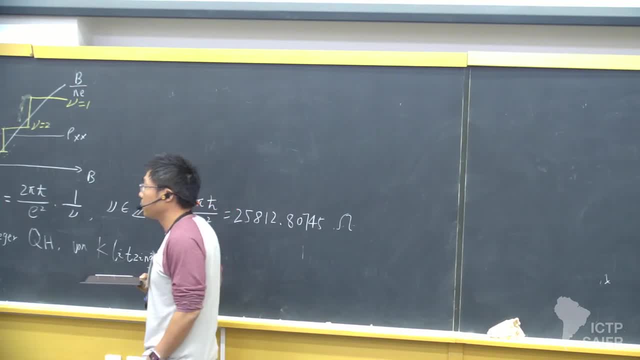 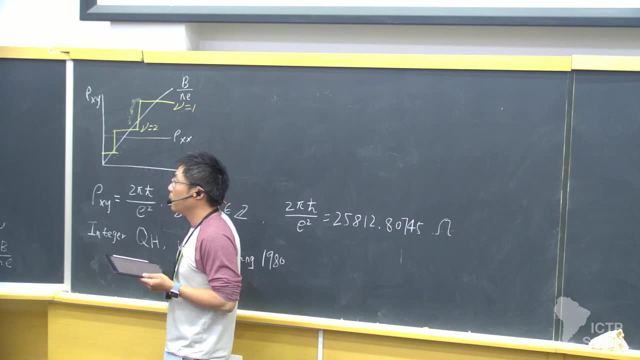 So first you tune the electric field to make sure the current is just in the x direction, right, Yeah, yeah, yeah. And so that gave a precise way of fixing the electric field. and then the current is in the x direction, then you determine rho xy. 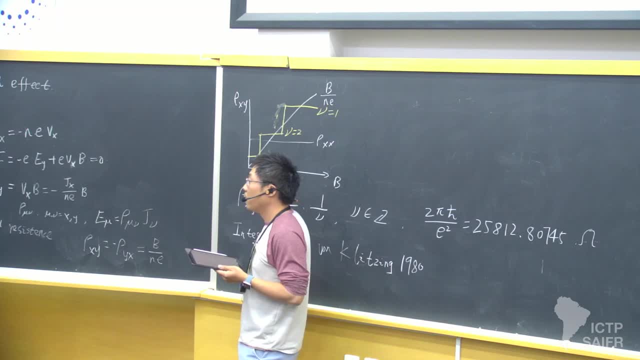 Yeah. From this point of view, I'm not sure I understand what's the definition of rho xx. Rho xx is zero right now, right, Yeah, yeah in this definition. So what's the definition that gives the constant line? 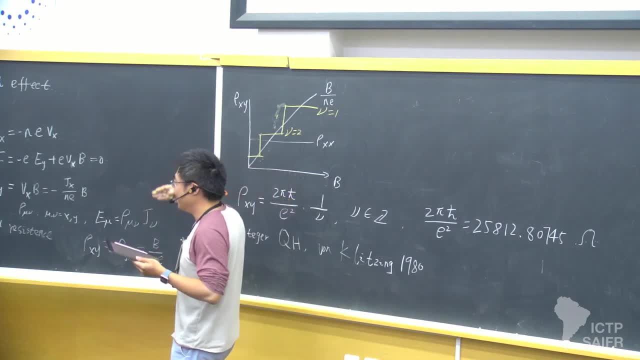 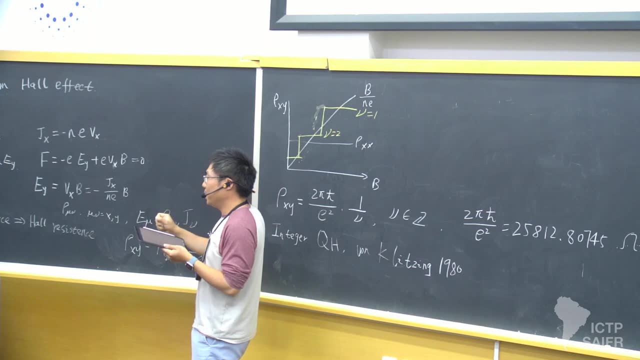 You need to work a little bit harder, like consider the so-called Jude formula and so on, to derive the rho xx. So you know the rho xx comes from the scattering, the scattering of the electrons, with impurities and so on. You need to include that. 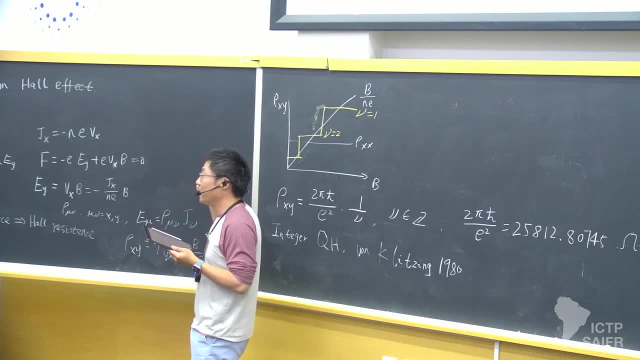 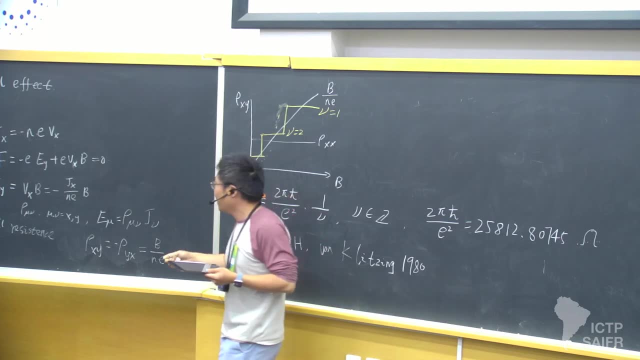 to properly define it. Ah, okay, Yeah, You can. So yeah for use. If you're interested in how to get to the entire things, like rho xx, you can check the Dev Tone's lecture notes In his lecture notes. 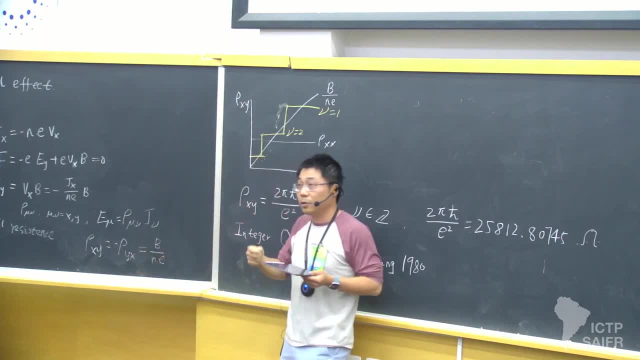 he has explained the full story in the classical world. So right now, naively, there was no rho xx. No, So you can check the whole story in the classical world. Yeah, So you can check the whole story in the classical world. 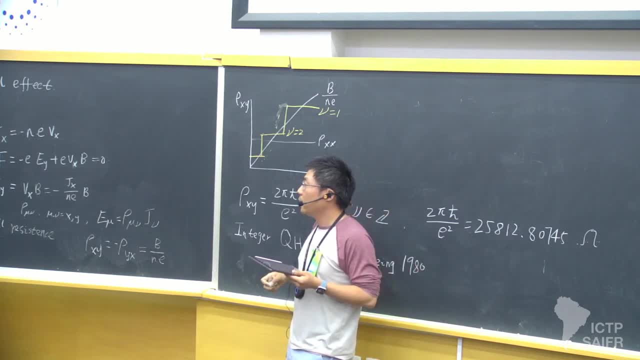 Yeah, So right now, naively, there's no rho xx. right, Right, right, Because you explained that there's only e, y and b. Yeah, yeah, yeah, But you are saying there exists electric field in the x direction. 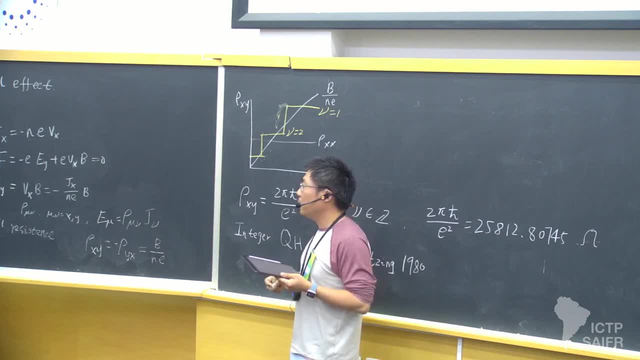 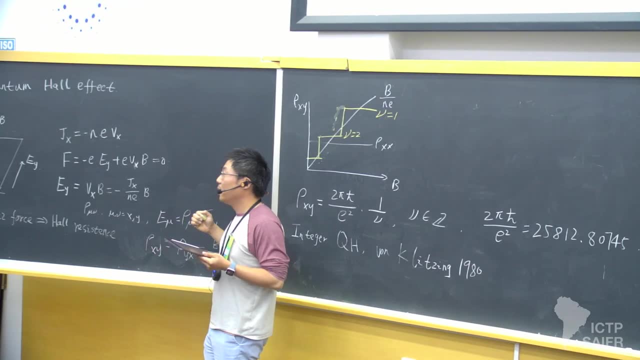 if we are more careful, but it's small Or it doesn't exist and you need a slightly different definition. You need- Yeah, you need a different mechanism to get rho xx right. Yeah, I think there's a question. Yeah. 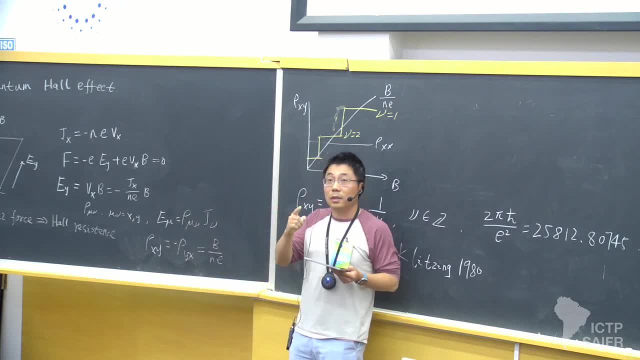 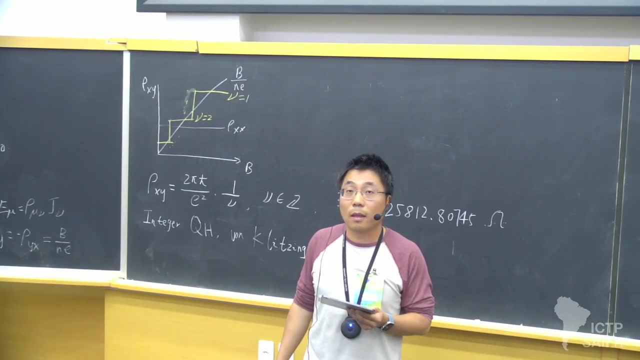 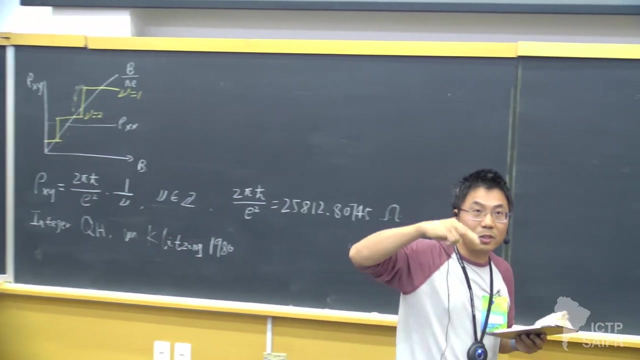 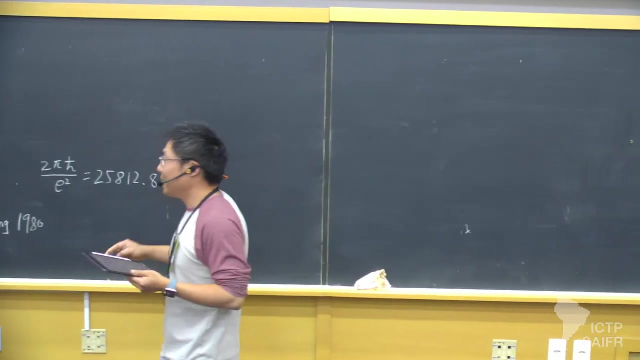 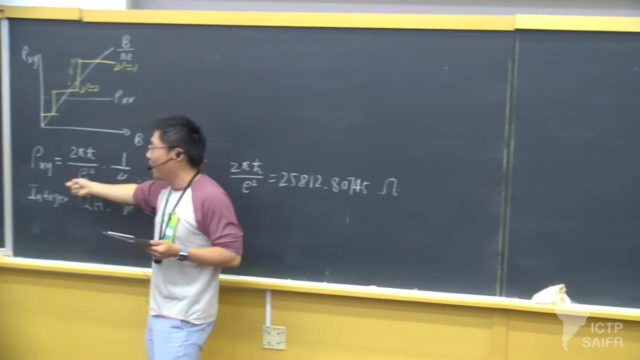 So maybe there's, and why do we get this remarkable quantization of the whole resistance independent of magnetic field? 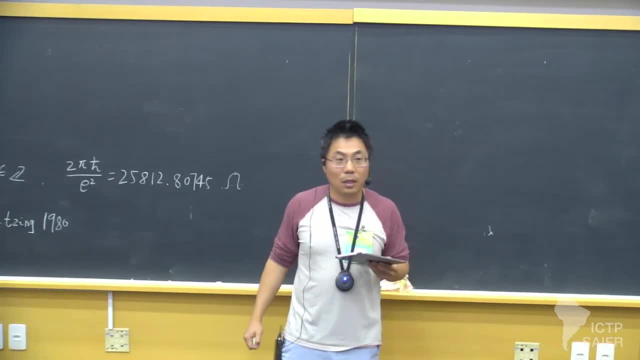 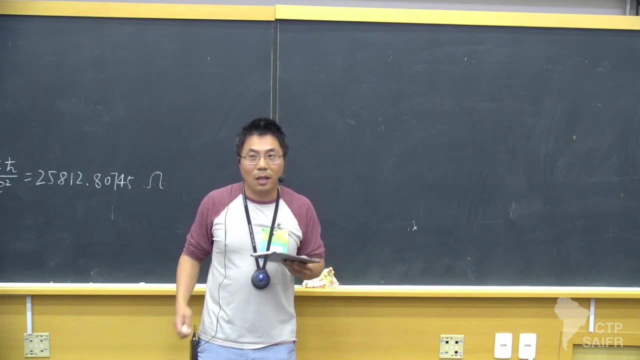 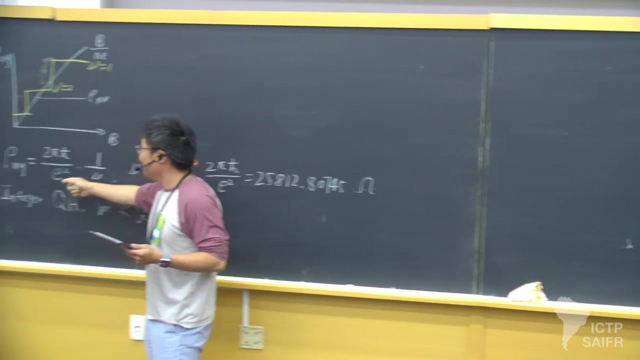 Yeah, But shouldn't you approach the line when, like, you take the limit as h-bar is zero, Because, like, But h-bar is not No? repeat the question. Yeah, the question is If I, Yeah, yeah, yeah. 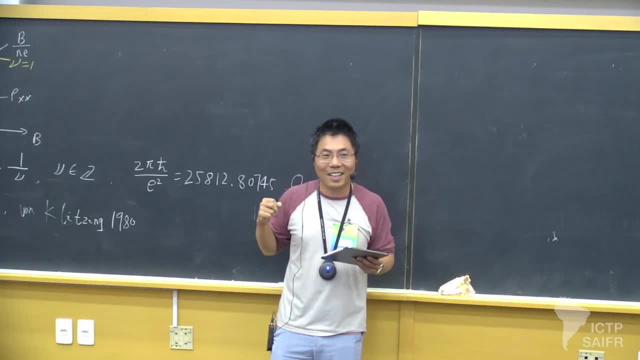 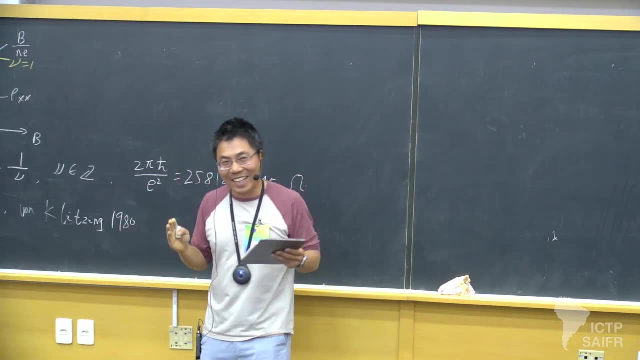 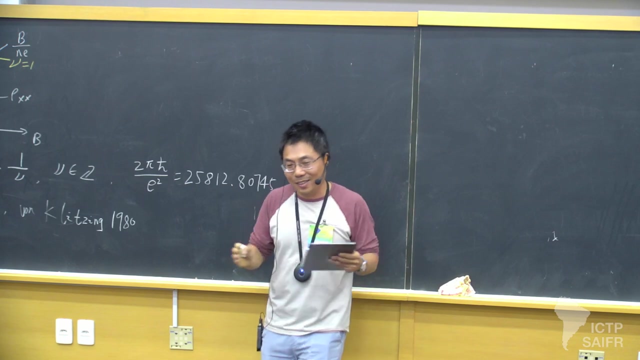 You should get the classical limit if you set h-bar to zero. Well, that's probably the remarkable point of this right. So that's probably the remarkable point of this right. So it's just a quantum phenomenon that happens macroscopically. 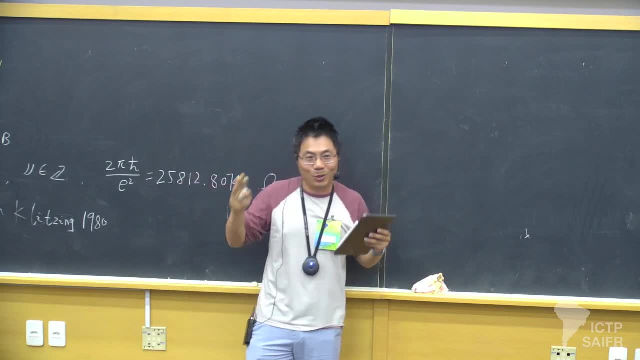 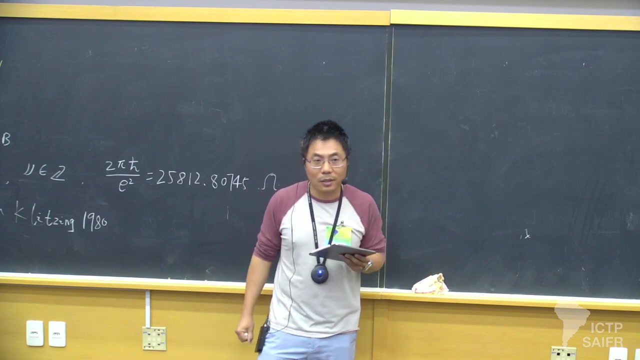 You cannot really take h-bar goes to zero to recover the classical physics. Ah, okay, so it's a separate phenomenon, not, You can't derive the classical whole effect from this one. Right right, right, right, Yeah, it's different. Yeah, yeah, yeah. 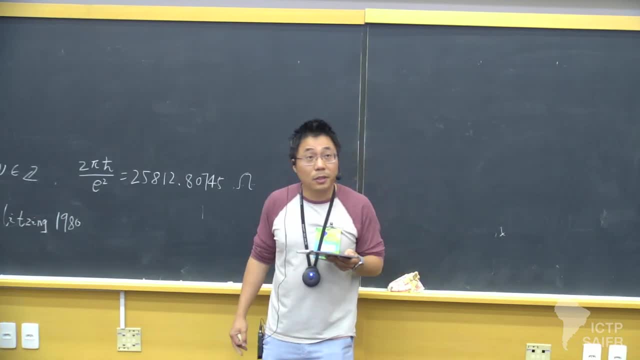 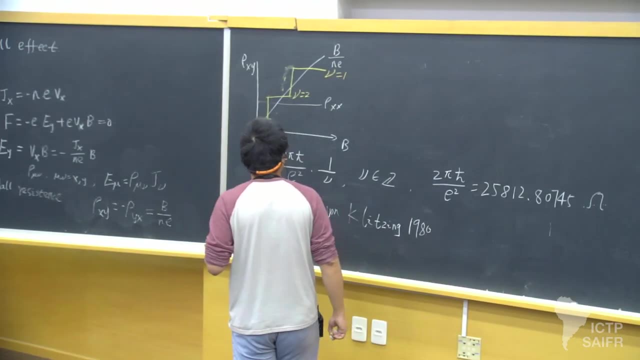 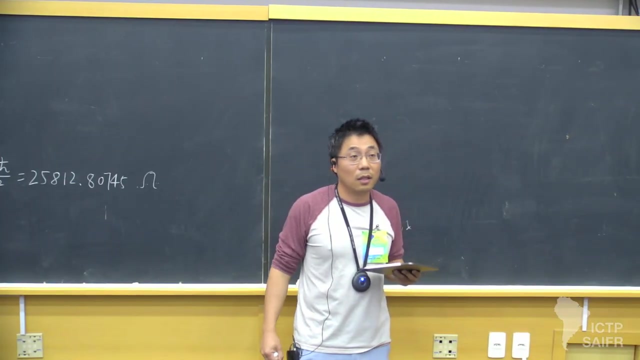 Yeah, So any other questions? Yeah. so the other thing I would like to mention is for those: There's one more question there. Okay, yeah, I was trying to do a question, Is that? Yeah, yeah, yeah. 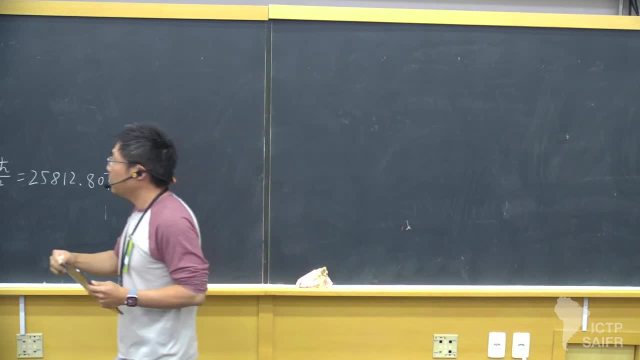 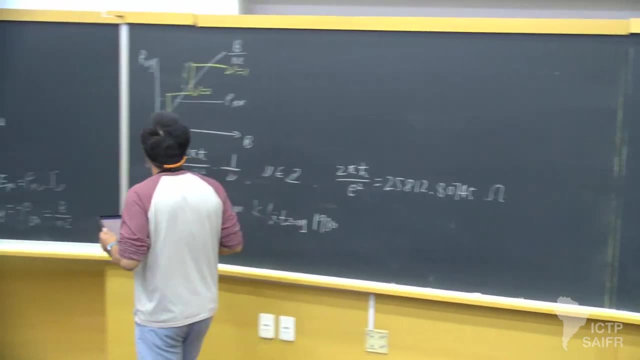 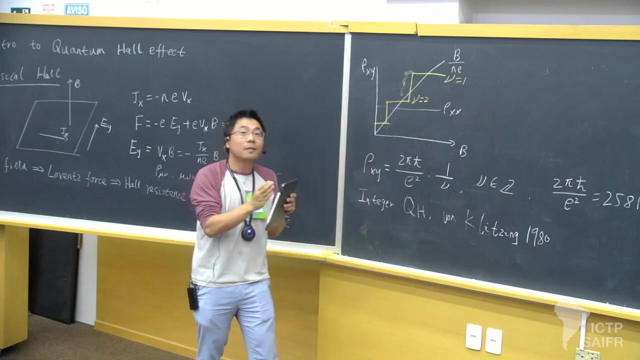 Can you repeat the question? So the question is: what happens if I increase the temperature? right, What will happen? So if I increase the temperature, what will happen is that you will see this, Let's say: this plateaus becomes narrower and narrower and eventually it will just recover this classical region. 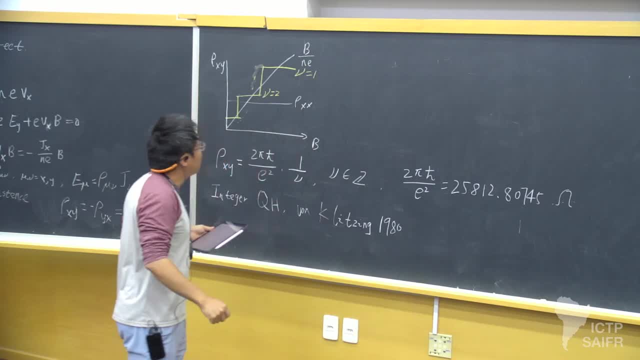 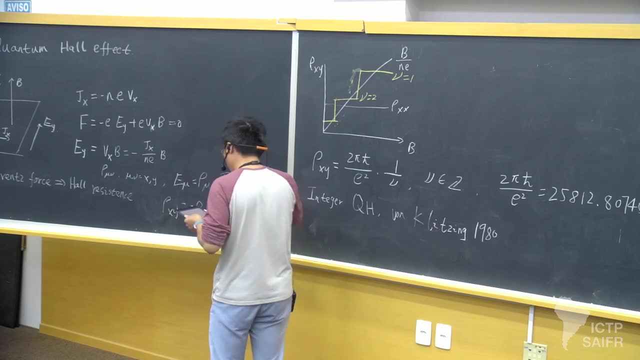 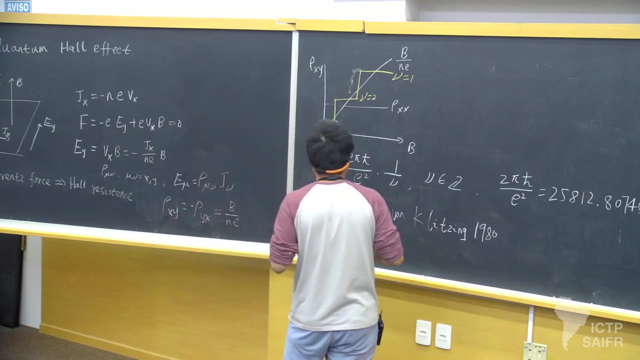 Yeah, Yeah. So the other thing I would like to mention is this: rho xx. So, on the classical side, what I said, What I tried to say, is that if you do the work more carefully, you will find rho xx to be the constant in the classical world. 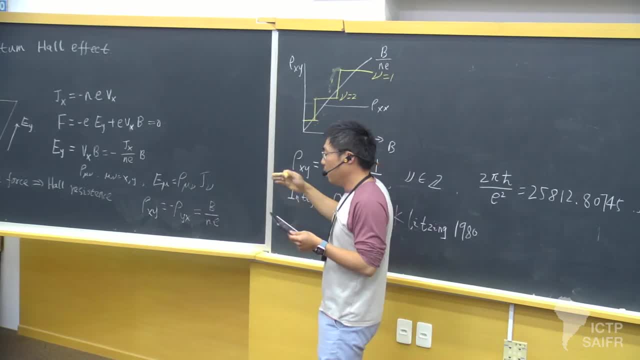 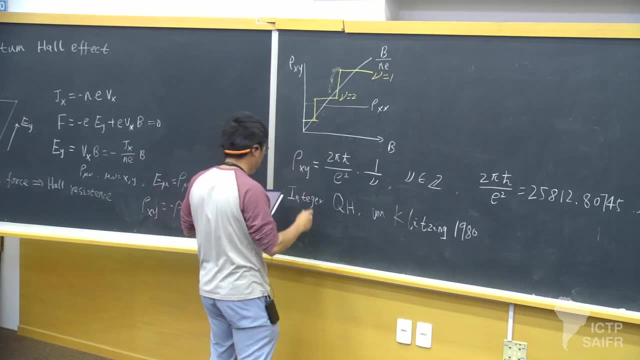 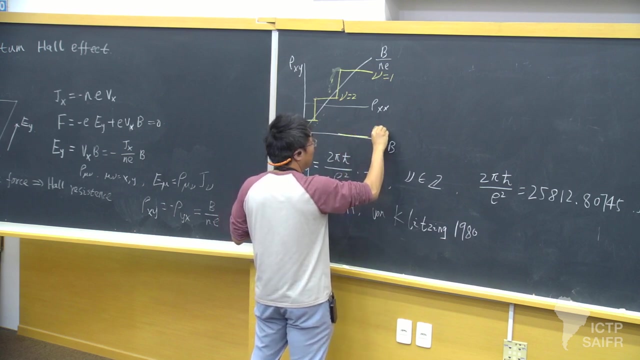 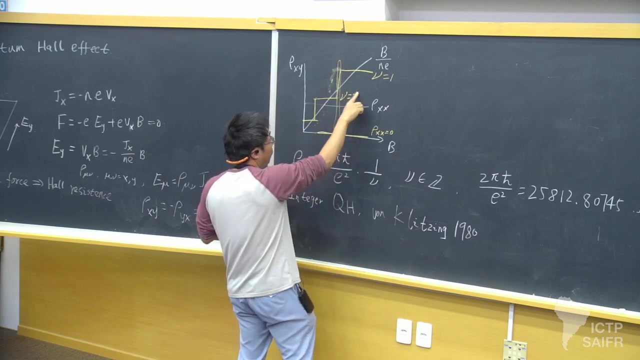 depends on the scatterings of the electrons and so on. That's some intrinsic property of your material. But for quantum Hall effect what you will find is that those rho xx stays exactly zero at those plateaus And it will only jump as you change from one plateau to the other plateau. 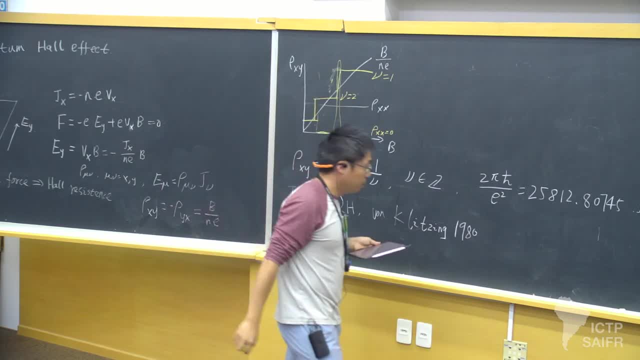 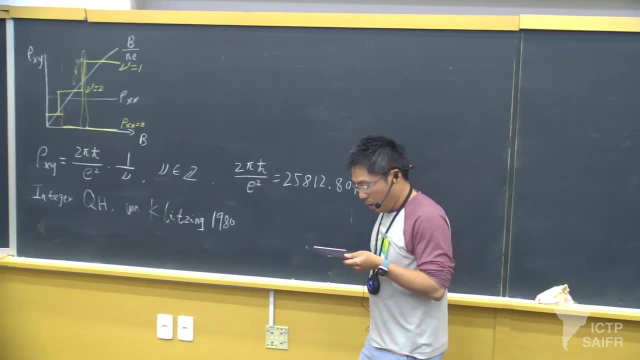 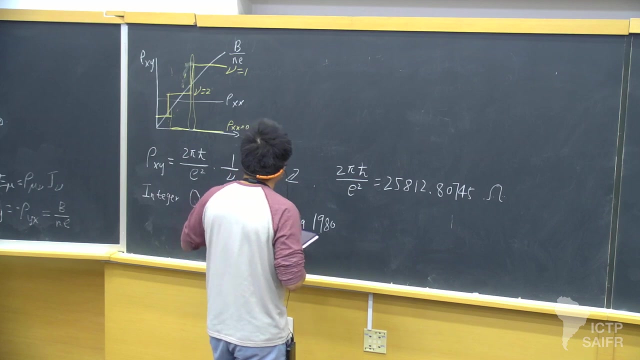 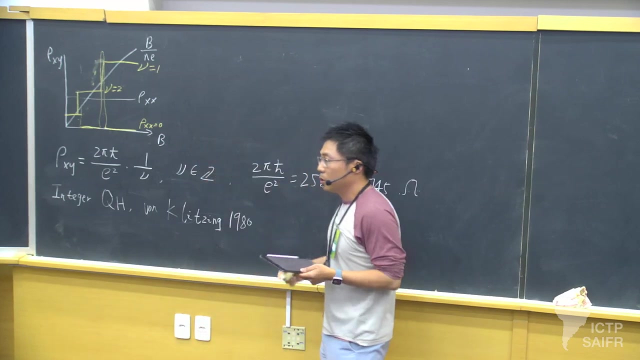 So that is also observed experimentally. Okay, So that is another property of those quantum Hall effect. Okay, So And so, as I said, this course will- I will try to explain how to understand this- those quantization of the quantum Hall, of this Hall resistance. 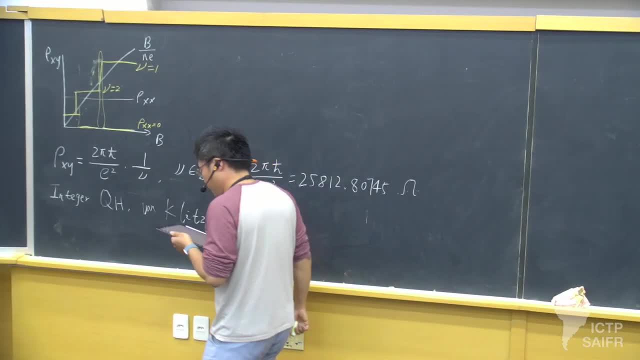 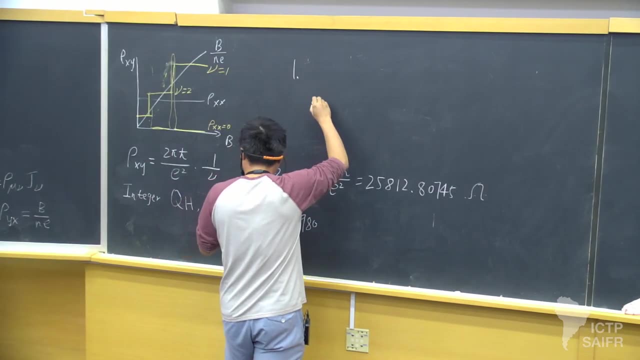 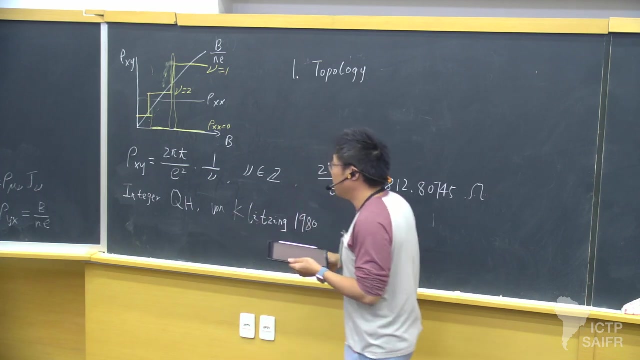 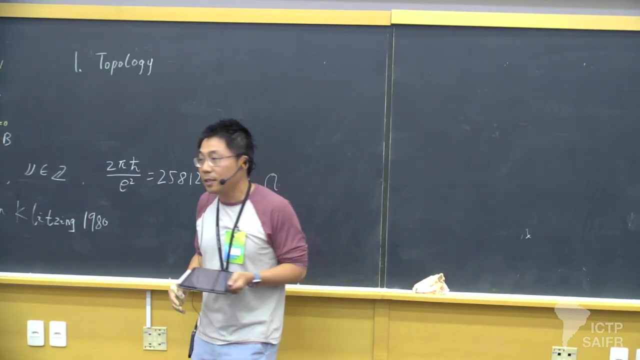 And, And, And. it could indeed be summarized as two words. One is the so-called topology, That is, turns out that this quantization, this integer number nu, is related to some pretty deep mathematics. that is called Chern number, Chern number or Chern class of in algebraic topology. 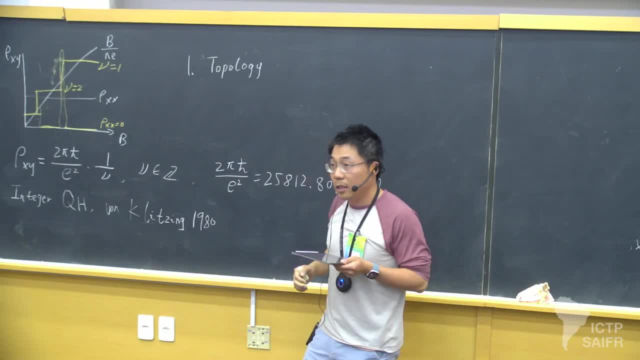 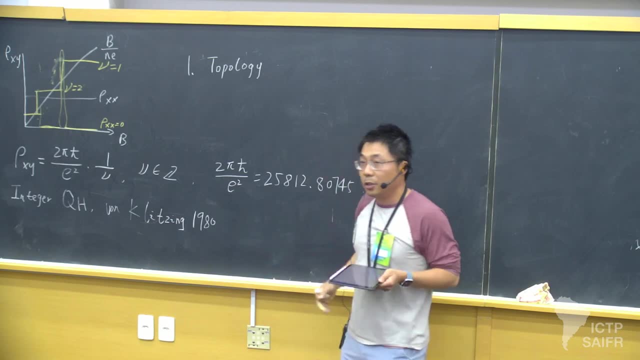 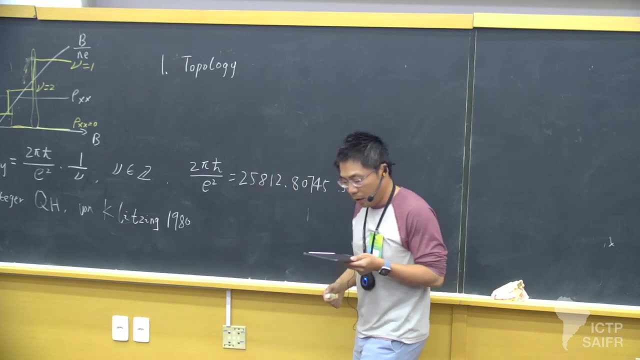 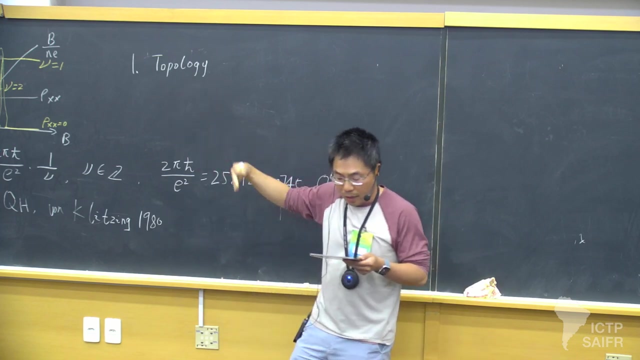 Chern number or Chern class of in algebraic topology, Which I will explain in the later part of the lectures, And, And this, The idea of topology, actually becomes a very, very important and popular topic in nowadays study of quantum matter. So, and this and this really was studied by in this quantum Hall effect. 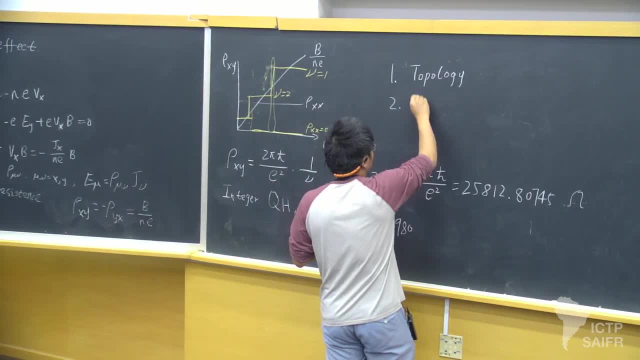 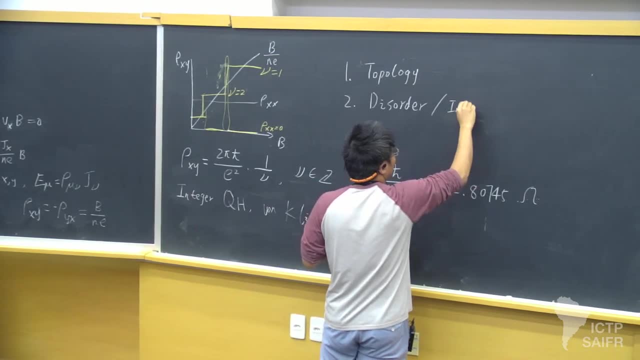 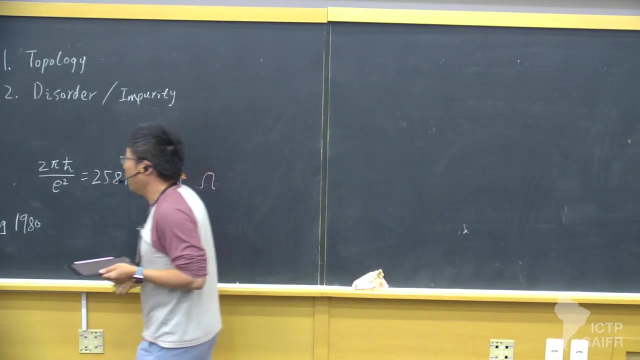 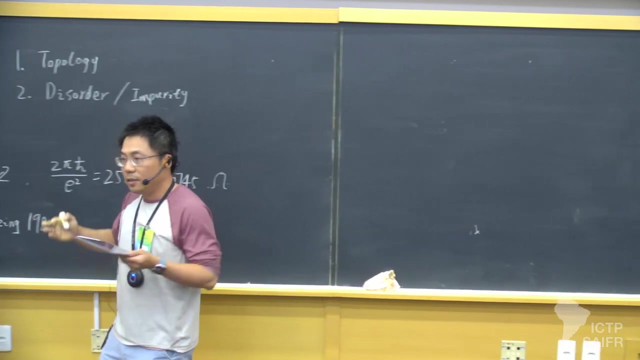 And Another thing that is A little bit more surprising is that the disorder, or you can say the impurity or the dirtiness of the materials plays a key role for this quantum Hall plateaus. That's really very counterintuitive compared to the things that we learned or we start or we deal with in physics, particularly theoretical physics. 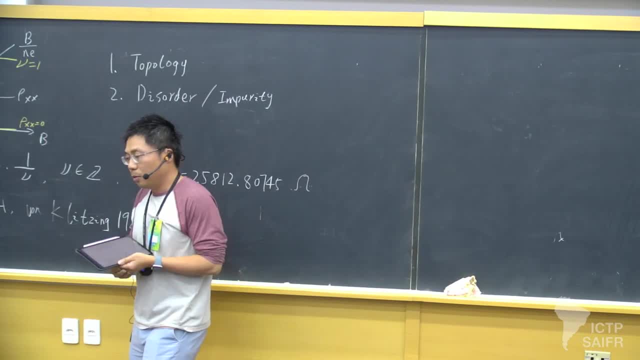 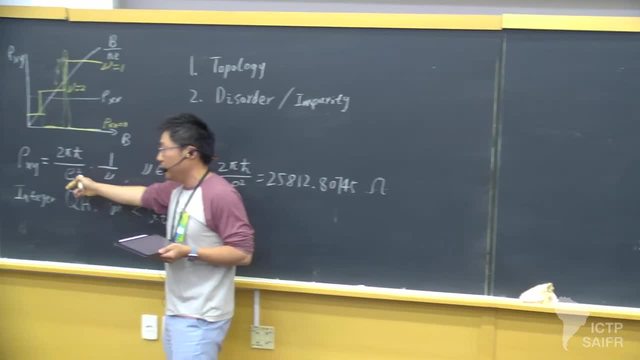 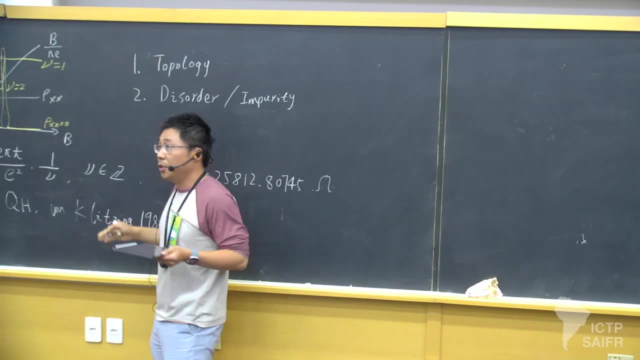 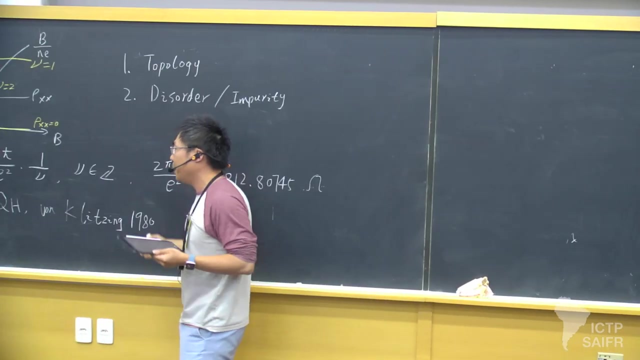 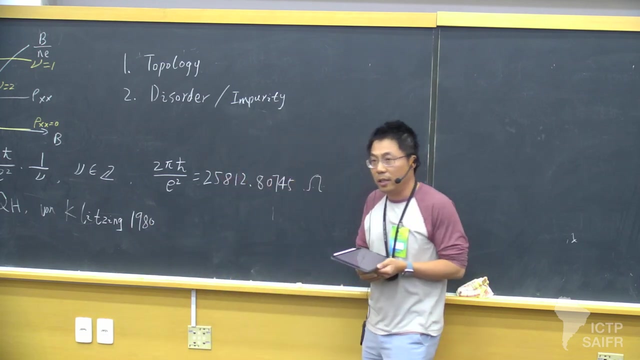 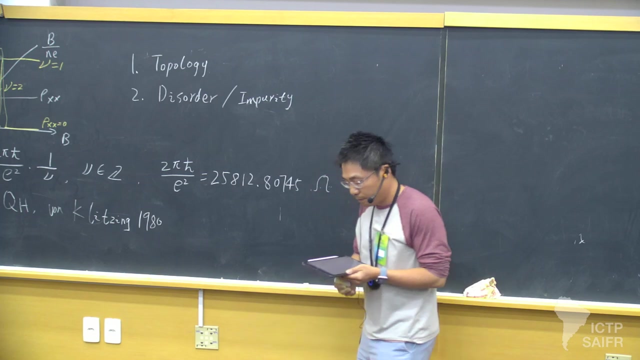 the factor that give rise to the plateaus of this whole resistance. And without disorder, without impurity, you don't see plateau at all. That's really, yeah, that's really very surprising and also a nice illustration that sometimes the dirtiness in nature can give rise to a very beautiful consequence in physics. 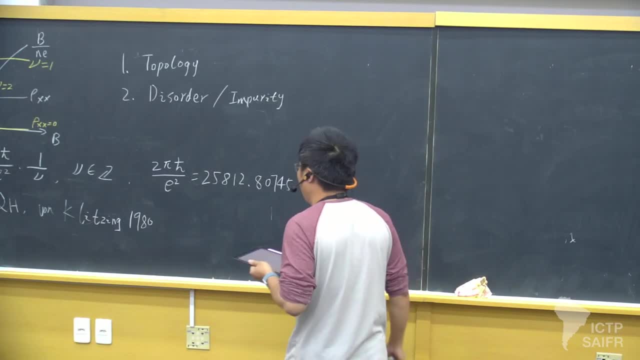 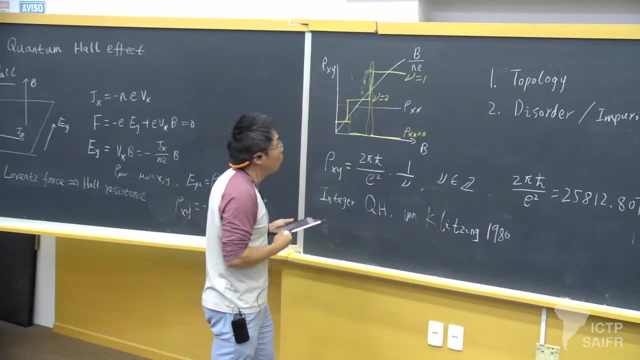 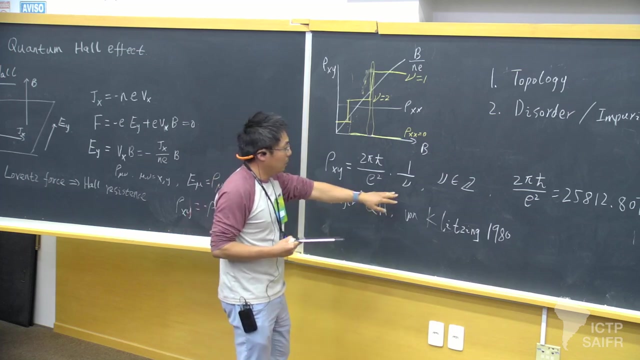 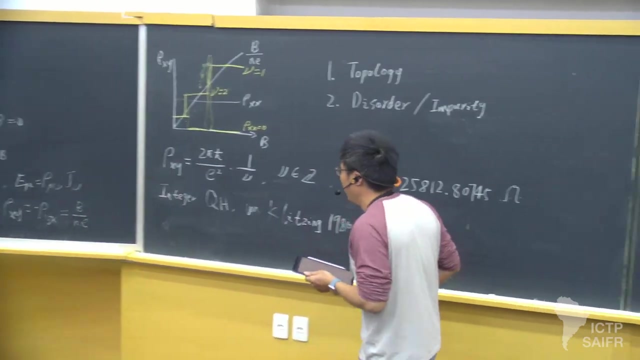 Okay so, and another thing that I would like to mention is that so you can ask what will happen if I go to a larger magnetic field, right, and then I won't have integer quantum holes, Right? But and it turns out that if you go to a larger magnetic field and and also make the 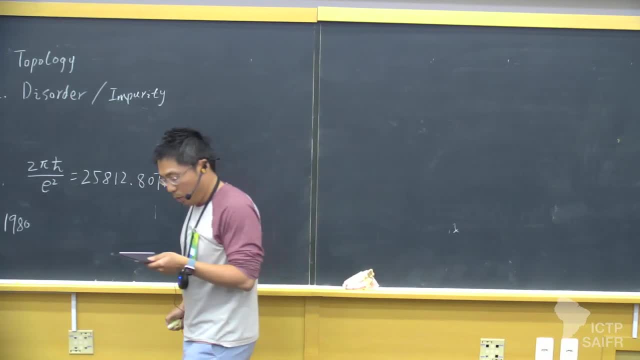 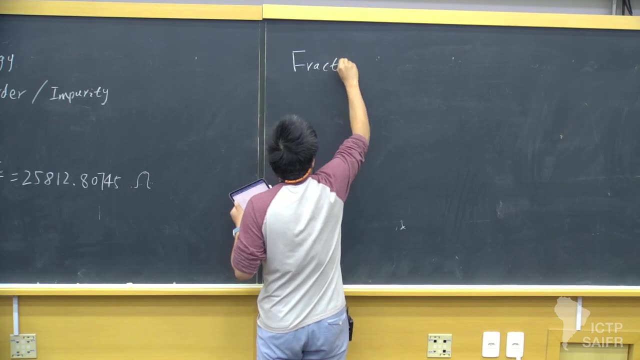 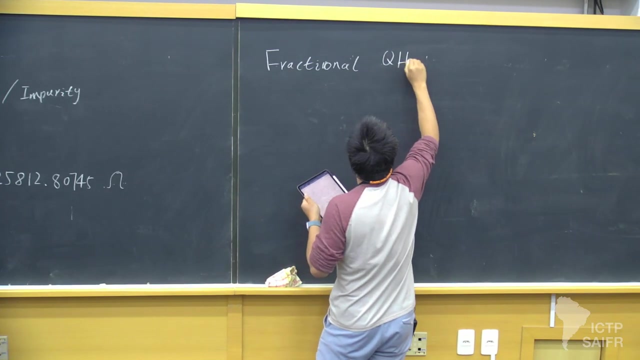 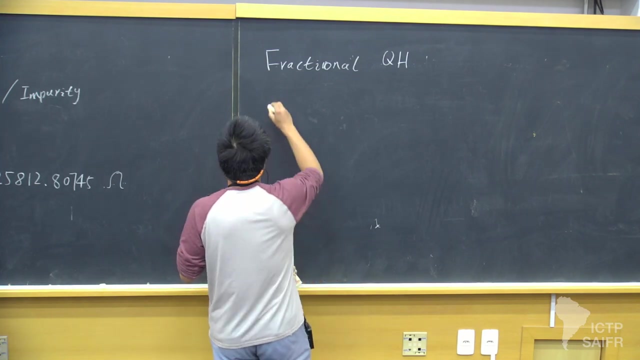 and meanwhile make the sample a little bit cleaner. what you will find is that the so-called fractional quantum holes effect that my. I still get those quantized plateaus, but now those filling factors becomes fractions. For example, I can get one-third state. 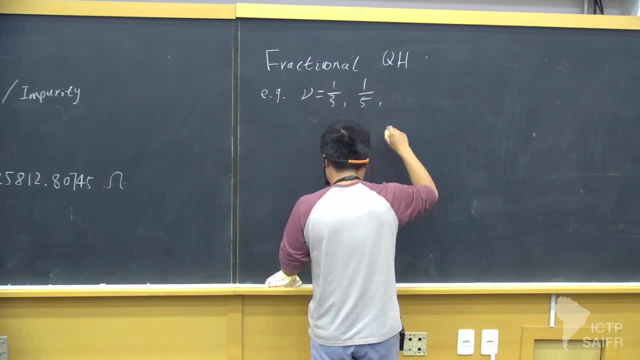 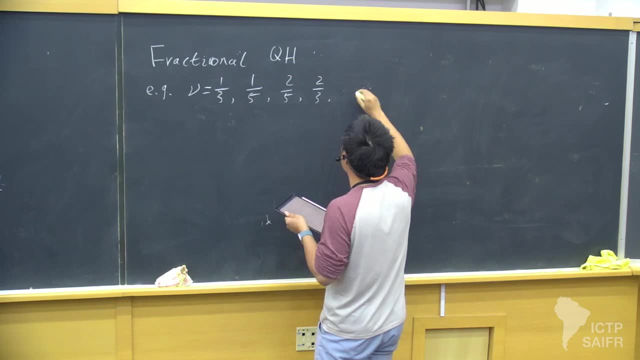 I can get the so-called one-fifth state like two-thirds, two-fifths, two-thirds and so on. Right, You can also get some filling factors, that is larger than one and so on. You get a bunch of fractions. 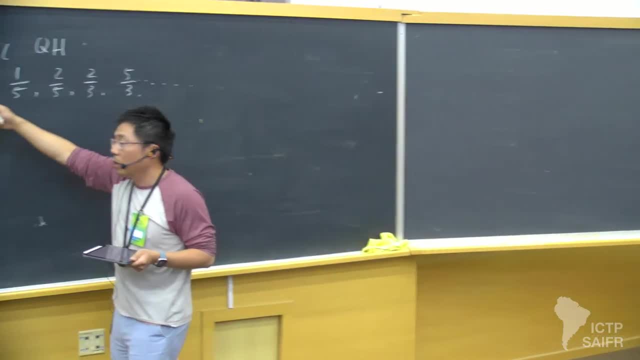 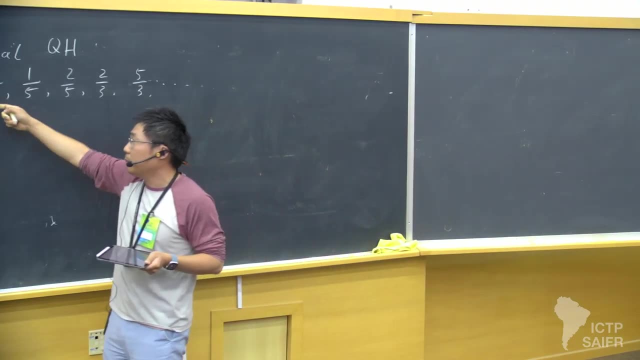 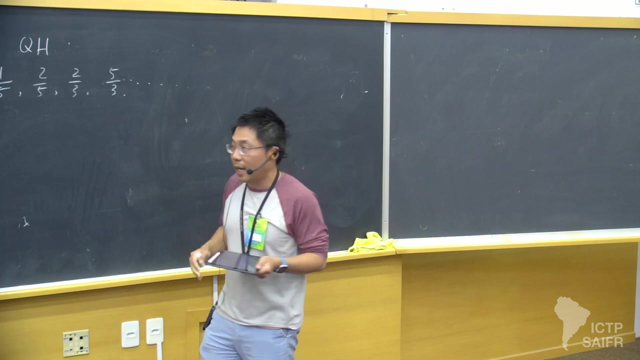 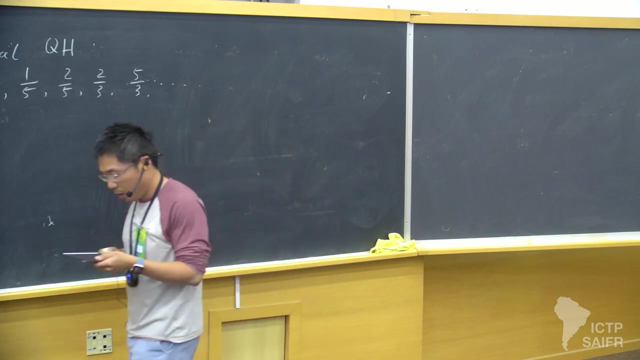 And most of those fractions Actually has all the denominator And there are only a few have even denominators. And the fact that most of those fractions have all denominator is related to the fact that the underlying system is a fermatic system. It's a consequence of the fermatic statistics of my particles. 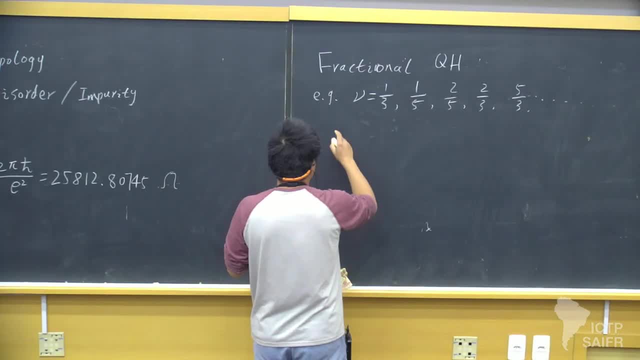 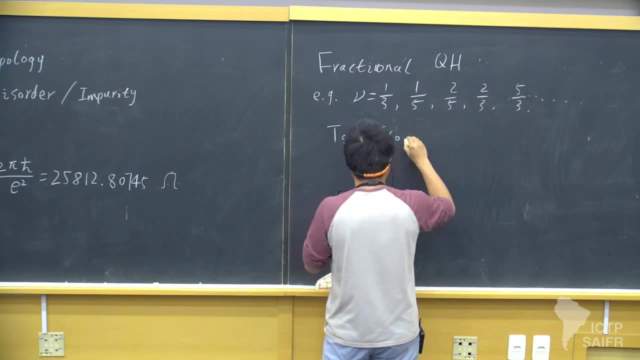 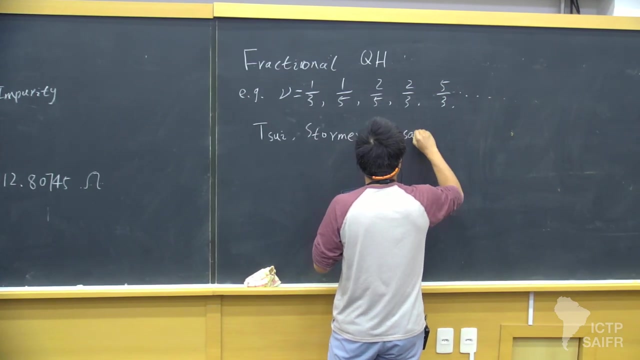 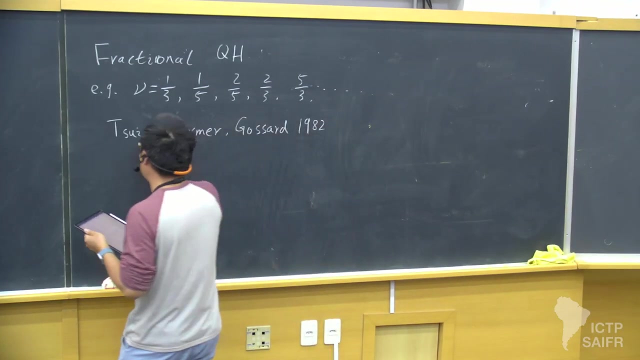 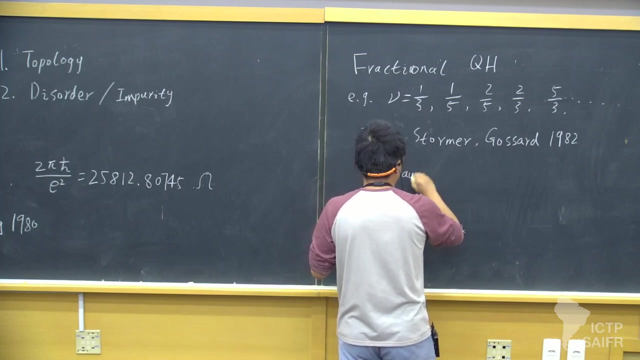 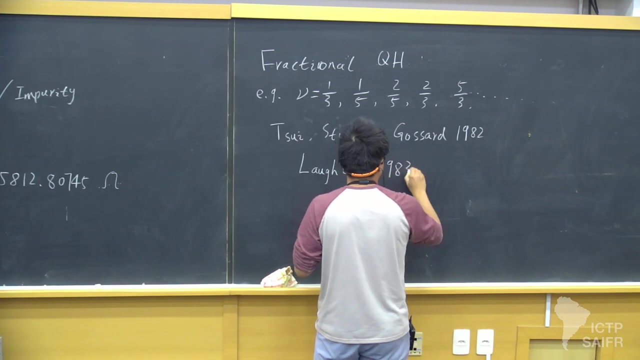 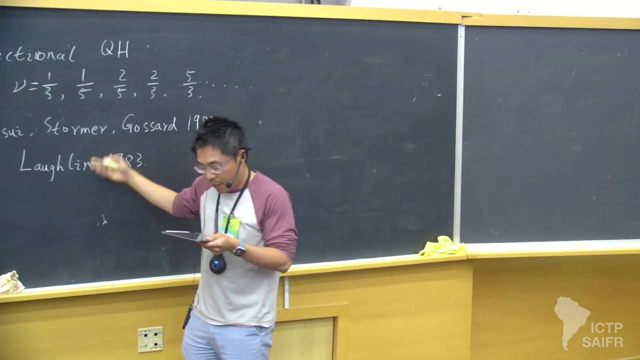 Okay, And this fractional quantum hole effect was originally discovered By those three gentlemen, Trey, Stormer and Gossard, in 1982.. And after this remarkable experimental discovery and Laughlin came up with a very beautiful way to understand, to explain those experiments one year later, and no doubt that those guys 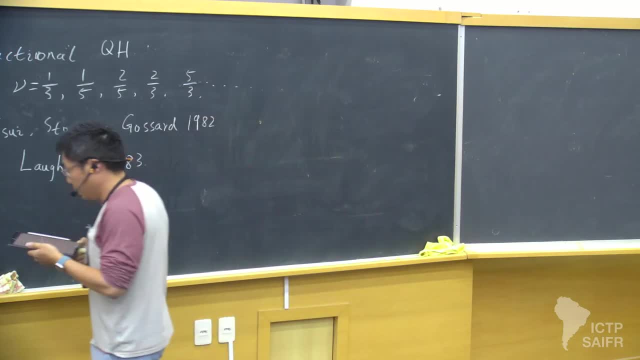 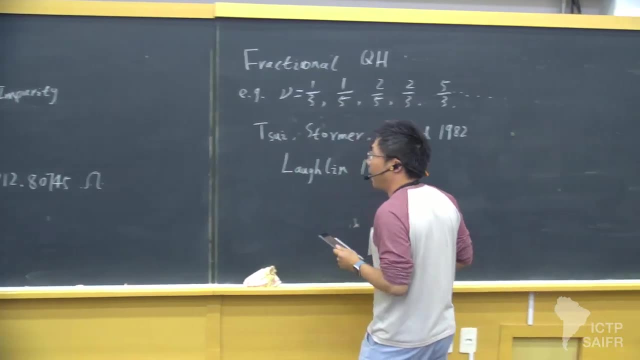 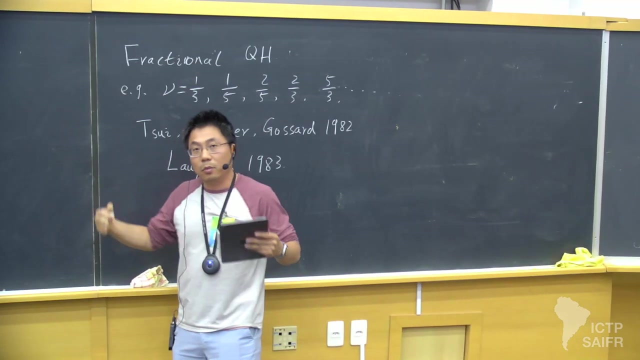 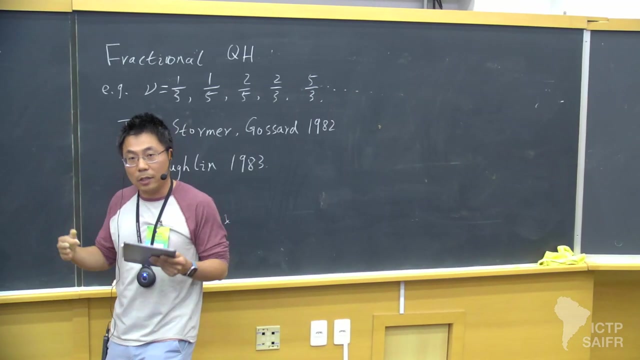 also got a Nobel Prize at some point. And the remarkable, a new physics of this fractional quantum hole effect compared to integer quantum hole effect, is that in those fractional quantum hole effect, the system, the excitations, The excitations that you can have in the system, turns out to carry a fractional charge, not 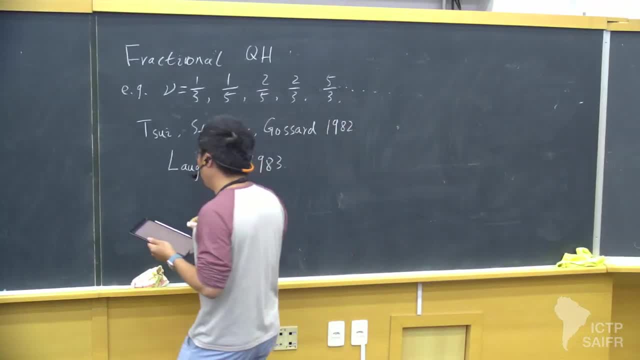 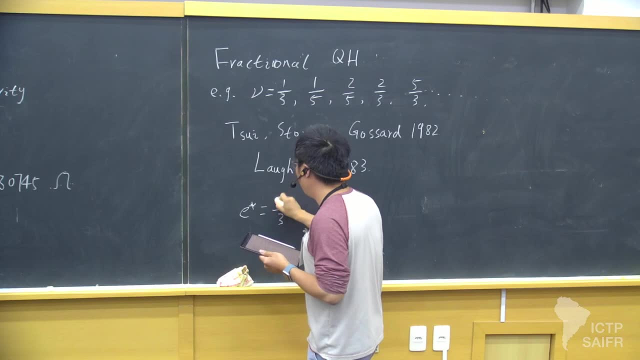 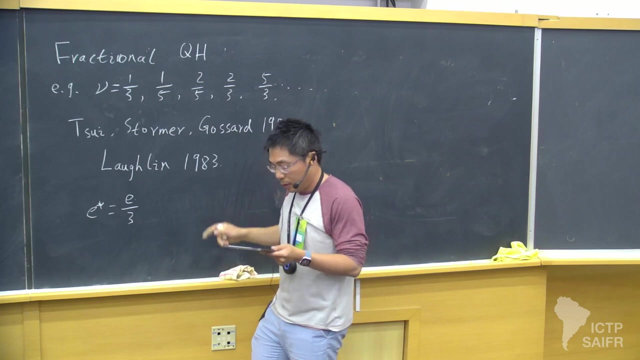 integer charge And for this one-third state, the elementary, the excitations that you can have in the system- turns out to be one-third of the actual charge And, even more remarkable, those excitations have the so-called fractional statistics right. 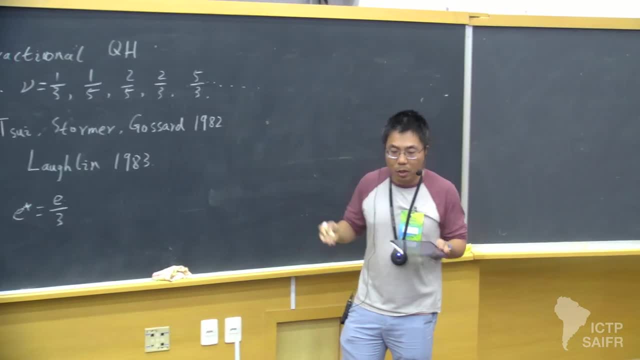 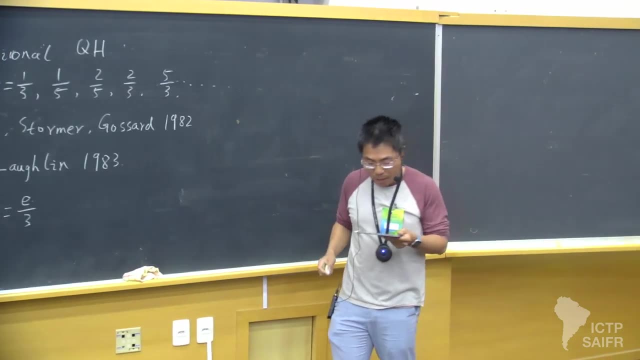 In the morning, Nathan. Okay, So we have reviewed the boson and fermions right And in the fractional quantum hole state, those excitations are neither boson nor fermion And this is what we usually call nowadays called anion. 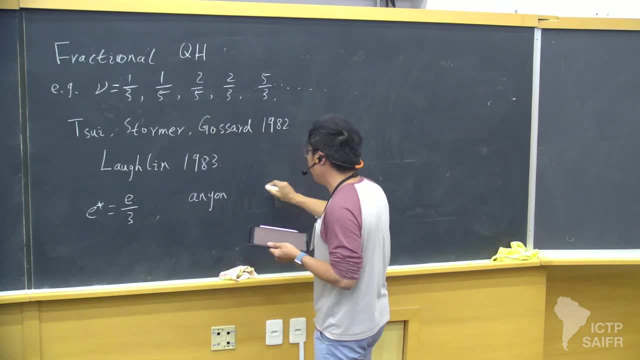 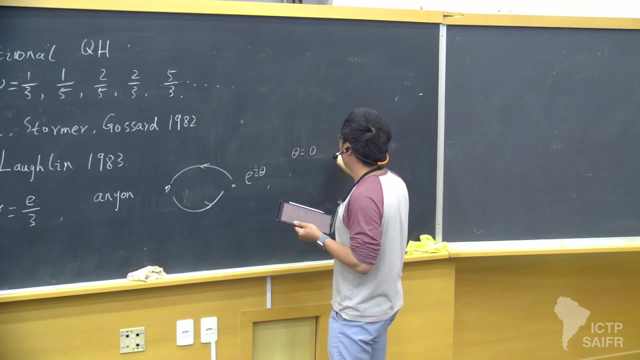 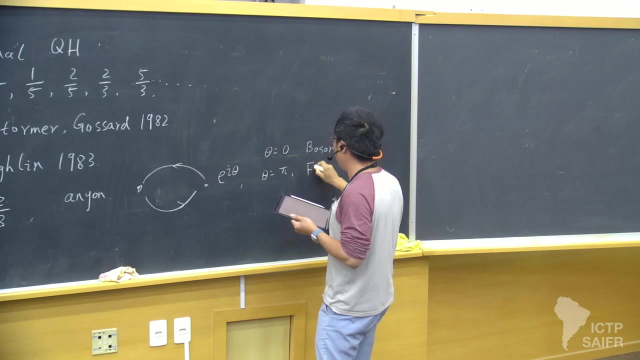 Namely that if you consider two of such excitations and you just exchange them right, You will get a non-trivial phase factor that say EI theta. If theta equals to zero, we know that's a boson right. If theta equals to pi, we know that's a fermion. 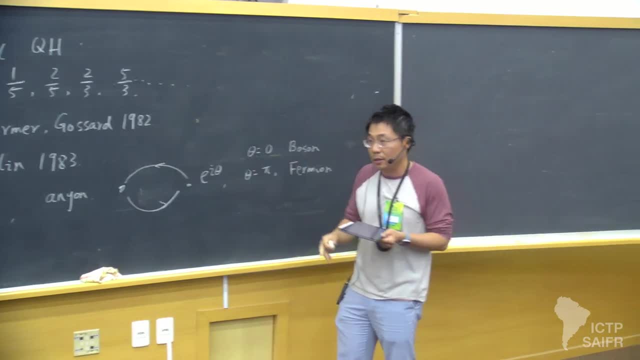 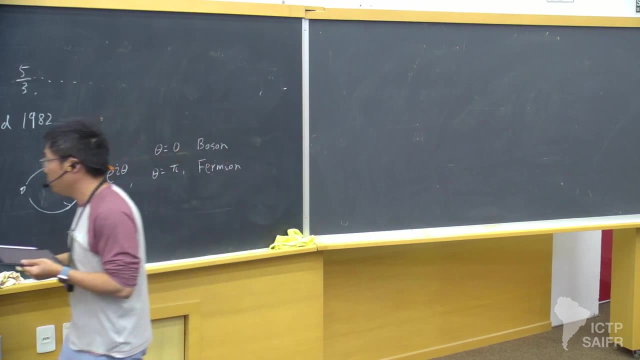 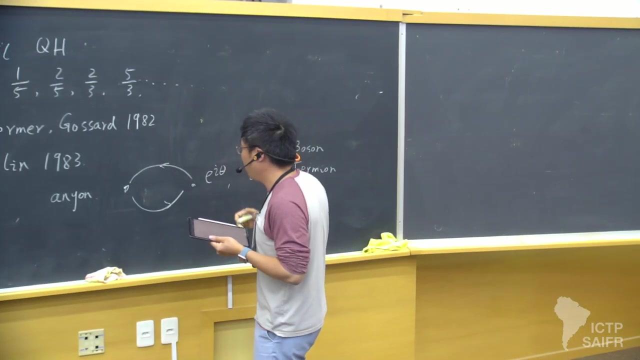 And for anions it turns out that theta is neither zero or pi is some fractional numbers. And for the one-third Laughlin state I should specifically say that this is one-third Laughlin state And for this one-third fractional quantum state, this theta goes to 2 pi over 3, right. 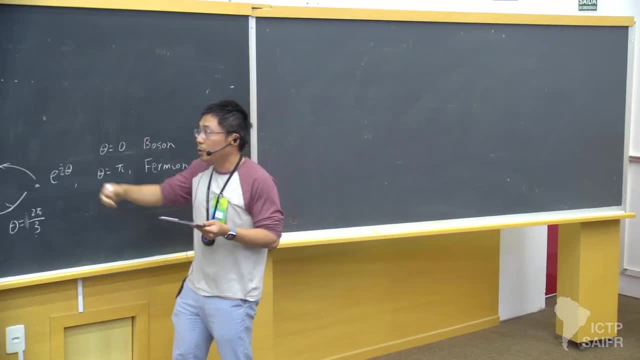 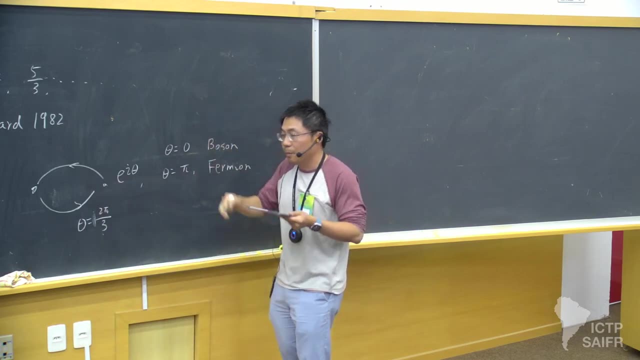 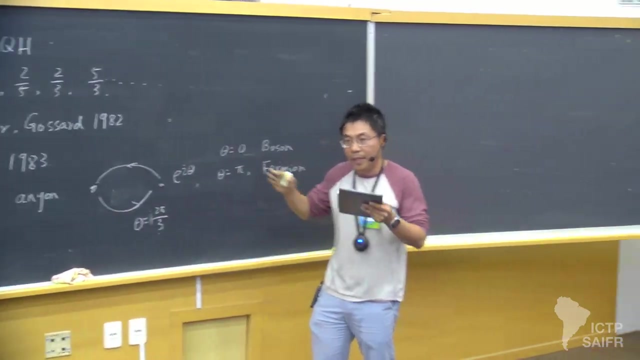 And this is a so-called fractional statistics, And for each different fractional quantum state you will end up with different statistical angles, And sometimes things can even become more exotic, like you can get those so-called non-trivial anions and so on, right. 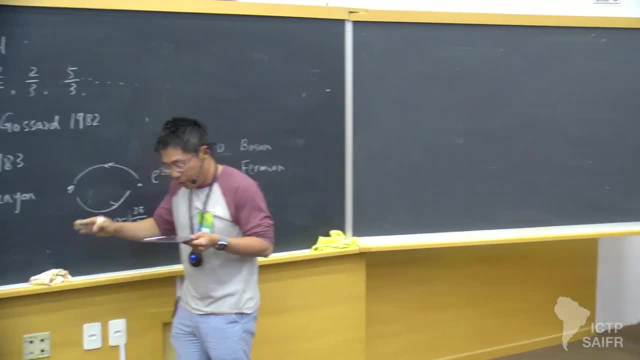 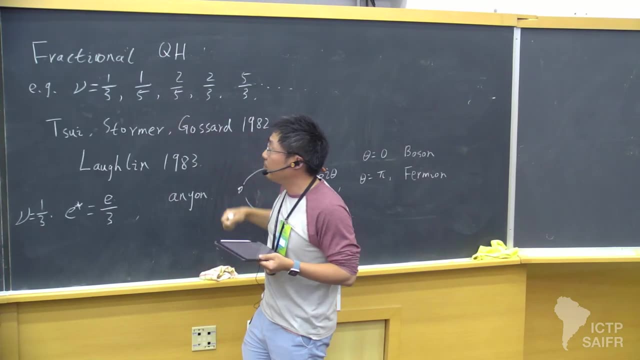 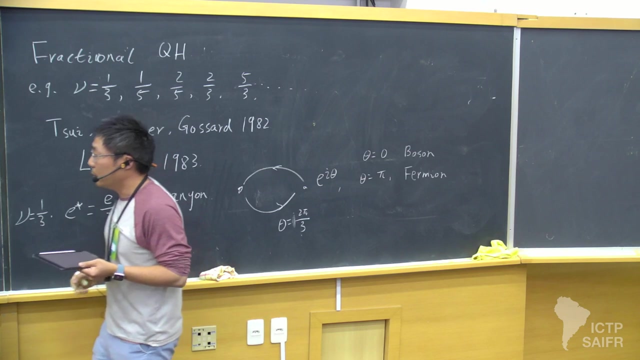 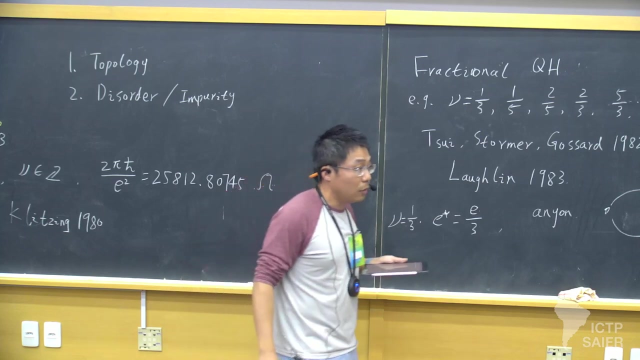 Okay So, but this lectures will not really touch that. If I have time I will. at the end of the lecture I will explain a little bit about the physics of this fractional-conhoy effect. The major part of this course is to understand the so-called integer-conhoy effect. 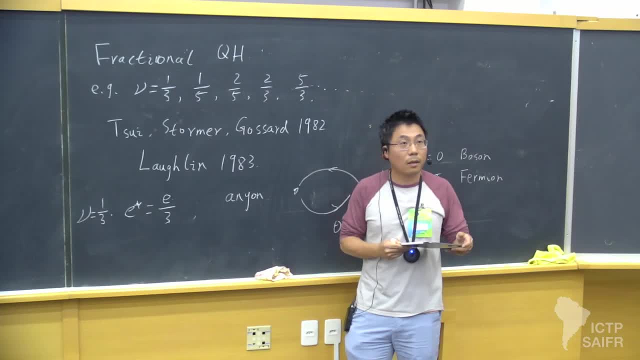 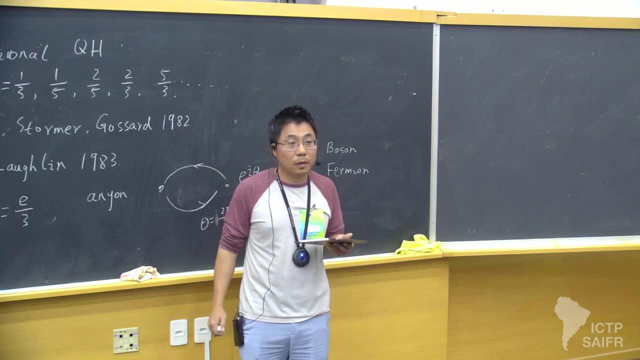 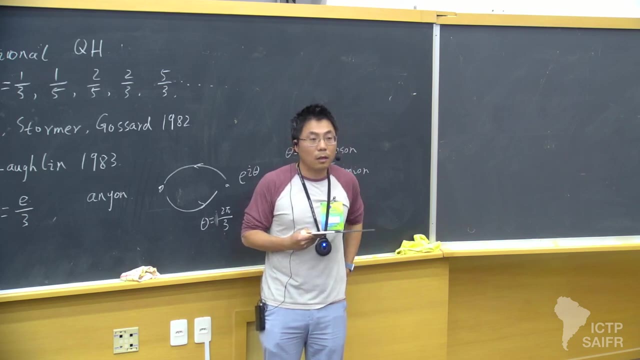 So any questions? Okay, Thank you, Got it Here in the next slide. Yeah, Yeah, You said that the expectations have a fractional target. Yeah, in the permisses of, And what do you mean exactly by excitement? 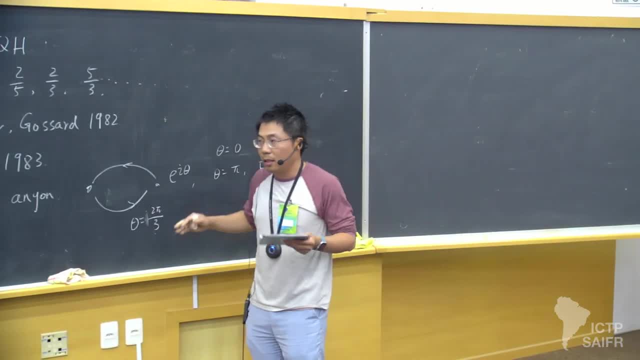 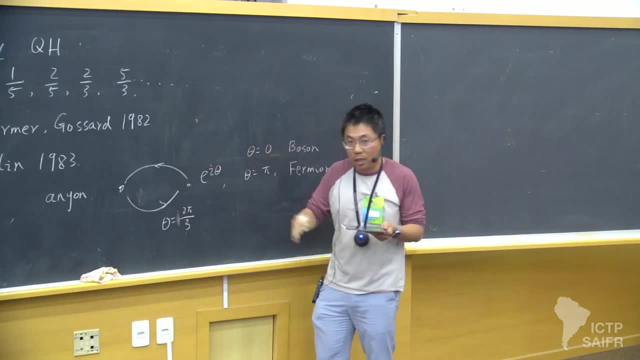 Thank you, Thank you, All right, All right, All right, Thank you, Uh, so I would like to ask one more question. Uh, so I have an objection. How come that, when you try to perturb the system, 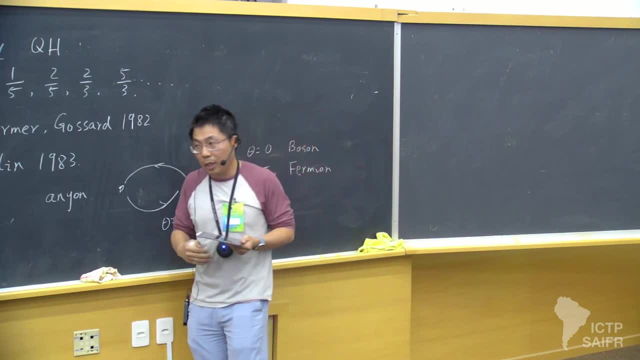 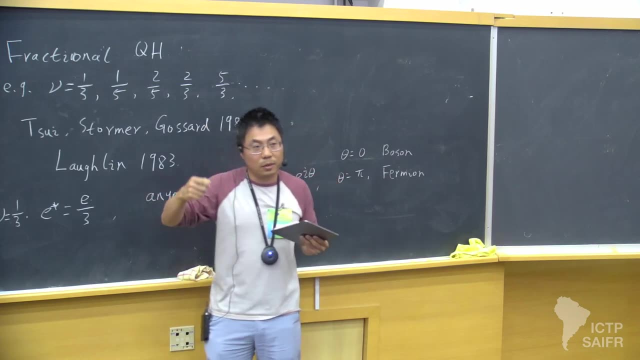 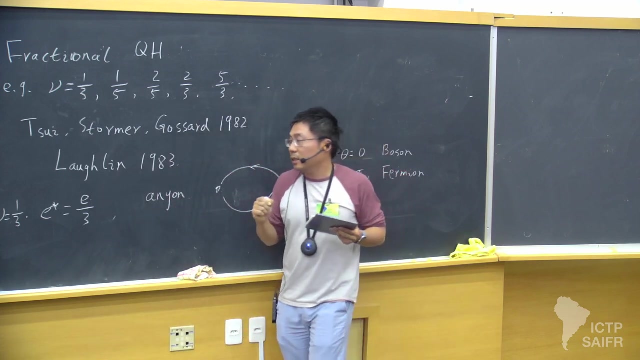 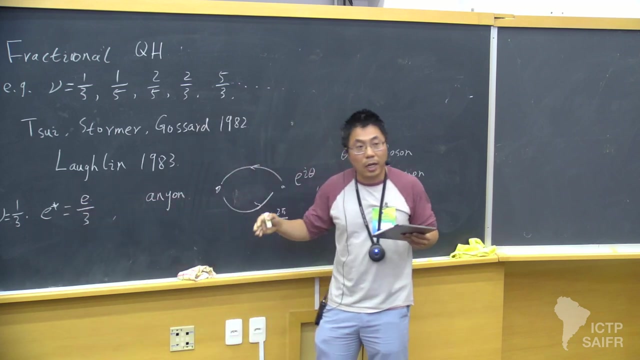 the system will respond, And you can quantify the response by just thinking about. you excite some particles in the system that move around, That is what we call the excitation, And here then you will find that the excitation will carry like one surcharge. 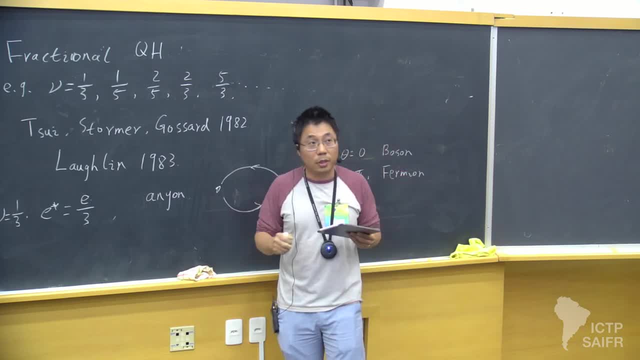 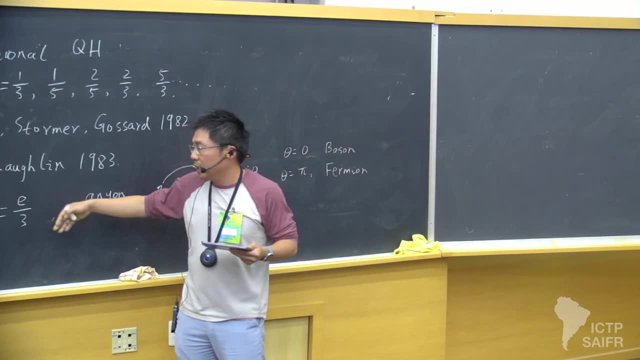 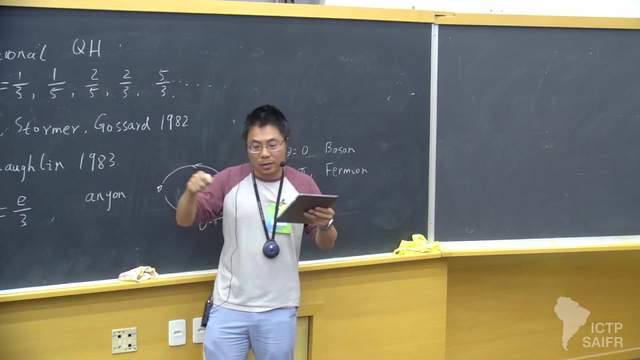 Of course the thing is, the system is always built using electrons. So then that means, if you really excite the system, what you will see is that you will simultaneously inject one electron in the system, And then you will see this one electron effectively. 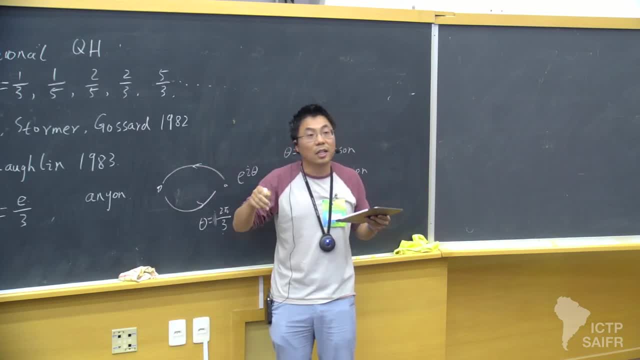 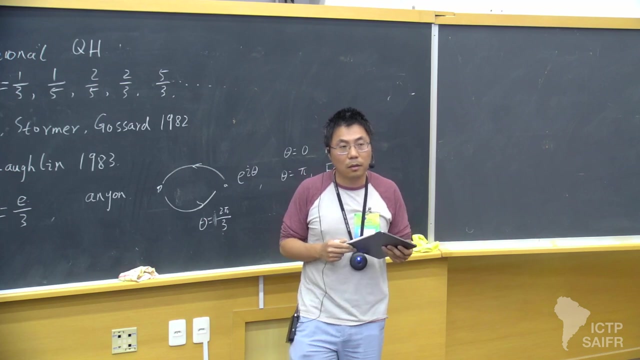 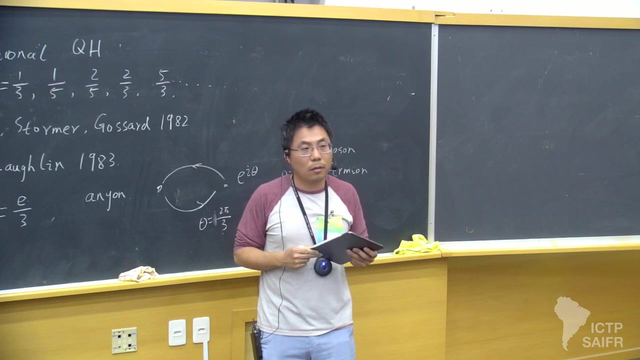 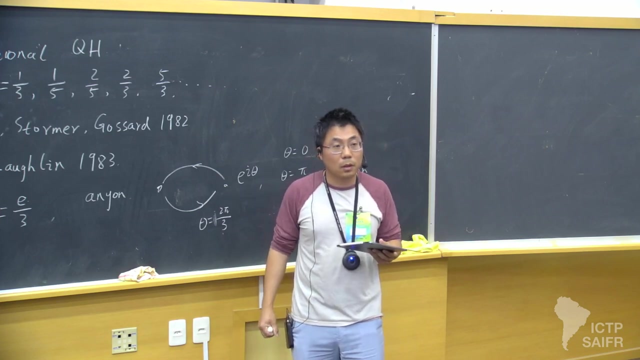 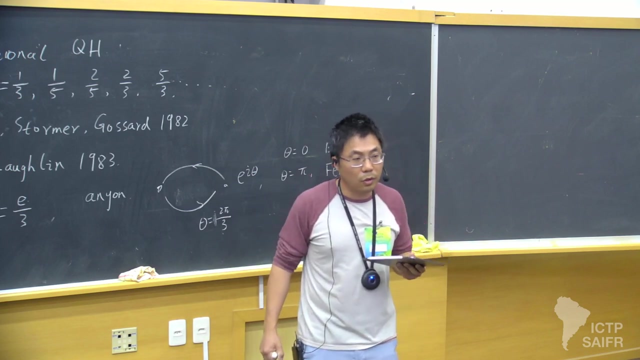 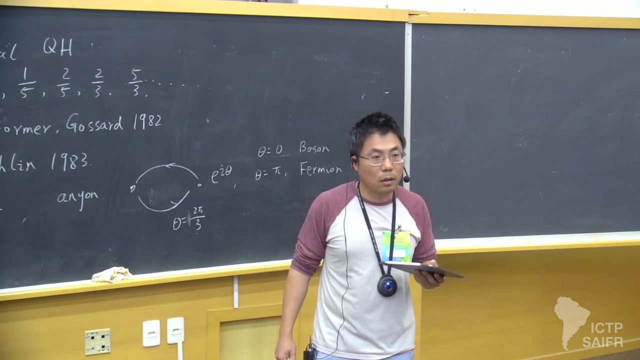 gets blitzed into three independent excitations, each carry one surcharge. They can move independently. That is what we call excitation. Yeah, Not sure. if you asked The excitation, they are in a similar activity to the whole particle in the incandescent. 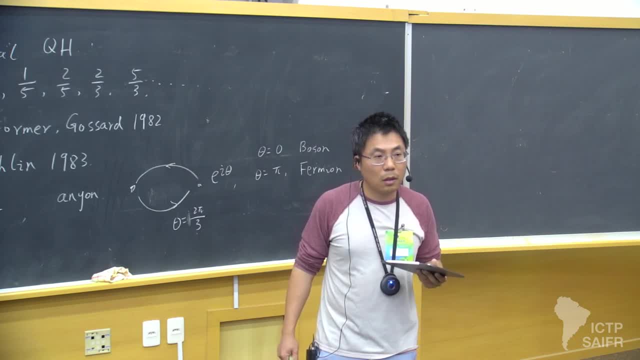 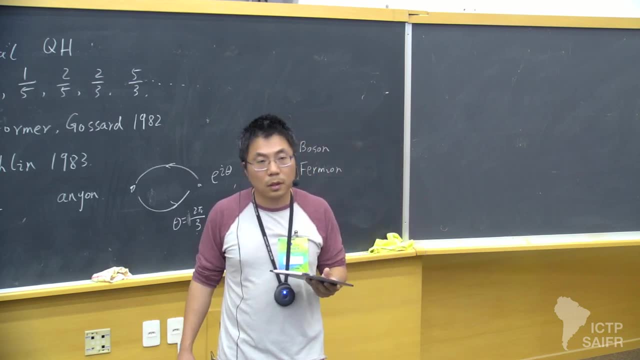 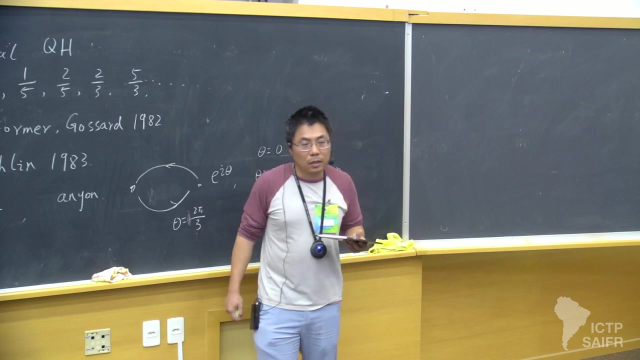 That is, it does not really exist, but you model the system to the whole. I think what you're trying to say is like the direct scene was modeled by electron holes, So the hole moves around the particle. It's a little bit similar. 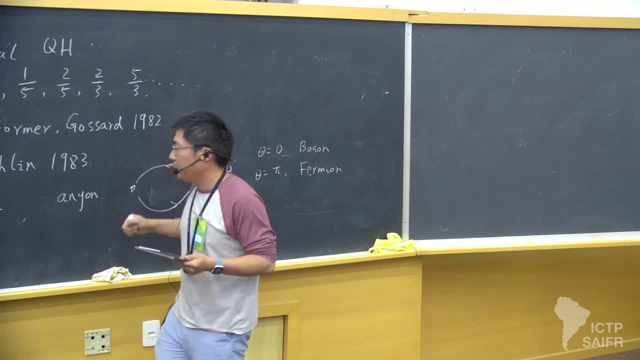 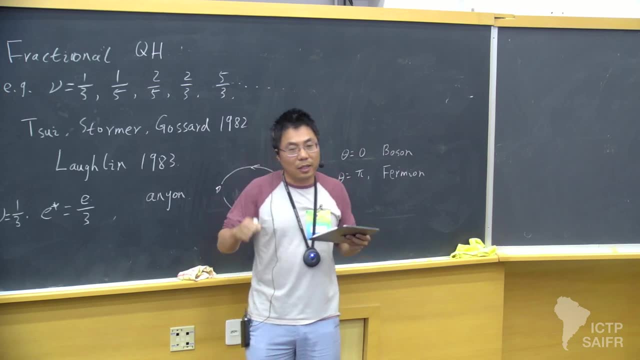 Yeah, The concept of excitation is that it's a collective behavior of the electrons, right, Yeah, It's like a collective behavior coming from many electrons. They move together and so on. Then effectively you can think it as some excitations in the system. 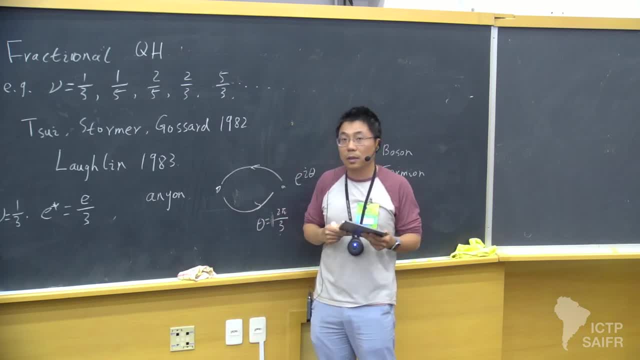 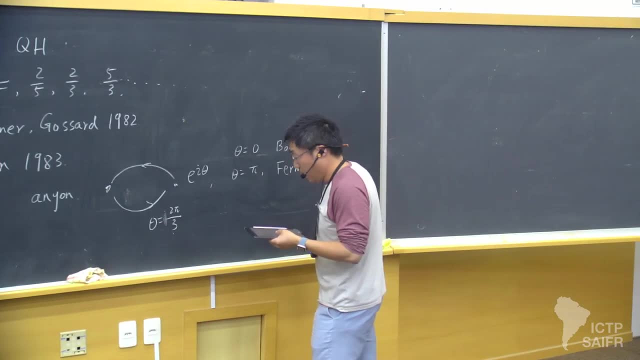 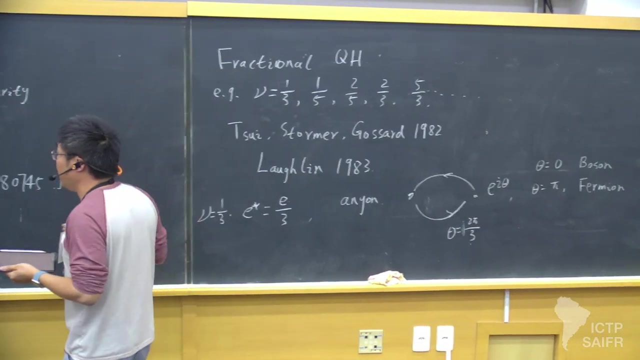 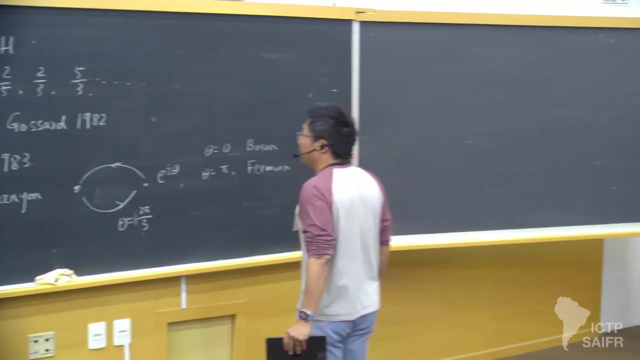 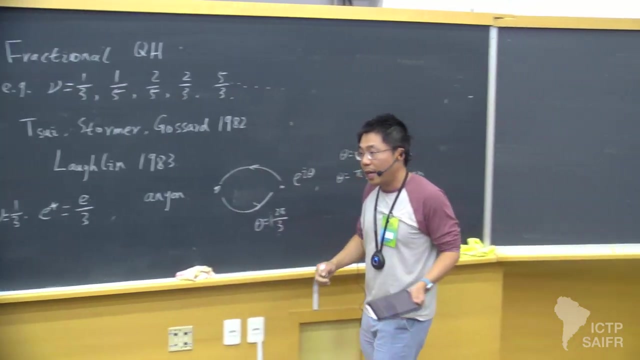 So that is the basic experimental phenomenology of the integer-quantum Hall effect, as well as the fractional quantum effect. right? And one thing you may say, that is okay. those are experimental phenomenon that has been observed for decades, so why do we still care? right? 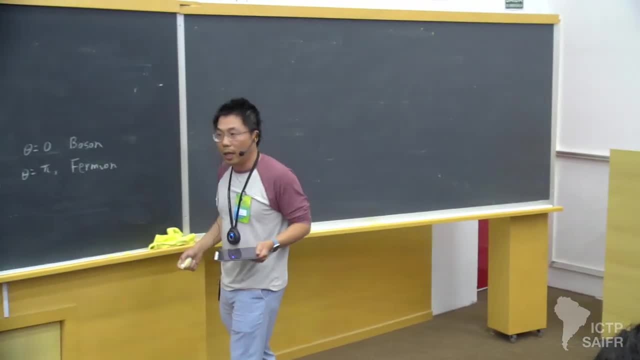 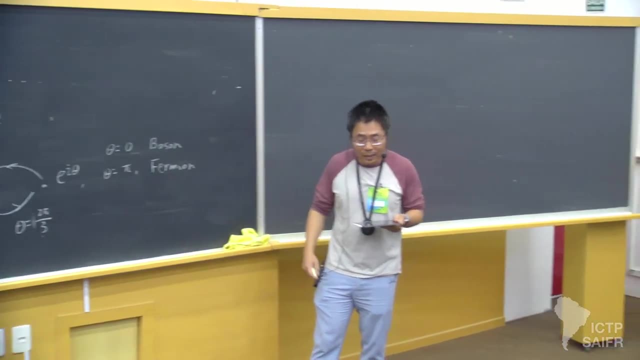 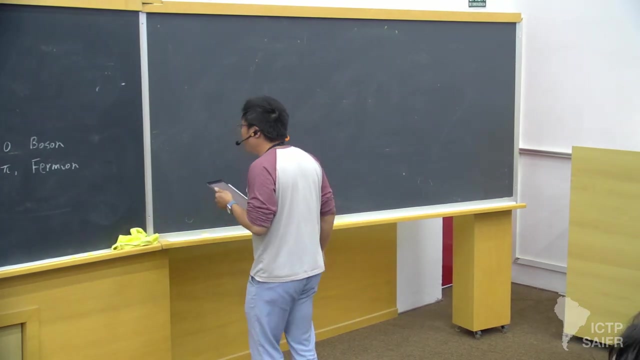 And indeed there are many reasons for us to still. It's still a very, very active research field right now and there are many reasons that why we really want to care about those quantum Hall effect. So one thing is that it do have application. 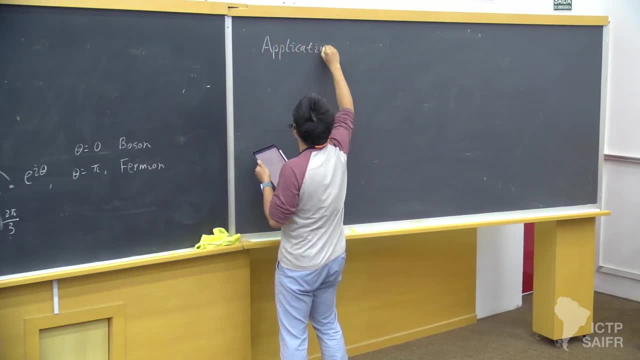 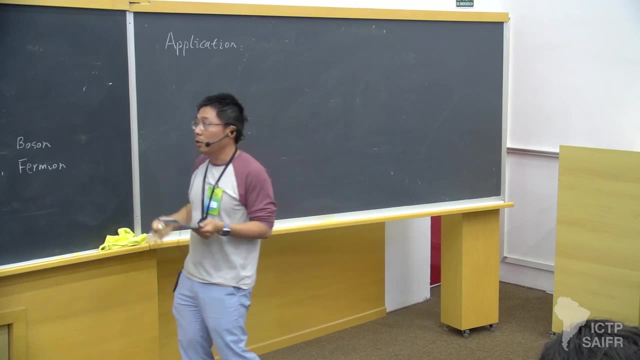 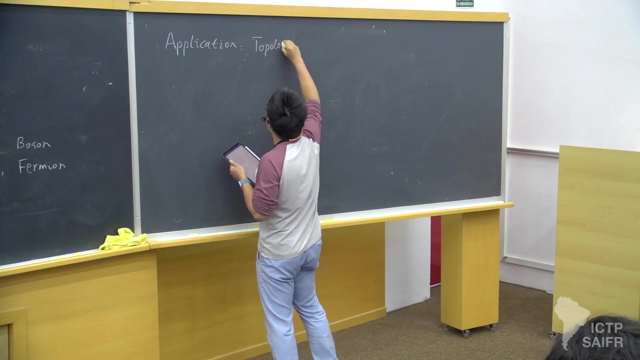 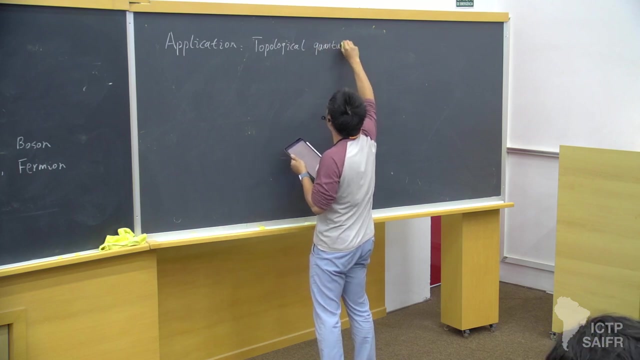 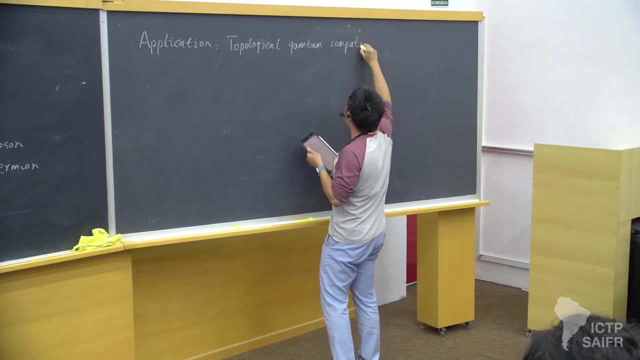 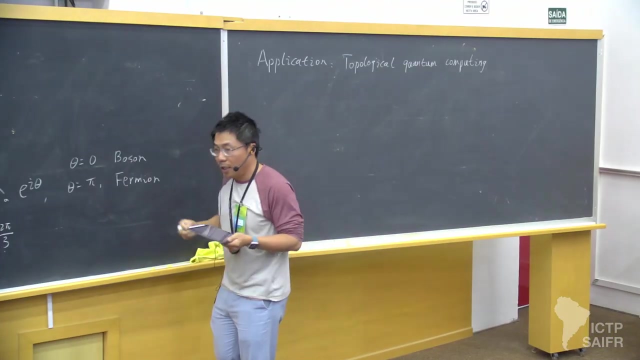 Pretty cool applications- Yeah, I should say potential applications. That is, you can make use of those fractional quantum Hall effect to make the so-called topological quantum computing, And the idea is that you make use of those so-called ANL36 that you can end up with quantum computing scheme that is error-free, right. 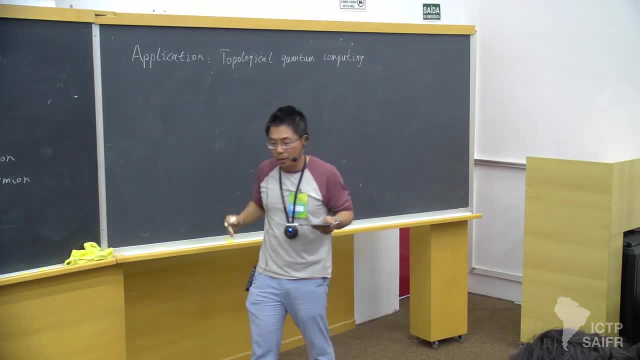 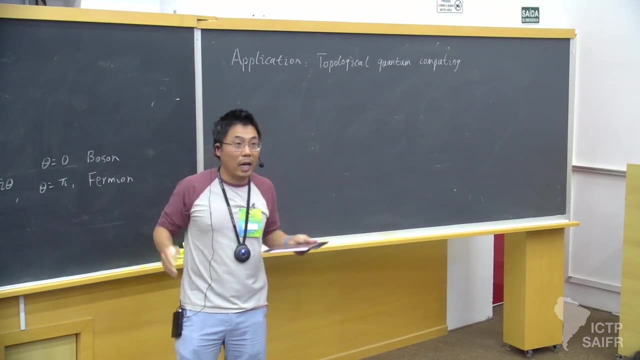 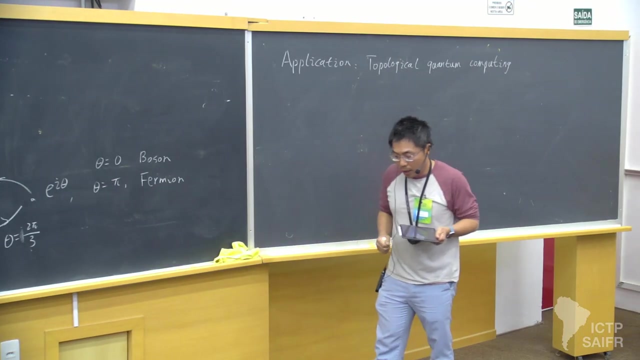 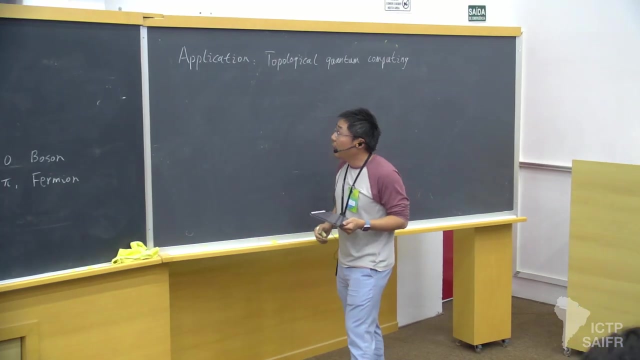 You know, nowadays quantum computing becomes very popular subject. Many big companies have their own quantum computing devices, but all those devices suffers very large errors, which is very hard to really use it to do to to apply to the problems that we are interested in. 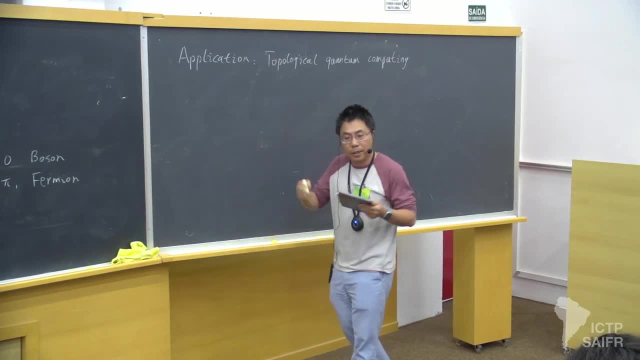 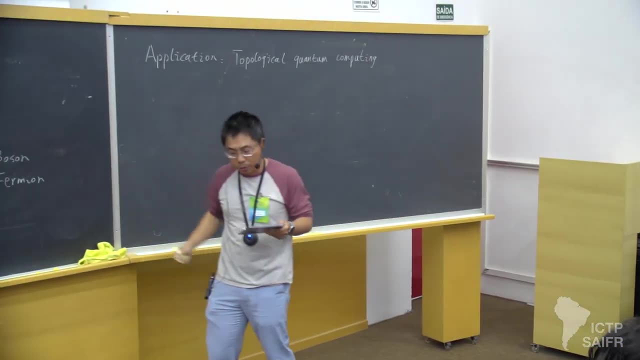 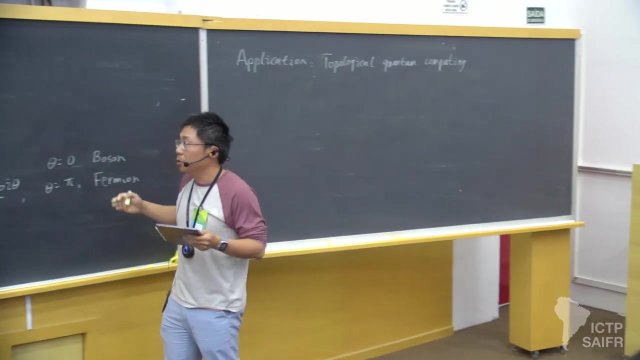 And the idea of those topological quantum computing is really a computation quantum computing scheme that is error-free, that there's no error at all in such quantum computers, And to build that we want to make use of the so-called topological order. 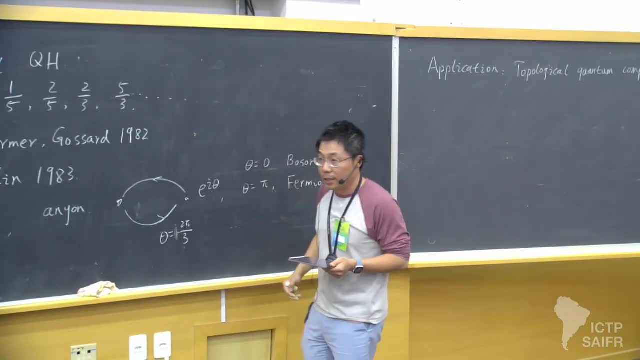 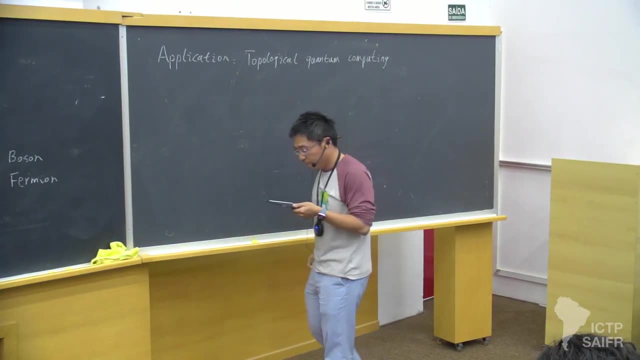 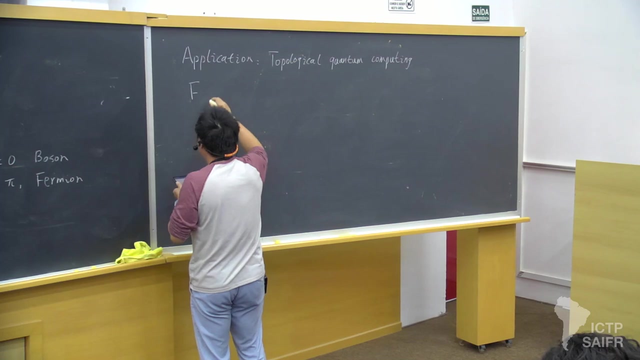 or topological quantum field series and fractional quantum Hall effect, is really the the most promising platform for realizing this topological quantum computing, And And So I'm a theorist. So then, For me, quantum Hall is really something that has a lot of fundamental importance. 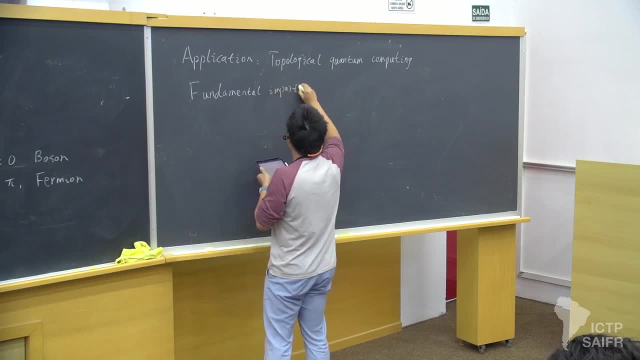 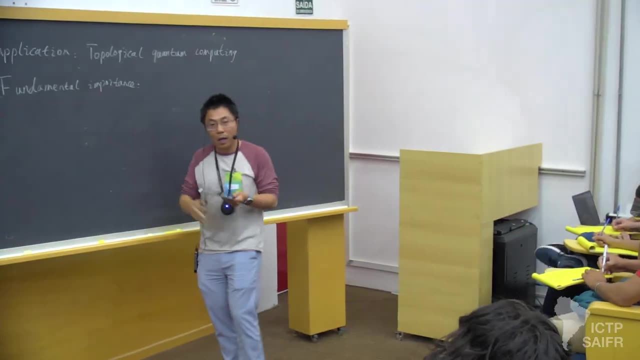 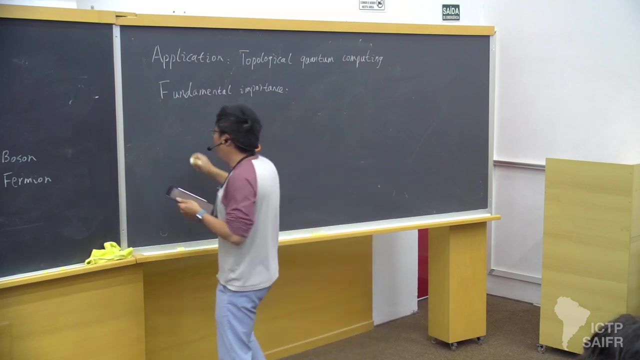 And very often that's the quantum Hall, is the? is the? is a resource that we can get a lot of inspirations of various theoretical physics in different field. For example, what I have mentioned is that topology plays a very important role. 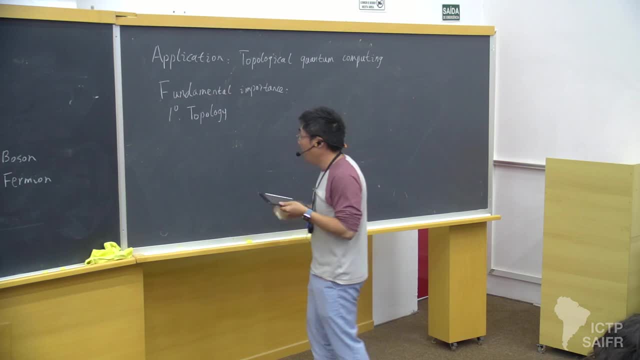 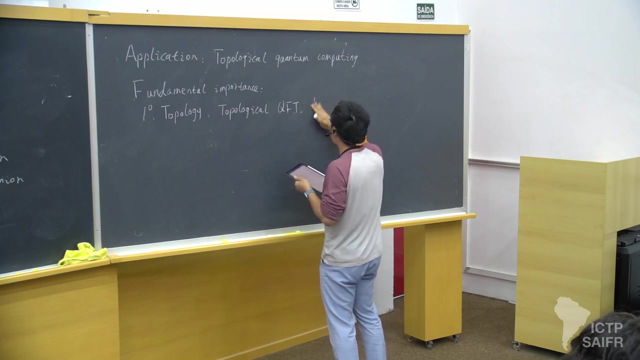 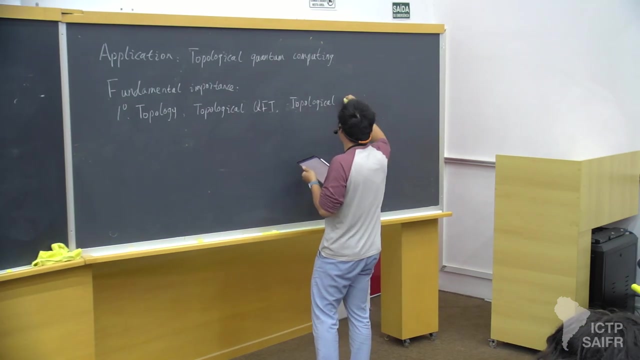 in the story of quantum Hall physics right, And more generally it's related to the so-called topological, topological quantum field theories- And in condensed matter, literature it's also called topological order- that people have been studied for decades. 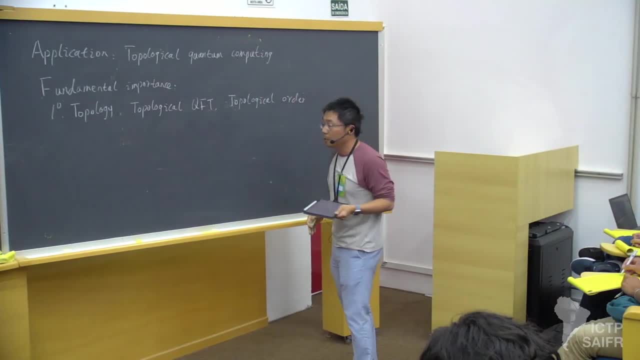 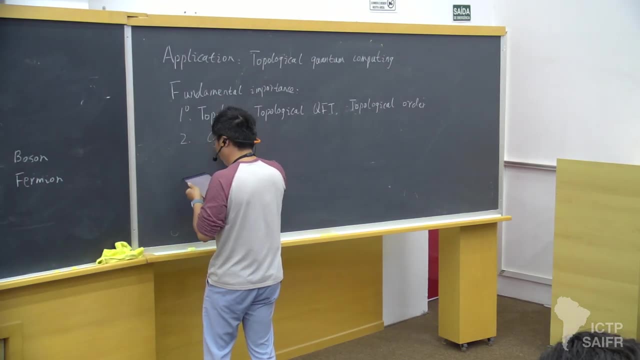 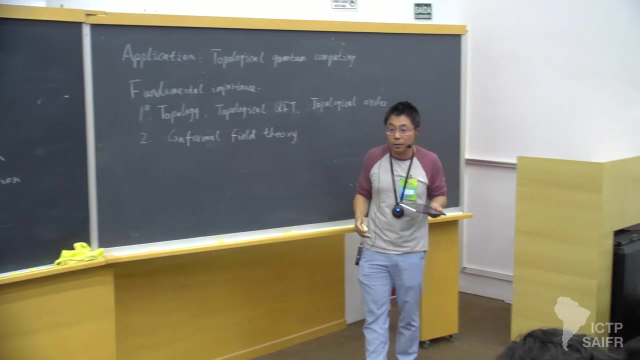 And all those really are studied from this quantum Hall effect. And the quantum Hall effect also have deep connections with the conformal field theories, which is another type of quantum field theories that is closely related to many physical phenomenons like phase transitions. that 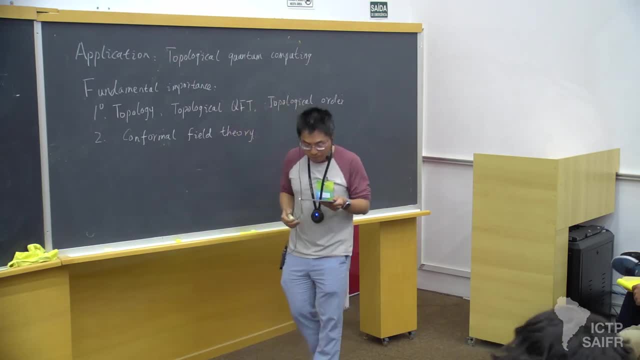 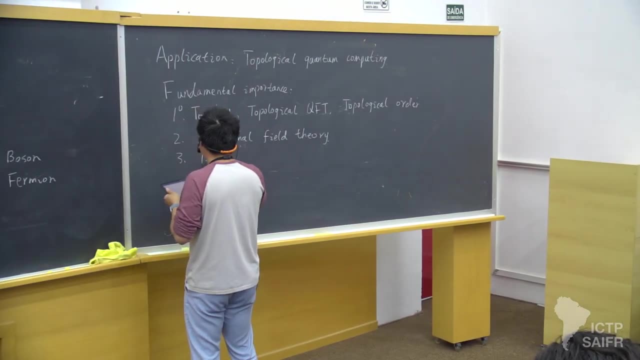 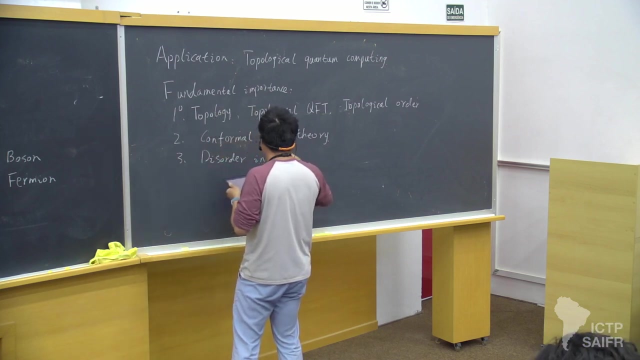 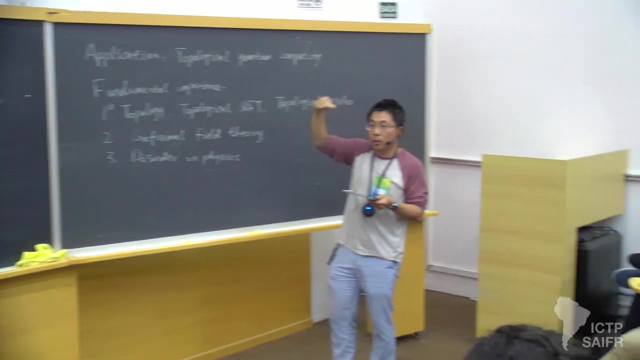 like phase transitions in Eisen model that Juan mentioned talked about in the morning. And the other thing is the like the disorder in physics. as I explained, the disorder is really the key reason for you to get the those plateaus of your Hall resistance. 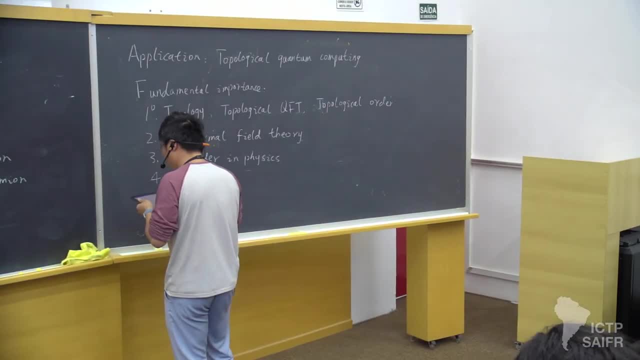 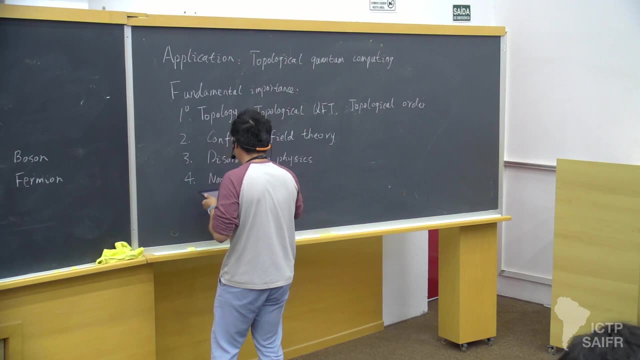 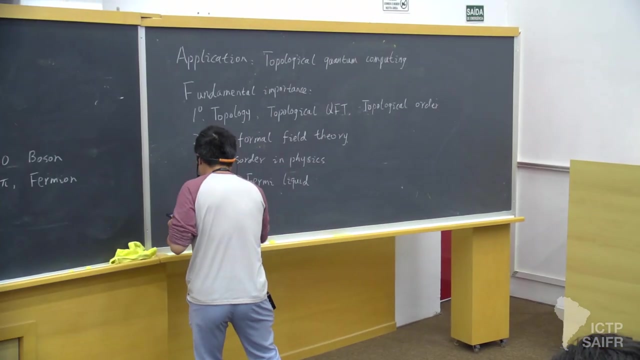 And the quantum Hall effect also have. the such is also related to can also realize the so-called non-Fremont liquid, which is a very important type of quantum matter. that also happens elsewhere And this also has close relations with the. 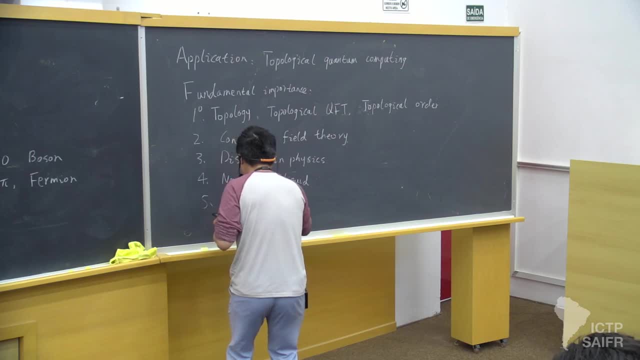 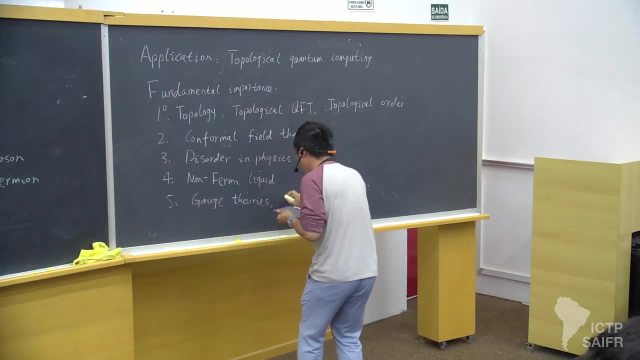 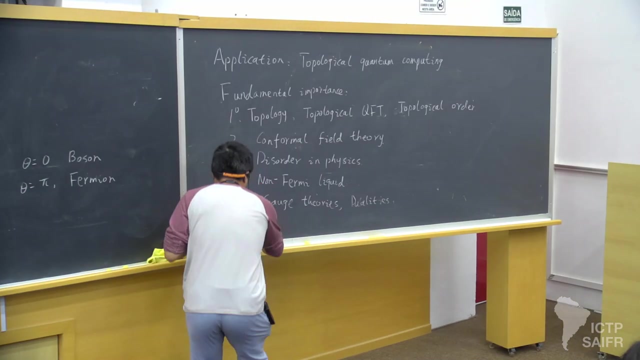 let's say, gauge theories, and as well as the something like dualities of gauge theories that Nathan has mentioned in the morning in his class of supersymmetry, And there also are some other things. One thing is that get me excited. 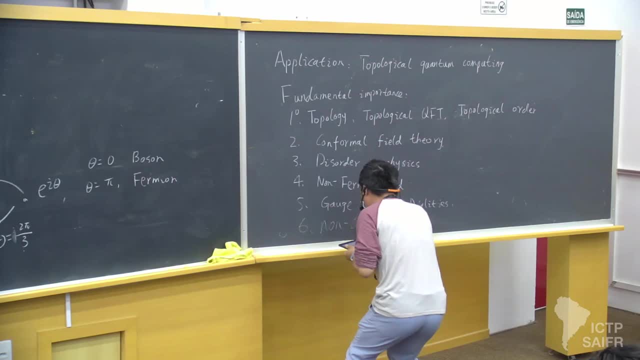 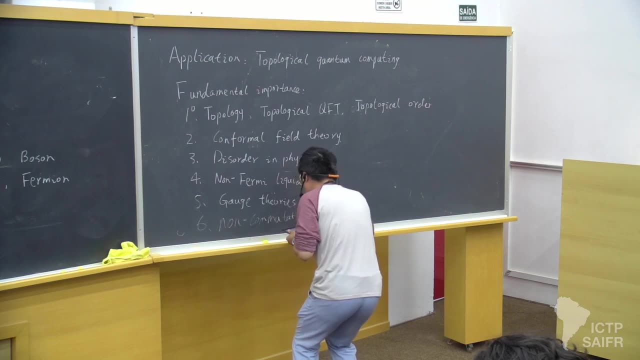 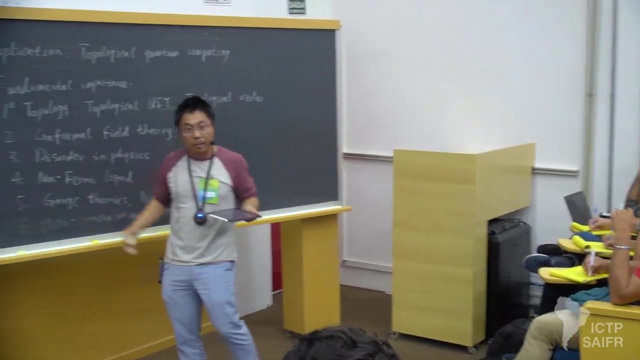 recently is the so-called non-commutative geometry, which is also naturally appears in the in the quantum Hall context. So this list can actually be much longer right, And I can. I can spend a semester or a year to talk about the physics. 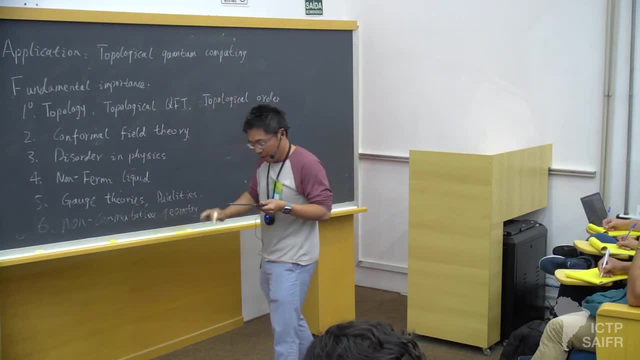 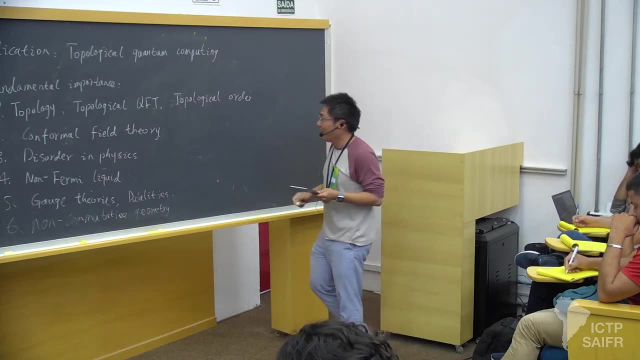 behind this quantum Hall physics, but I will not do that. But let me also mention one slogan about quantum Hall that I really like is that it's like all in Hall, And that's literally true. Oh, No, no, no. 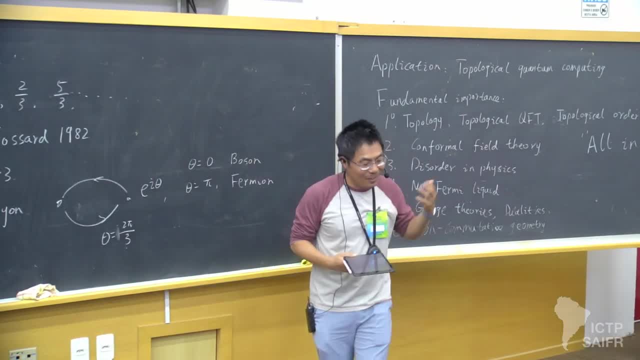 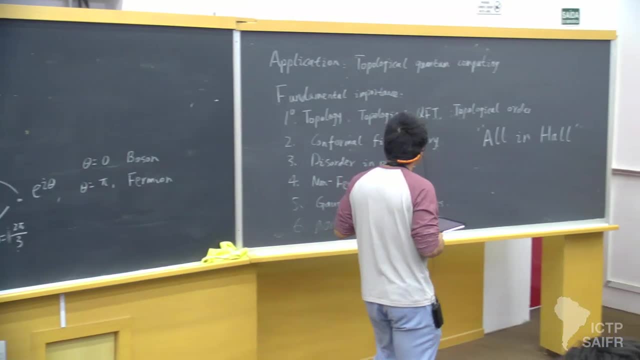 It's just a slogan. Yeah, Yeah, Some people wrote a paper with this title, but it's probably not. Yeah, But it's not really what I want to say. So the point is that the physics behind quantum Hall effect is really very, very rich. 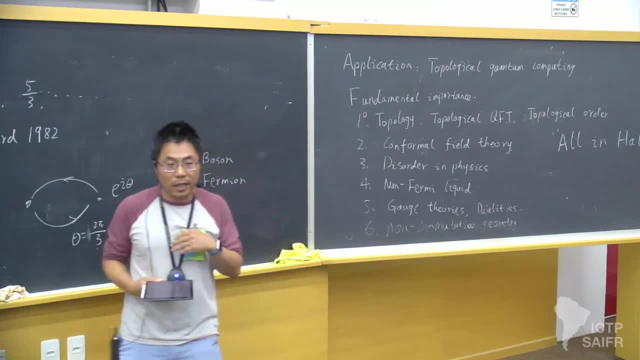 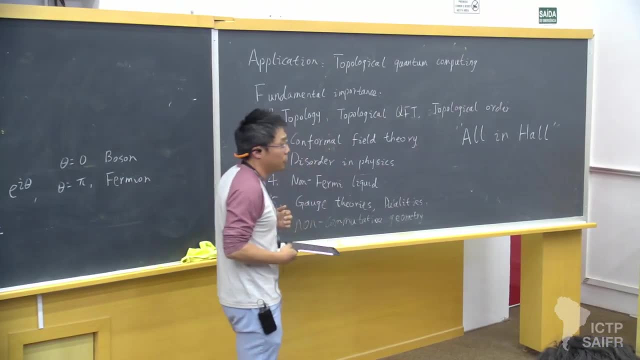 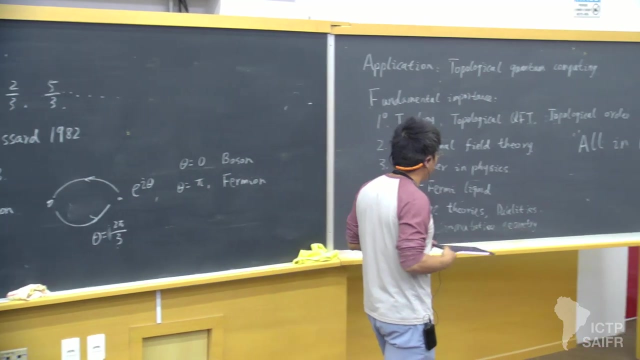 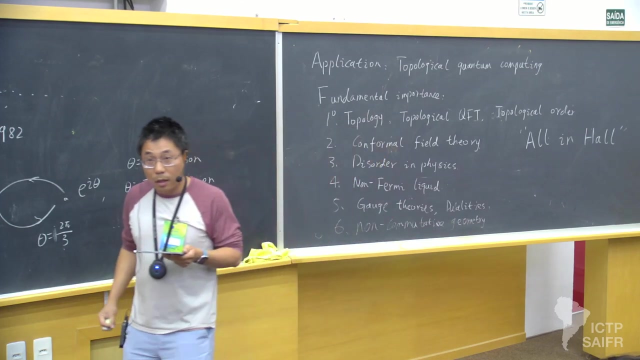 Yeah, It connects almost every single things that we think, we thought theoretically And that's really give us a lot of inspirations about, about various physics- theoretical or even experimental physics that could happen in quantum matter, as well as the high energy physics. 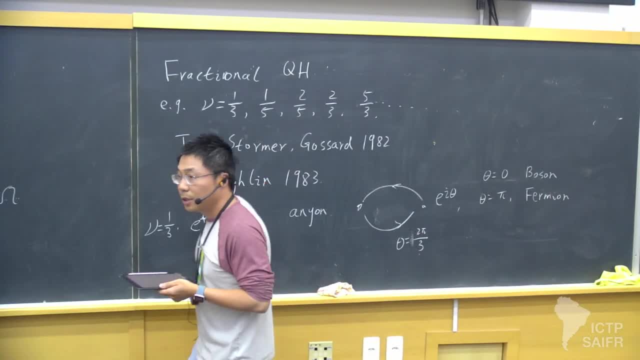 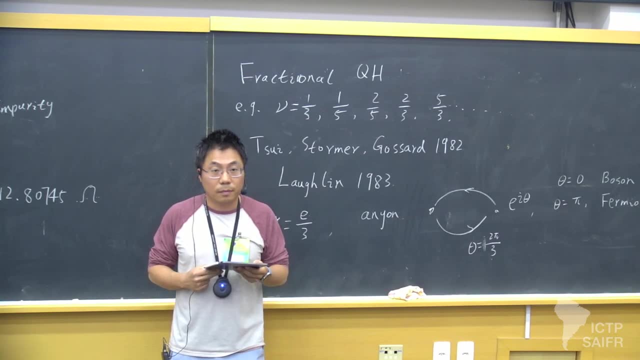 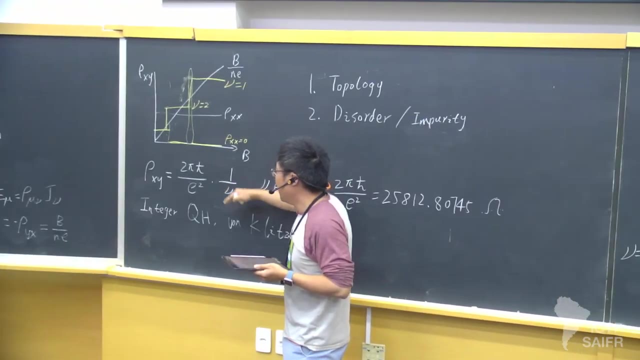 Okay, So I think I'm done with the introductions So I can pause a little bit for questions. So the plan of the rest of the lectures will try that. I will first explain the physical mechanism behind this integer quantum Hall effect If I have time. 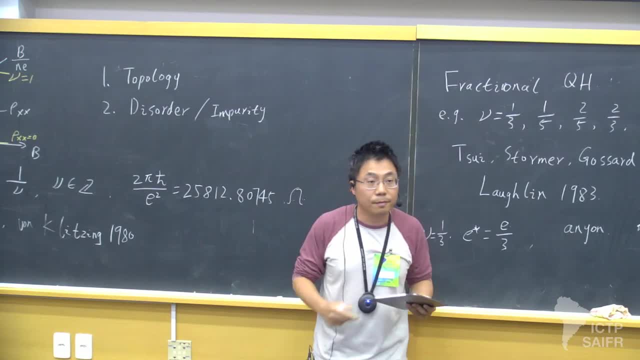 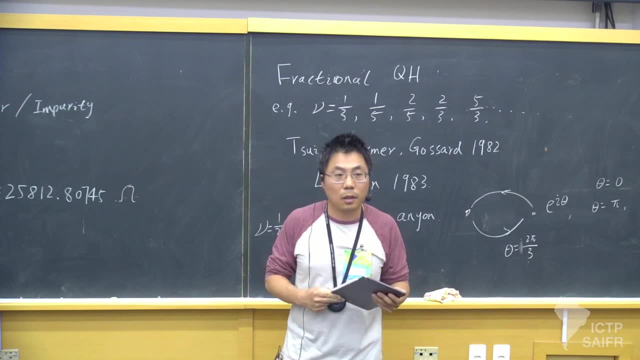 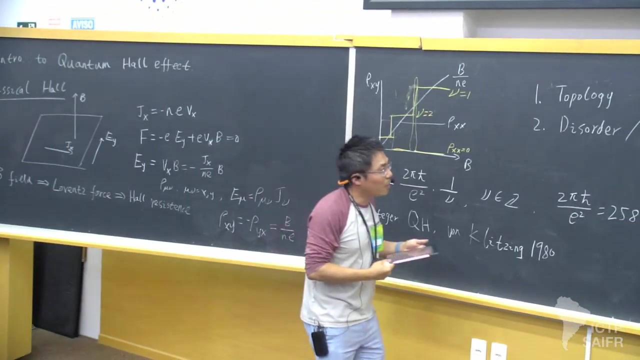 I will also talk a little bit about fractional quantum Hall effect. So I'm asking the: the size of the plateau Is that? Yeah, Yeah, Yeah, It turns out to be controlled by the disorder strength. Yeah, The stronger the disorder is. 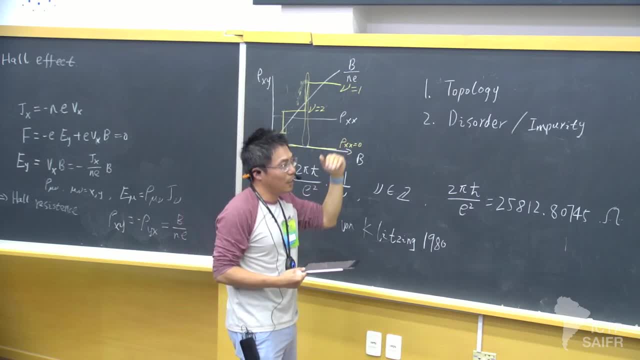 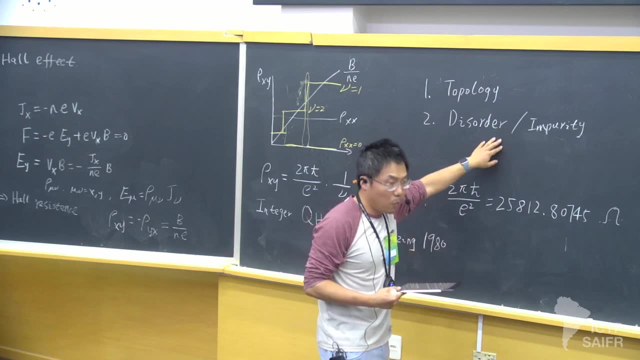 the wider of this, of the plateau is, Of course, there there's a some cutoff. that you cannot have disorder to be infinitely strong, Right That That I will explain this later in this talk- Right, If you don't have disorder. 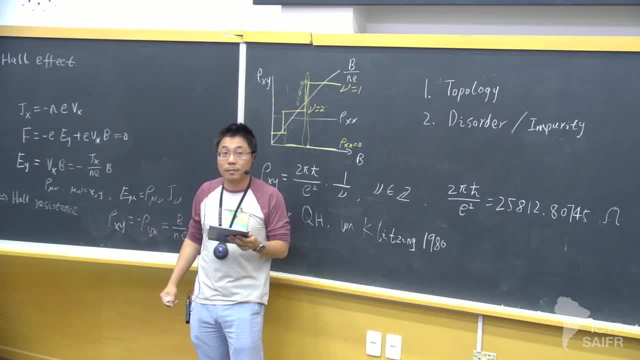 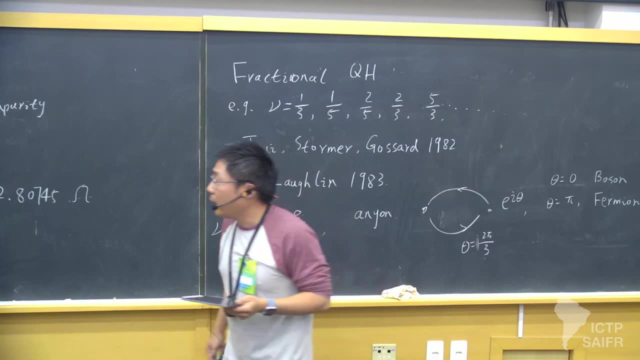 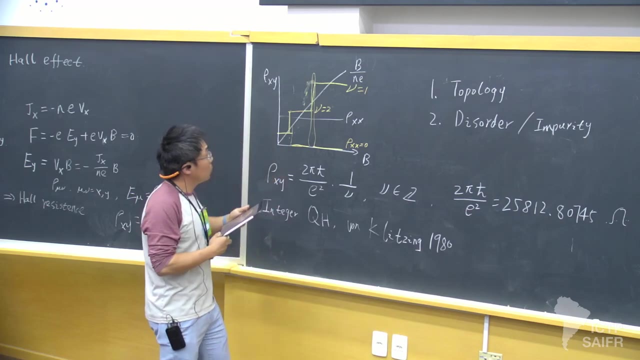 then you don't have plateau at all. Yeah, Yeah, Yeah, Yeah, Yeah, Yeah. So yeah, One thing I, I I didn't mention, is that one thing you, you could notice that I, I draw it in purpose- that 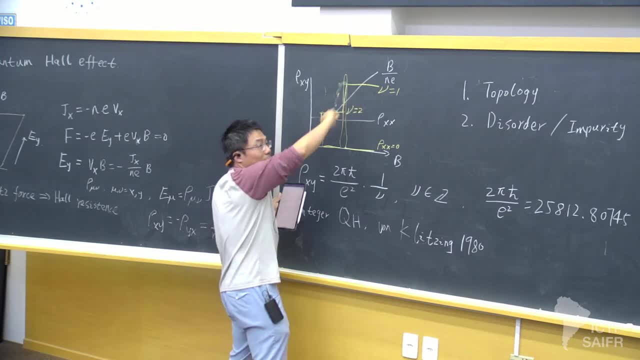 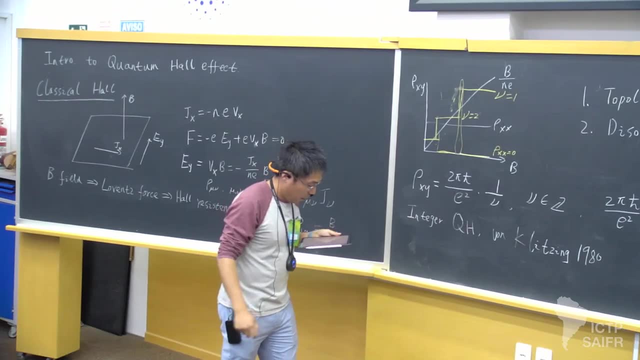 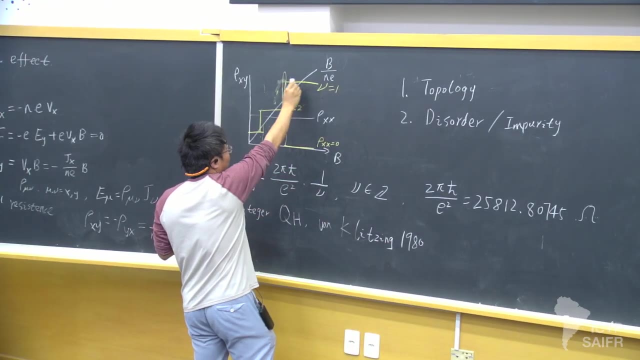 on purpose that each plateaus actually intersect with my classical trajectory of the of this Hall: resistance Right And And And then actually you can, you can read out the the rough, the rough value of the magnet field. 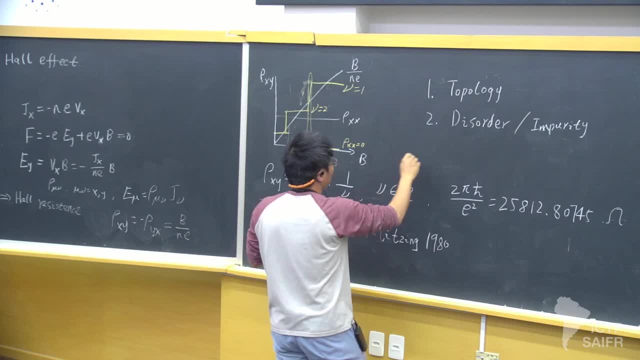 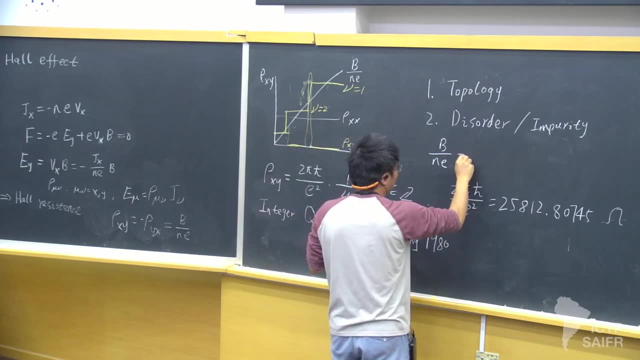 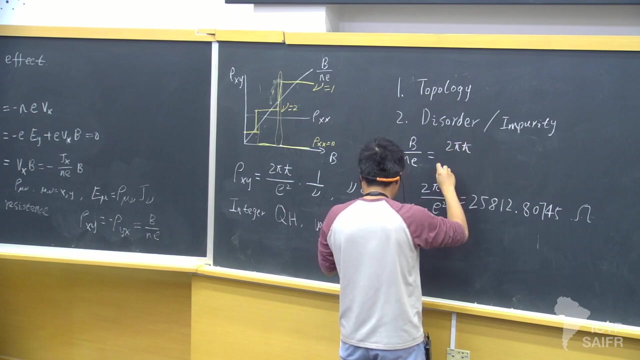 So. So the thing is, we should have this guy as some For For certain magnetic field. we should have this classical resistance equals to my quantum Hall resistance, Right, And then what you can get is this classical resistance. So 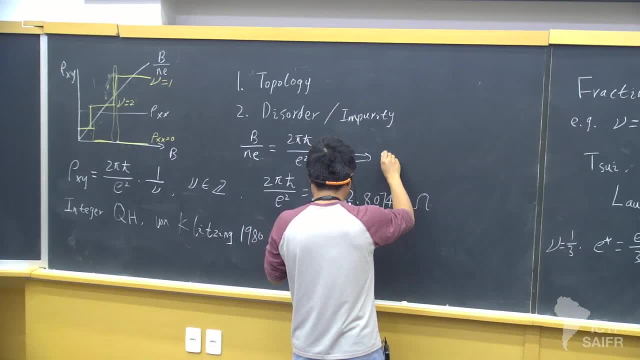 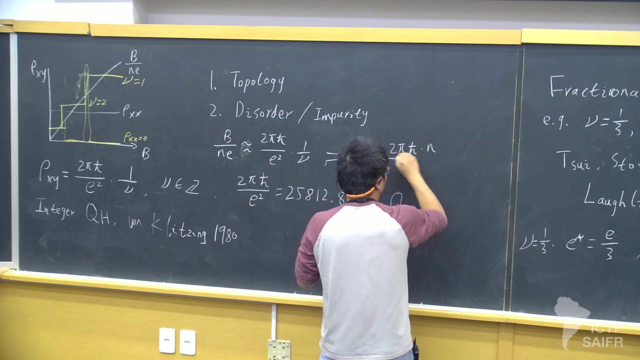 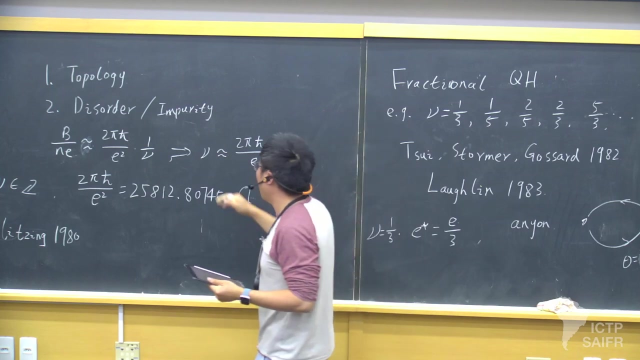 what you get is the roughly new. Let me use approximate value And then, roughly, this new will equal to 2 pi h bar times n over e times b Right, And So if you want a very large new, 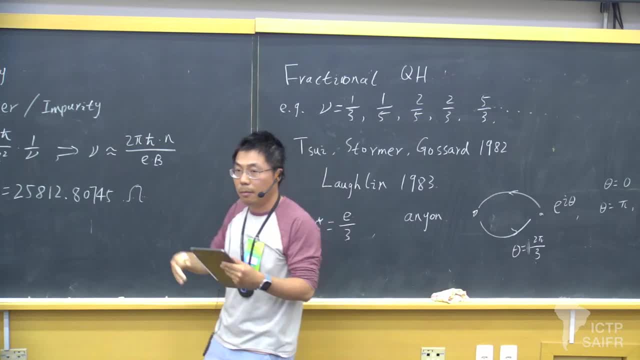 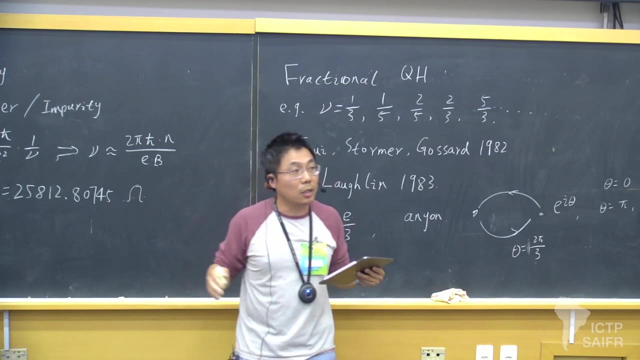 So the density of the charge carriers in my, in my material, and then, if you want a very large b, what you end up with is a very small magnetic field, And for that it turns out that there are some other. 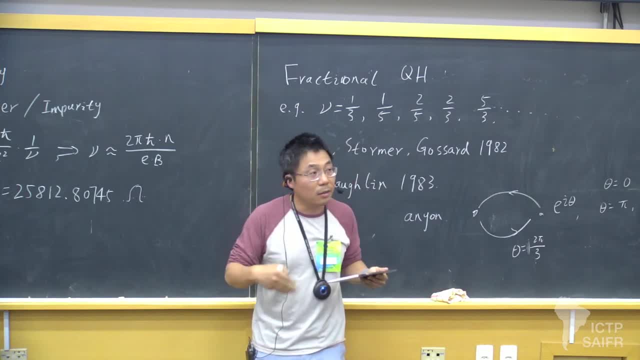 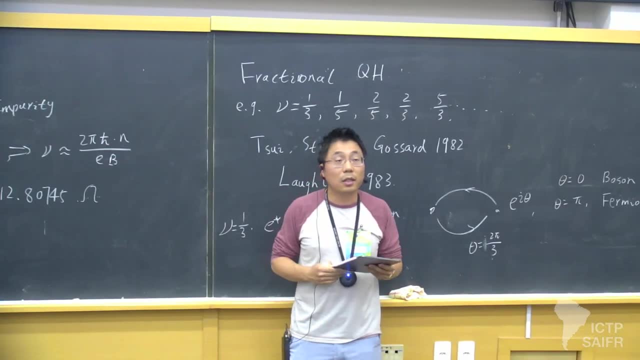 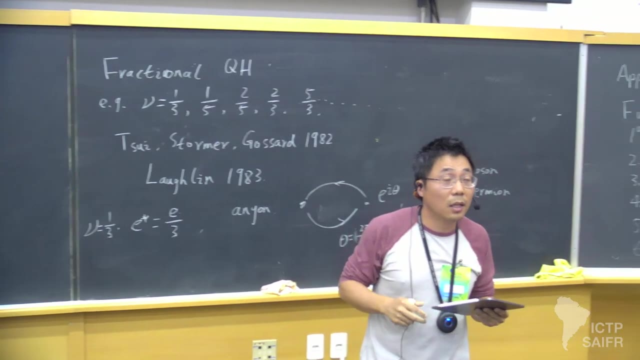 competing factors which may destroy the quantum Hall effect. So that's something I I will. I think I will explain more about that in a little bit, So let's go back to the previous question. Sorry, again, That's a good. 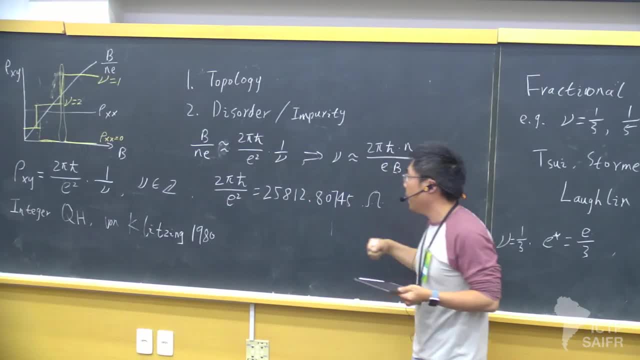 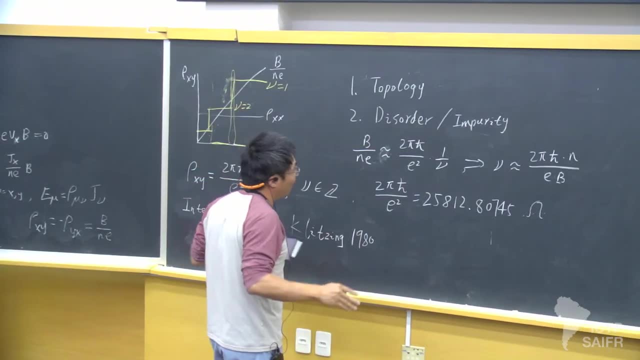 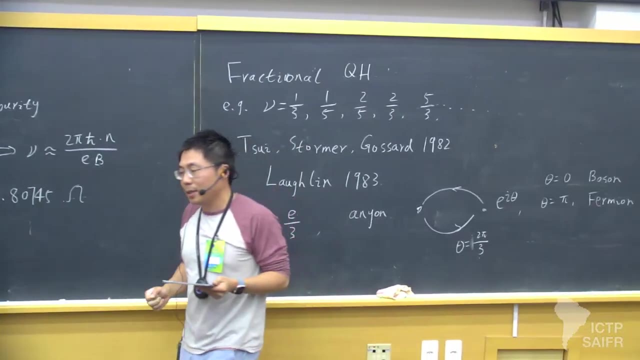 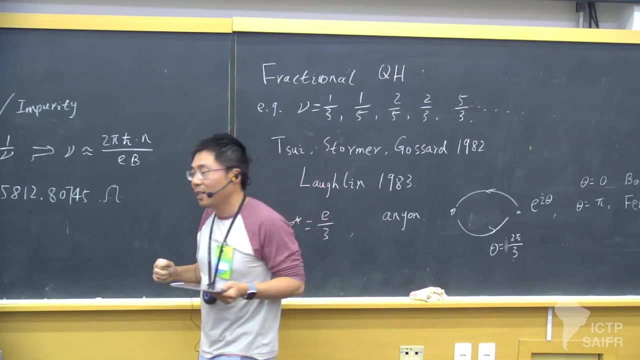 question. So I will. Okay, The question is: does it depend on the spin of the charge carriers? So the So the question is: does it depend on the magnetic field of the charge carriers? And then you can. 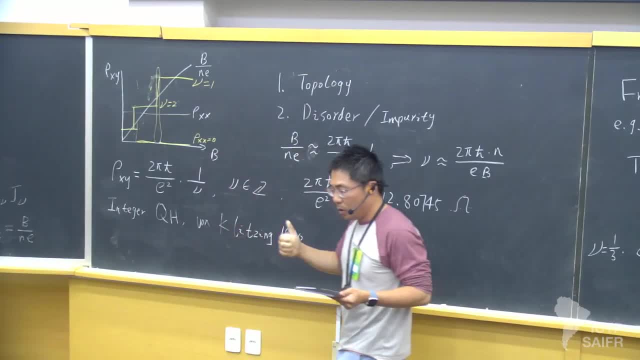 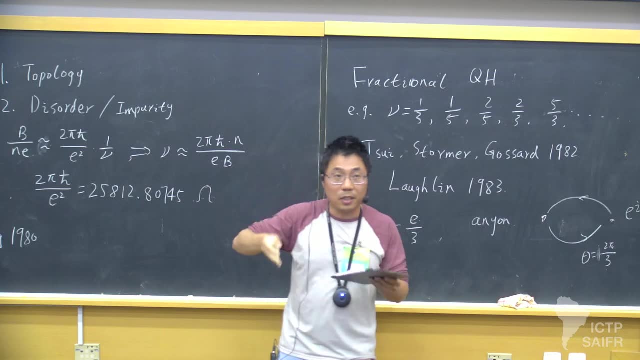 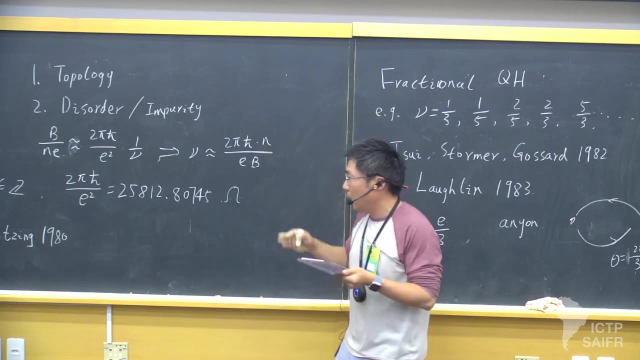 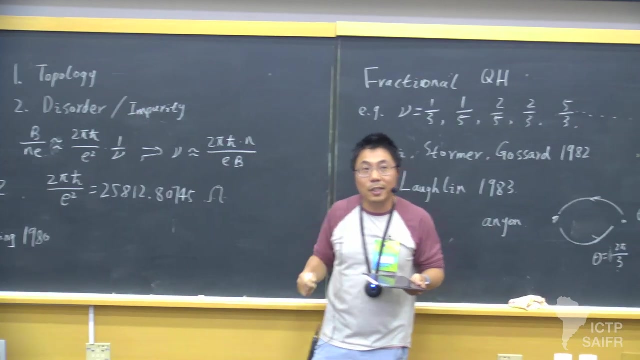 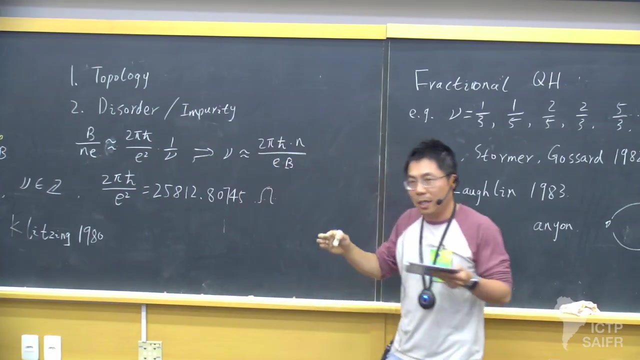 ask whether this spins plays a role in the quantum Hall effect. So a naive answer is that when you apply a magnetic field, we can ignore the spin degree of freedom in the quantum Hall for those quantum Hall effects. But in reality the story 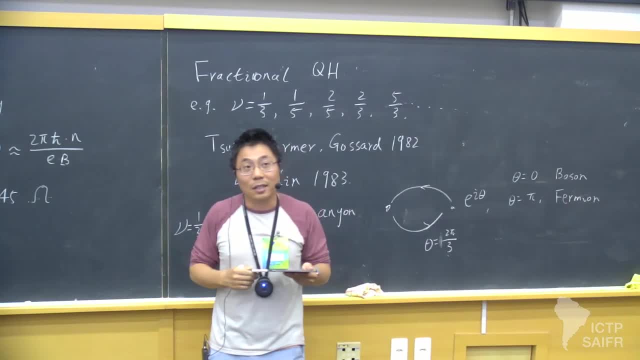 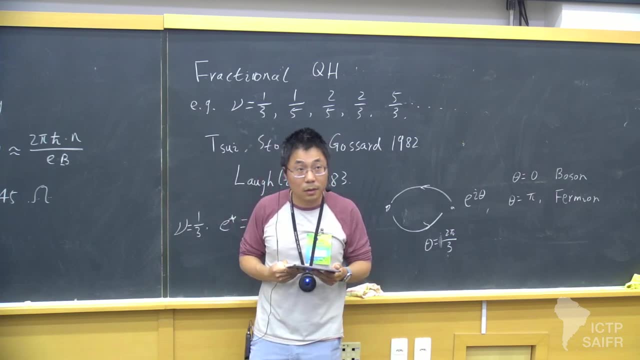 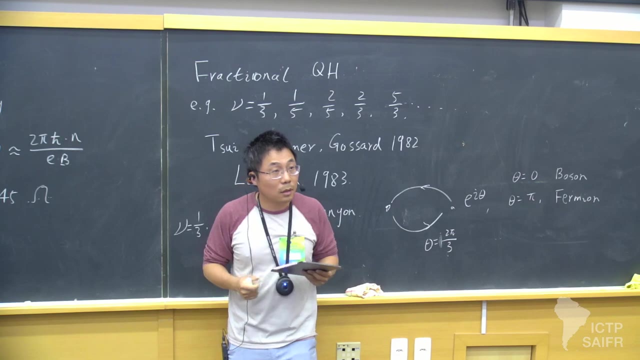 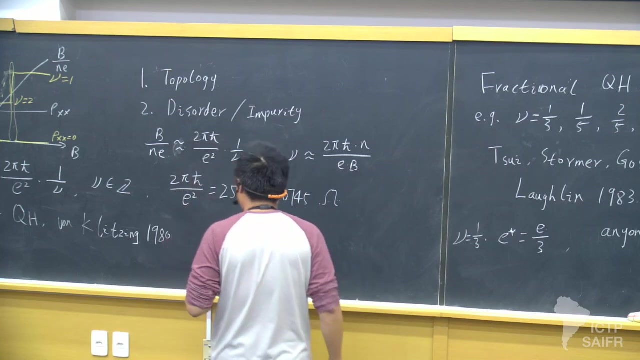 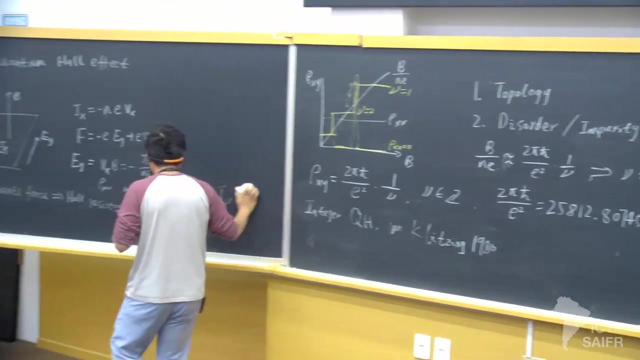 is much more complicated and also interesting if you consider the spin degree of freedom. So yeah, So, if not, let's start encoding the understanding, the physics of the integer quantum Hall effect And the most important thing to, I mean. 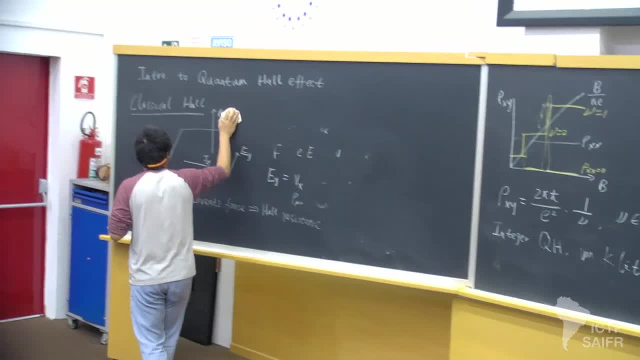 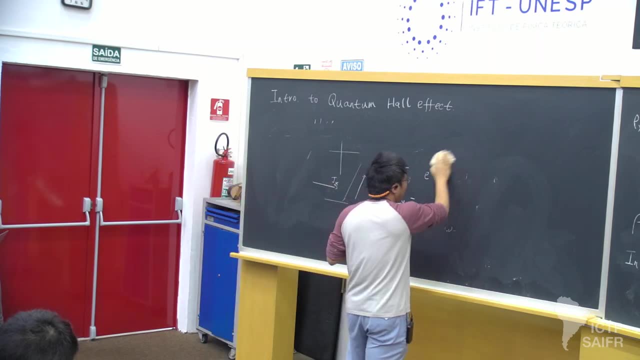 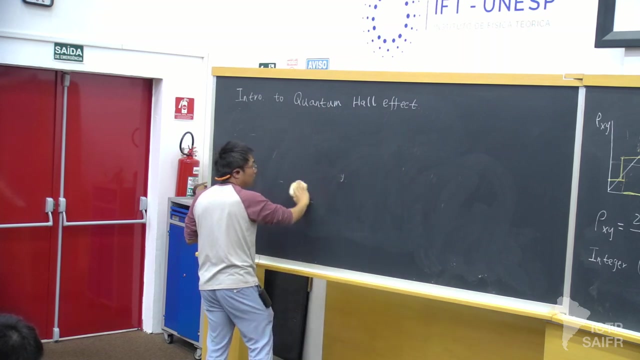 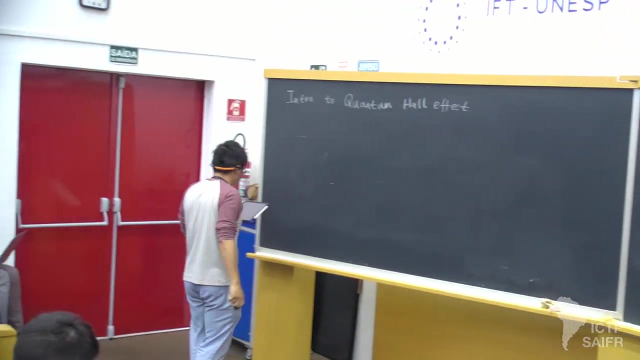 the starting point is to try to understand just single particles, Single electrons, moving in the presence of a magnetic field, And that's probably some problem that you have deal with or learned in quantum mechanical, quantum mechanics course And that is called Landau. 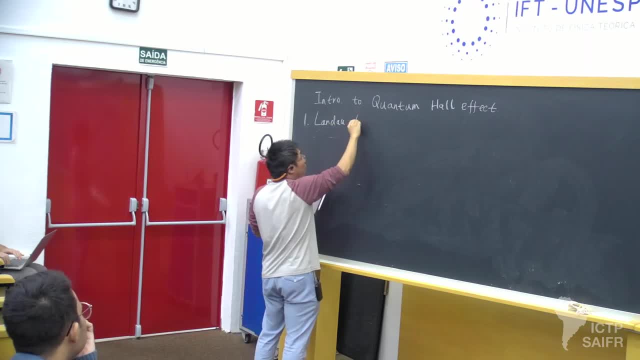 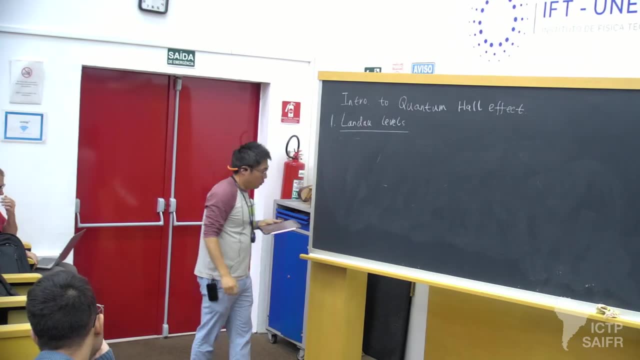 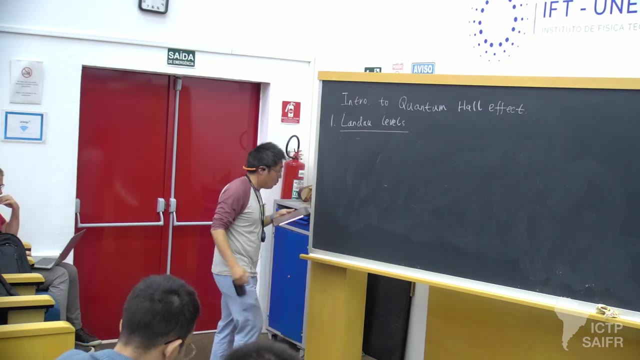 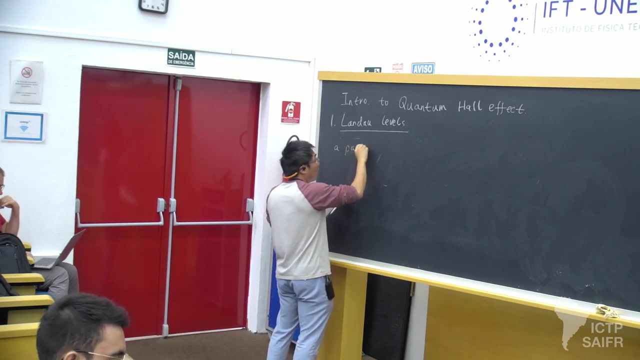 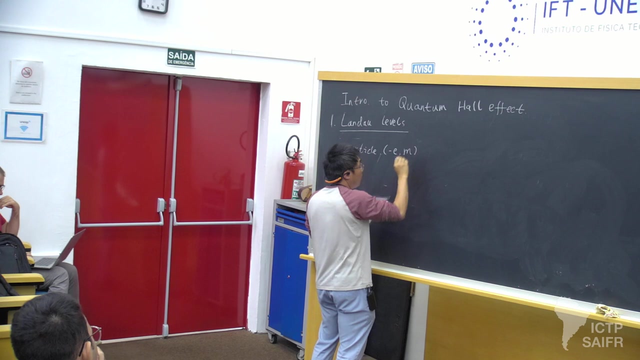 levels, So again. so now we want to consider again just this: electrons, that say we have a particle, which is an electron in my case, that carries charge minus E and with mass M right, And it's moving in the presence of a B field. 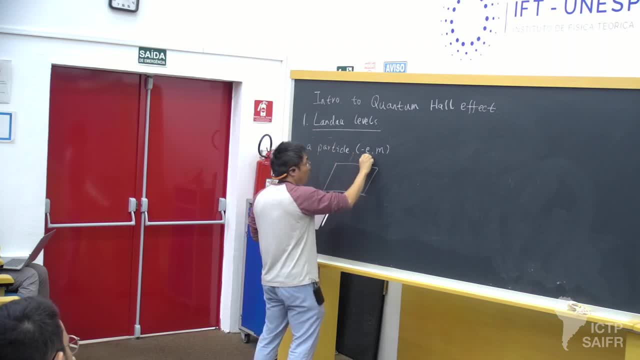 I should not erase this. So I do have an electron right just moving in the presence of this B field right. And now we? so it's a quantum, now we want to deal with a quantum mechanical version. 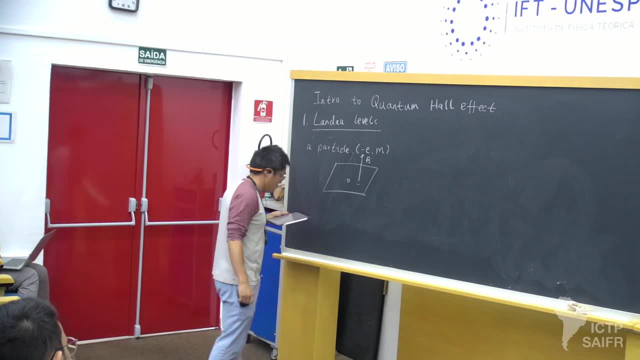 of that right And we so, and this and this. the solution of this problem is called Landau levels. So I will. so then I will, I will do those Landau, expand those Landau. 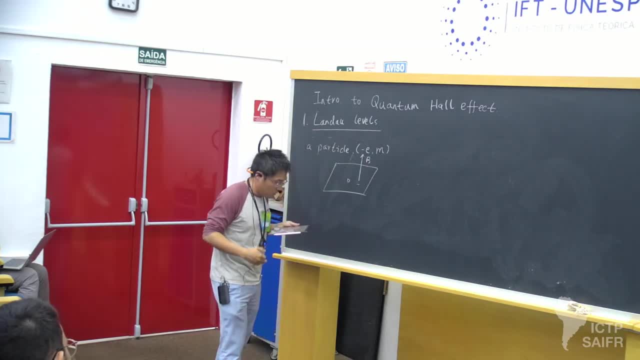 levels and what's the physics of Landau, levels for this and probably next lectures. And that's really the the important starting point to understand both integer quantal effect and fractional quantal effect. Okay, So we know, you probably 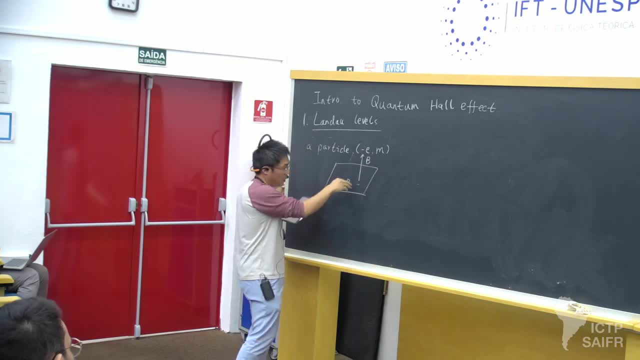 know that the, the, the particles, the electrons will couple with the electric, the magnetic field through the so-called minimal coupling, And what you need to do is that you you need to introduce a vector potential that I will call the A. 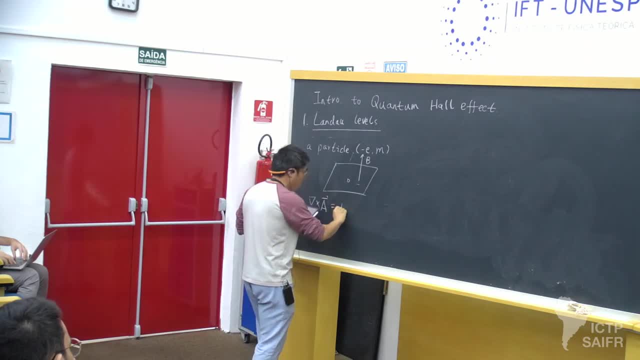 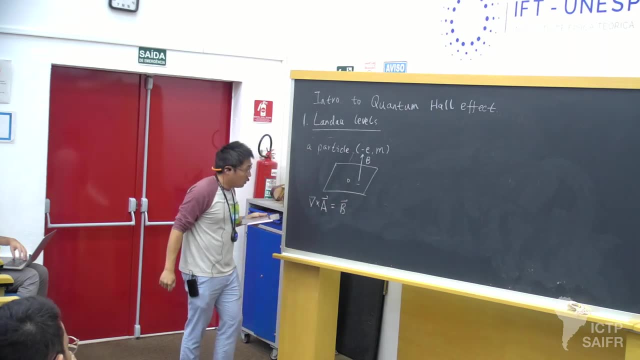 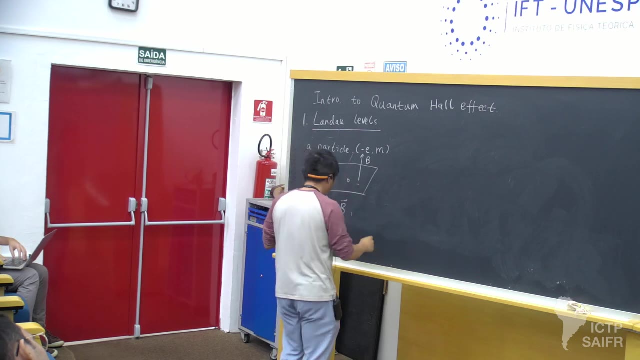 which, which. this is a potential for the, for the magnetic field, right. And then we know that the you can write down the, the, the single particle Lagrangian for these electrons, which will be just my. 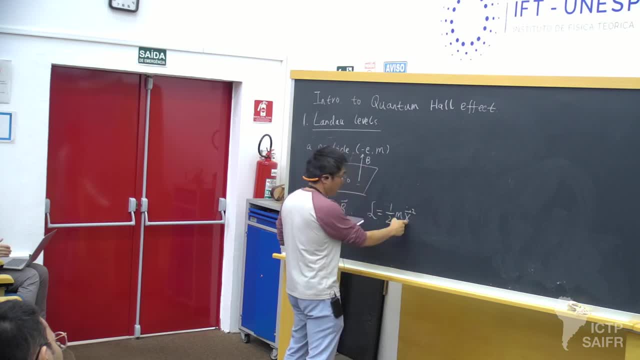 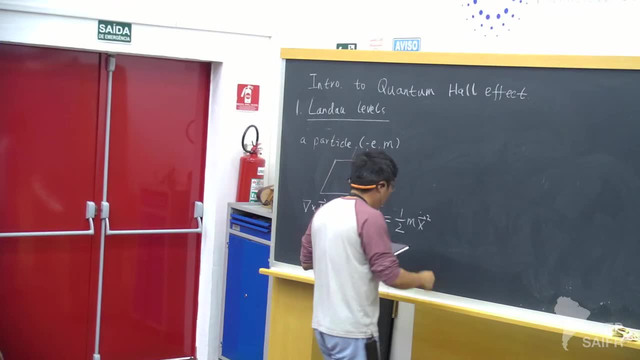 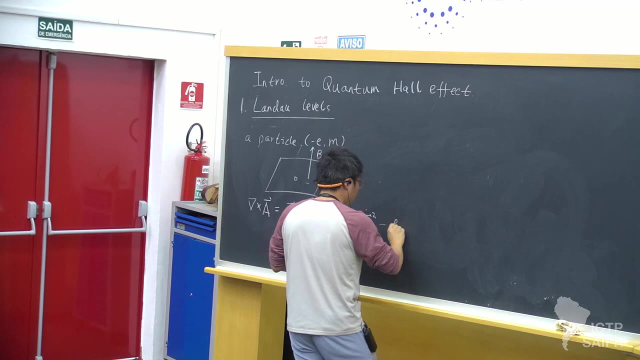 ordinary kinetic energy that I. I'm using X to represent the, the positions of my electrons, and X dot, and this is really just conventional kin kinetic energy And I do have a minimal coupling. that is my velocity of the system of the. 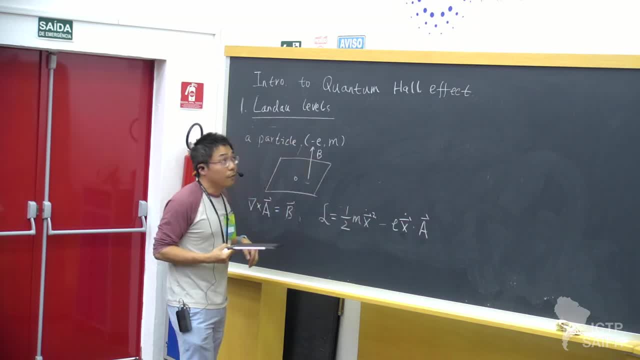 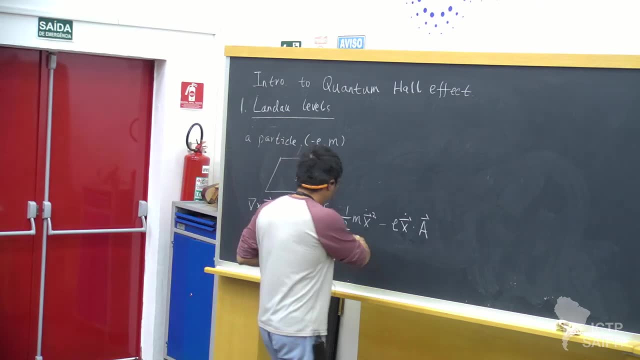 electrons coupled to the vector potential. Right, If? if that's the first time for you to say this, you can. you can convince yourself by showing that from this Lagrangian, what you can do is that you can compute its equation of motion. 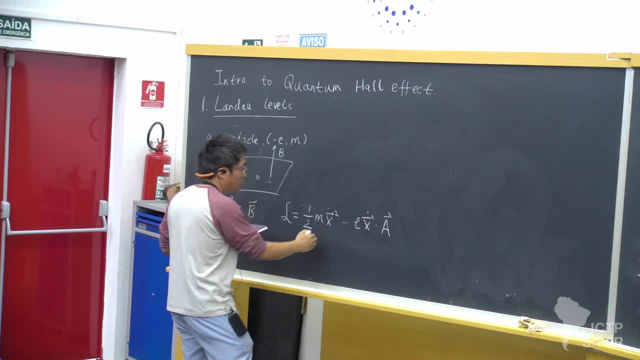 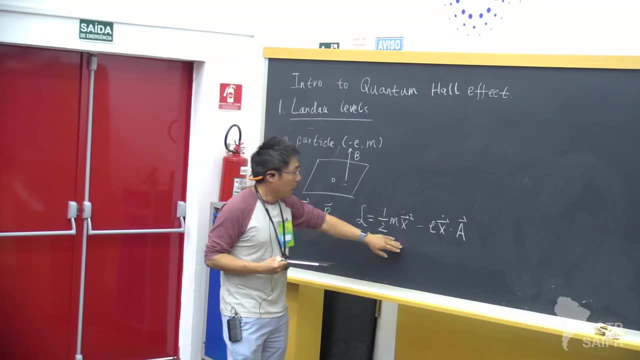 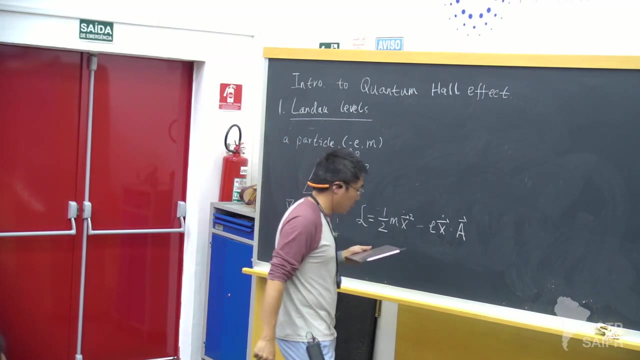 right, And then you can show that the equation of motion of this Lagrangian is: give you exactly the Reynolds force. That's how you end up with this Lagrangian describing the electrons moving in a in a two-dimensional 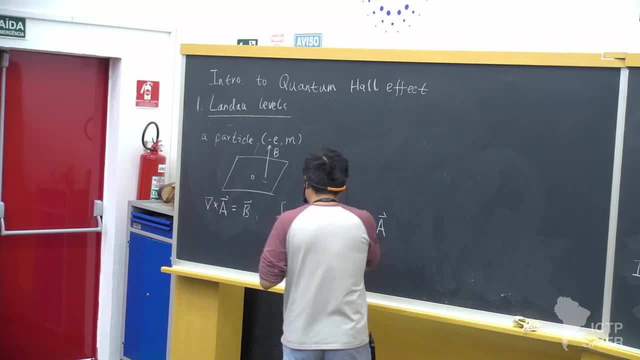 plan. Okay. So, and with this Lagrangian, what we can do is that, for example, we can compute the canonical momentum that I will call P, and just I should- no, I should use, let me just use. 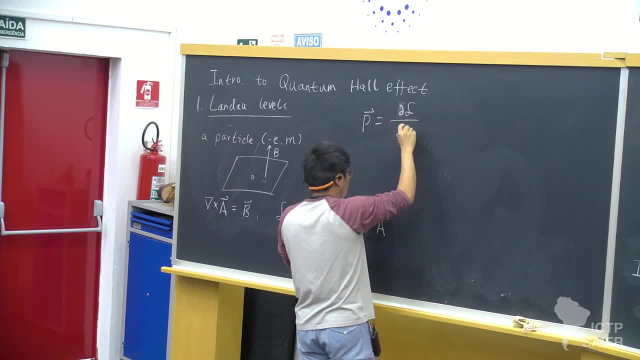 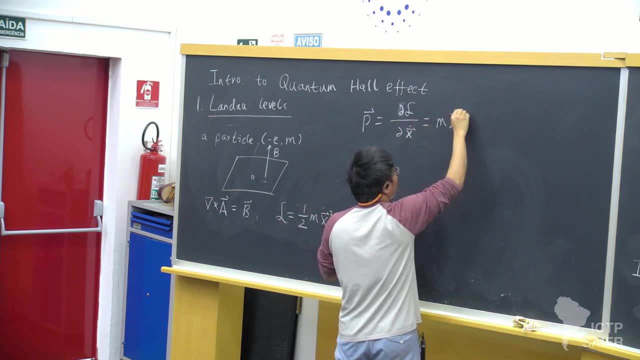 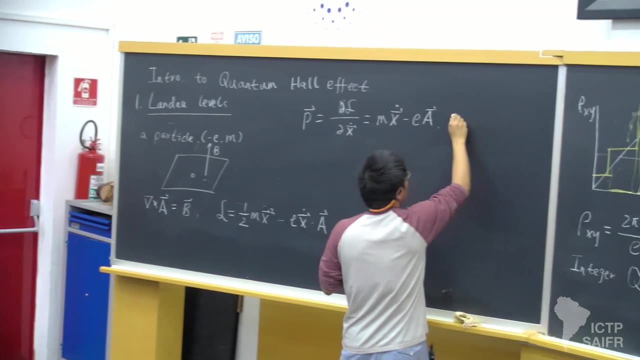 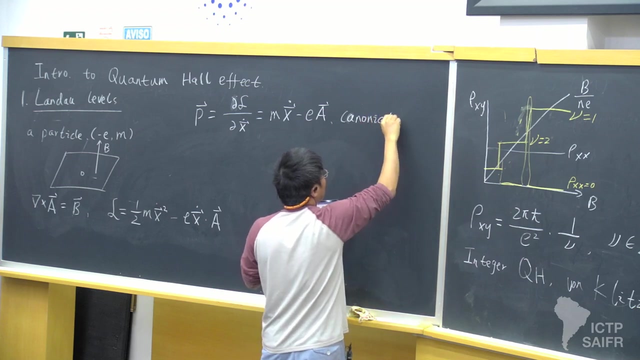 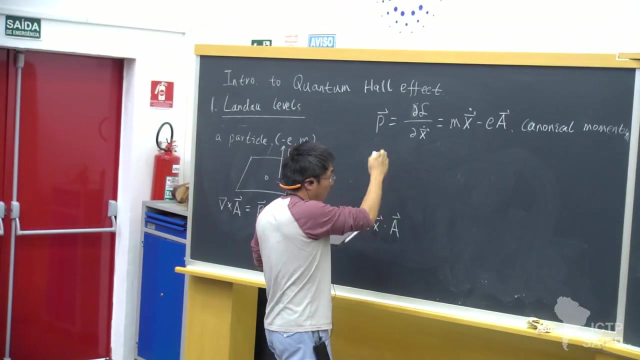 partial. We can define the canonical momentum which turns out to be this, and I call it canonical momentum And that's the observable that has this and it can this relation right, And one thing you can say is that this canonical 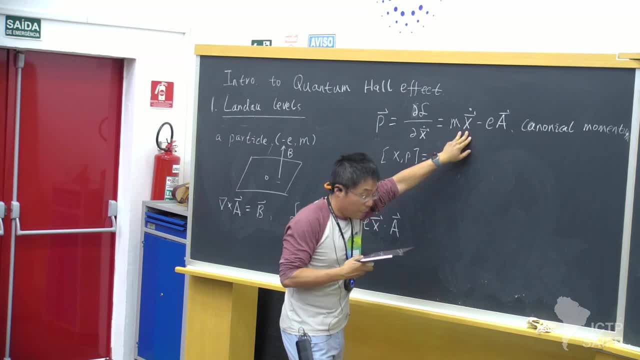 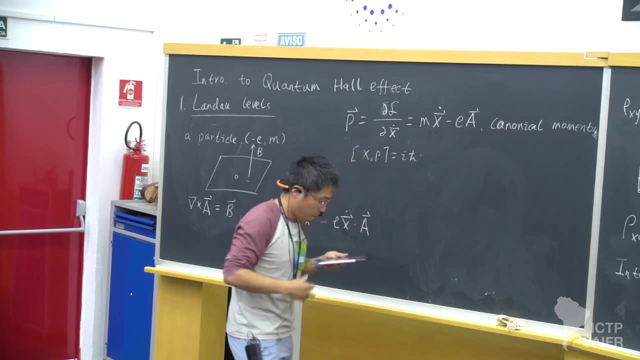 momentum is now becomes gauge, non-invariant, right, Because it has this vector, potential term. Okay, And I can define a mechanical momentum, right, The mechanical momentum is really, and then that is like this and: 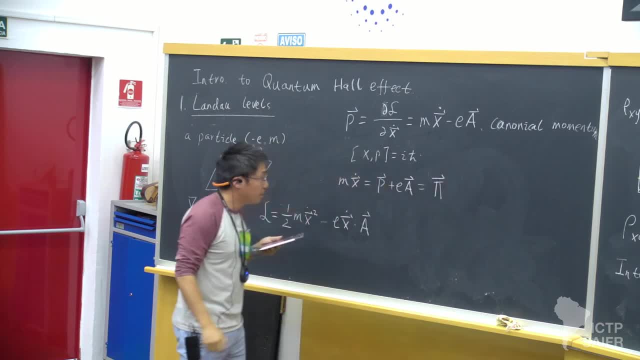 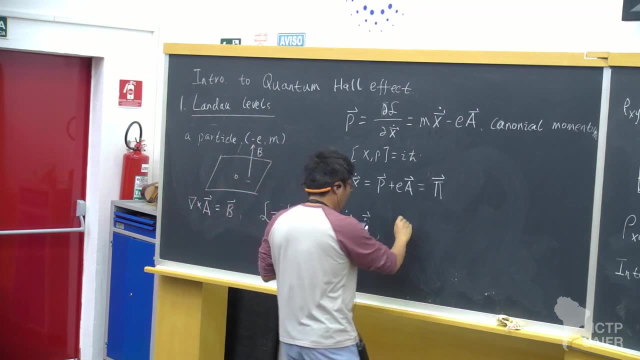 throughout this lecture, I will call it pi, And then, with this Lagrangian, what I can do is that I can write down the Hamiltonian right, And that's the Hamiltonian- is what we want to deal with. 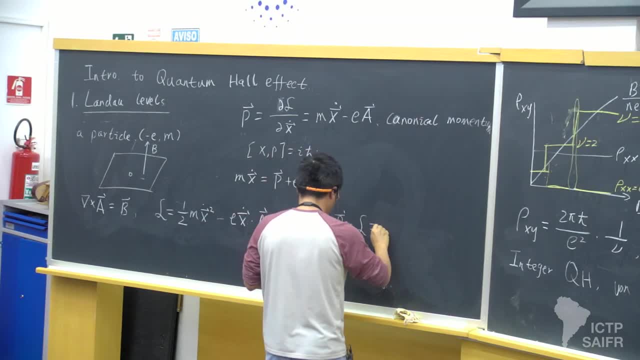 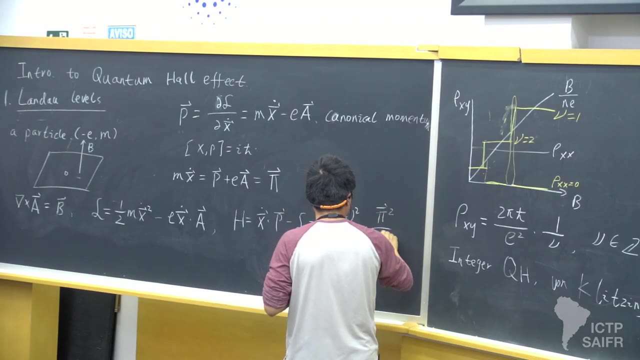 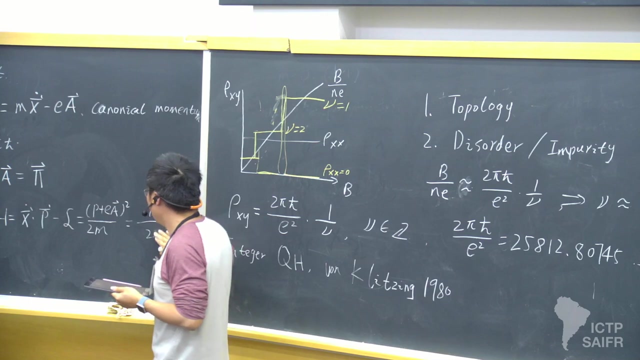 In this quantum mechanical problem, And you can write it as, indeed, as the, using the, the mechanical momentum, right? It's really just something we're familiar with, right? The energy is relative to momentum, so this formula that 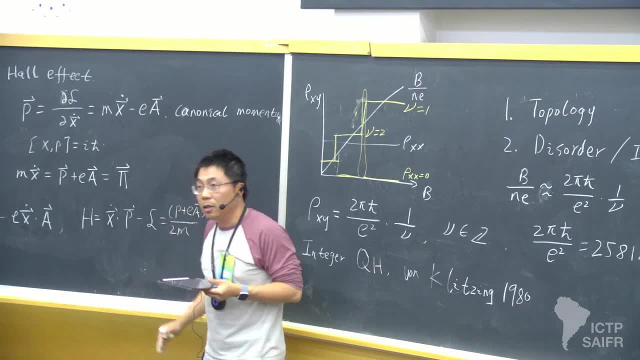 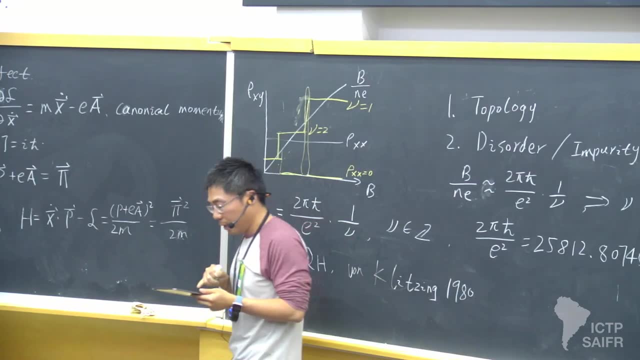 we learned in high school. right, That is the Hamiltonian of this, of this system. right, The Hamiltonian of two-dimensional electrons moving in the presence of a magnetic field. Okay, So now we want to solve this single-particle. 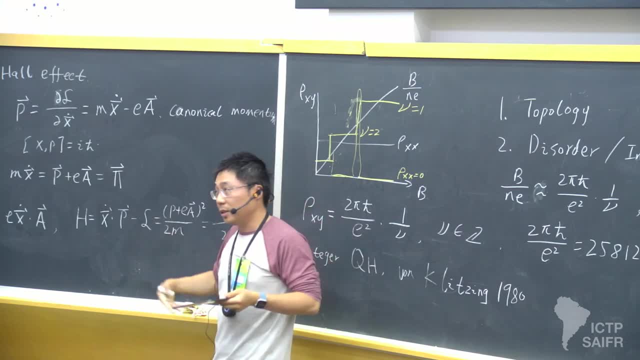 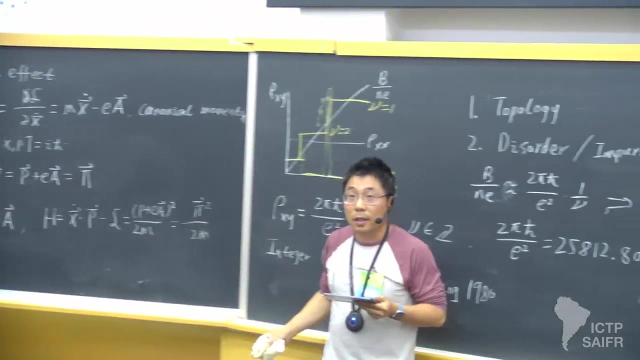 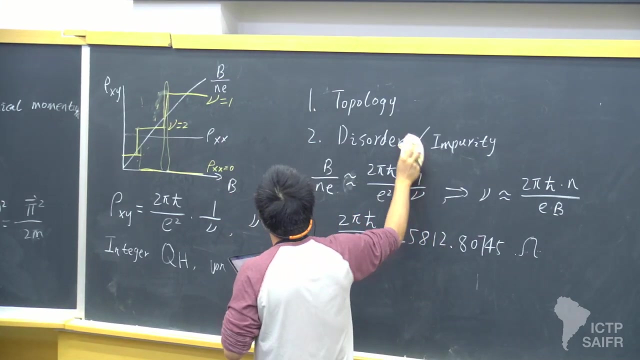 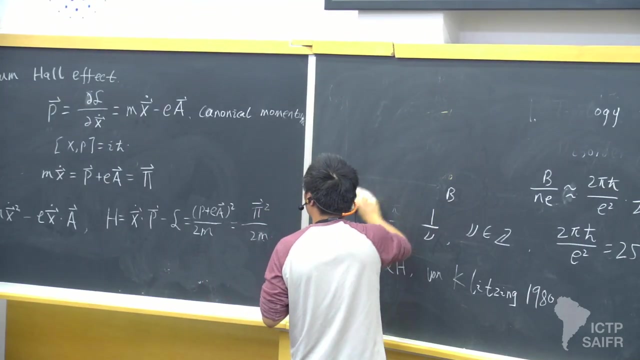 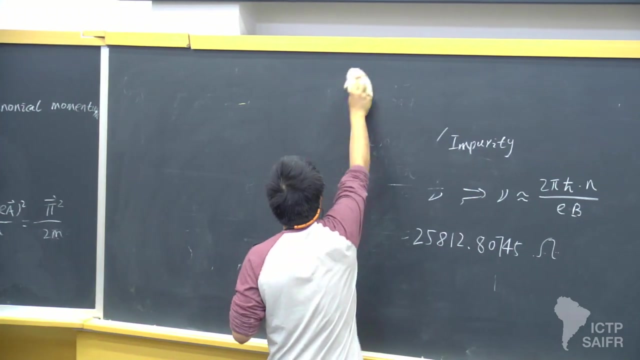 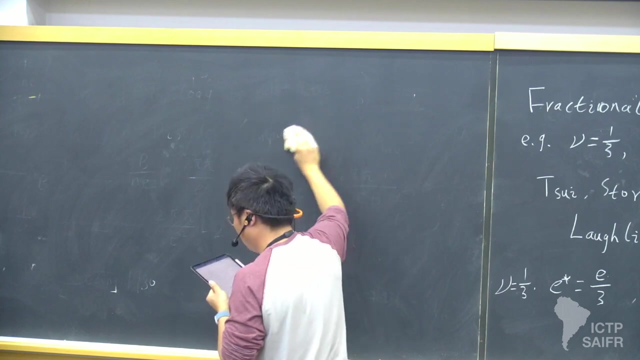 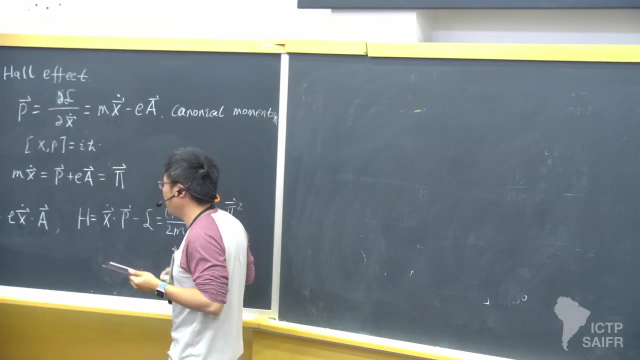 problem to to say what's its eigenstates look like and what does the eigenenergy look like, And its eigenstate is what we called. there is one of three eigenstates in the real world, in real world. Okay, the first thing that we can do, which turns out to be pretty simple, is just to 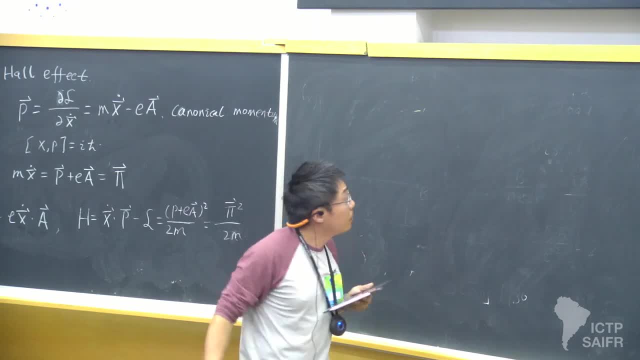 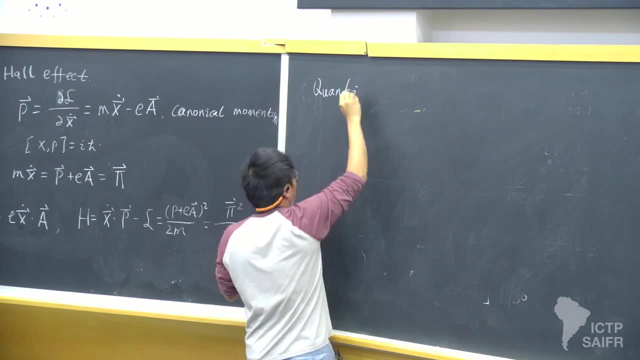 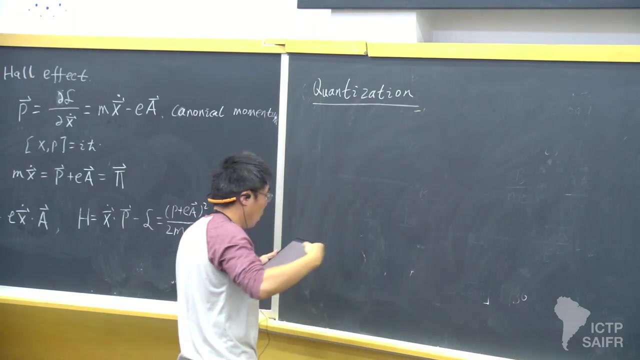 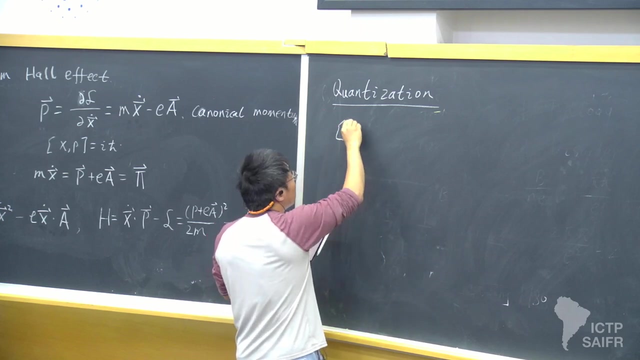 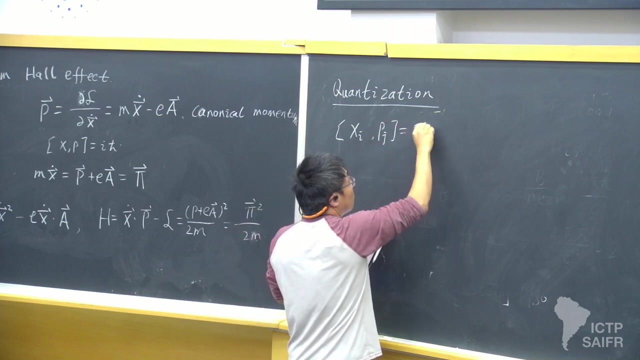 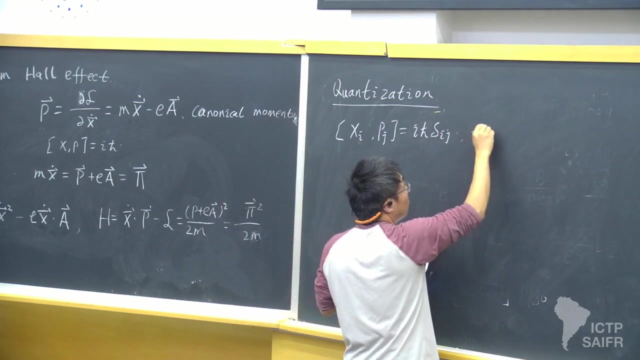 compute the eigenenergies of this Hamiltonian. So we can call it, and you will soon see that the eigenenergies of this Hamiltonian is actually quantized. So let's start with this canonical quantization. Now I'm putting indices into this, commutators, this- i and j are really just taking values. 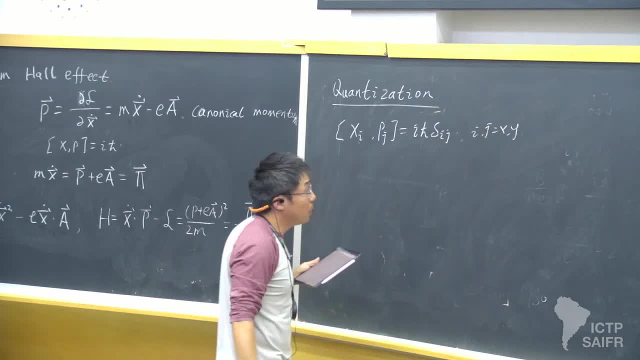 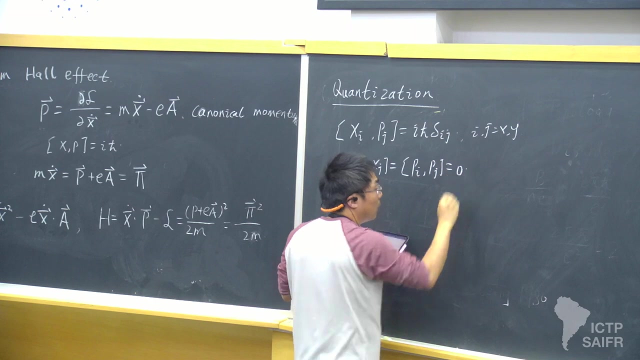 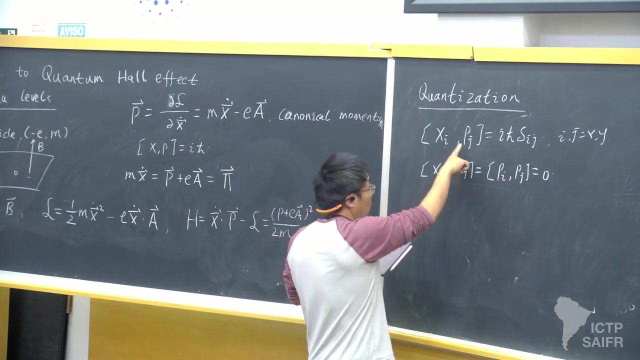 between x and y, or 1, 2,, if you prefer. And we also know that the coordinates, as well as the momentum, are commuting between themselves. That's quantum mechanics that we learned. So now, what do you? yeah, again, what you know is that you can rewrite this canonical. 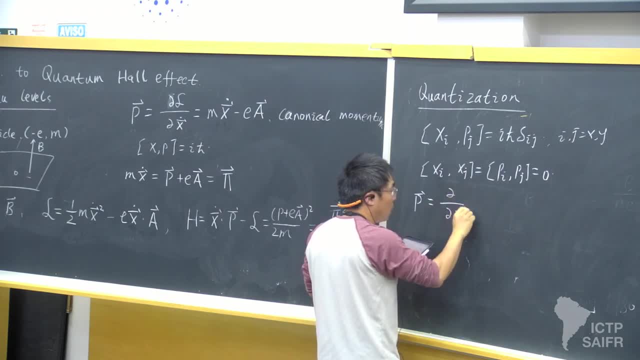 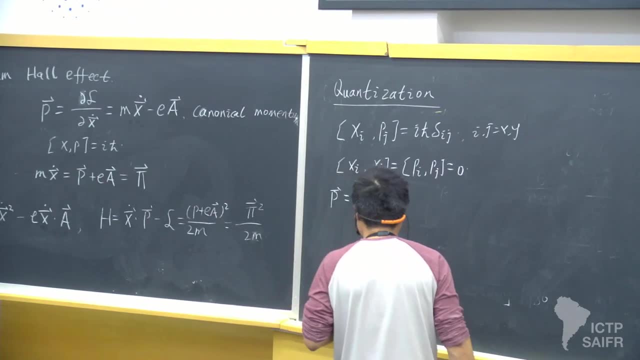 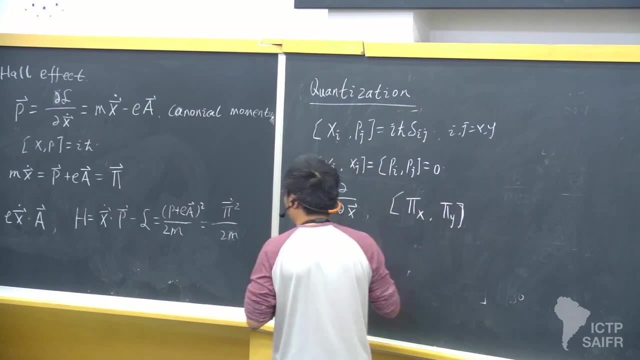 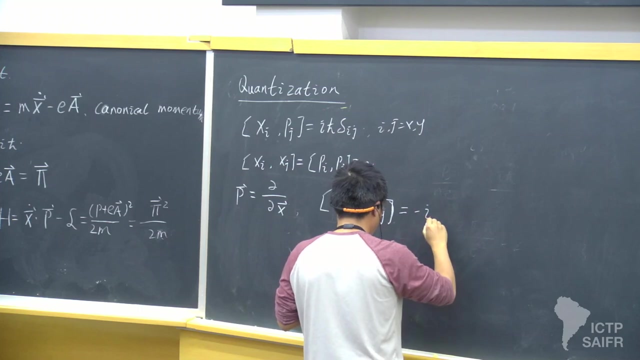 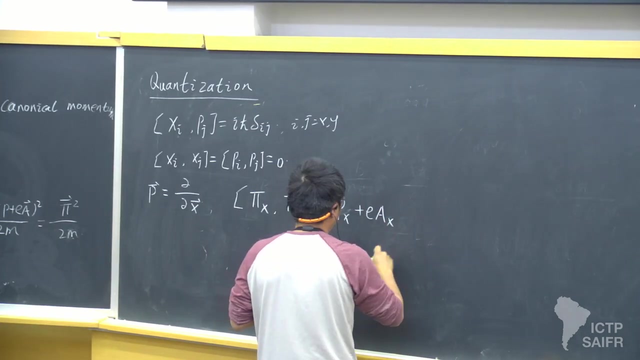 momentum, just as the derivative of my coordinates. Now what do you can show is that now the mechanical momentum, the pi that I defined here, will satisfy the commutation reaction. that is so that may be more concrete. You just rewrite your mechanical momentum as p plus e. 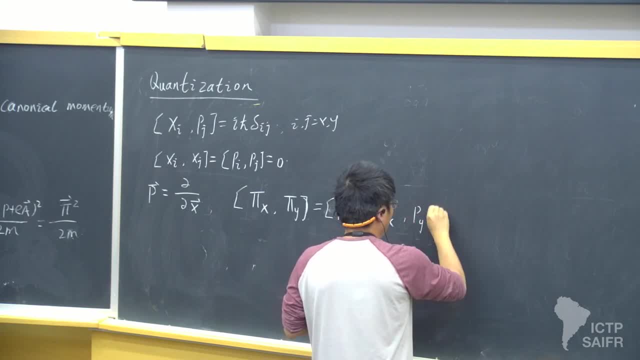 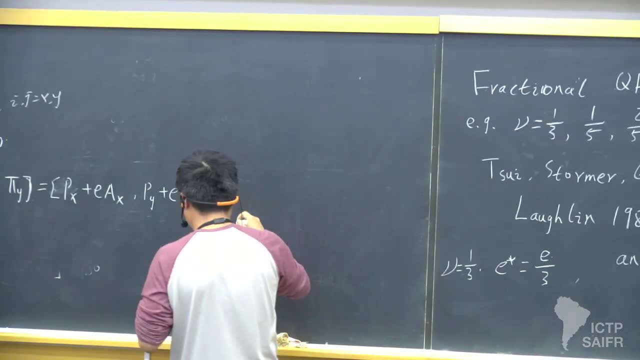 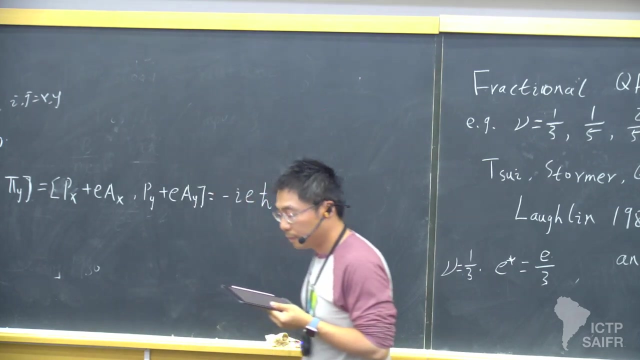 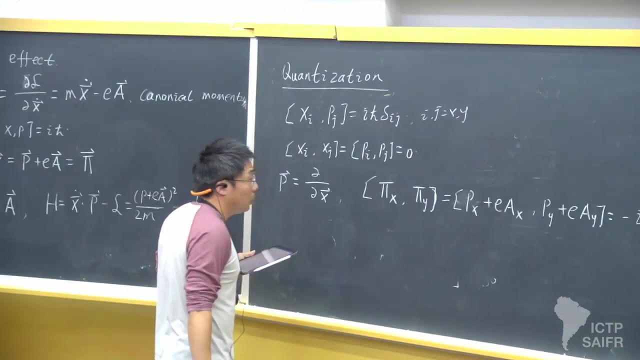 And 1, 2.. That's the commutationals. Okay, and you can show that this commutation relation to be minus i times e, h, bar times magnetic field, right? So, and then what you can do is you can define. 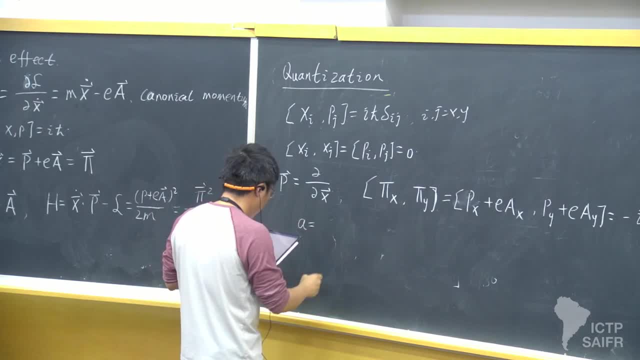 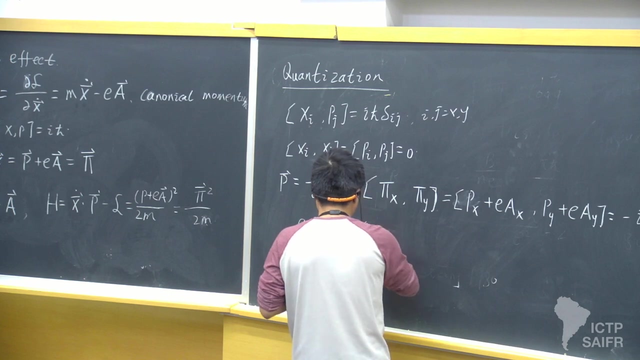 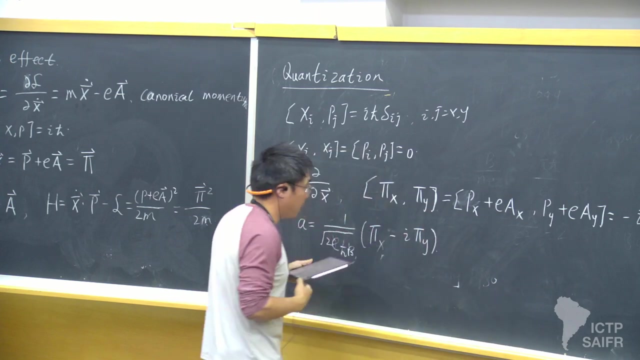 an operator that I call the a, which is the. I defined it as one over root of two e times h, bar times the magnetic b, and then I use the canonical, a mechanical momentum to define such an operator, and naturally I will have ad. 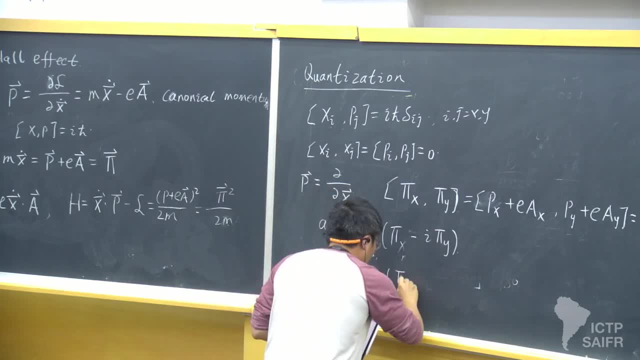 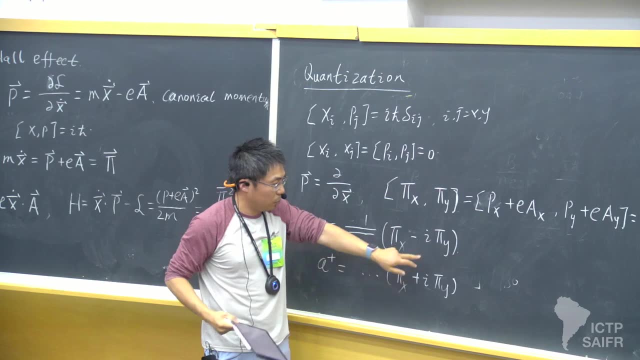 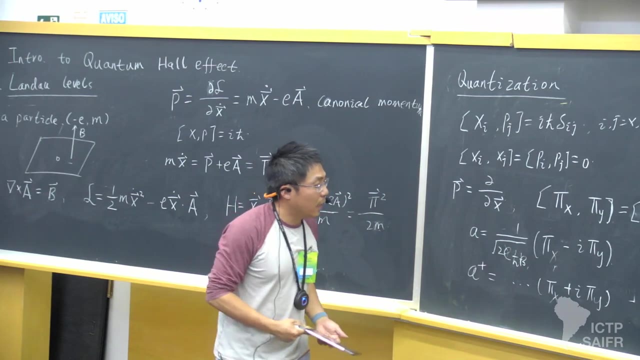 dagger to be some similar, to have a similar expression, but with a different sign. for this, due to the yeah, I'm conjugating i, So I get. I define those operators. and the reason that I want to define those operators is that, on the one hand, you can show that 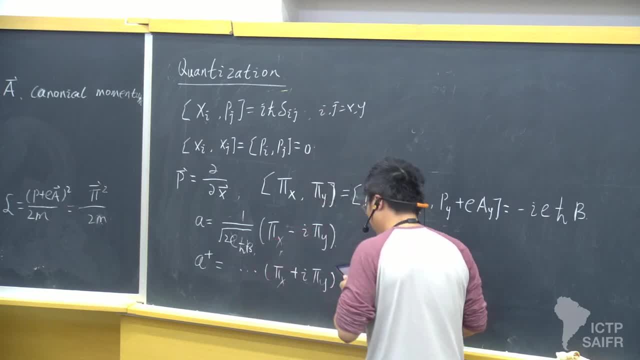 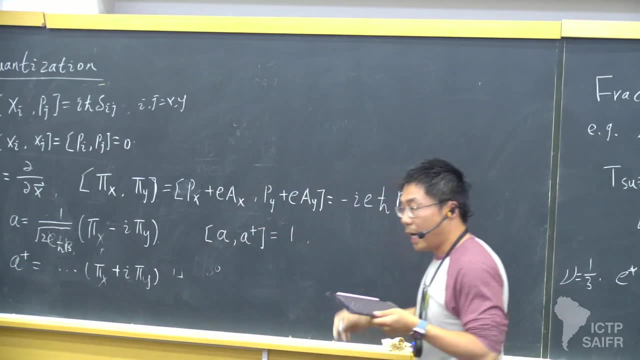 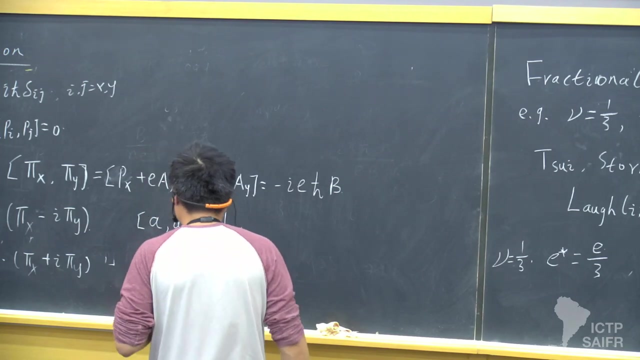 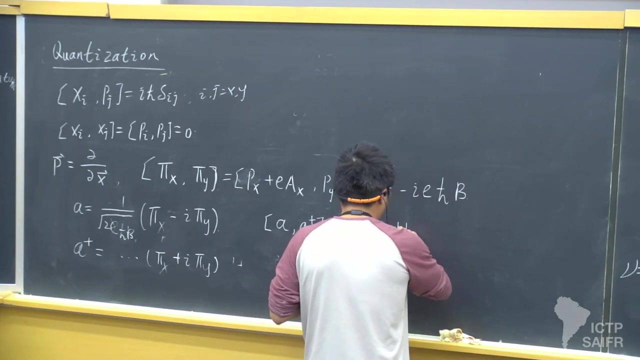 the commutation relation between a and a dagger are, now just becomes one. yeah, And that's the commutation relation of creation and annihilation operator that we also use to study the harmonic oscillator right And more importantly, what we have is the. 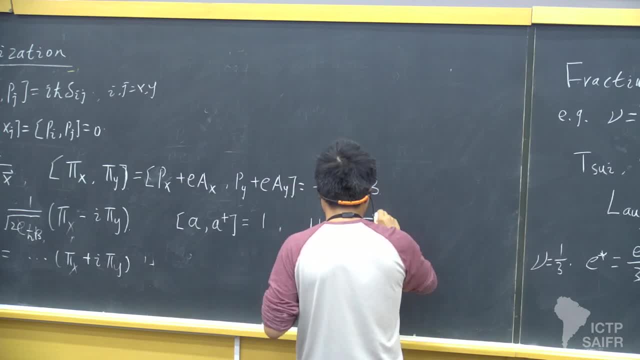 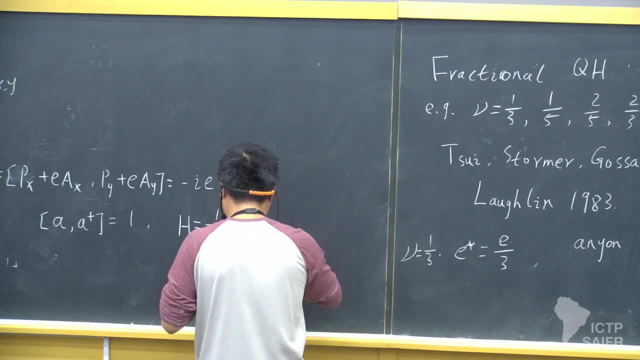 for the Hamiltonian, which is the square of the mechanical momentum, and that's what we're going to use to solve this problem. So what we're going to do is we're going to solve this problem with some one or two lines computation. 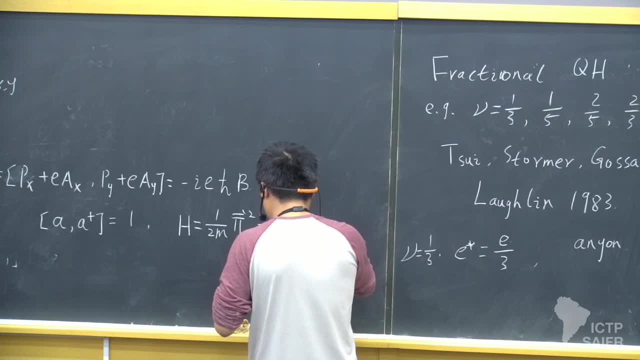 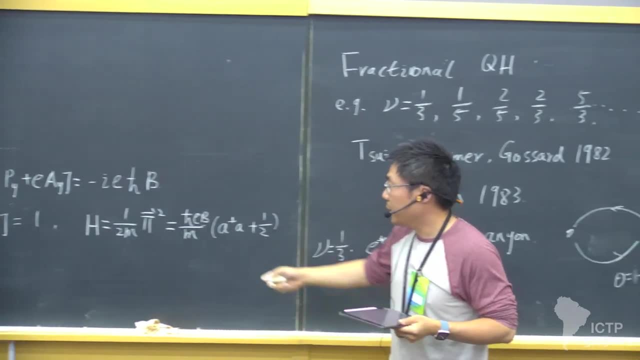 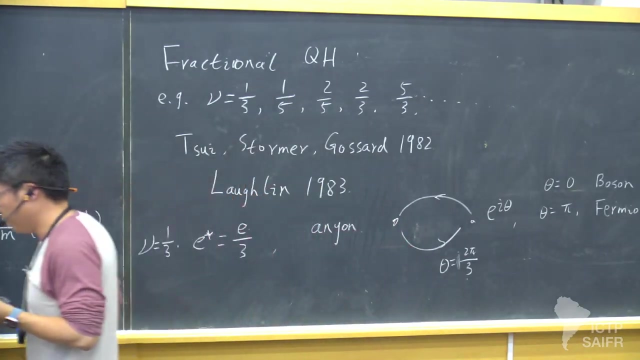 You will realize that it's actually close to h bar times e, times b over m and times a dagger a plus one half right. That's really just an expression that we also encountered when you solve in the harmonic oscillator using those creation and annihilation operator. 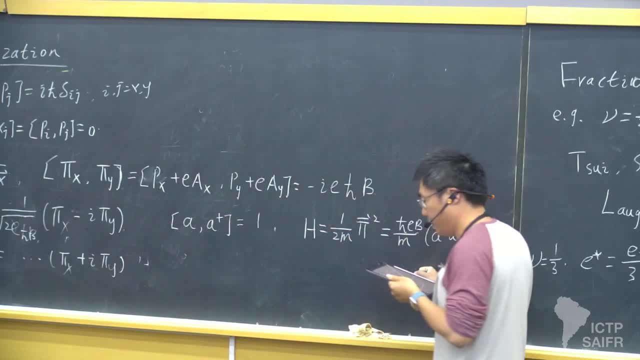 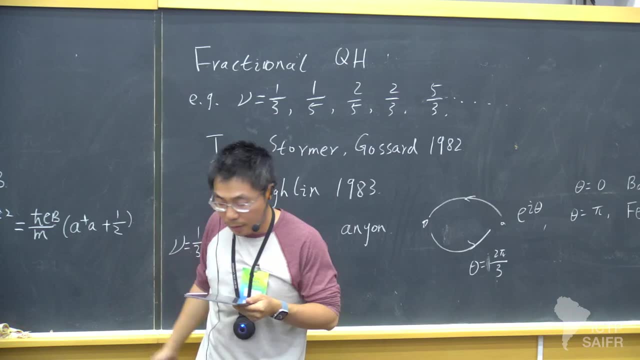 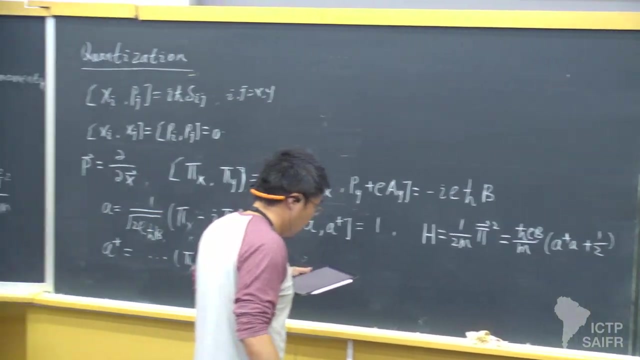 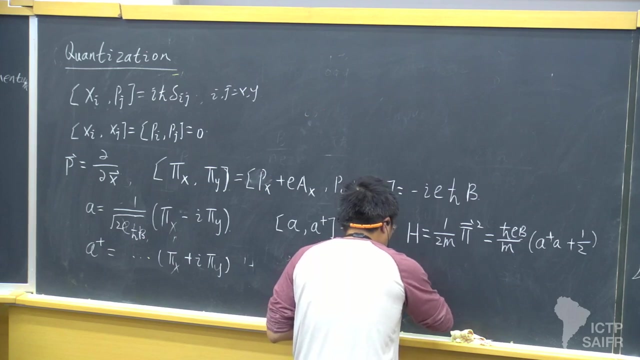 And now we immediately would know that, what are the eigen energies of this Hamiltonian, which will then be, just be quantized, quantized right, Just like a harmonic oscillator right, And here I will define one quantity, that is what we called cyclotron frequency. 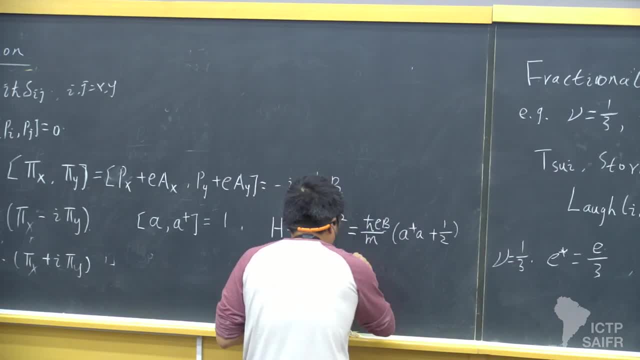 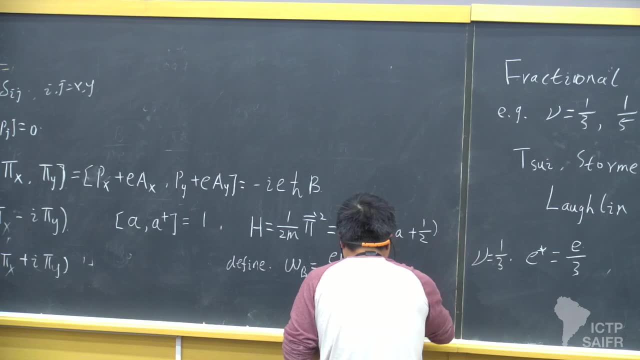 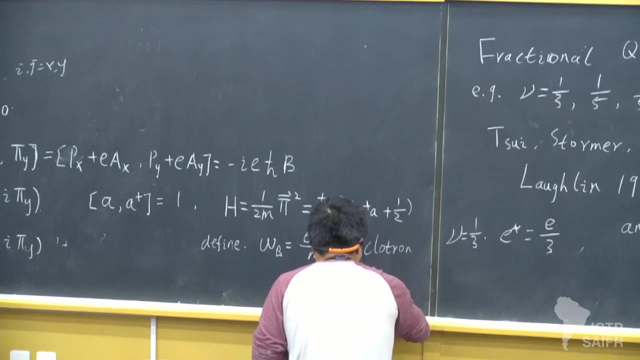 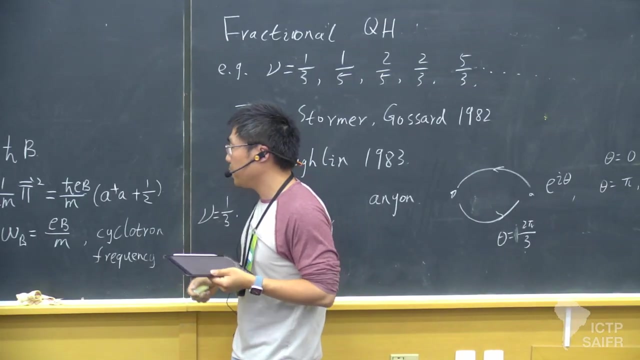 it's- I will call it omega b, which is e times b over m, and it's called- let me also write it down- called cyclotron frequency, And this is a, that is, an energy scale that we will enter many times when you want to consider. 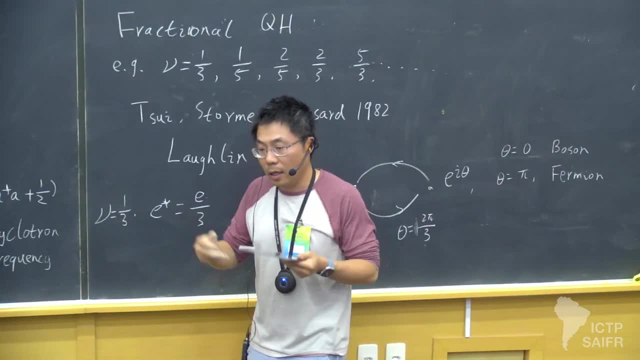 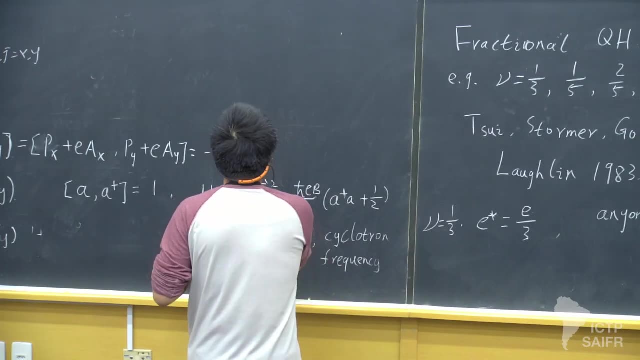 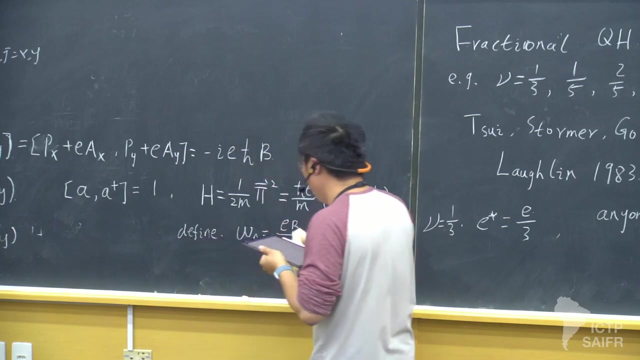 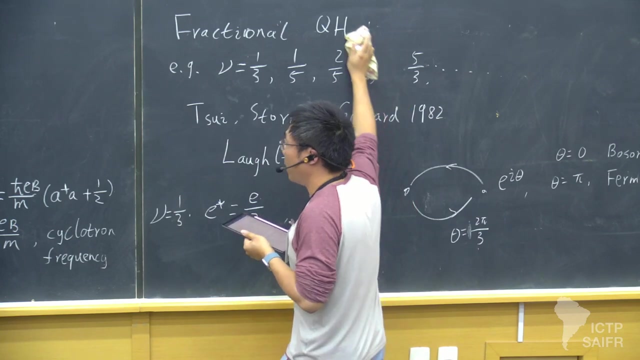 quantum Hall physics and, more generally, the physics involving a magnetic field and electrons. Okay, so we can. now we can solve this. So let me, as I said, it's immediately clear that the energy levels of this single particle Hamiltonian. 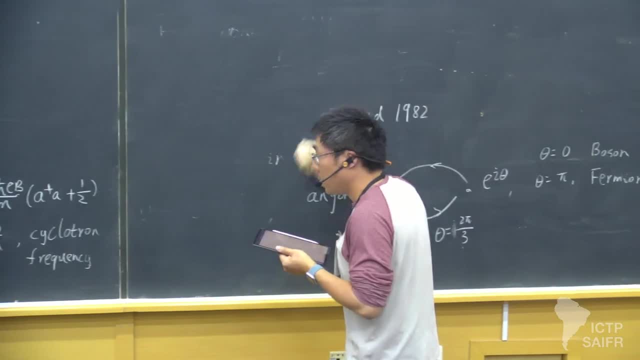 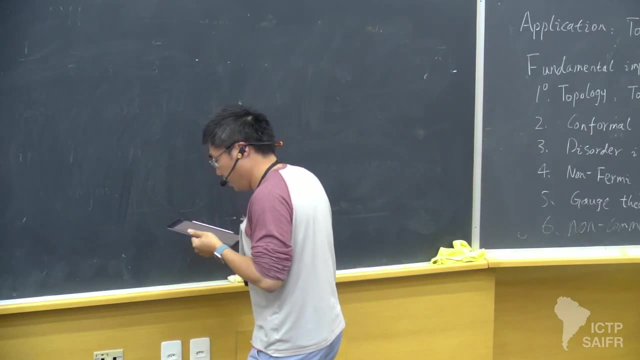 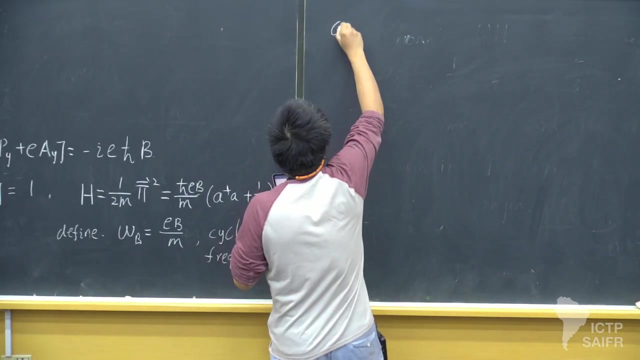 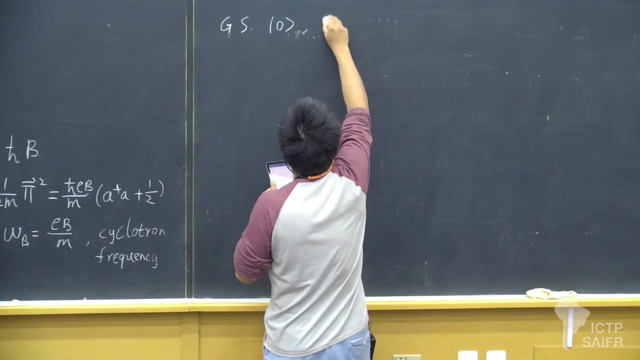 will be quantized And we can write down its energy levels, right, Just like what we have for the harmonic oscillator, right? We can first start with the ground state that I call it zero, and it satisfies the relation that if I apply the annihilation operator a to ground state, 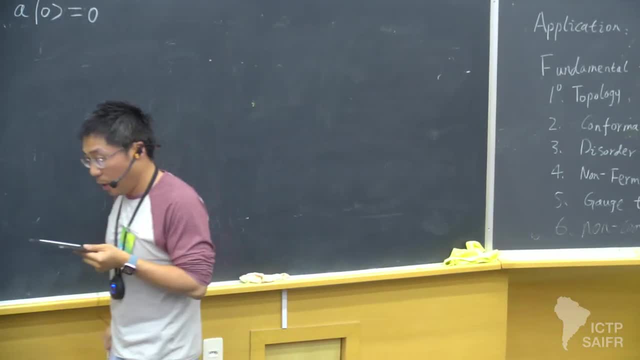 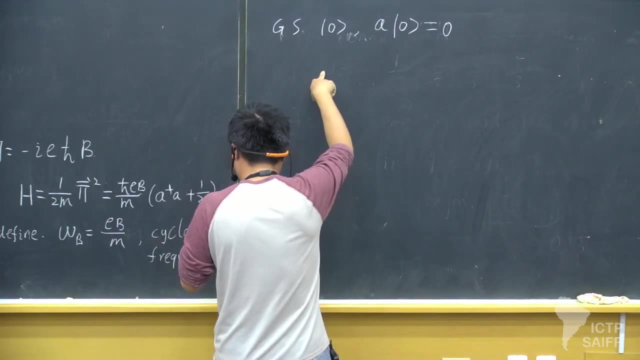 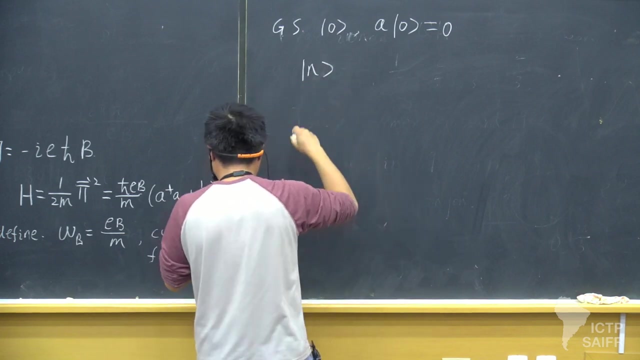 I will just get zero, right, That's just okay. so that's just a harmonic oscillator, right, And then we can define the state that we call. we can label at n. don't confuse this n with the charge carrier that I also talked about. 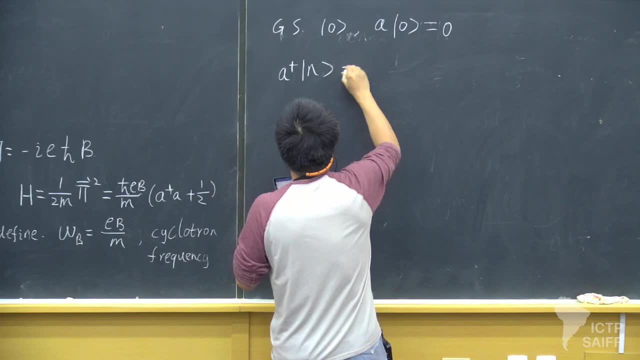 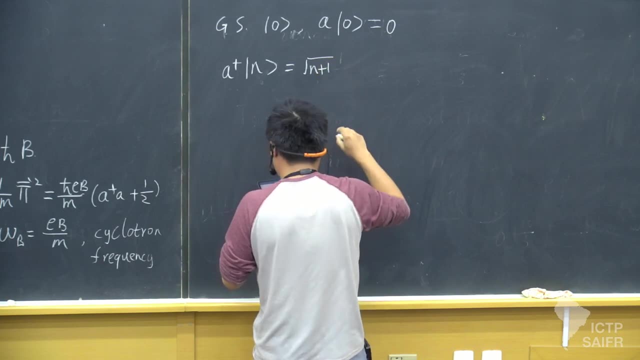 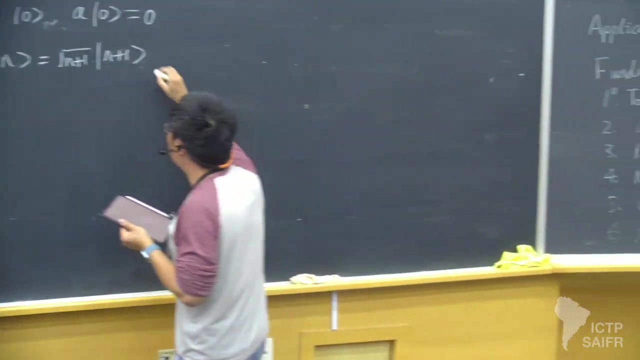 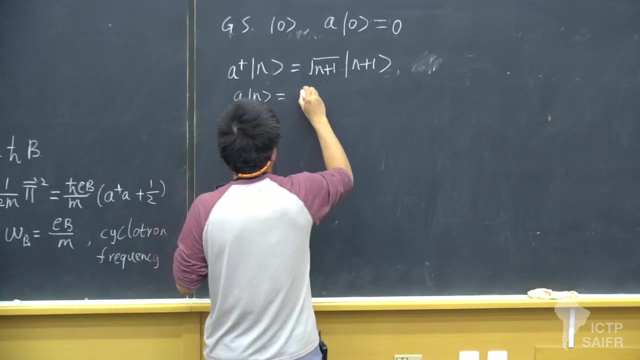 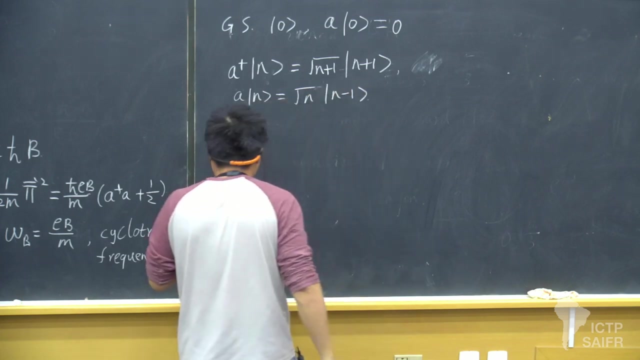 So if I I can define this n state and if I apply a creation operator on top of it to it, then I will increase this n by a number one. And similarly, if I apply annihilation, I will get- yeah, and you will know that, the energies 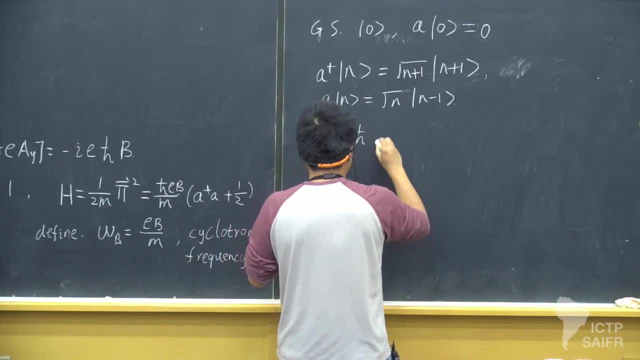 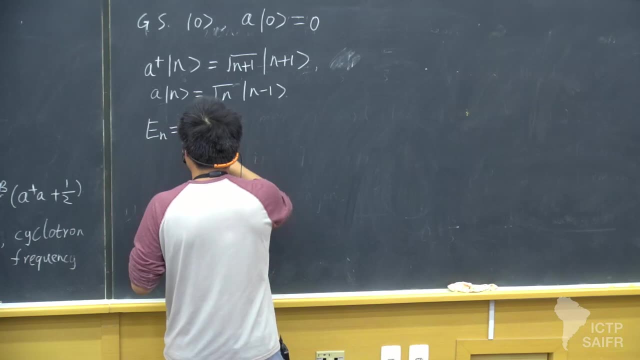 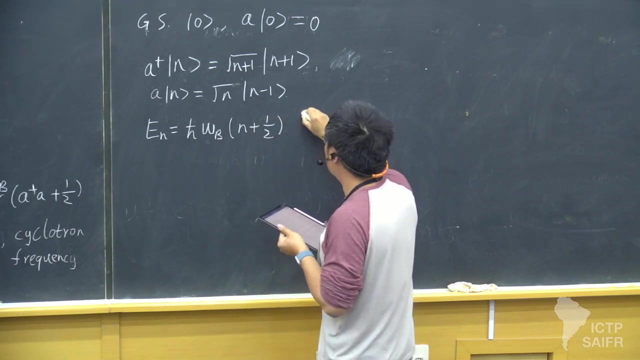 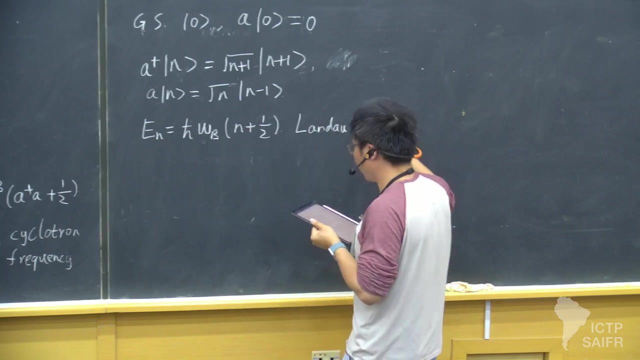 of those of each state will be this: omega b is really just the cycle channel frequency and it's h bar omega b times n plus one half right, And this is what we called lambda levels energy, lambda levels right, And that's how we get the eigen energies. 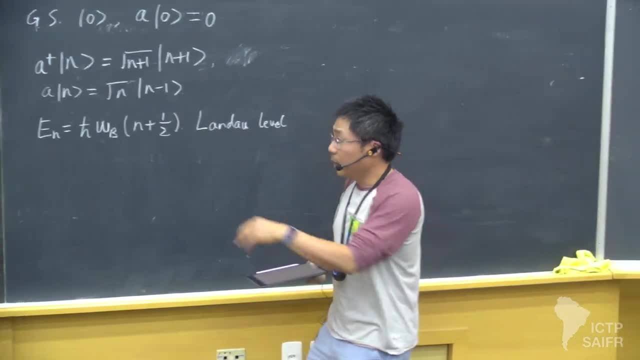 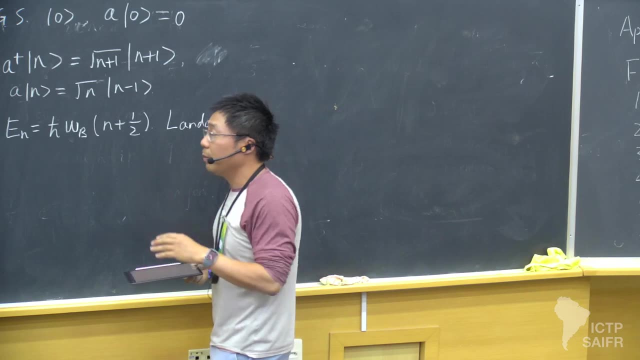 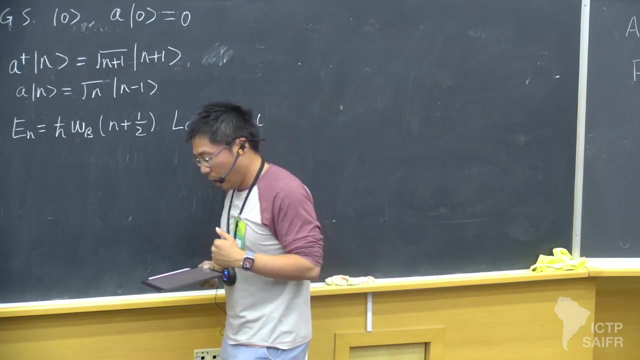 of that Hamiltonian right And you can say that the version is really very straightforward. I would suggest you, if you it's the first time for you to say this, I would suggest you to repeat the computations for both and also for what I would talk about later. 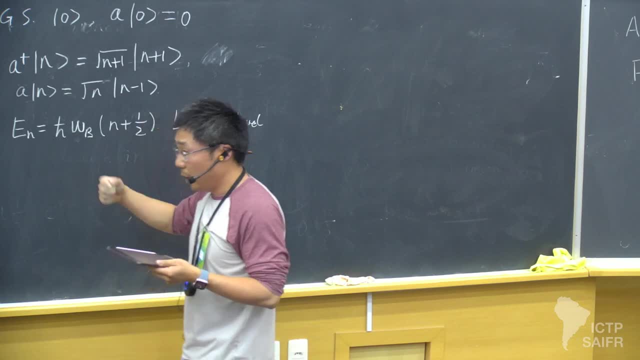 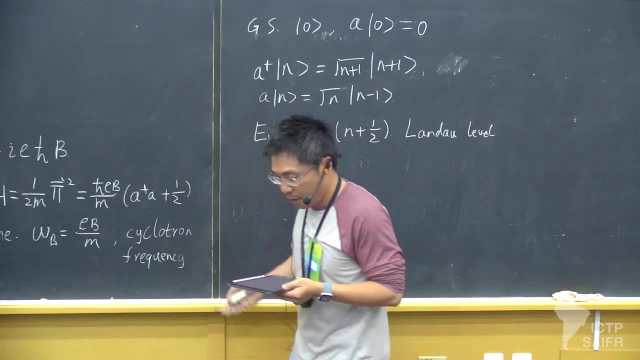 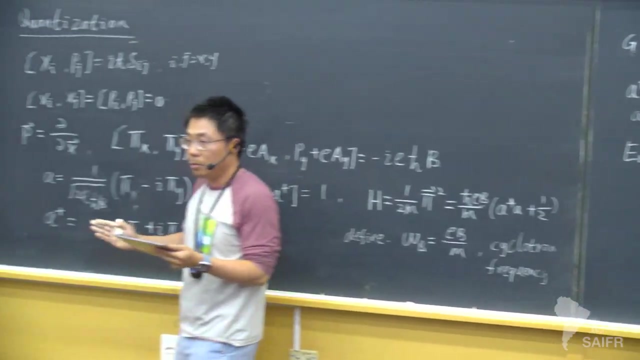 It will be very helpful to understand this basic physics. Okay So, but now you may realize that we actually miss one thing, right? So the problem that we start with is actually a two-dimensional problem, right? It has two degree of freedom- x and y- for its position. 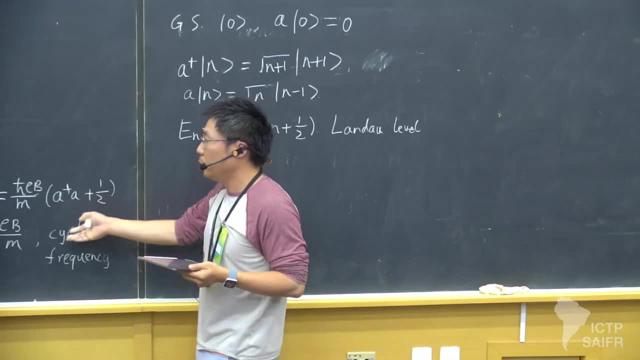 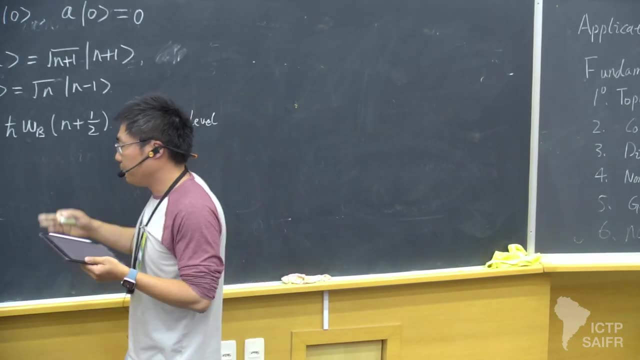 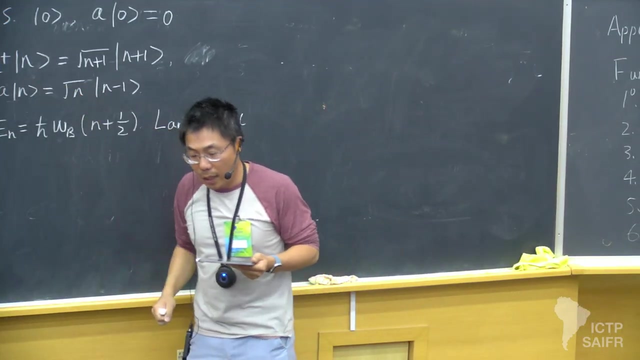 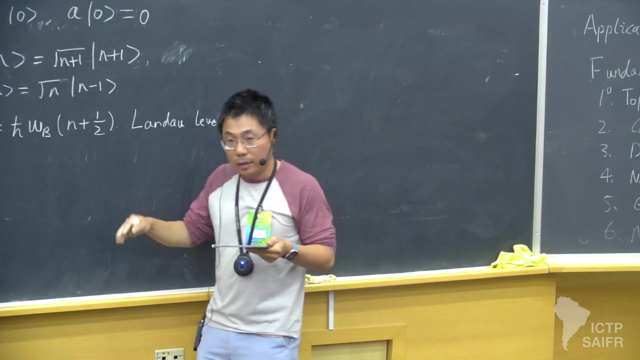 right. But now I convert it to some creation and annihilation operator and then I end up just mapping it to the harmonic oscillator, which seems only I have one degree of freedom, that is, that is I denote as this n state. So it seems there's one degree of freedom missing, right. 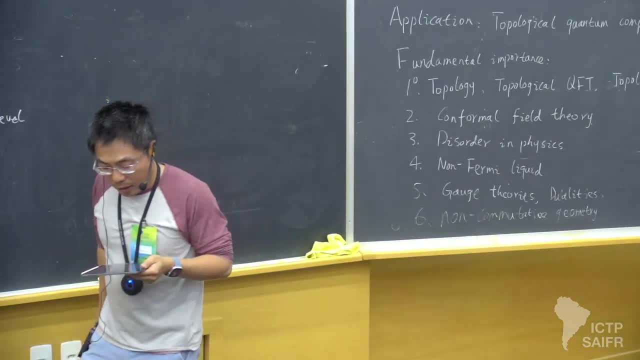 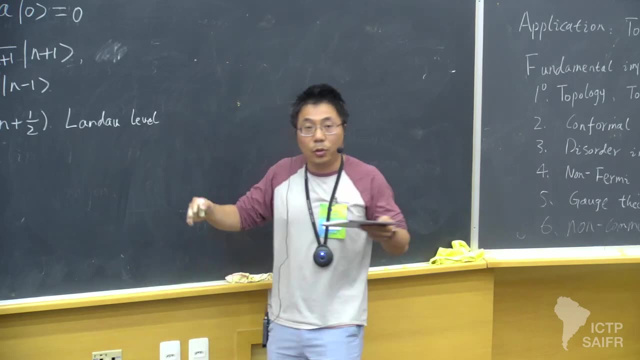 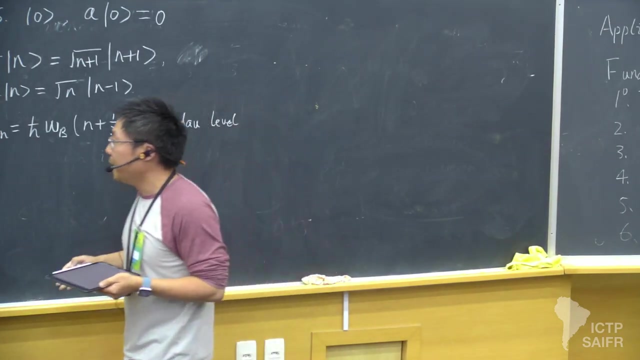 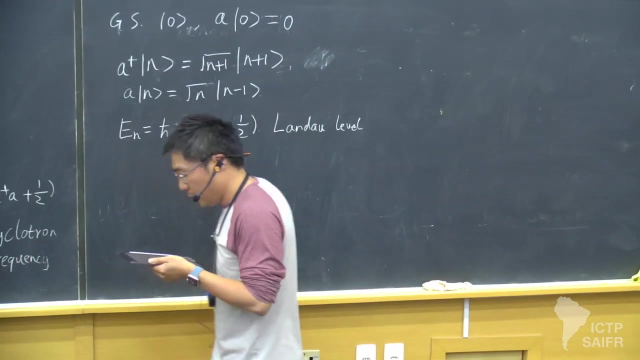 And the solution out of this contradiction is that actually for each levels, for each lambda levels, it has a huge degeneracy right. That's the other degree of freedom will correspond to. It may not be immediately clear that how to understand that degeneracy just using this second quantized language. 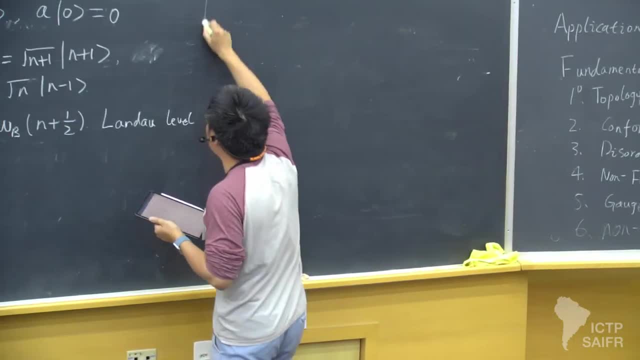 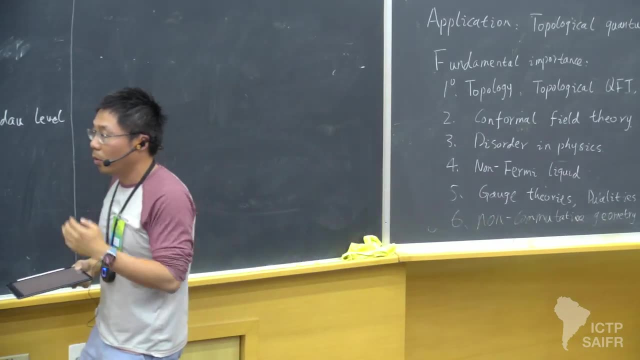 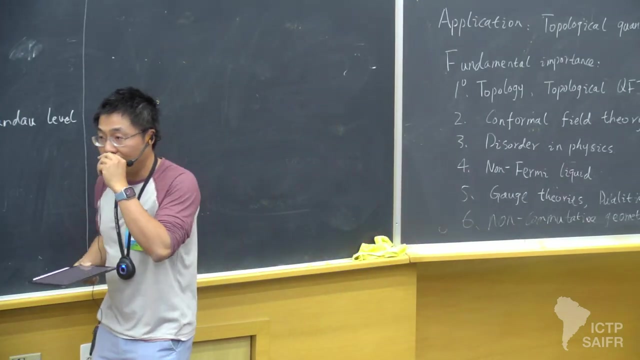 So it will be helpful to understand that We should do to study this problem in a more tedious way. That is, we want to try to solve that shortening equations corresponding to that Hamiltonian to get its wave functions to have better physical understanding. 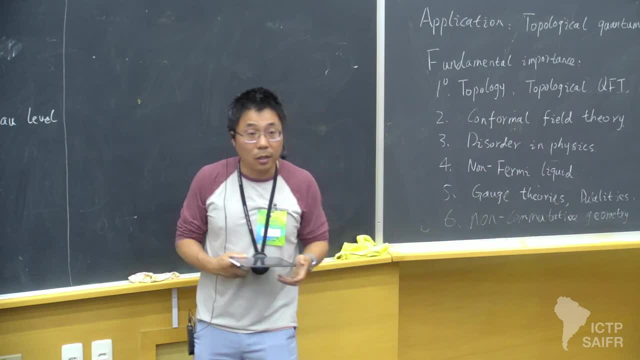 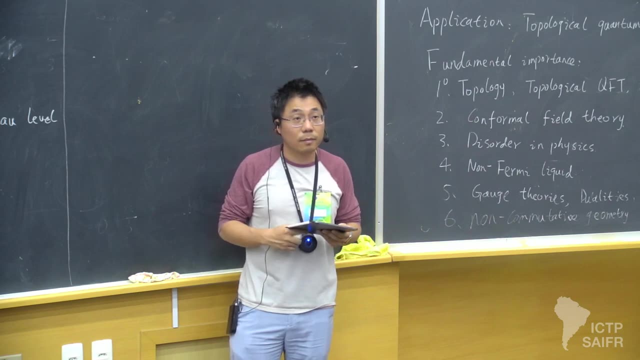 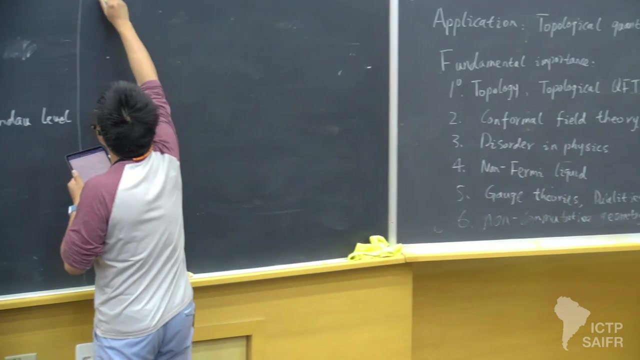 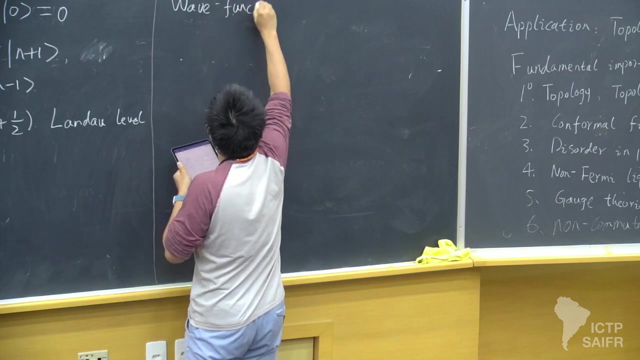 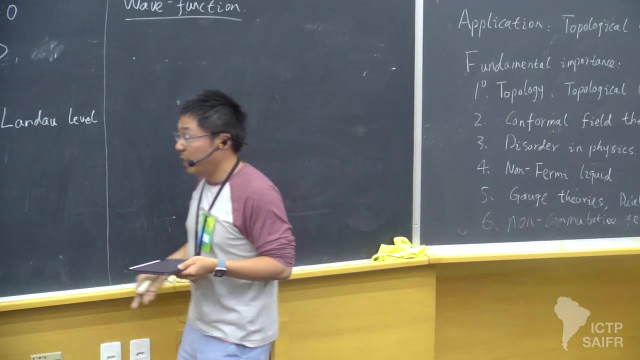 about the physics of lambda levels, So I can pause a little bit for questions. All right, so now let's think about the wave functions right of those state. So again, we want to solve that Hamiltonian that I wrote there. 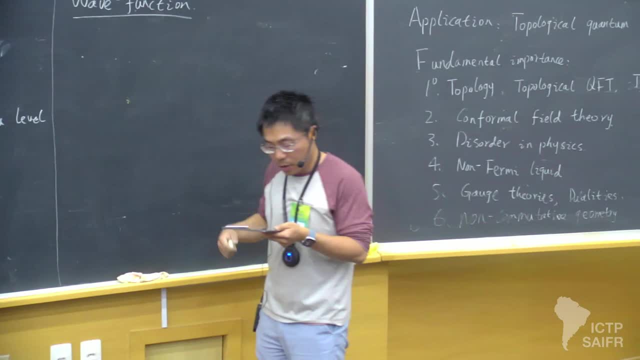 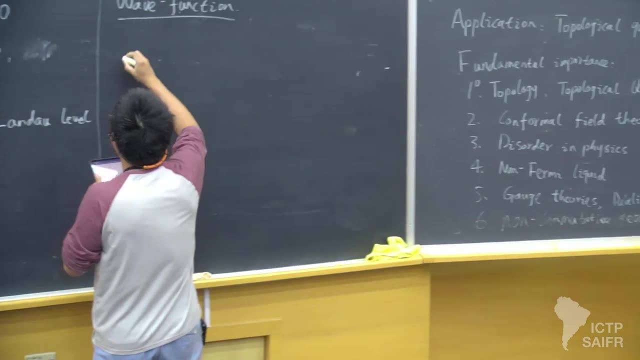 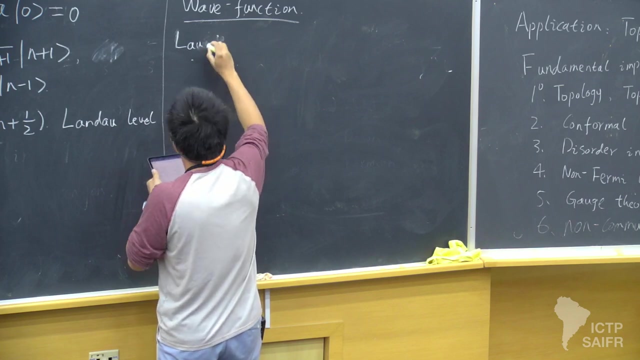 And, as you know, yeah, first we. as you may know, the first thing that we need to do is that we need to choose a gauge, right? So I would first choose the so-called Langdahl gauge. Let me pronounce it. 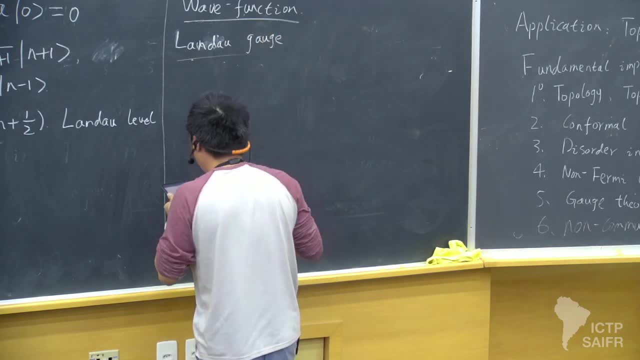 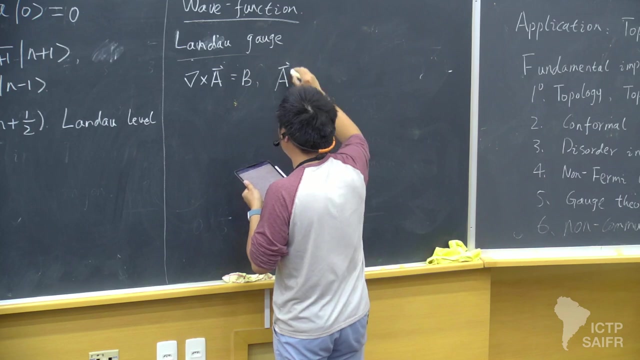 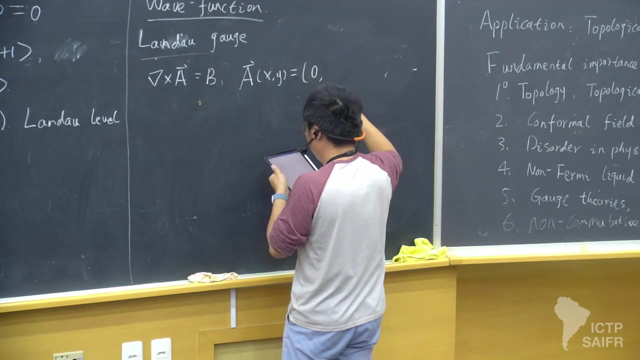 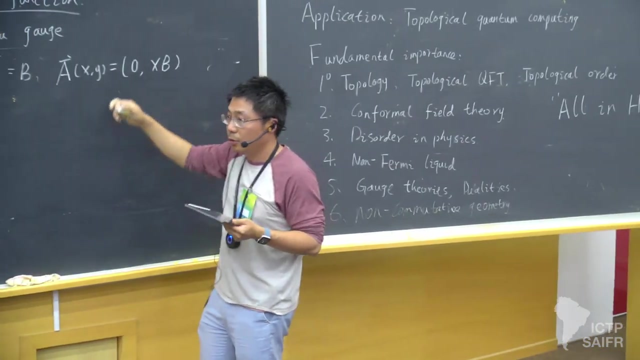 So remember that I do have the there's. my vector potential is defined in this way. So then what I can do is that I can choose a specific gauge that has my- that is what we usually called Langdahl gauges. So it's like the vector potential is zero in the X direction. 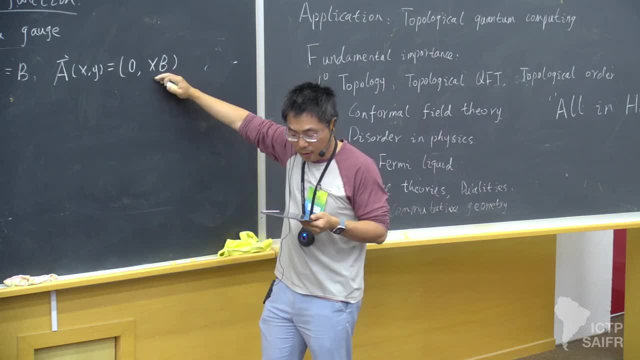 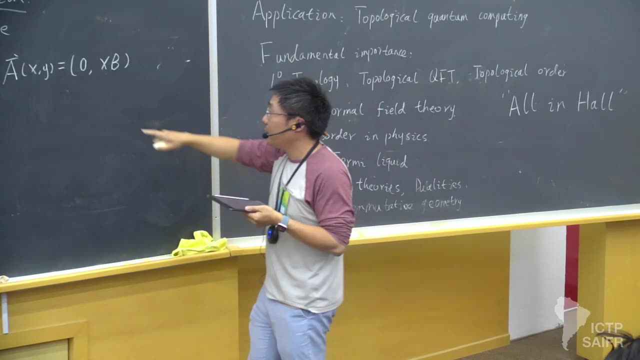 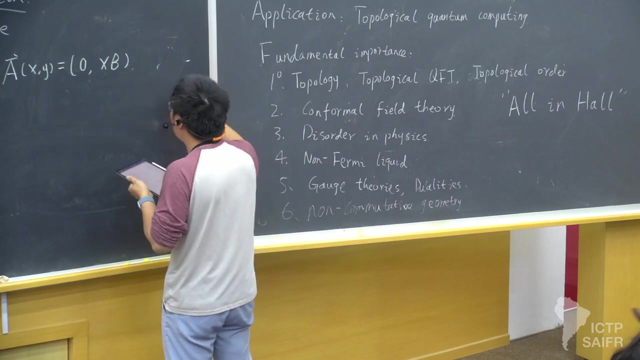 and it's non-zero only in the Y direction, And the value of this actually depends on X, right? So one thing you can immediately see is that this Langdahl gauge actually preserves the translation Along. let me see along the Y direction, right? 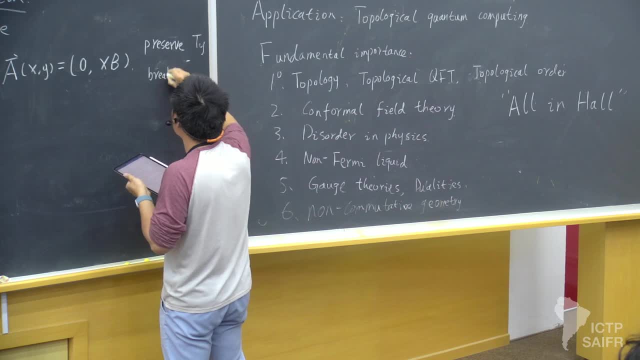 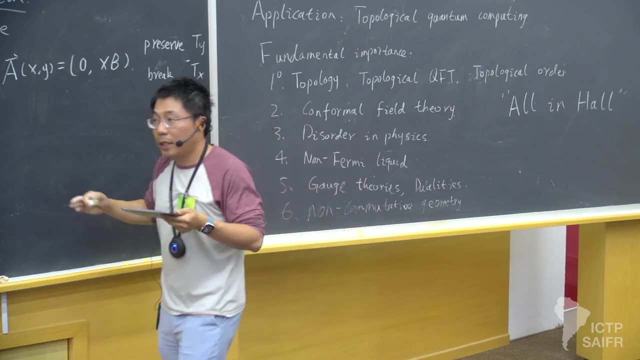 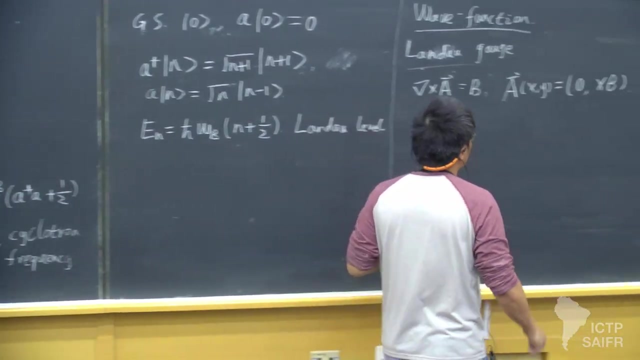 But it's break the translation in the X direction. That is the that the price we have to pay when we choose a concrete gauge. Okay, So now, what we can do, okay, is we can simply write the value of a gauge. 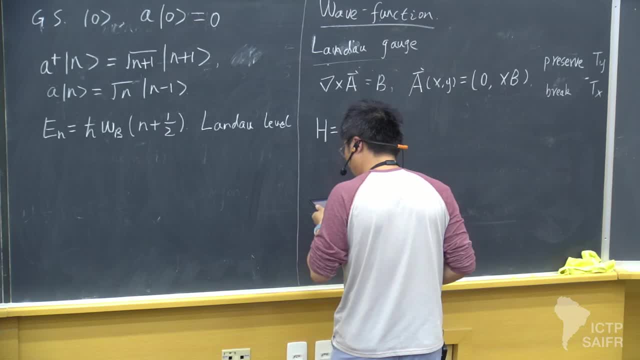 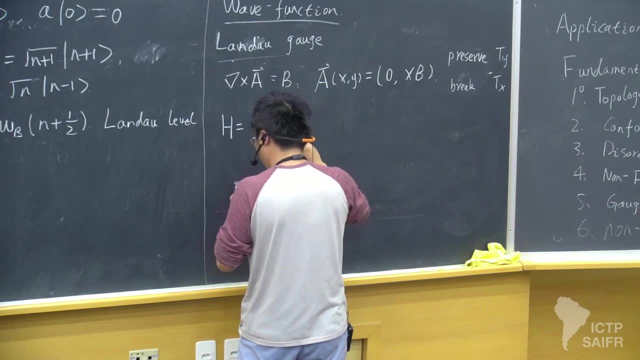 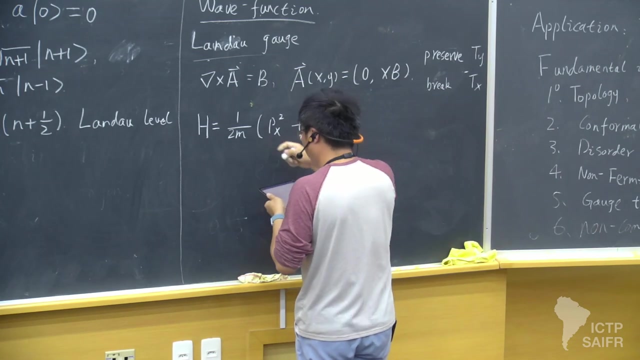 That's all that we need. If we don't write the value of a gauge, the price we have to pay for a gauge, Okay do is that we just rewrite our Hamiltonian using this gauge, which is 1 over 2m and times my px squared, and also because the vector potential I 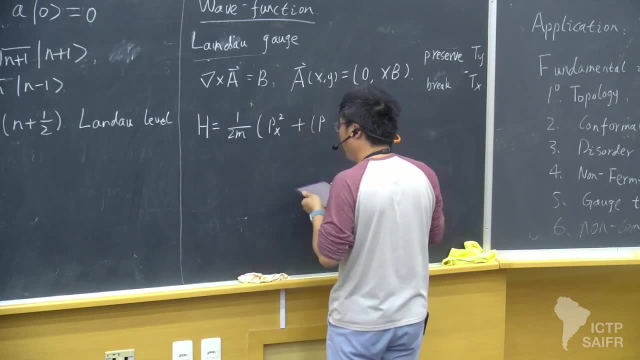 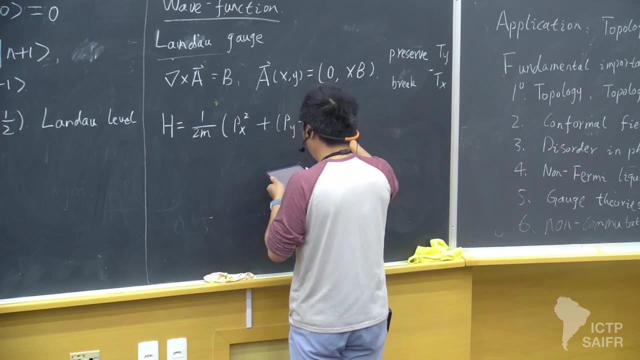 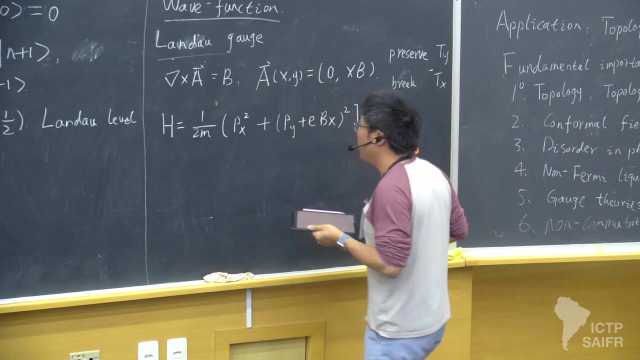 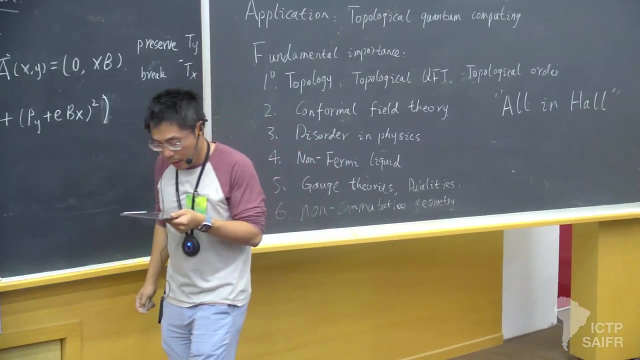 choose, have the zero component in X direction and plus py time up, plus my gauge and square. okay, that's the Hamiltonian we are going to. we need to solve right. we want to solve the Schrodinger equations like that is what we want to find state. that is the. 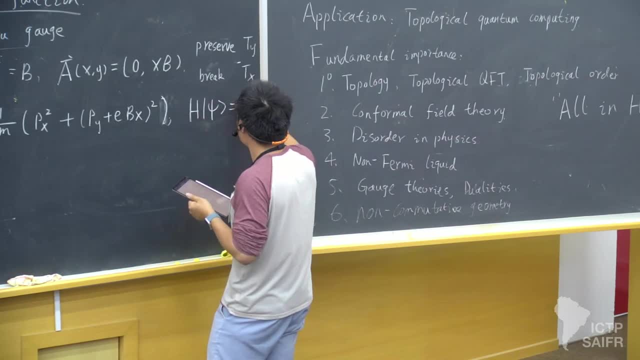 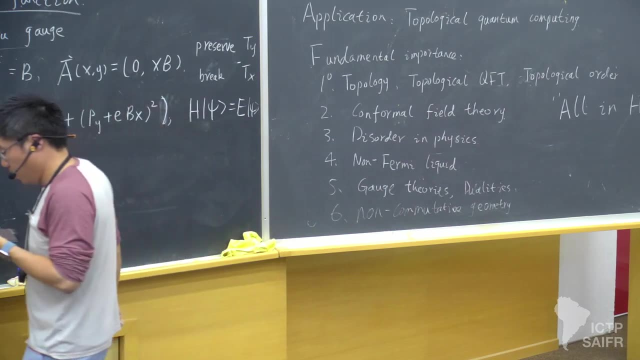 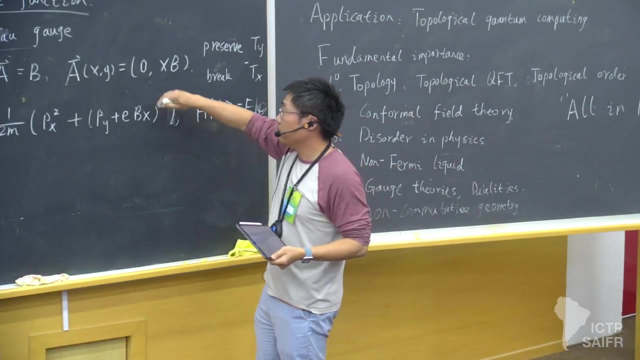 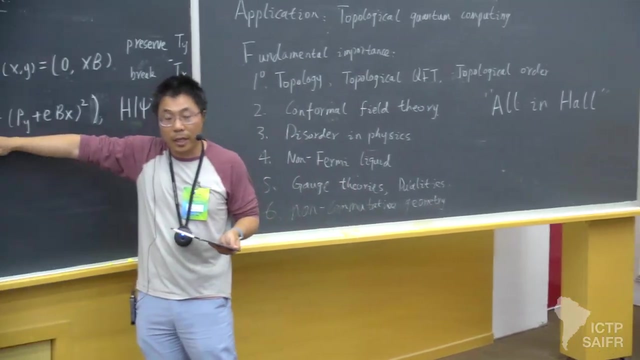 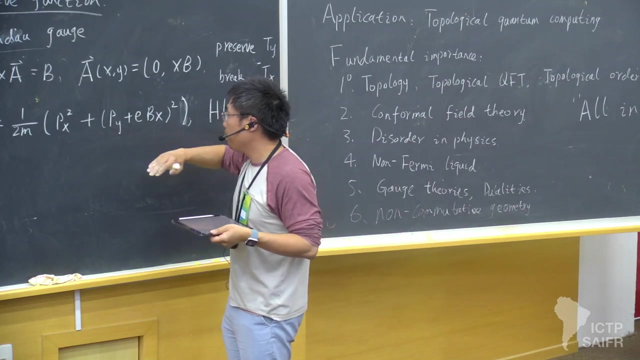 eigenstate of my, of my Hamiltonian right. so the first thing that you, you, you should notice is that, as I said, this vector potential preserves translation along ty, but breaks tx right. that also means this Hamiltonian preserves tx, but sorry, preserves ty but breaks tx right. that. 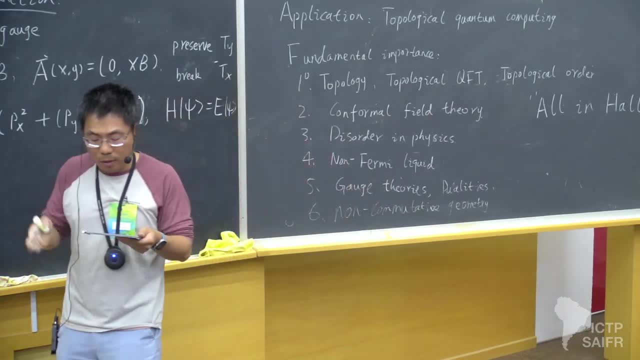 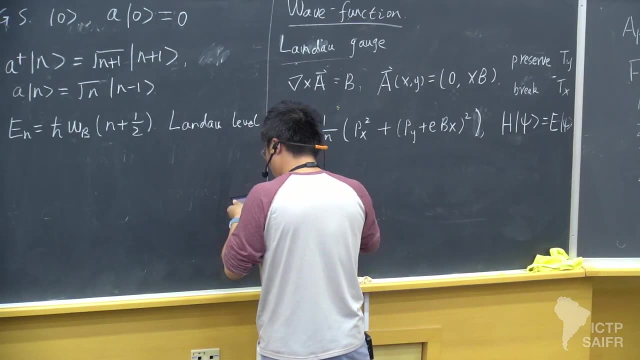 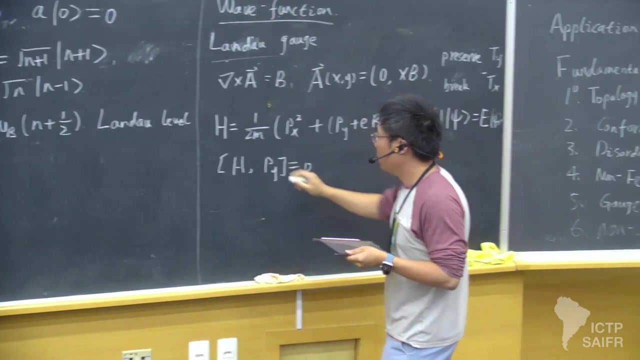 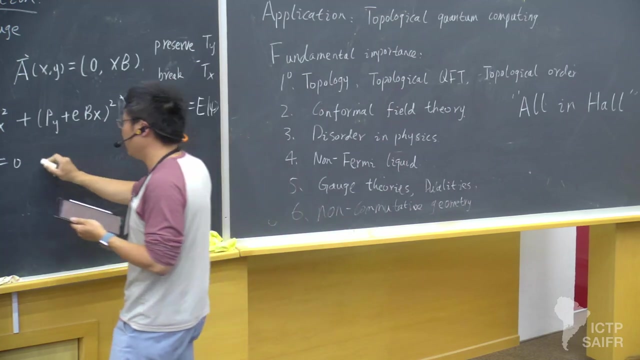 means there's a good quantum number, that is a momentum along the y-direction. so we can. so, in other words, what you can show is that this Han Tony commutes where's the, the momentum Py, and then we can say: py is a good Quran, burr right py. 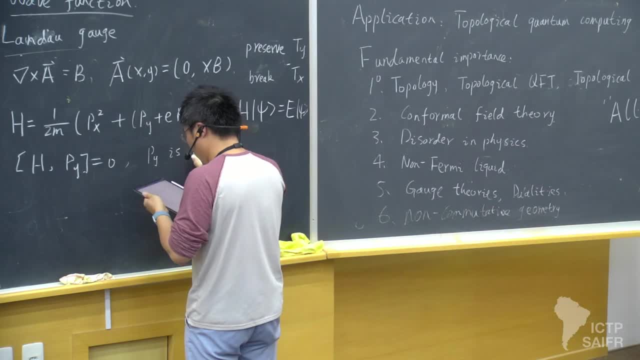 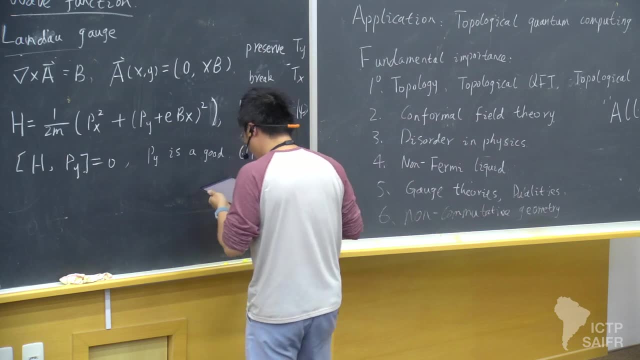 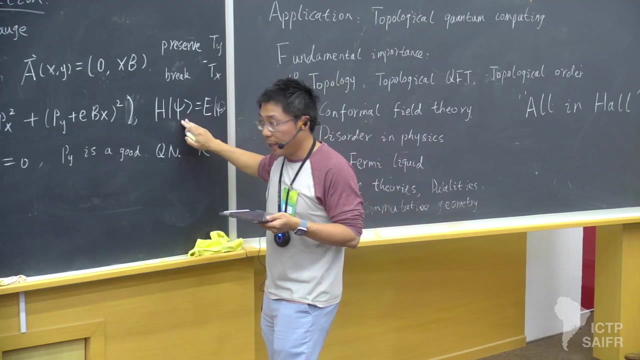 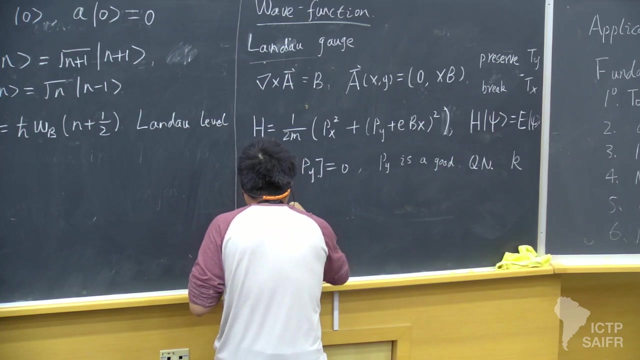 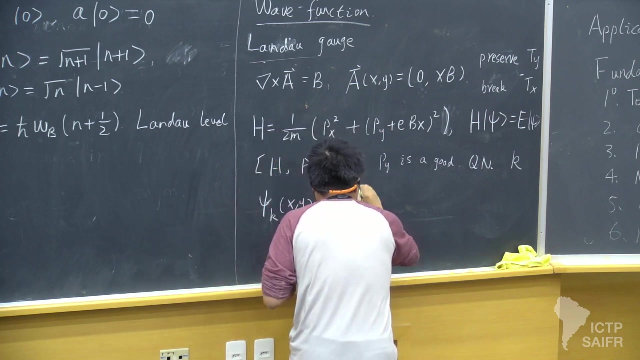 is a good quantum number for the state. It's a good quantum number for the state, which I will call it k Okay. so now that means I can label each eigenstate with this quantum number, k Okay, and it will have this exponential i, k, y factor. 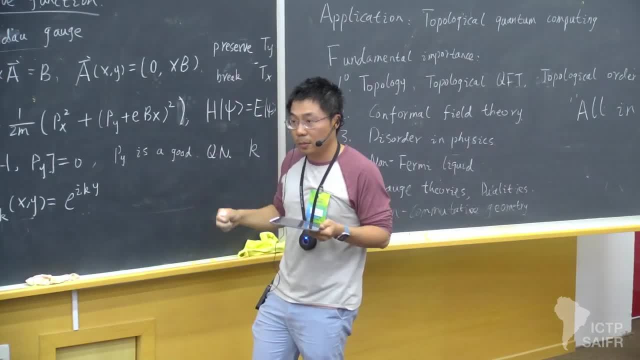 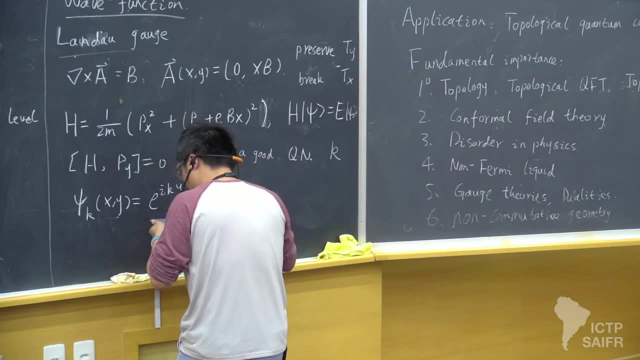 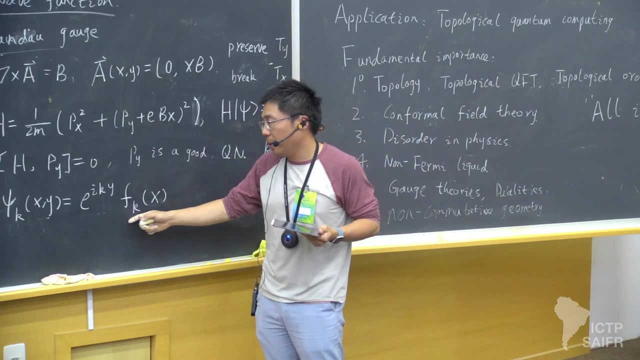 just giving me, just gives me the momentum of along this y direction, right, And then it will be some function that only depends on x, right, And it also depends on the momentum- k, right? Okay, that's the the wave function answers you can write down. 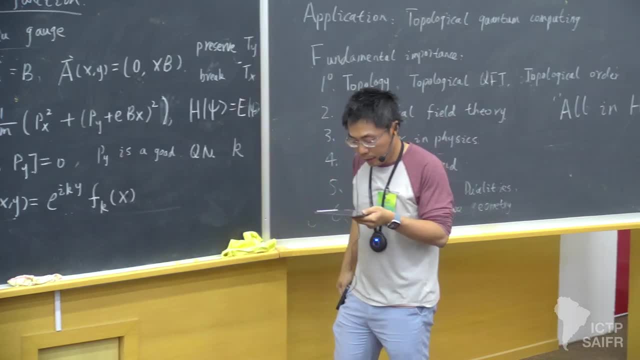 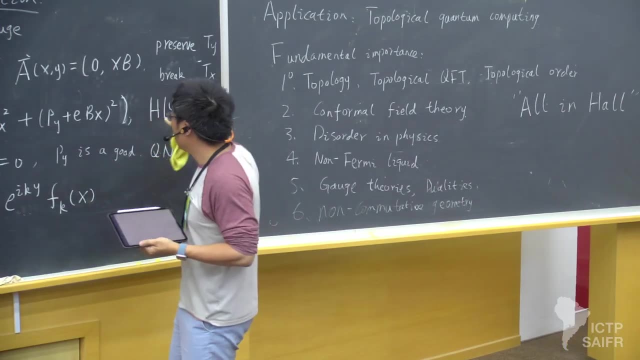 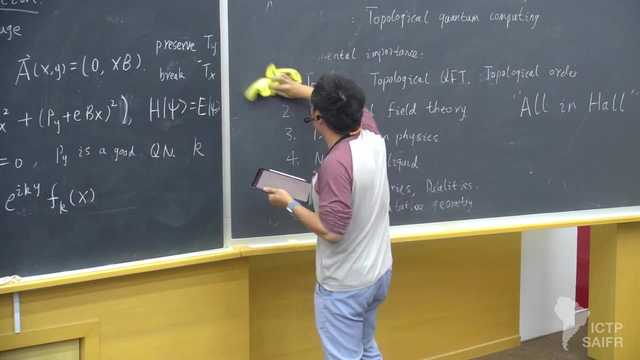 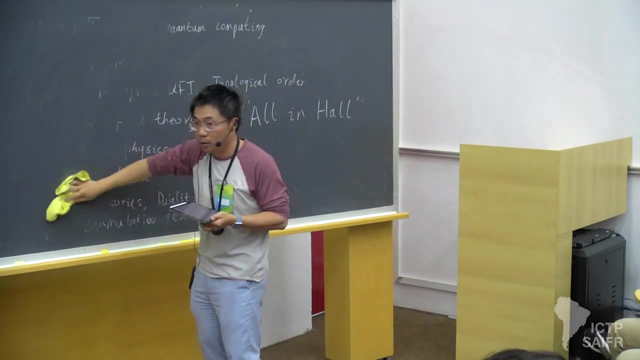 for this eigen problem. right, And now? what you can do is that now you just insert this wave function answers to this eigen function equation and then you end up with a differential equation, which actually was no surprise that you will say it's again reproduced, the harmonic order. 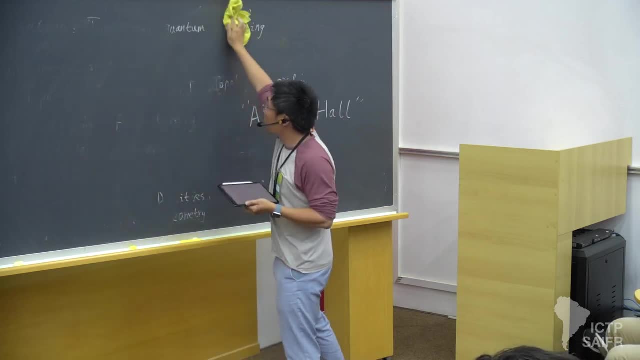 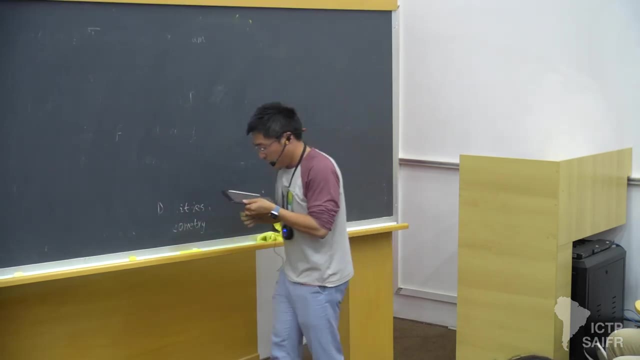 but, like I said, you kind of do the same thing So you can do something like differentiate the selves, Okay. so I'll just give you a bit of a test here. I'll just give you a little test. So, in fact, 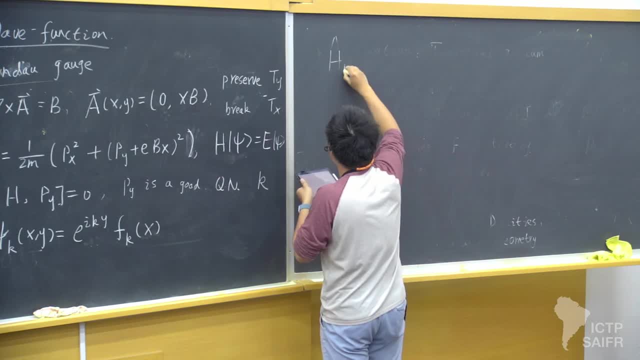 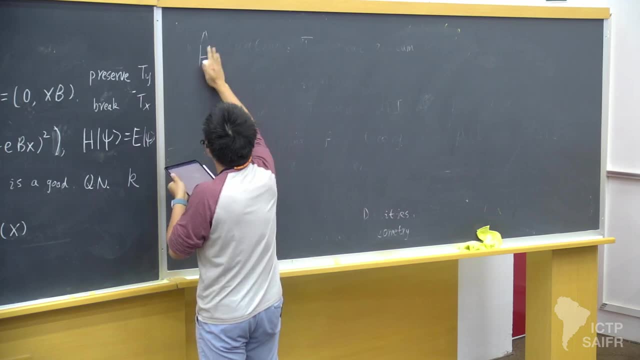 I think that's what we're going to be doing, And so I'm just going to give some incorporate into the algorithm. So that's the parsing method, And here what I'm doing is I'm just going to solve this stuff, And so I'm going to do this. 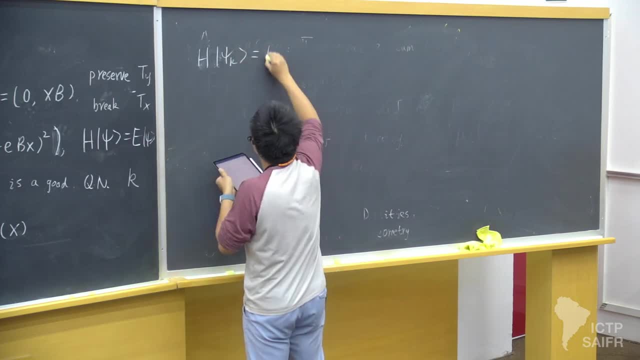 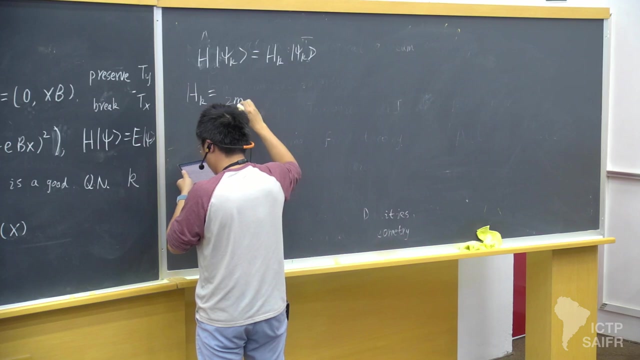 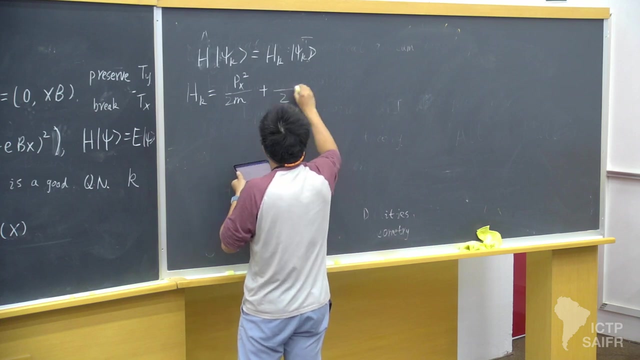 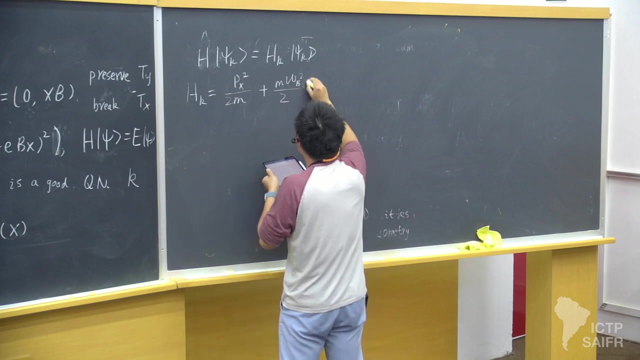 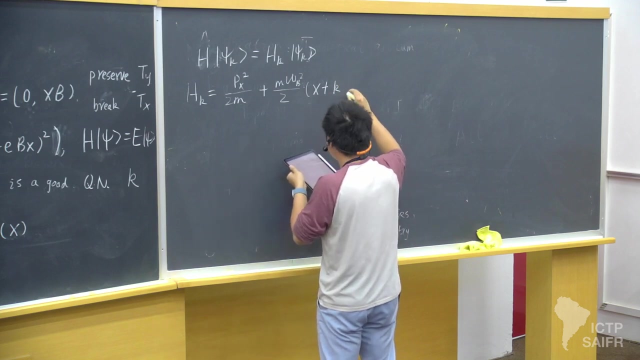 Okay, All right, All right. you will end up with something like this: hk times psi k, And this hk is 2 pi m px squared plus 2 m omega b squared over 2 times x, plus k times h bar over b, right? 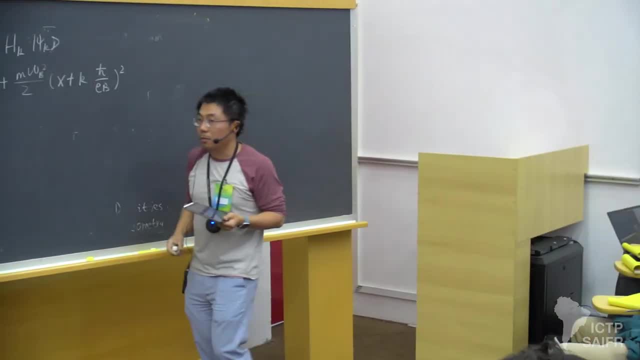 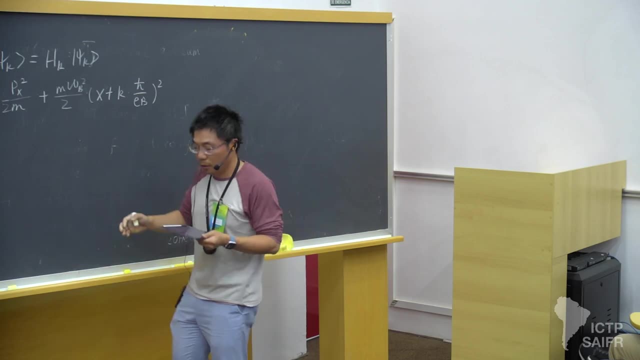 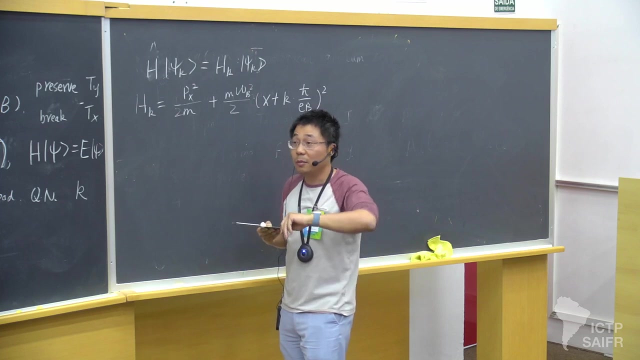 And that's what you end up with, And you may quickly recognize that that's actually the Hamiltonian for the harmonic oscillator, right? And then you can solve it and get these wave functions. I think I'm running out of time, right. 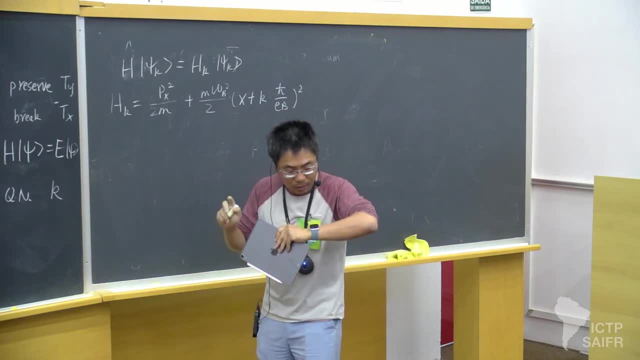 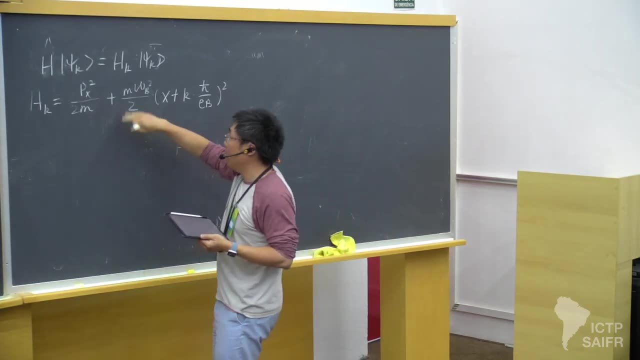 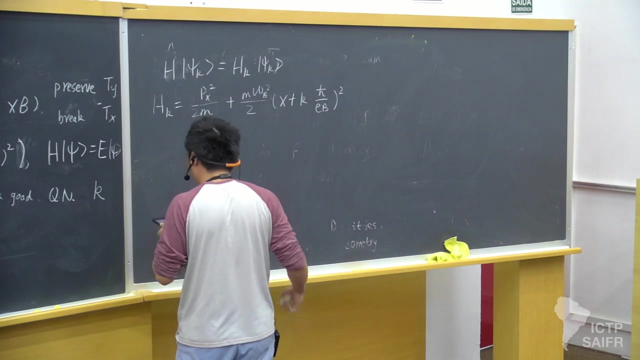 Yeah, let me like maybe spend around 2 or 3 minutes to finish this. Yeah, So you end up with this harmonic oscillator. Then you can solve its wave functions just like what you did for the harmonic oscillator. right, You can get this energy. 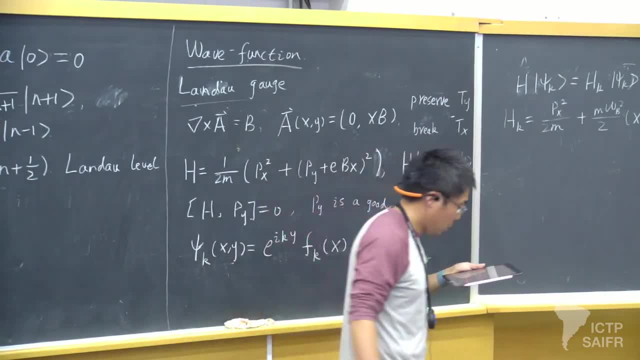 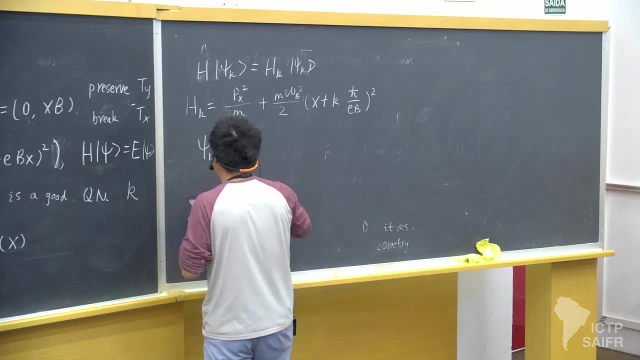 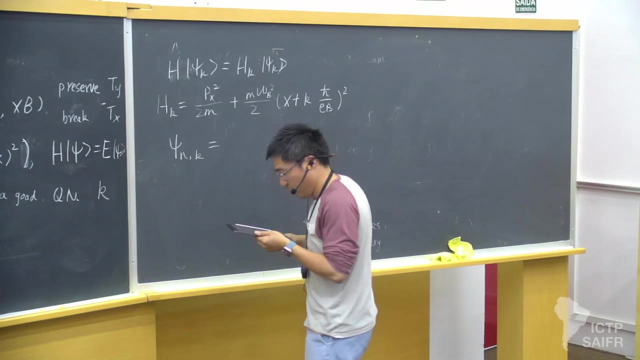 which will be identical to this guy, So I will not write it down. And the wave functions. now we say it's clear that I get another label right, that is n, which is really just the level of my harmonic oscillator. My wave functions will be: 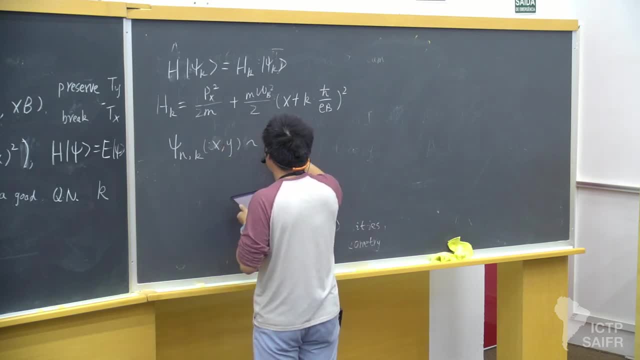 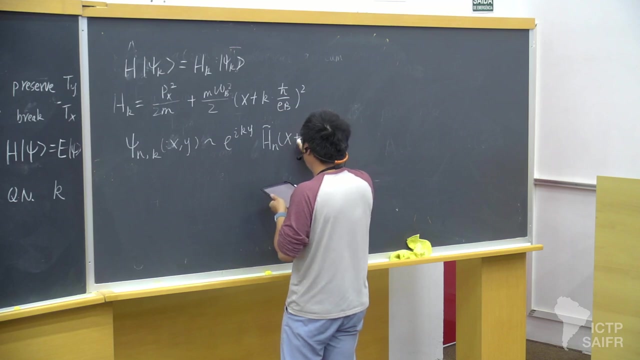 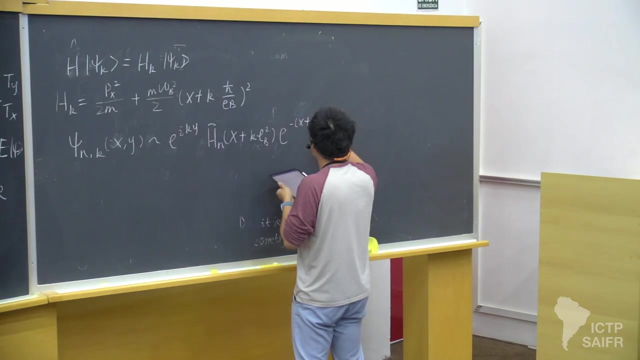 like I get this exponential iky and then I get this exponential iky And then I can get the y constant, which is 100, that is the solution of the harmonic oscillator, that is Hermit polynomial that we learned in the quantum mechanical course. 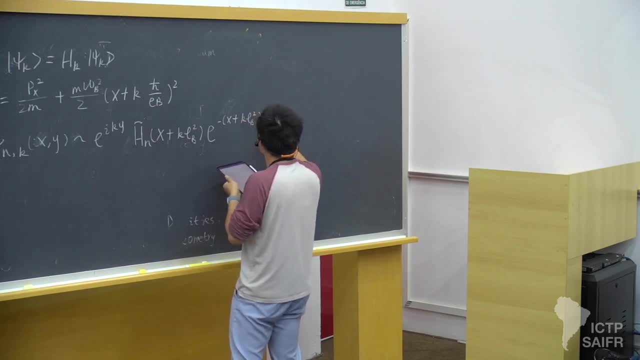 And that is my solution. So so, basically, I would be able to solve this. So let me call it Htelda, And that is the solution of the harmonic oscillator, that is Hermit polynomial that we learned in the quantum mechanical course. 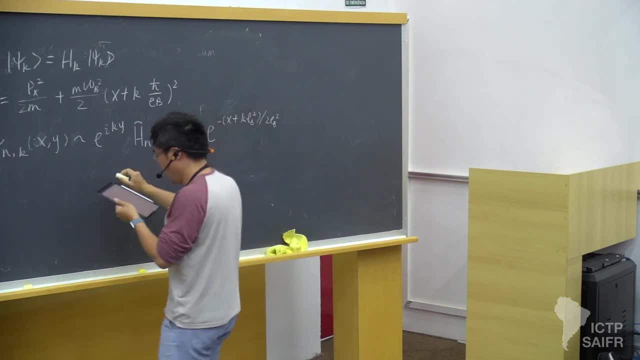 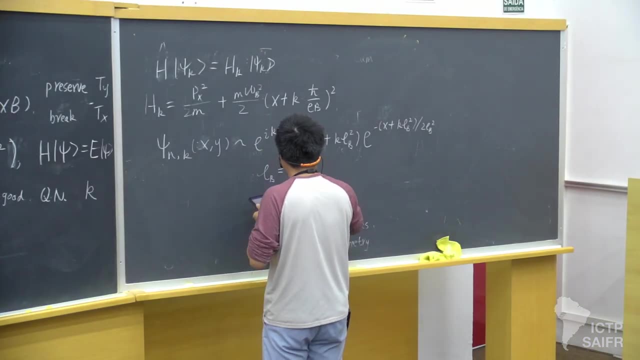 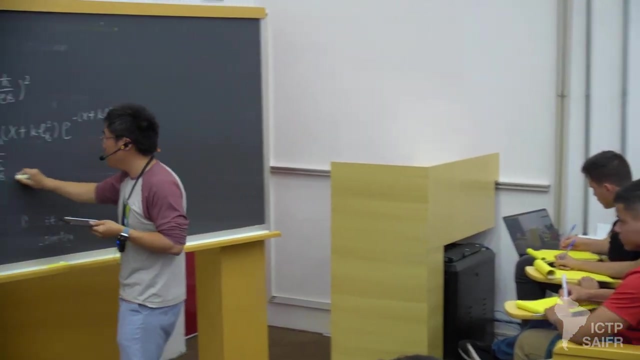 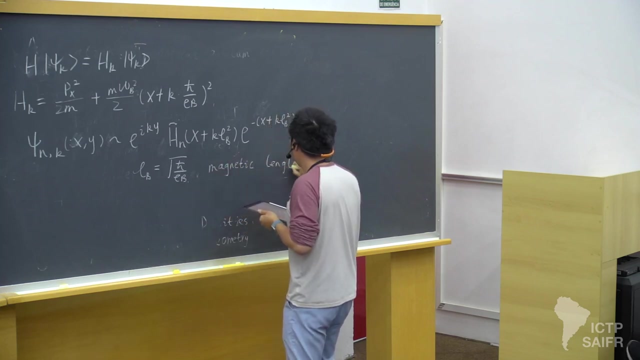 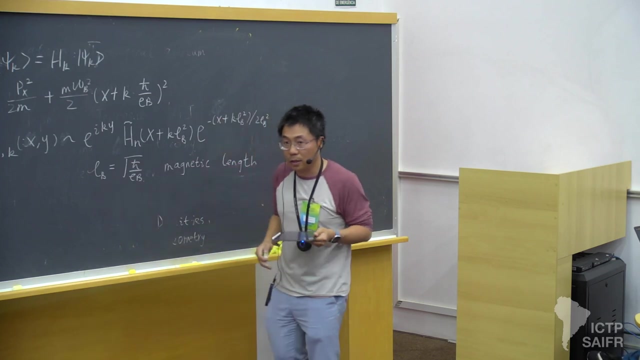 That is my solution. And here Lb is what we usually called magnetic lens, which is really just this guy. It's another very important scale that again it's called magnetic. It's another very important scale that would enter at many places in the physics of quantum Hall effect. 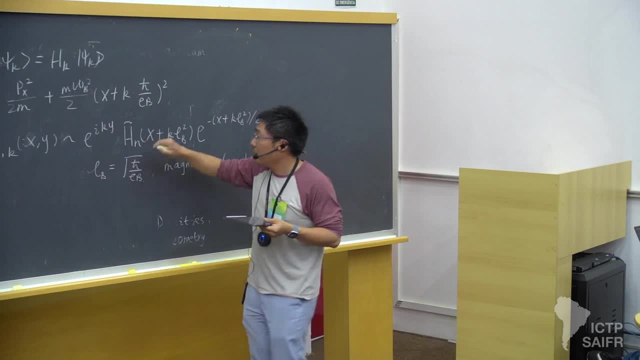 So yeah, that's H-Hermit polynomial. Yeah, probably you are right. Yeah, I. yeah, that's something should be easily figured out in quantum mechanics. If you open up quantum mechanics and you look at the textbook, then yeah, 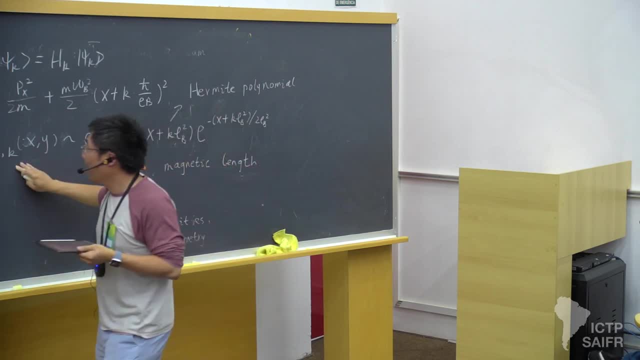 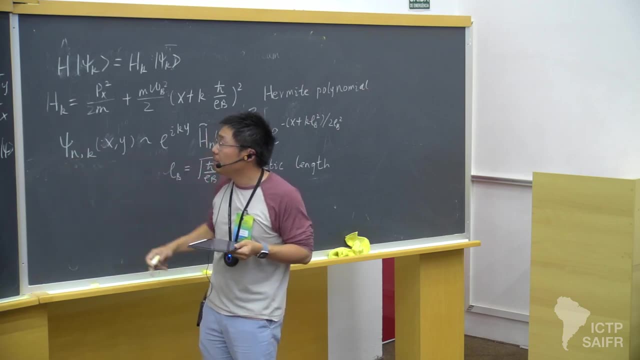 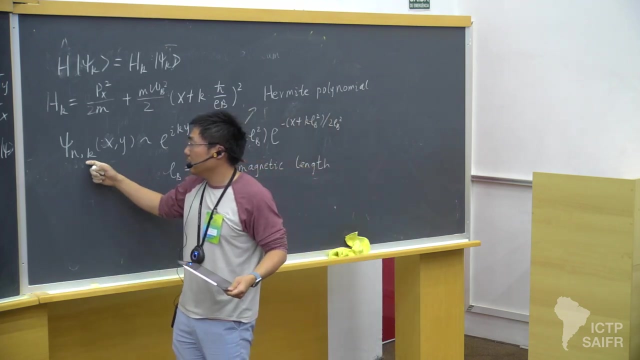 So the important thing is that here the eigenstates will have two labels. One is that I called n, which is just labels the state of this harmonic oscillator right, And the other label is the momentum, that is, the momentum along the y-direction. 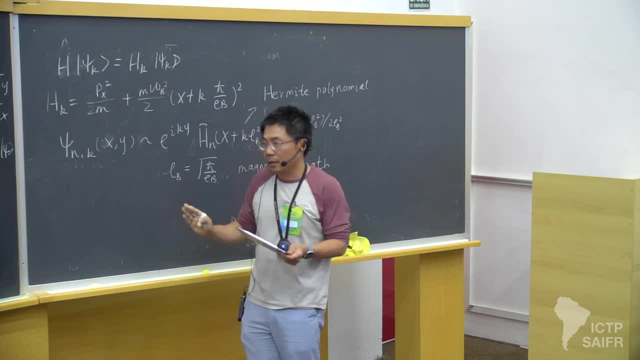 that I called k, And now you see that this momentum makes it different from the usual harmonic oscillator, And that's also the arranging of this degenesis of lambda levels, that so, which I will explain in the next lecture. Okay, so I think it's good to stop here. 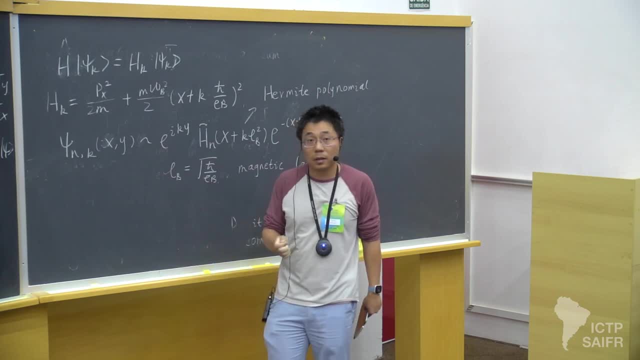 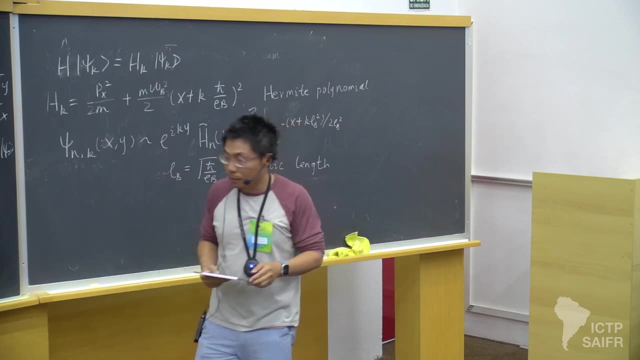 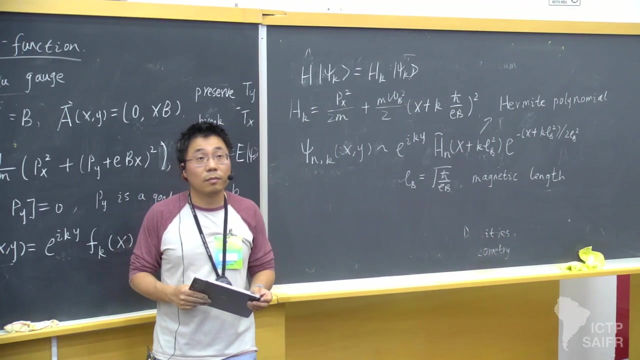 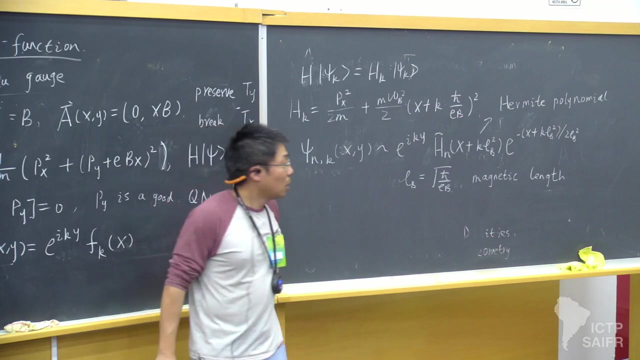 Yeah, so now we have time for questions. Maybe wait a little bit for the microphone with. yeah, you have to speak quite close to the microphone. So it is just a quick question: why couldn't we have one k for y and one k for x in the wave function? 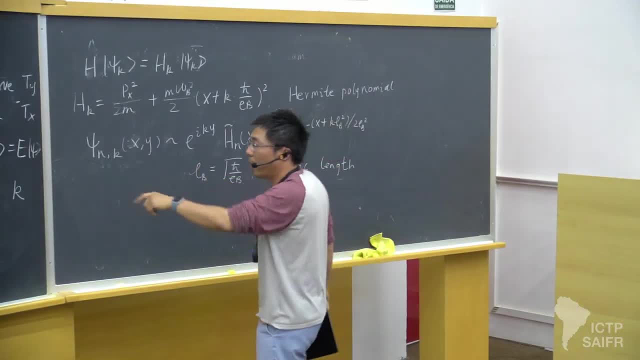 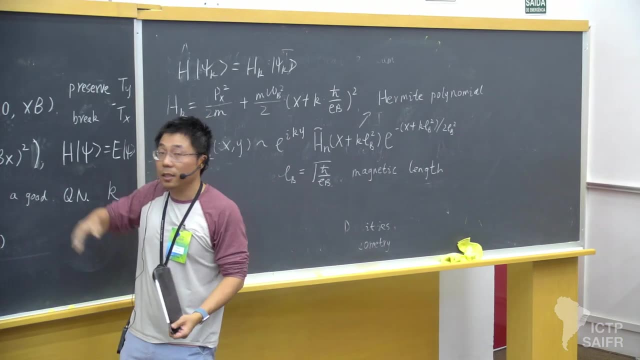 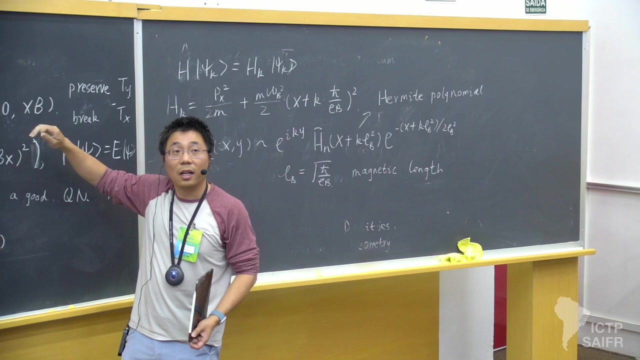 Yes, so the reason is because the only p y is conserved, right, p x is not conserved. all right, That's. my gauge breaks the translation along the X direction, I mean, but the momentum in the X direction must be the same of the Y direction. Yeah, that's a good. 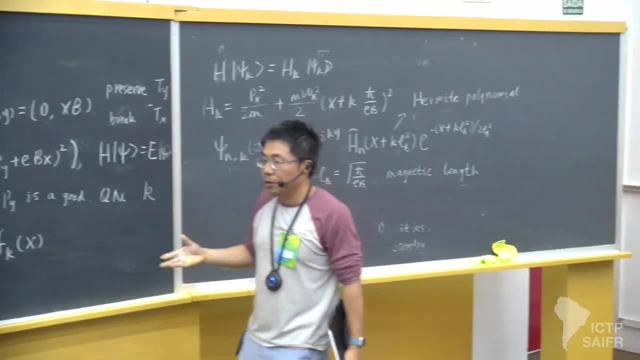 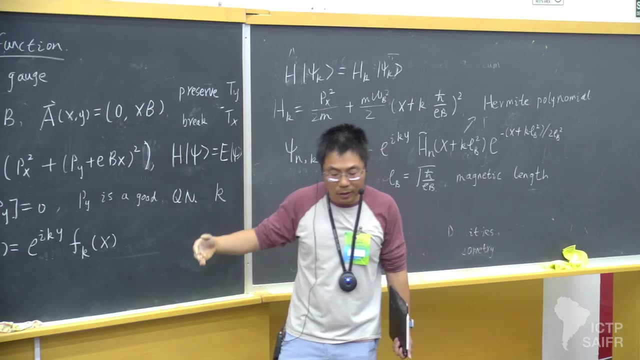 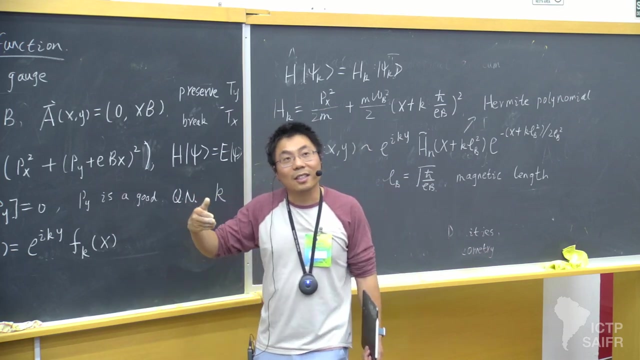 question. So in the end you can also choose another gauge. let's say you just swap those two guys, then you end up with wave functions that has momentum along X direction but it doesn't have momentum along the Y directions. It has to be break some way right And that. so in other words those 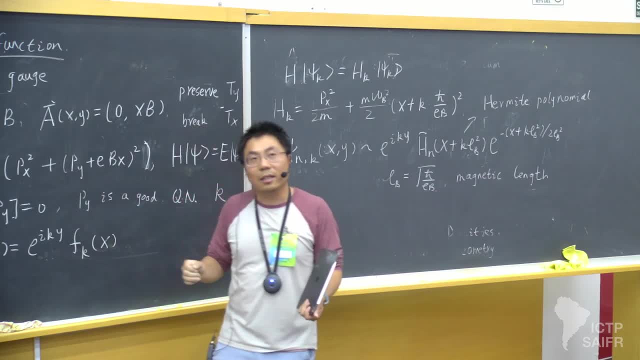 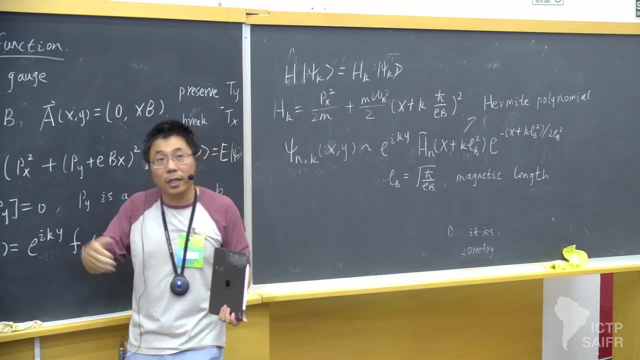 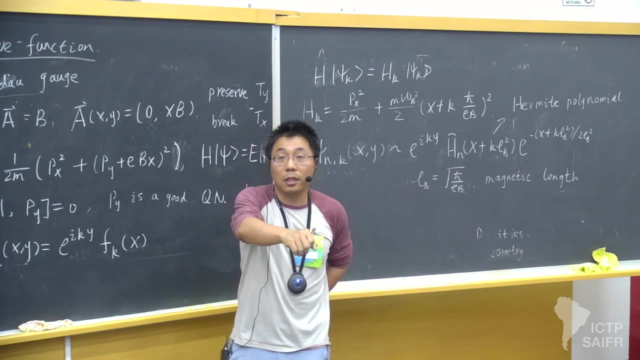 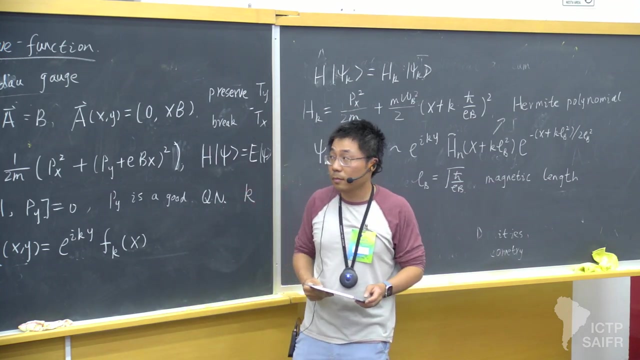 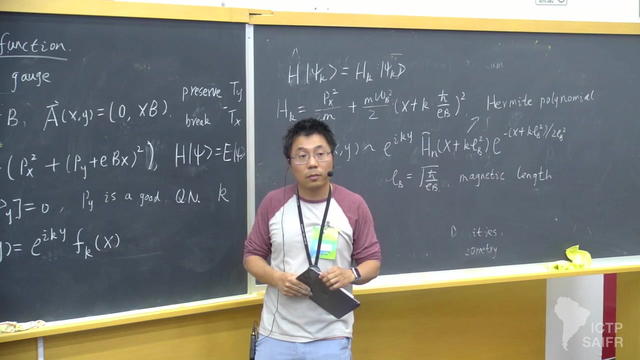 wave functions are not gauging invariant. That is also something we learned in quantum mechanics, right? If you have magnetic field, then the wave function may not be gauging invariant. So there's a question. I just want to know how you have there the presumption that the momentum in the Y 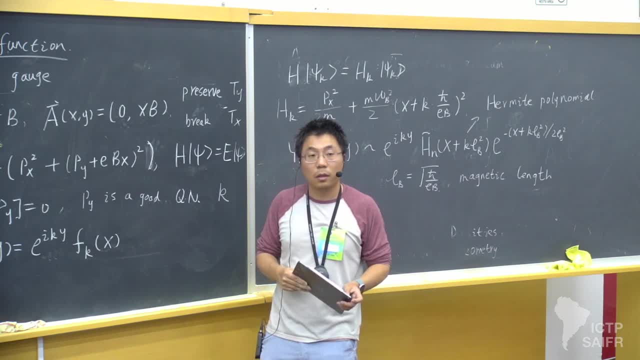 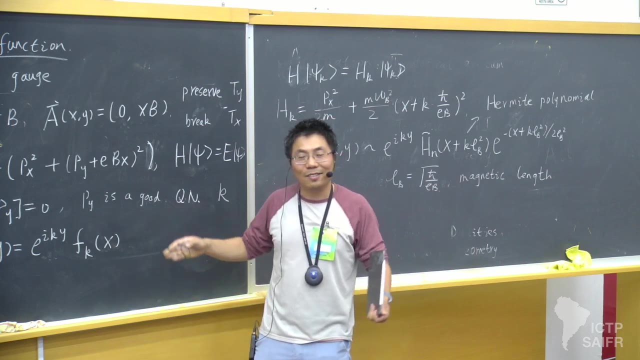 direction. eigenstates are also eigenstates of energy. Can you? what in the problem gives you the, let's say, the hint that you can make this assumption? Well, it's, I think it's a basic principle of quantum mechanics, right? If some symmetries, if the Hamptonian has some symmetries, then 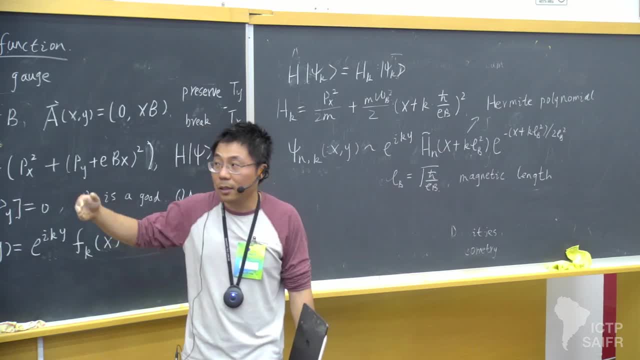 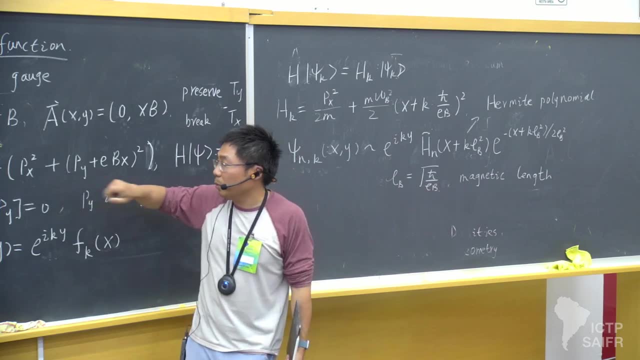 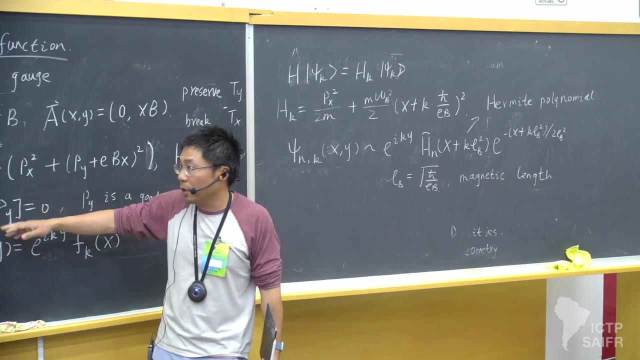 I can label the eigenstate of that Hamptonian using the quantum numbers of that symmetry. right, And here this is what I'm doing. right, I write down the Victorian function which is called Crimea, It's. I'm writing down the Centaurus, and. 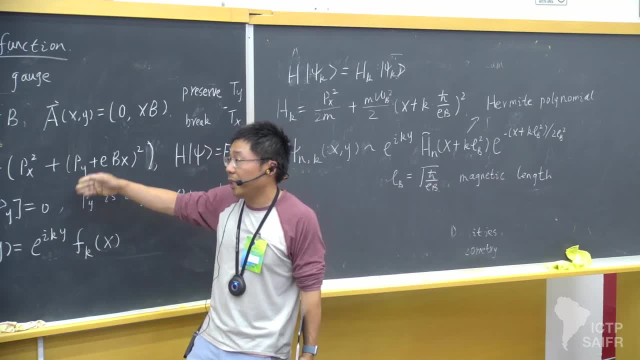 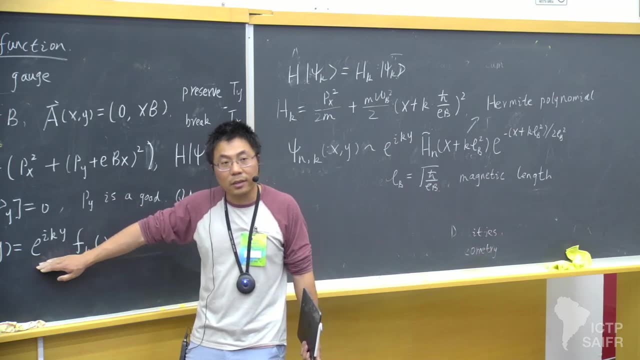 it's like the diameter of the working perimeter right. If you can write down the Hamiltonian and then I realize that it commutes with P Y- that is, a generator of the moment- along Y directions, then that means I can simultaneously diagonalize my. 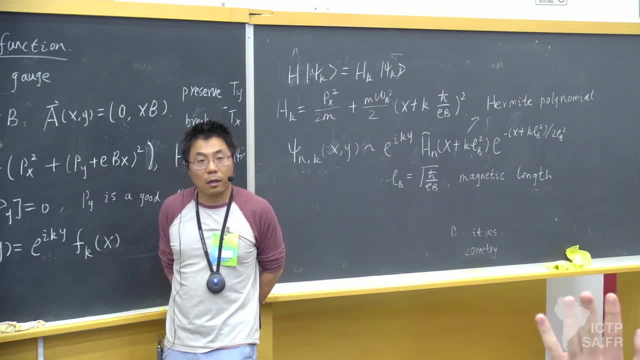 Hamptonian and the momentum operator. right, That's, I end up with this. answers right, Okay, understood. Then why can't you also assume it's a eigenstate in the X direction? at the same time, it is a 90 state in the y direction? Yeah, the thing is that this Hamptonian 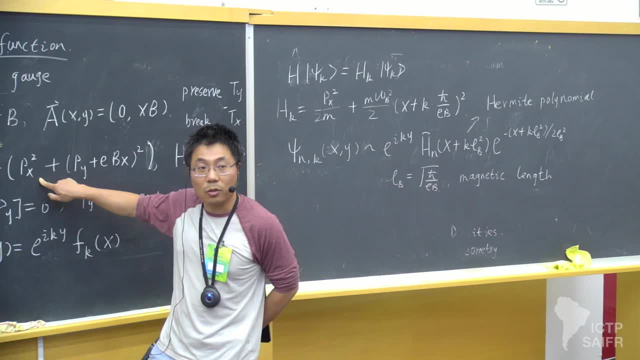 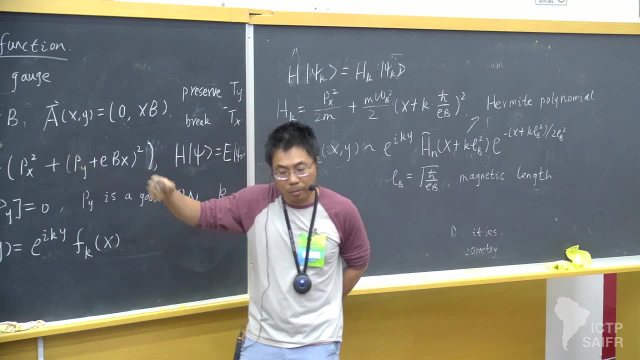 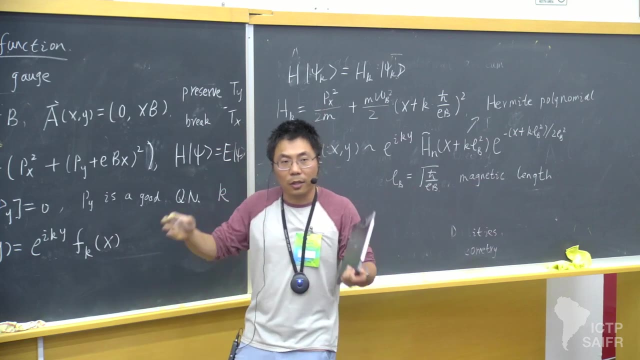 does not commute with px right, so then I'm not allowed to do so. Okay, It all comes from the choice of my gauge. I will also come back to this point about the choice of gauge. I will play with different gauge choice and then to give. 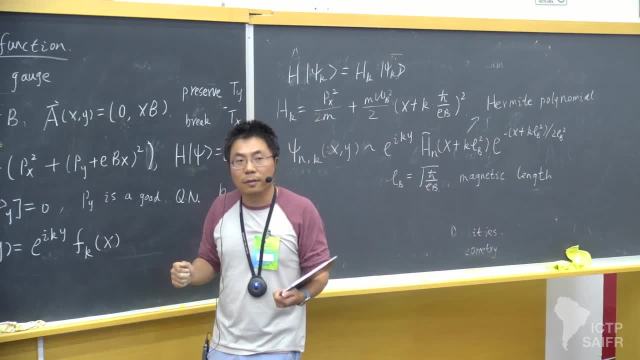 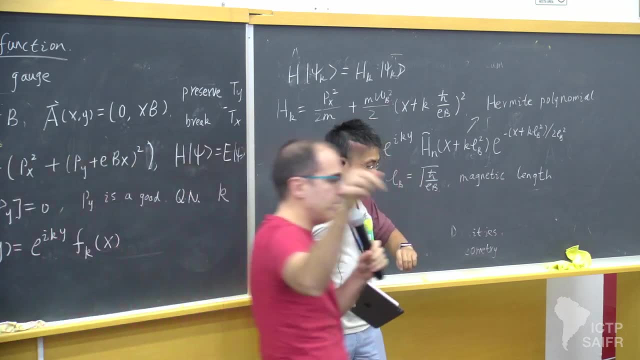 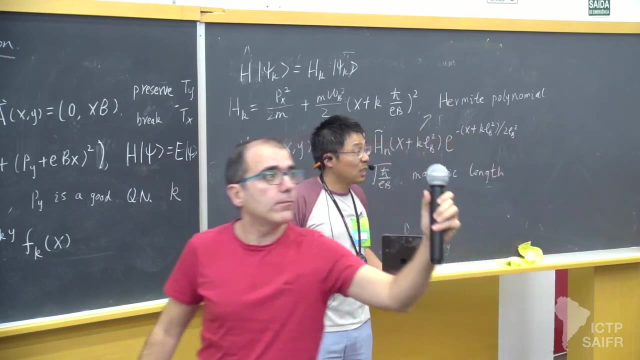 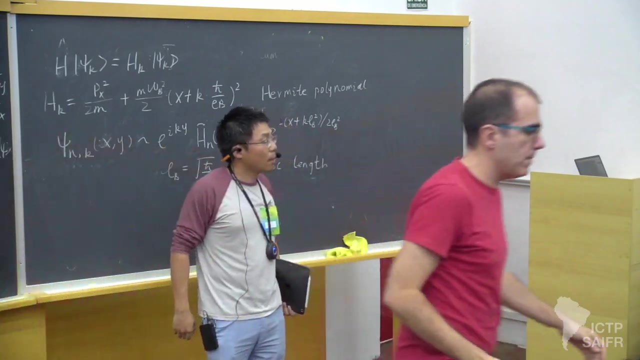 you idea about what the wave functions look like? Thank you very much. More questions? You can keep this microphone. perhaps pass it to someone. Okay, how you can realize that in the quantization here in the first part you can have the case for the, for each n, I think, because here you have two quantum numbers, n and 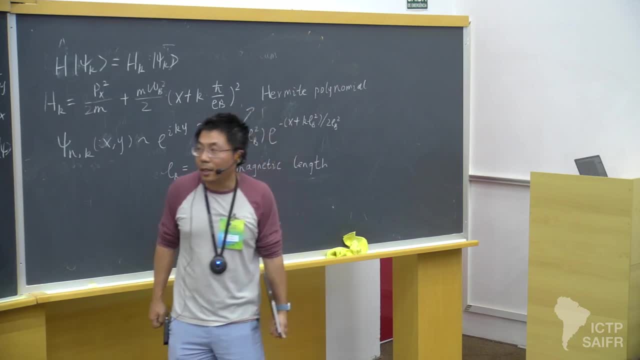 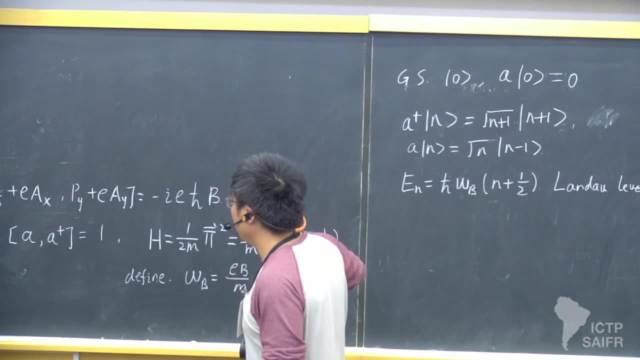 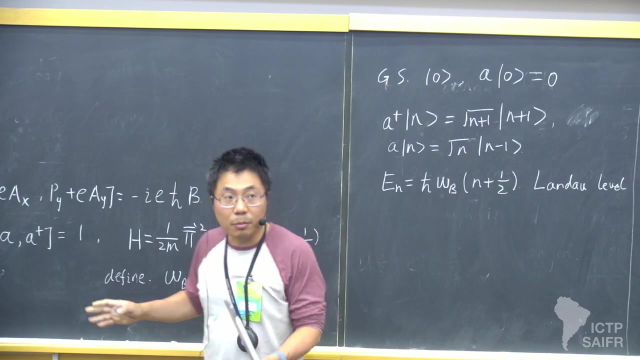 k and here you only have just one. Yeah, yeah, yeah, yeah. that's why that was what I said: this problem using those creation and annihilation operators- I miss some degree of freedom, right? It's kind of obvious if you just think getting a very 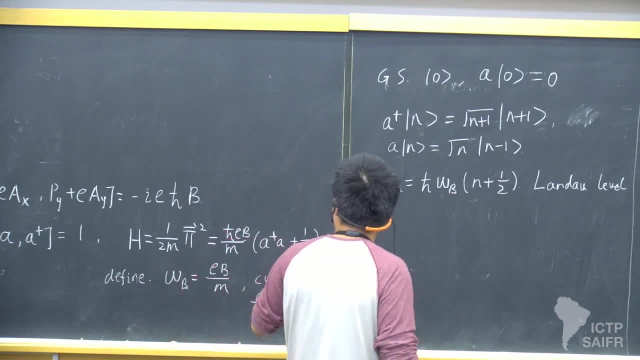 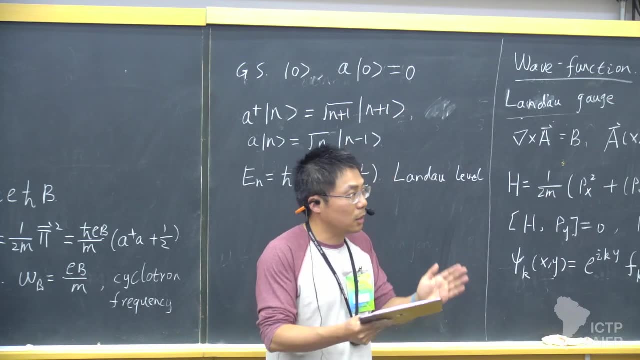 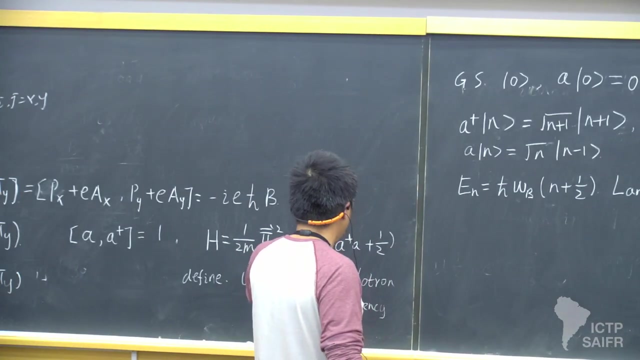 simple way that my harmonic oscillator only have one degree of freedom right, But the original problem has to degree of freedom x and y right And then so it's not totally obvious that, So it's not totally obvious that EX, how to get that degree of freedom back using this approach, although you can. 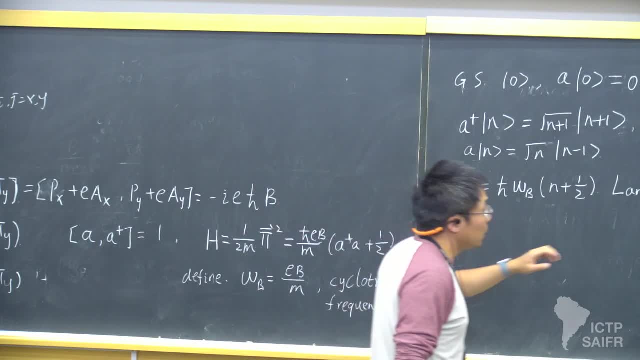 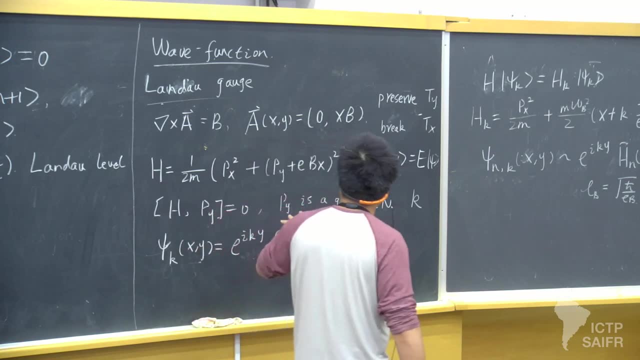 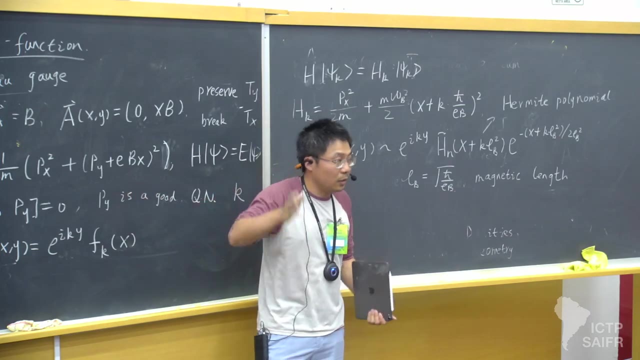 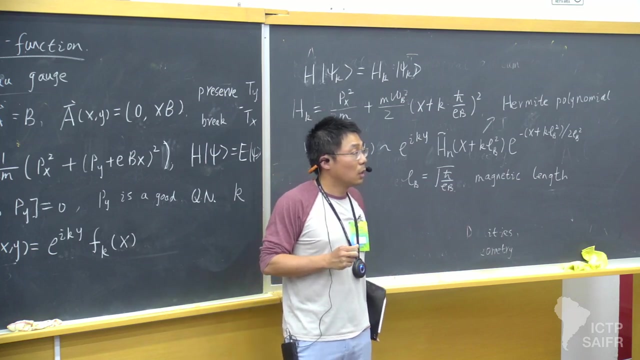 after you realize it's a momentum And in this explicit formulation that I derived the wave functions of this problem- then it's very clear that the other degree of freedom that I have in the problem is a momentum along certain directions after I choose the gauge. Also in this first part, it works for any. 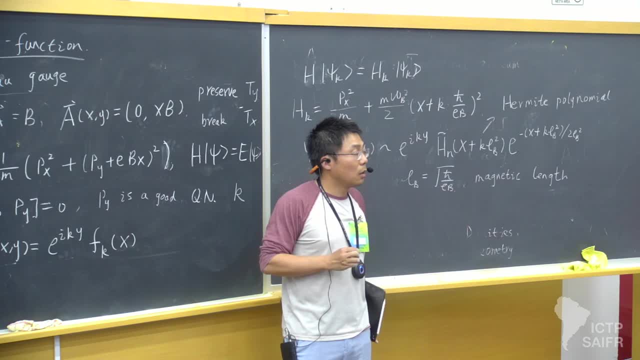 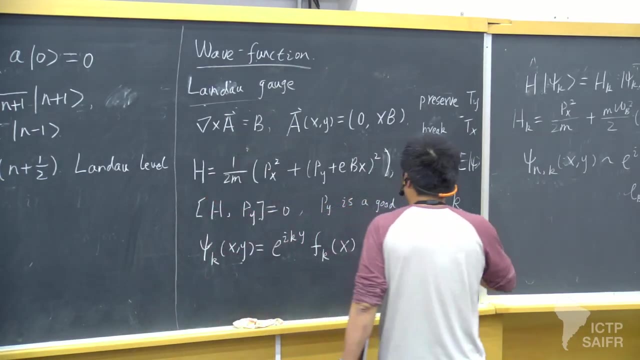 gauge, for any gauge, I think, because here you choose, you choose one. Yeah, we choose one gauge. So yeah, one thing I think I didn't mention is which is actually obvious, is that at each lambda level it's highly. 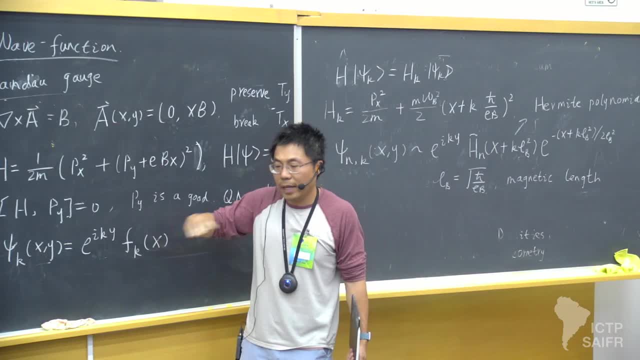 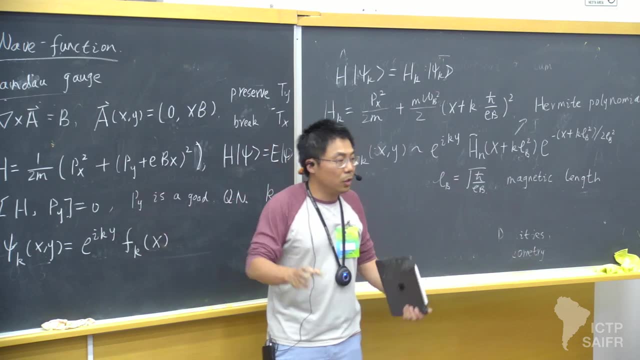 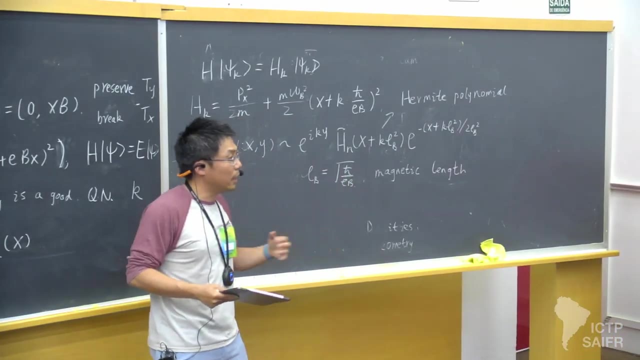 degenerate right, Yes, And meaning that their energies are exact same, and I do. I can have those momentum, take different values, And then what you can do is that you just have those. use those wave functions to do some superpositions. You can get another. 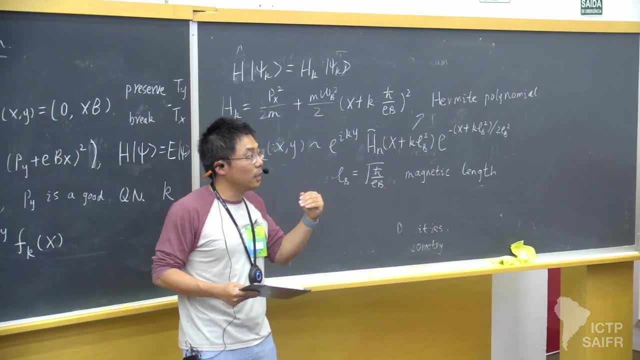 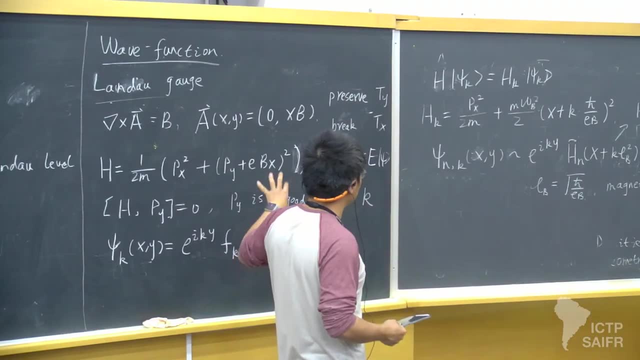 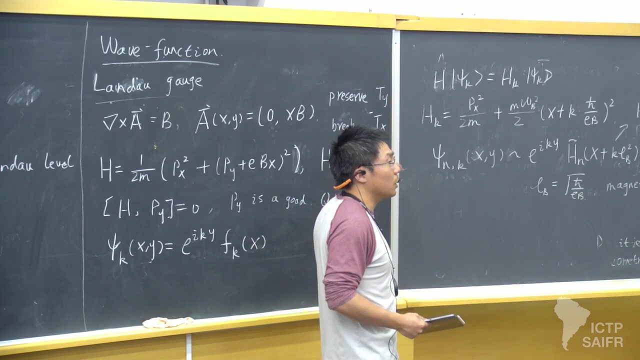 basis of your eigenstate right And you can actually choose some way to superpose them such that those eigenstates have exact momentum along Tx directions But not have momentum along Y directions. You can also do other more symmetric tries and so on. 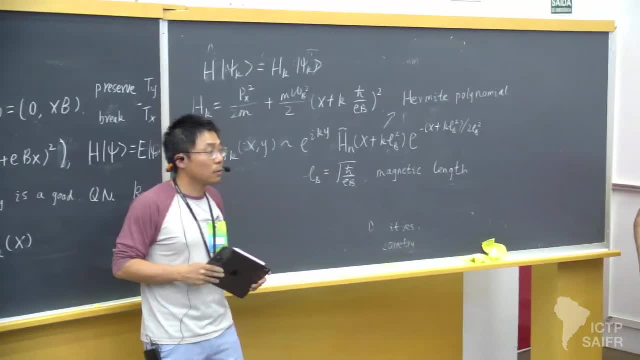 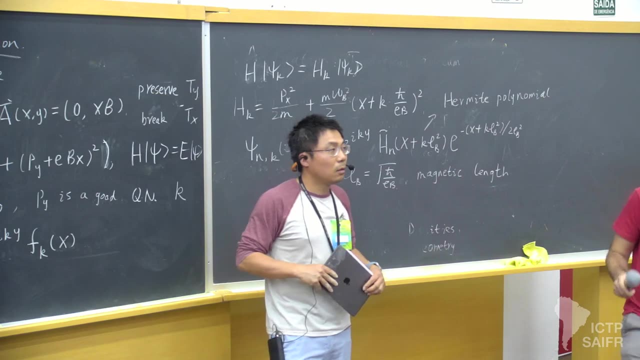 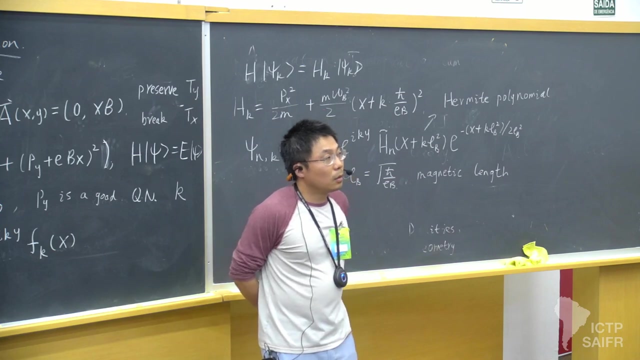 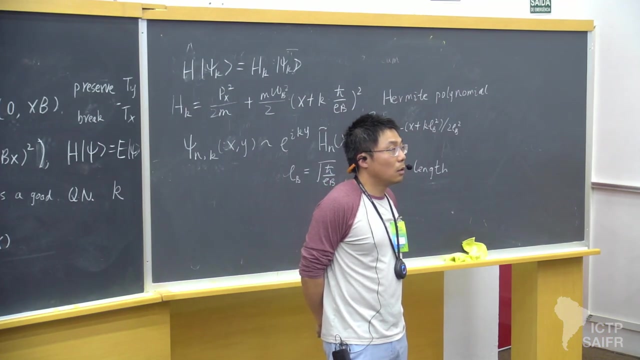 My question is about fractional quantum Hall. I know that when theta is equal to zero, it's a boson And when theta is equal to p, it's a fermion. How do you interpret the physical interpretation? What is a physical interpretation for a fractional value of theta? 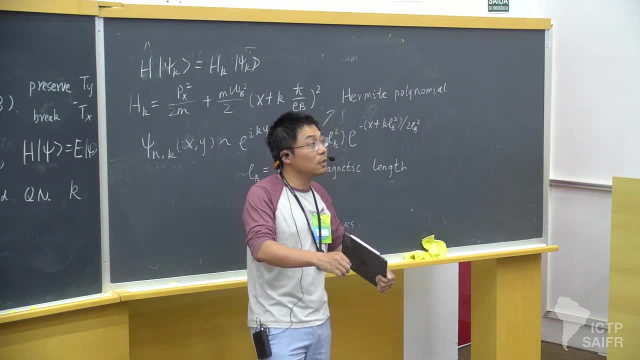 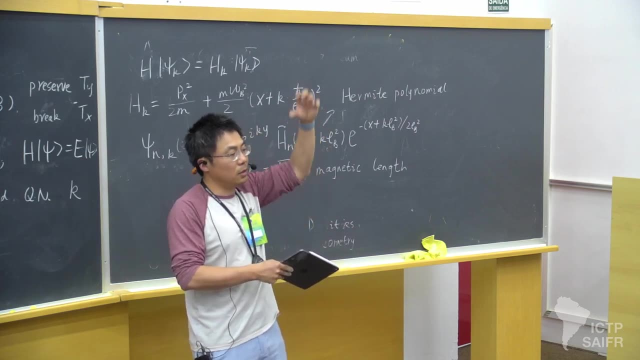 Yeah, that is what we call fractional statistics, And it's a. it's a phenomenon would only happen in 2 plus 1 dimensions. Plus 1 means the time dimensions. The thing is the the yeah, the one way to think about it, and that's again the logic behind it, is that the time dimensions is scooper right. 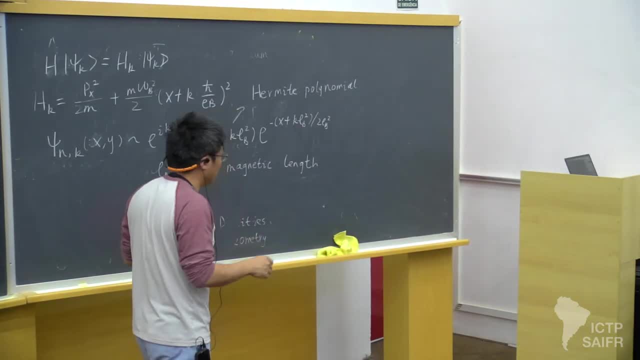 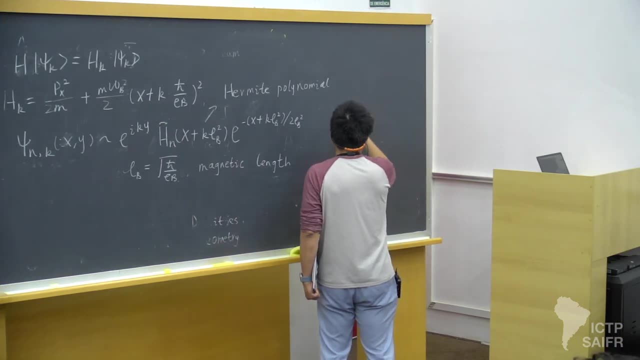 The, the, yeah. the one way to say it is that the time dimensions are the time dimensions of the departments. One way to say that Y is two-dimensional, is special is that let's say you can consider another process. I mean, it's the same process that I have two particles right. 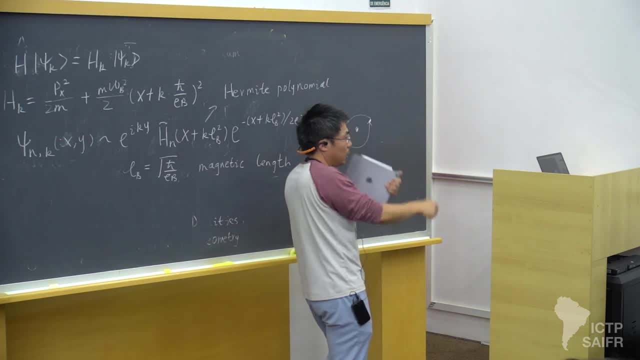 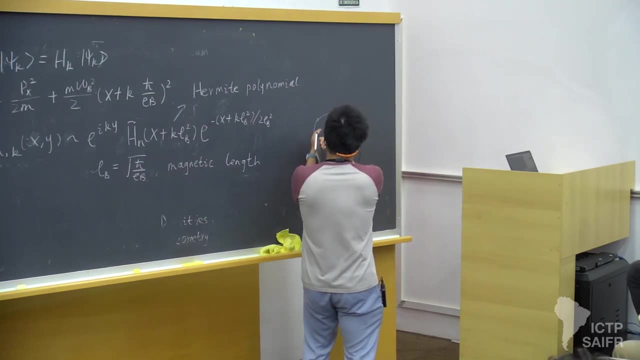 I wind one around the other. That's really like exchanging twice right And now in higher dimensions. what you can do is that you can shrink this loop into trivial right. There's another dimension for you at disposal, that you can just shrink it to identity right. 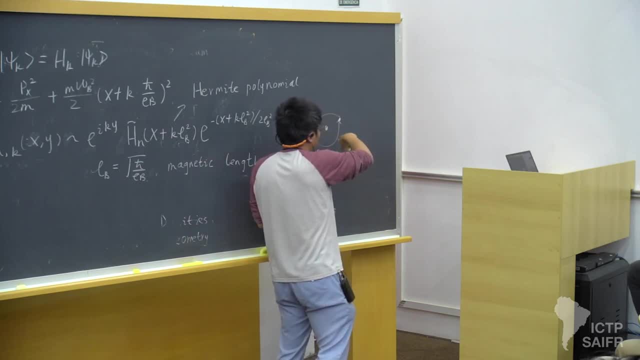 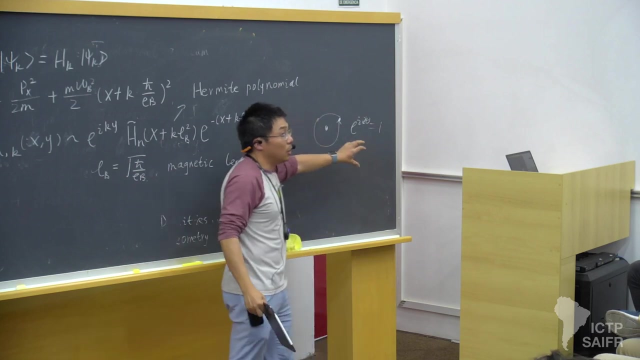 That means for this process the face factor I get will be identical to identity. That gives me EI2 theta. EI2 theta equals to Y, right, That means theta equals zero or pi. But in 2D you are not allowed to do so, right? 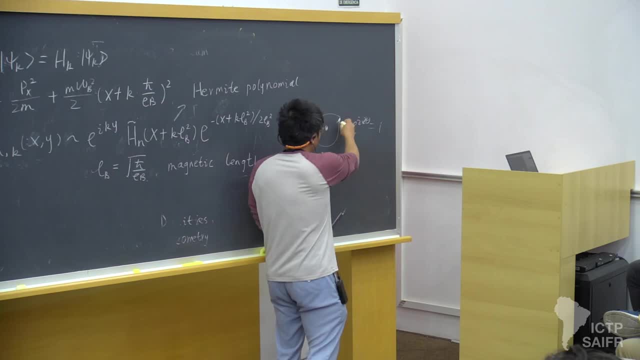 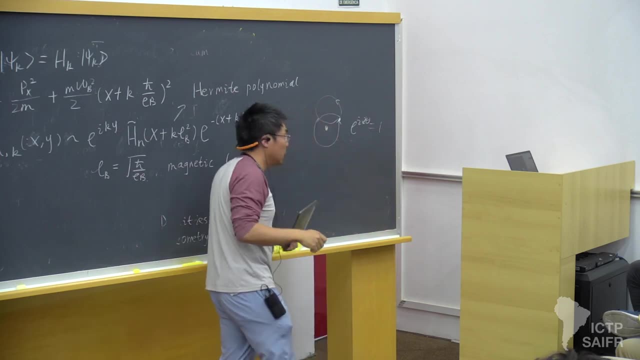 There's no extra dimension for you at disposal, And that means this kind of loop is different from this kind of loop right, And it's related to the topology right People in math literature that is called homotopy right. 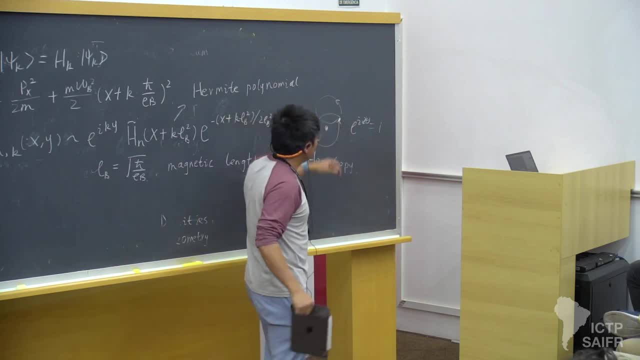 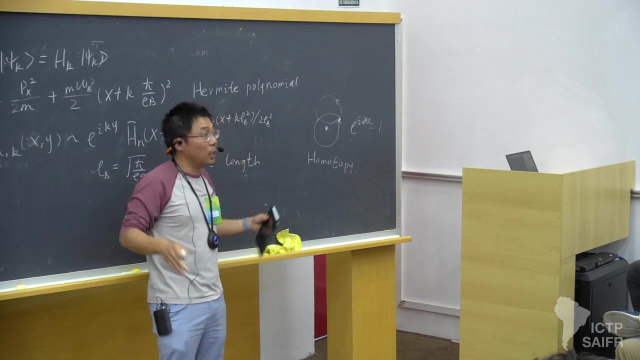 Of this, yeah, And that means in 2D, then I can have, I can have a non-trivial loop, right, And then that means generically, I don't need this exponential I2 theta equal to one. That's how we get, in principle, we can get fractional statistics. 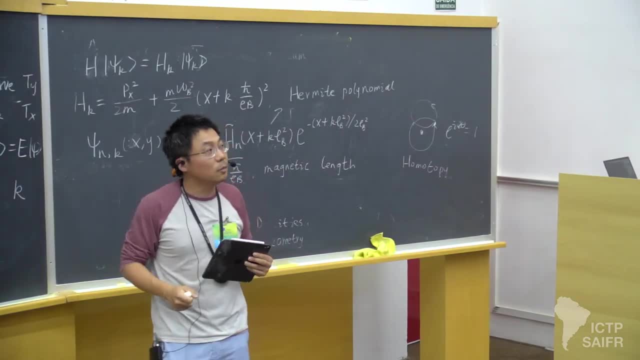 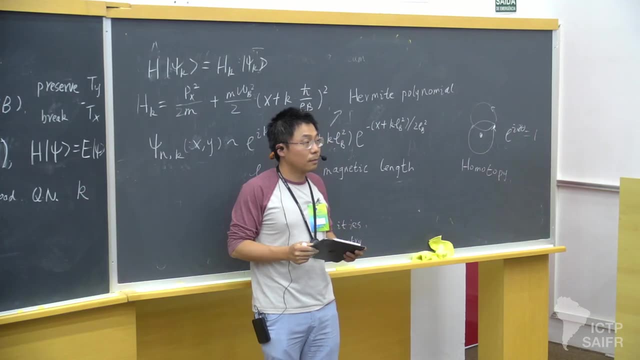 And it turns out that it happens in this quantum whole systems. Yeah, In the fractional quantum whole systems. Yeah, Thank you. In the solutions you found, it's not clear to me what values you're going to use, right, Yeah? 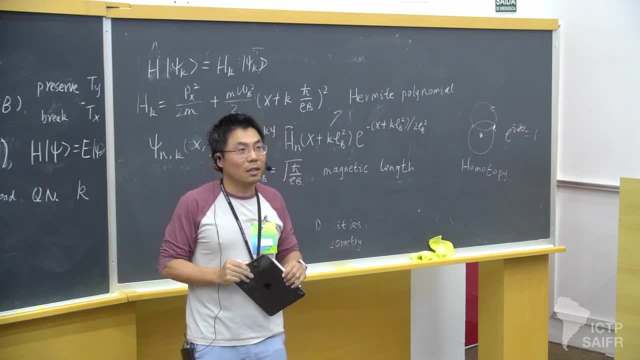 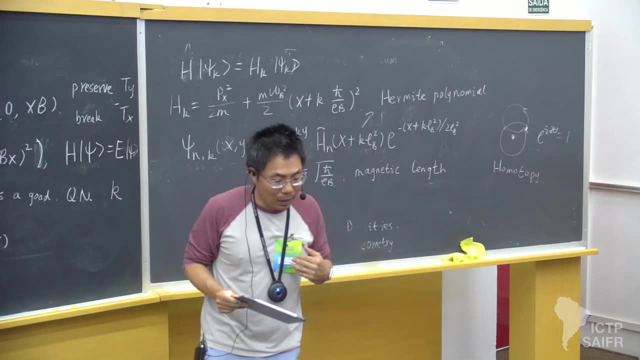 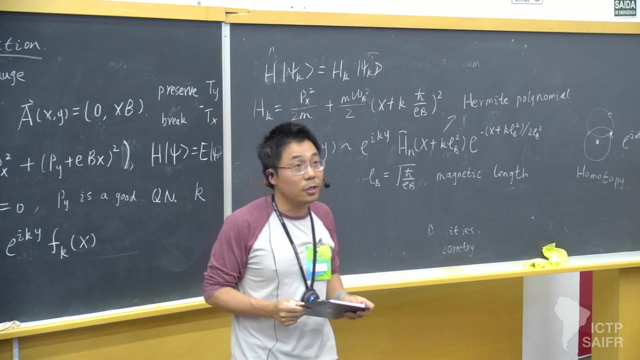 What values can k take? Are they real numbers? integers, natural. Yeah, That's a very good question And that's how you can understand the degeneracy of lambda levels, And I will talk about this in the next lecture. Okay, 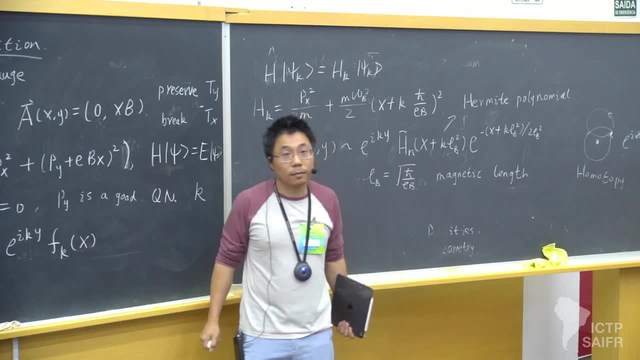 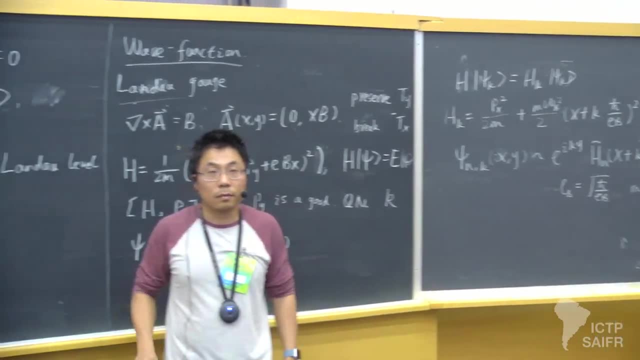 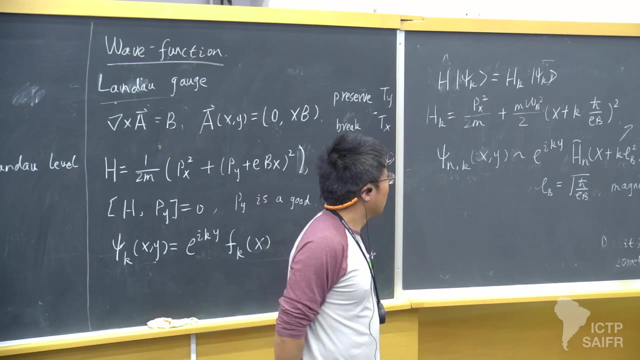 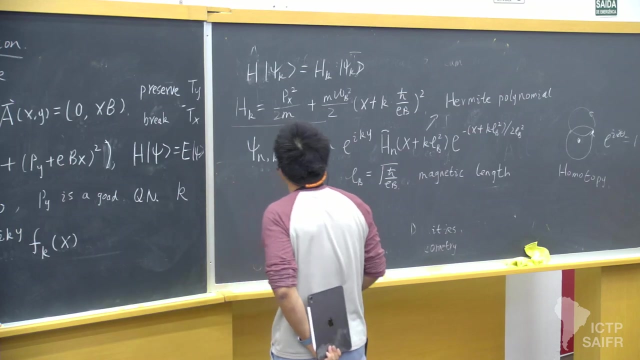 More questions. Can you pass the microphone? Sorry, Maybe I missed something, but how did you get to the final h, q, k, the Hamiltonian? with the You mean this one. Yeah, Yeah, So From what? Yeah? 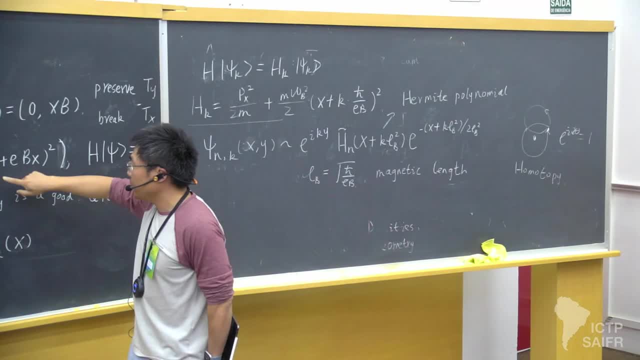 The point is: yeah, it's a very simple thing, right? So what I said is: py is conserved, right? Yeah, It's a good quantum number, Yeah, And then what you can do is that you just replace py. 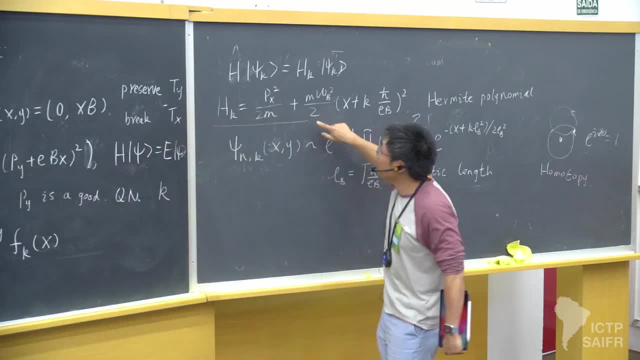 Yeah, Py with k, Then you end up with this: Oh, okay, Okay, Okay, Yeah, But here I probably redefined my The parameters a little bit, and so on. right, You didn't use the answers, right. 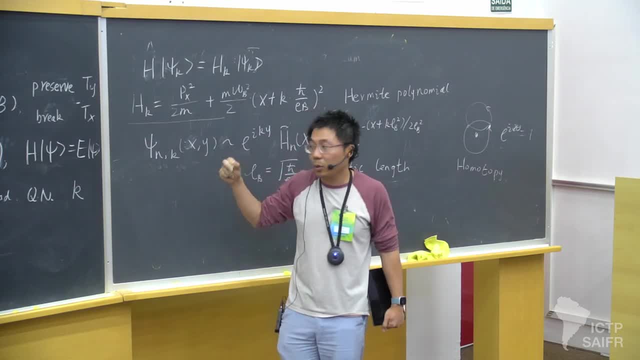 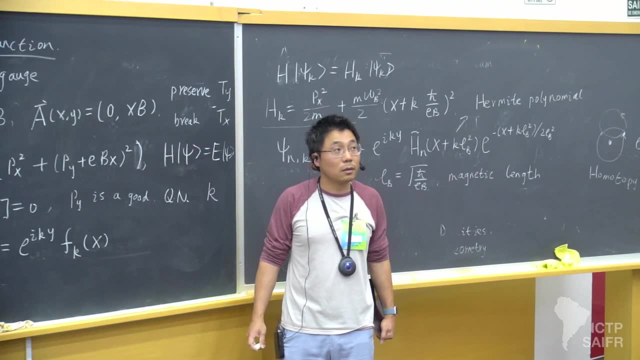 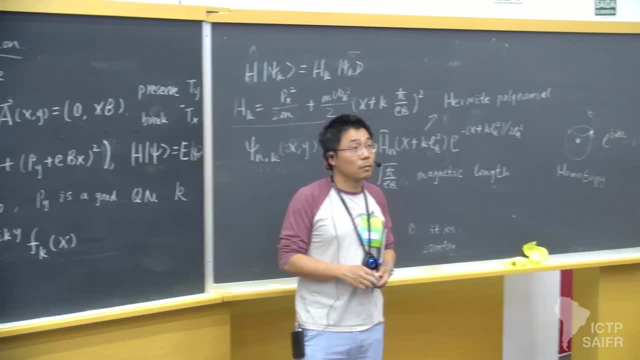 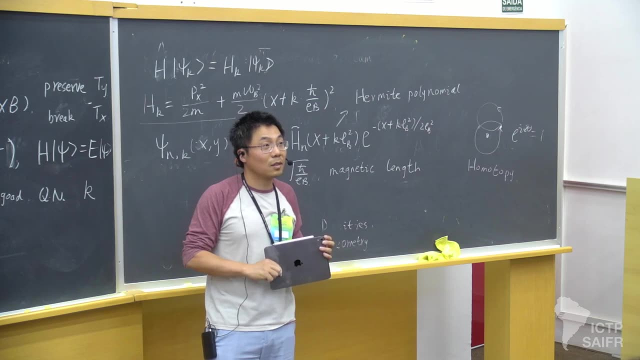 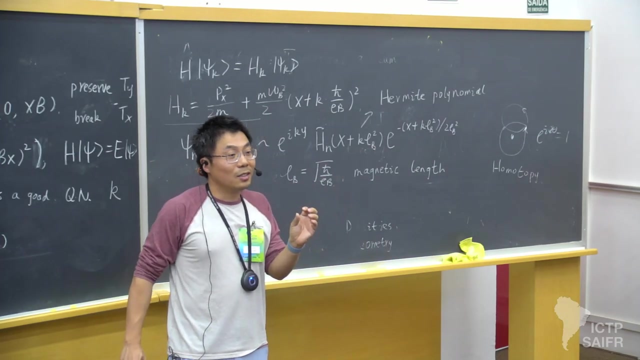 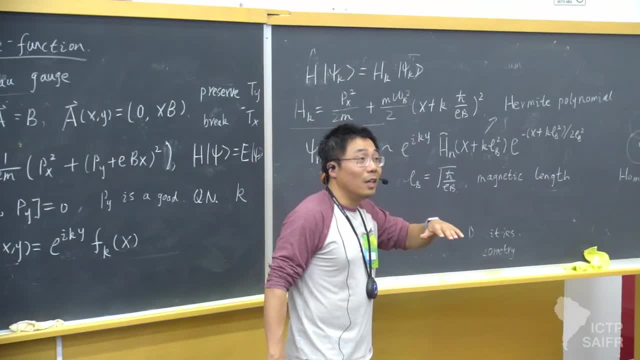 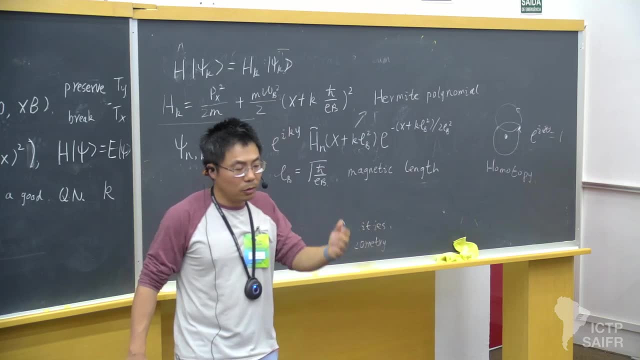 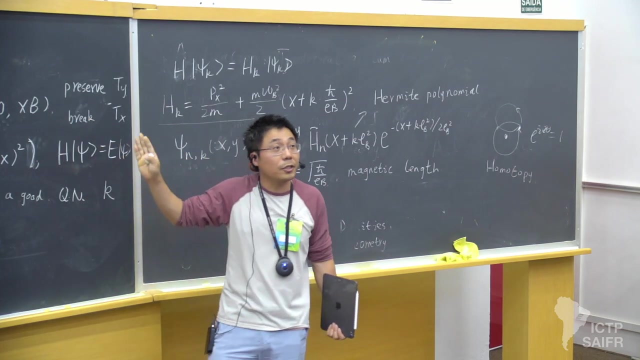 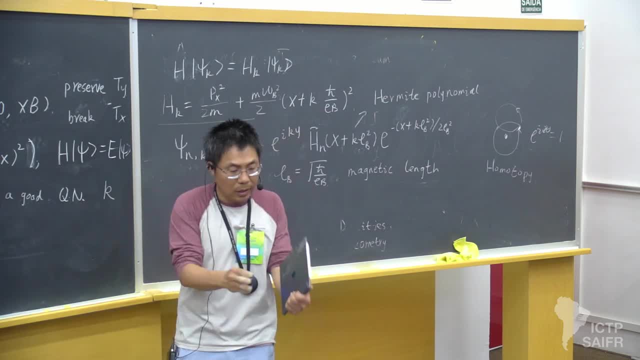 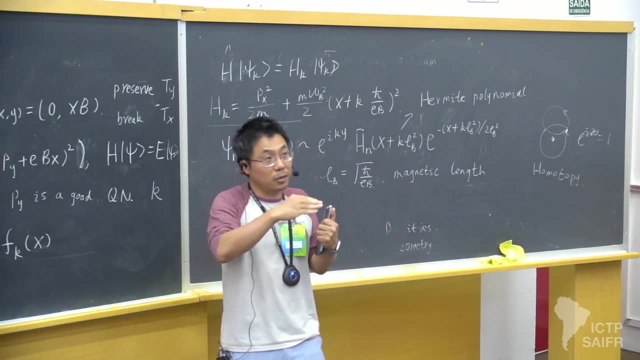 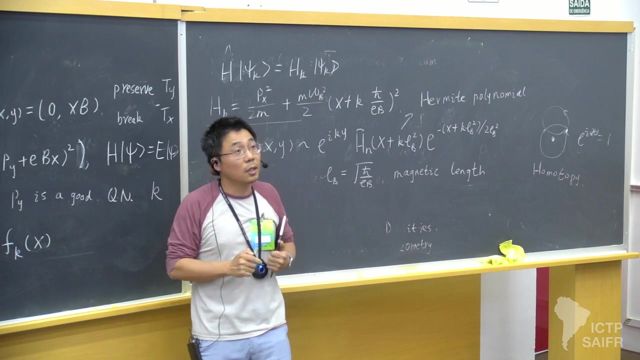 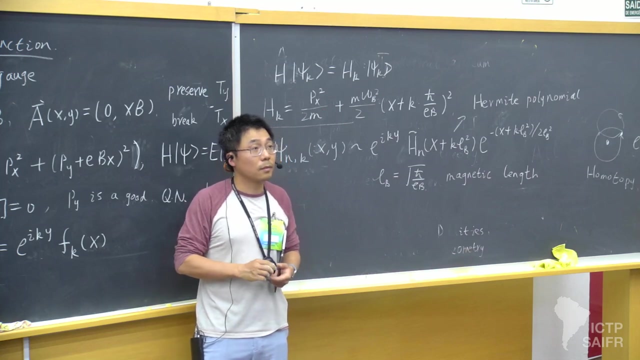 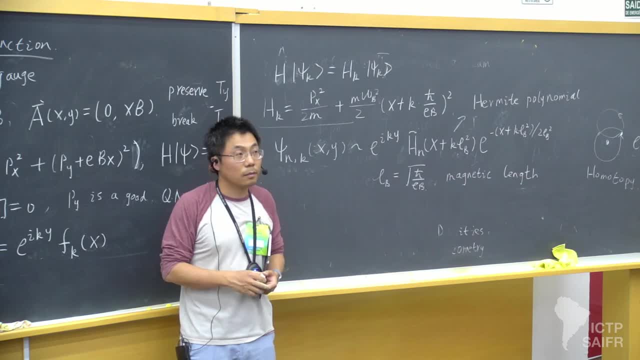 Thanks, Thanks, Thanks, Thanks, Thanks, Thanks, Thanks, Thank you.